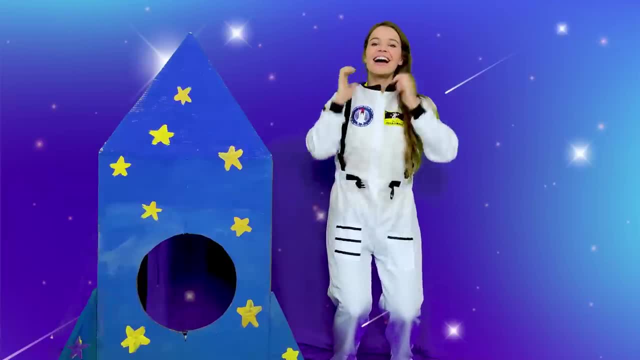 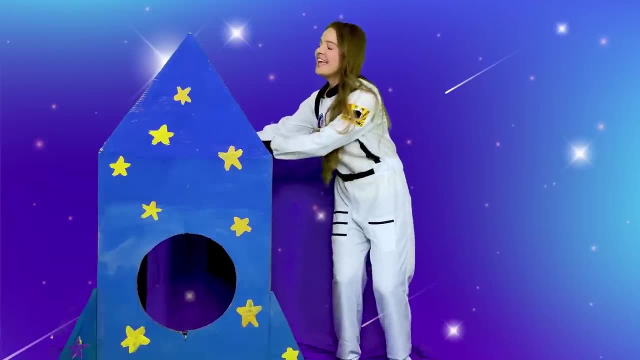 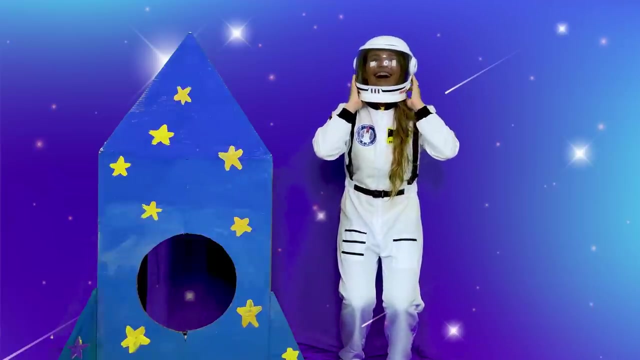 Zoom all the way up. Now I've got my space suit Buckle up And I'll need a space helmet. Here is my space helmet. I'm going to put it on, All right. All right, now we're ready to go into space. 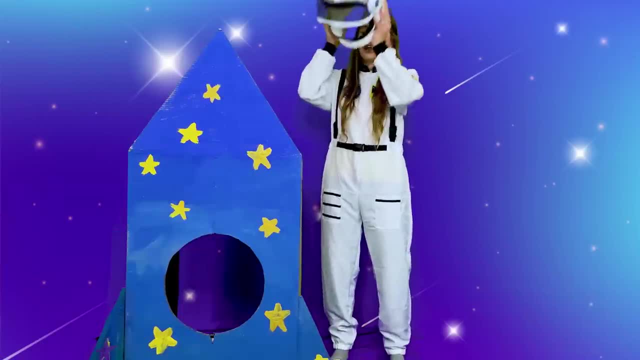 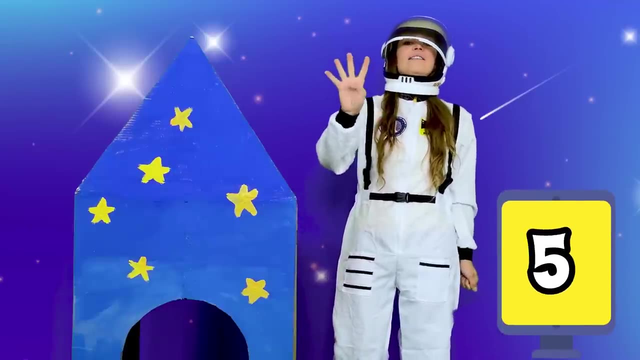 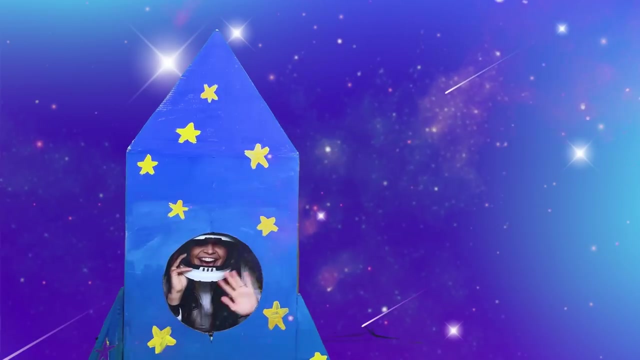 Come on, Here comes the countdown. Ten, nine, eight, seven, six, five, four, three, two, one. Blast off, Here we go. Whoa, Oh, wow, We made it to the moon. How cool. 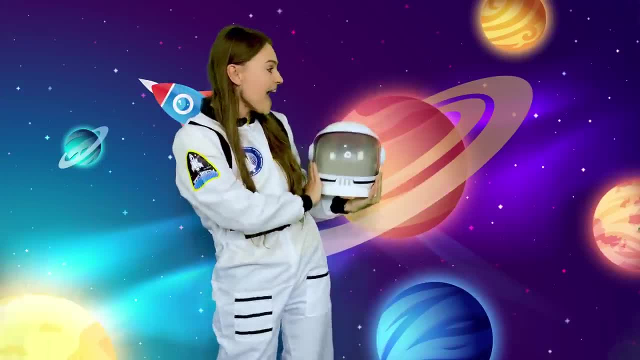 Oh, it's a little cold in space. Whoa, That reminds me of freeze dance. Should we do the moon freeze dance? All right To play the moon freeze dance when the music plays. we're going to do the moon freeze dance. 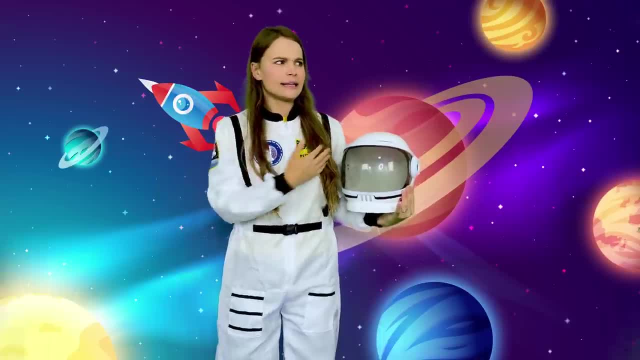 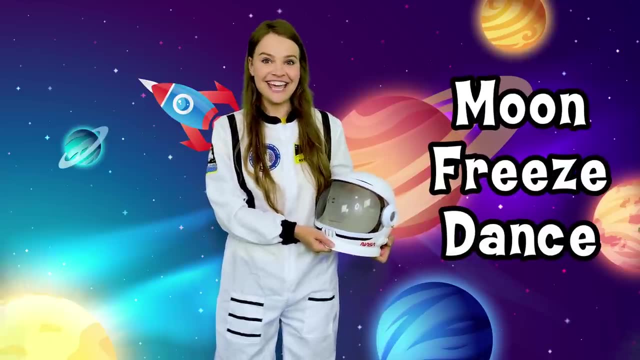 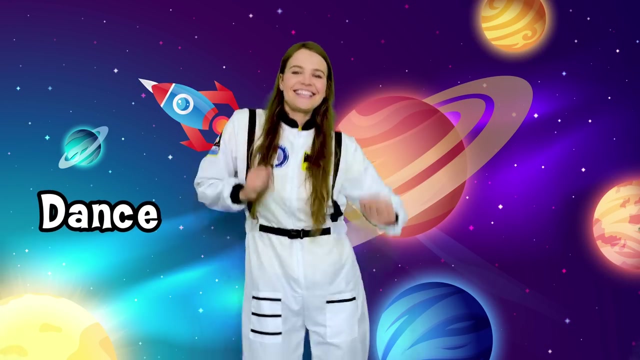 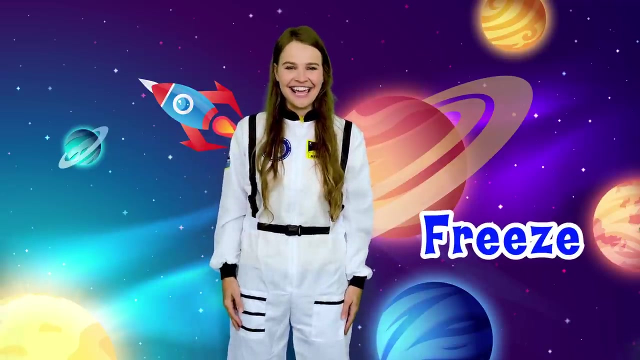 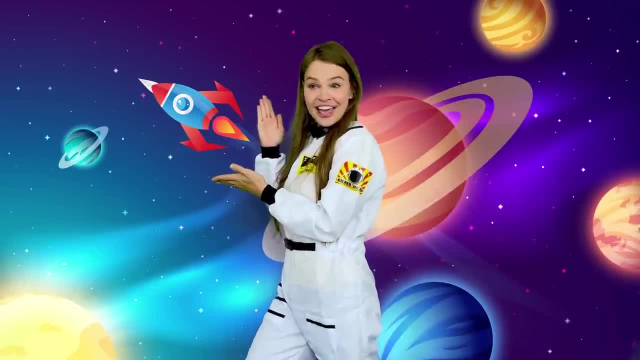 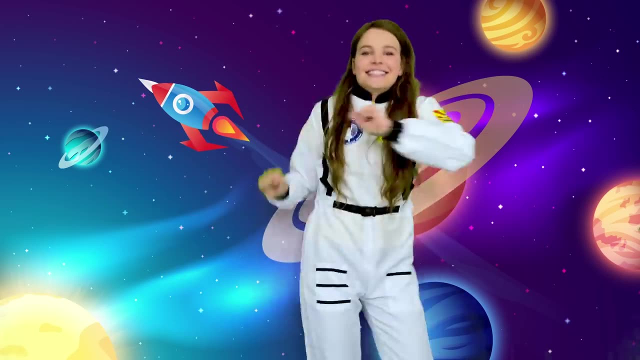 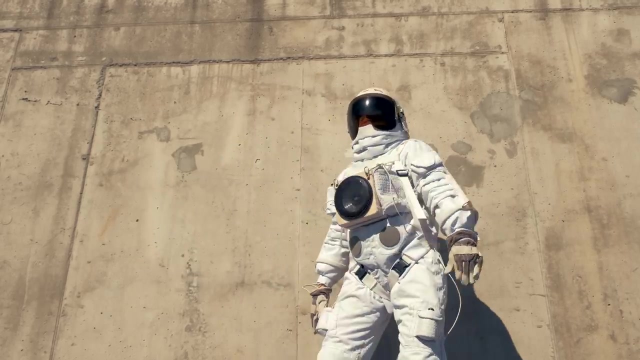 Doot, doot, doot, doot, doot, doot And freeze. Did you freeze? That was sudden. Let's do it again. Let's dance, Dancing, dancing on the moon, Dancing, dancing on the moon. 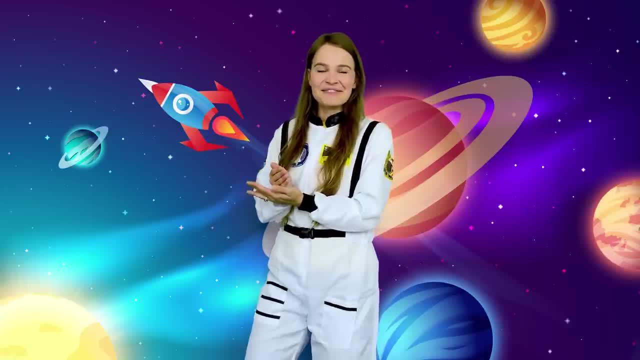 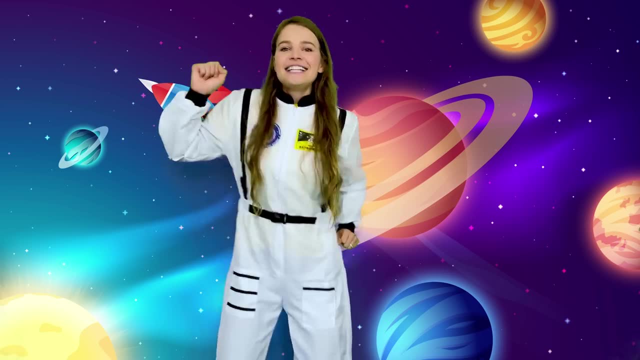 Dancing, dancing on the moon Freeze. Whoa, That was sudden. Was that surprising Freeze? Did you freeze? Good job. Okay, let's do it again and we'll dance one more time. Are you ready? Dancing, dancing on the moon Dancing. 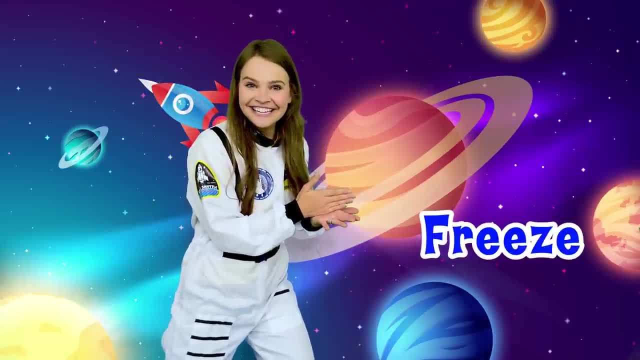 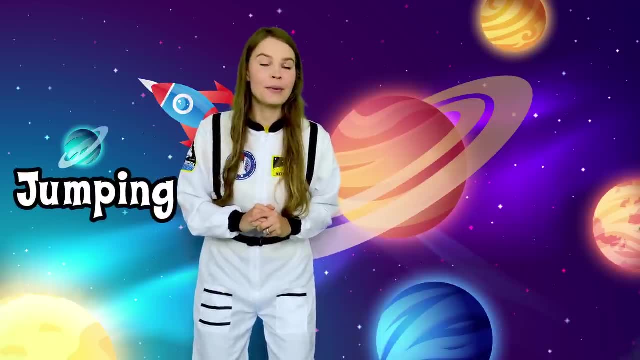 And freeze. Wow, Did you freeze? Oh, that was sudden and fast. Now let's do jumping. When the music plays, we're gonna jump, jump, jump. But when it stops we're gonna freeze. You ready, Let's jump. 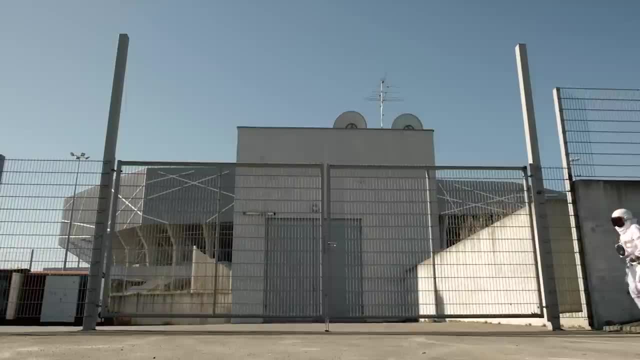 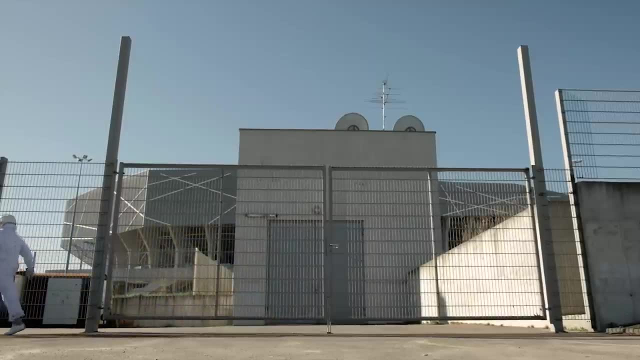 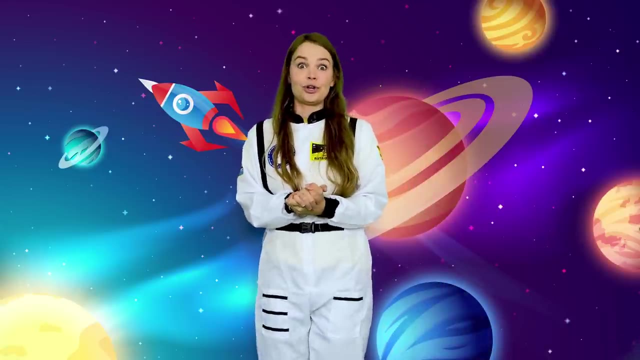 Jumping, jumping on the moon, Jumping, jumping on the moon. And freeze. Did you freeze? Great job. Now let's do stomping, Stomping, stomping on the moon, Stomping, stomping on the moon. 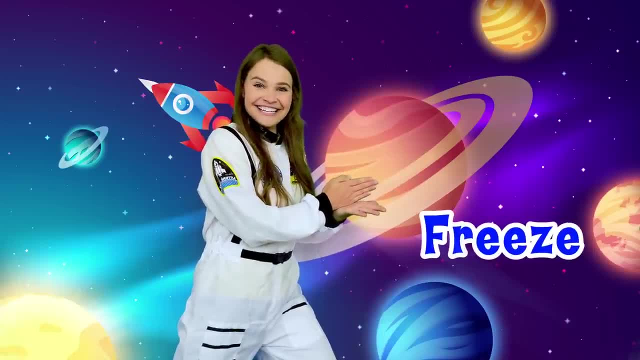 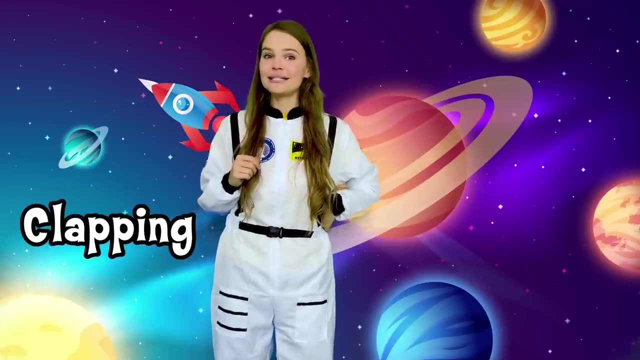 And freeze. Did you freeze? Great work. Now let's do ooh clapping. When the music starts, we're gonna clap, clap, clap. But when it stops, we're gonna freeze. You ready, Let's clap. 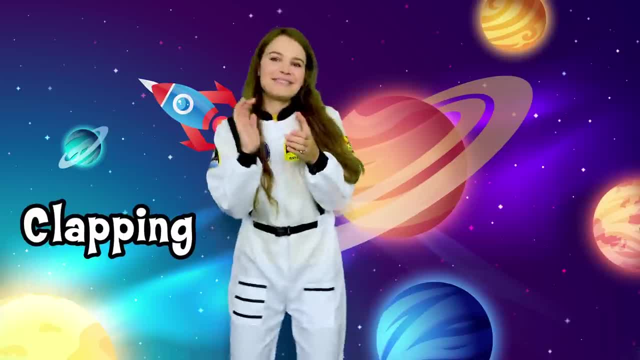 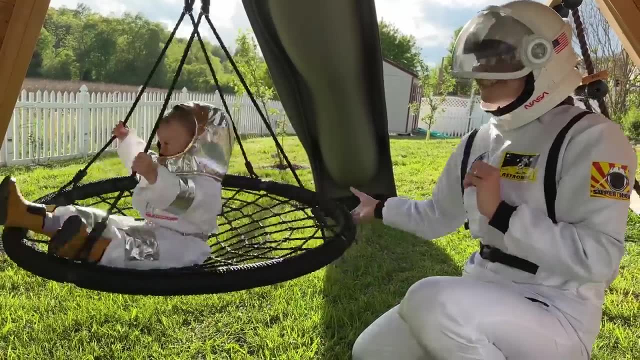 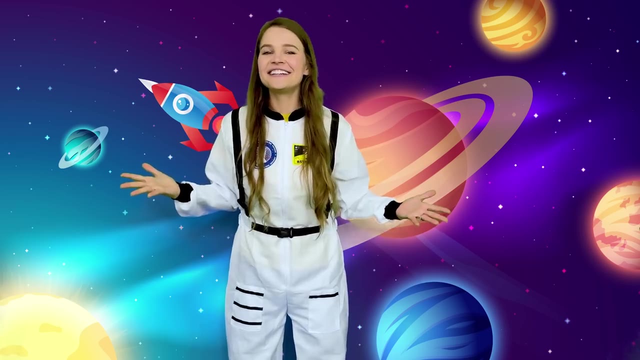 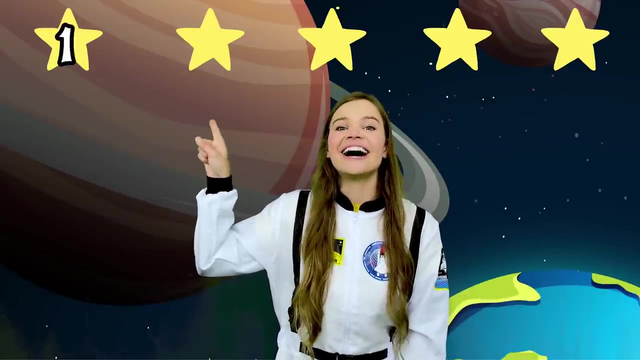 Clapping, clapping on the moon, Clapping, clapping on the moon And freeze. Did you freeze? How silly. Thank you for dancing with me. Will you help me count these stars? We've got one star, Two stars. 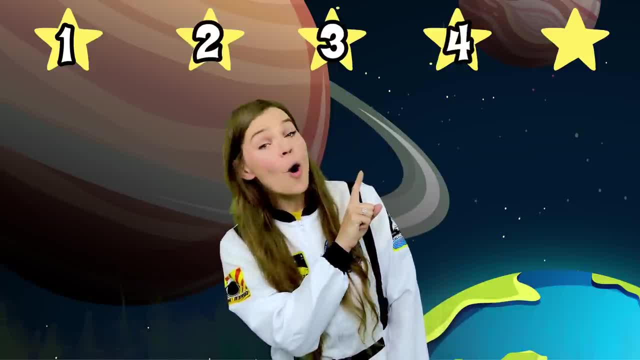 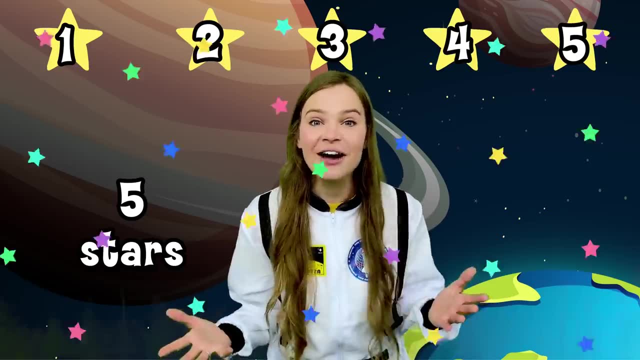 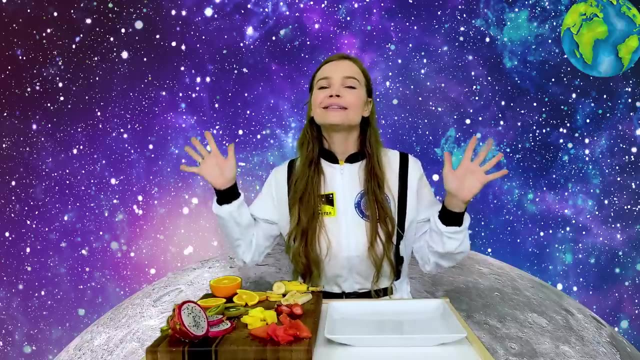 Three stars, Four stars And five stars, Five stars. Thank you for helping me count. Wow, all of this dancing and playing sure made me hungry. Let's make a little out-of-this-world space snack. I've got some fruits and a plate. 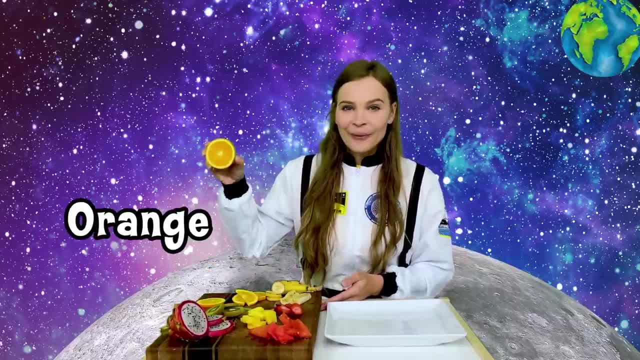 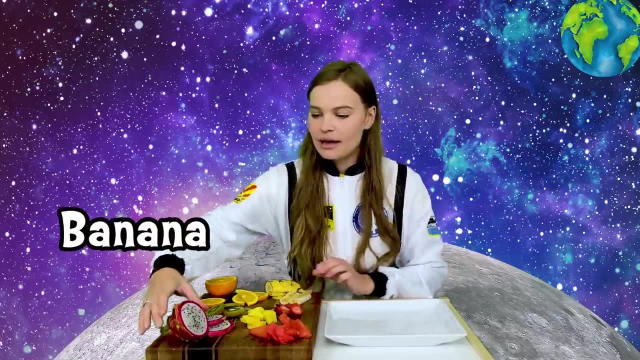 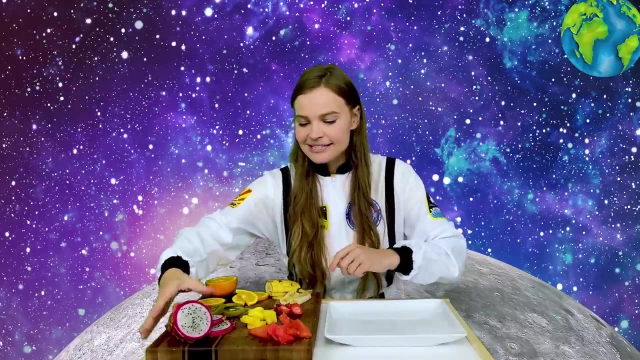 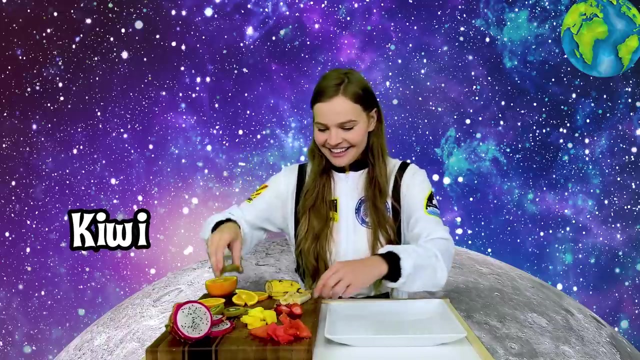 Let's see what kind of fruit we've got. I've got an orange, Some banana. I also have a dragon fruit that's round. It has little seeds inside. I've got some pineapple, Watermelon, Kiwi And strawberry. 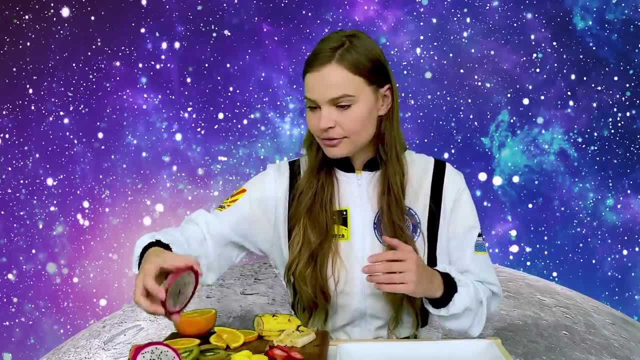 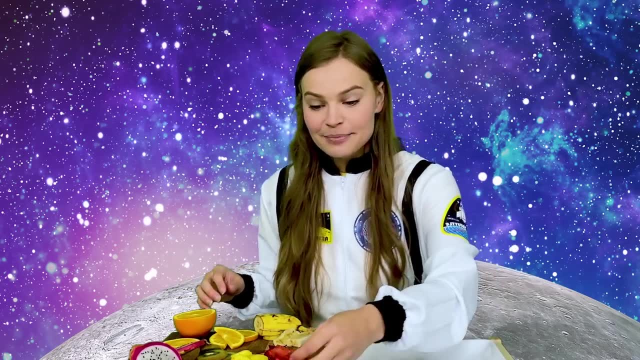 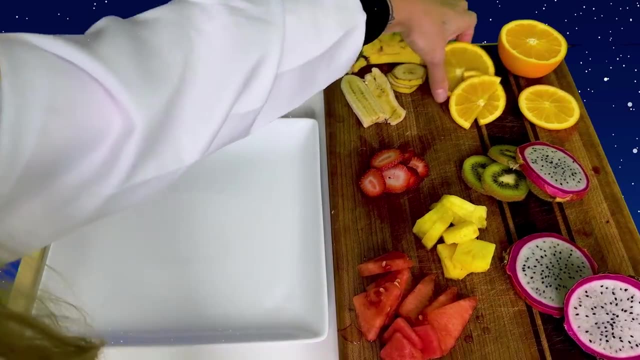 And they're all cut up in different shapes. I've got some fruit that are circles And some that are triangles. Let's put them together And make a really fun snack. Let's make our space snacks. I'll use this orange as the sun. 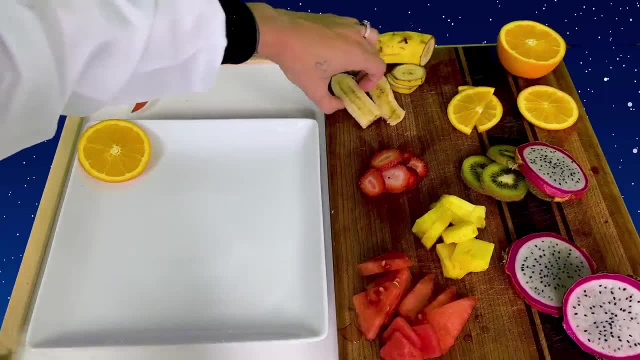 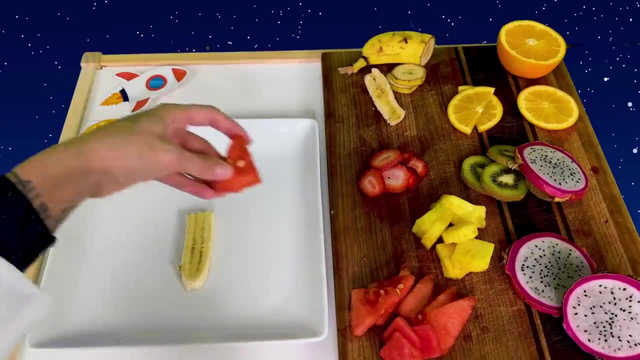 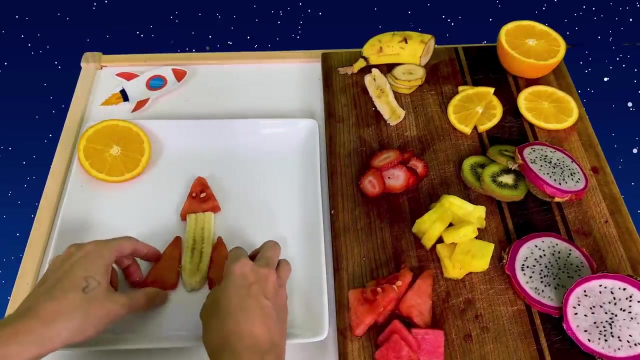 Here we go, And we can use this piece of banana as a rocket ship. Hmm, We need to put a little triangle up top. Here we go, And let's put two more triangles on the side of a rocket, And we'll need something like this: 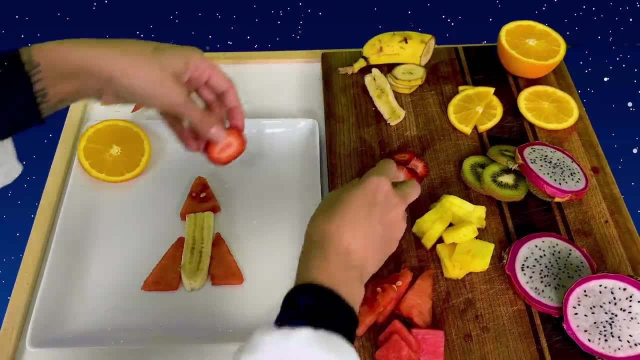 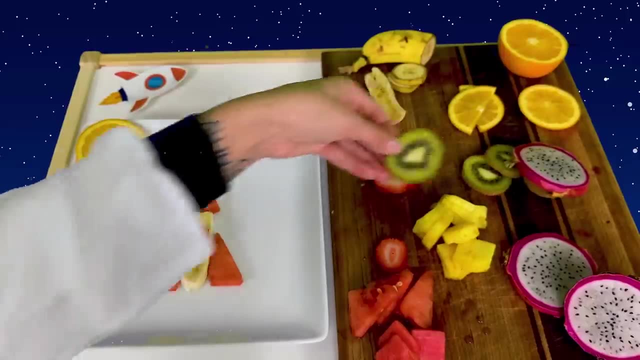 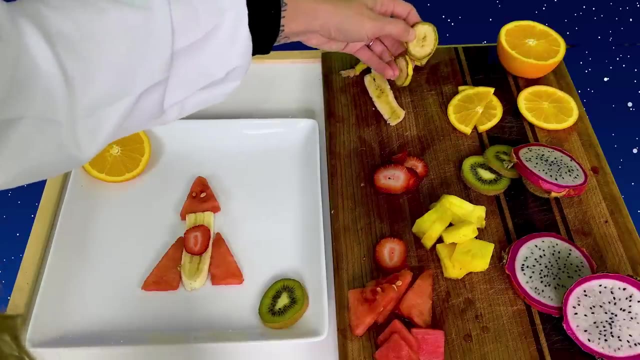 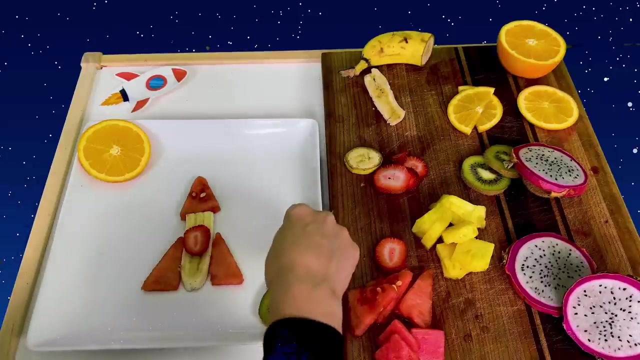 And some windows. How about? How about this strawberry window? That's cute. We can pretend that this kiwi is planet Earth. How about this slice of banana? We can pretend that this banana is the moon. Here we go, Little moon. 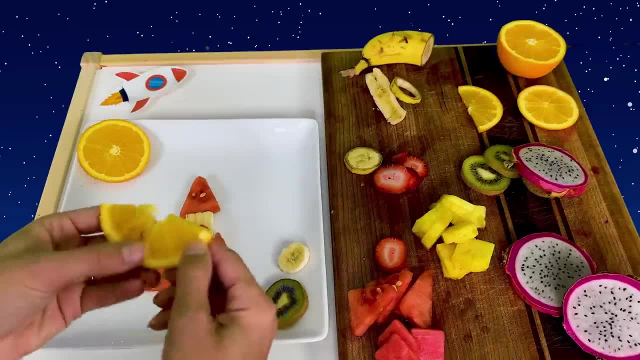 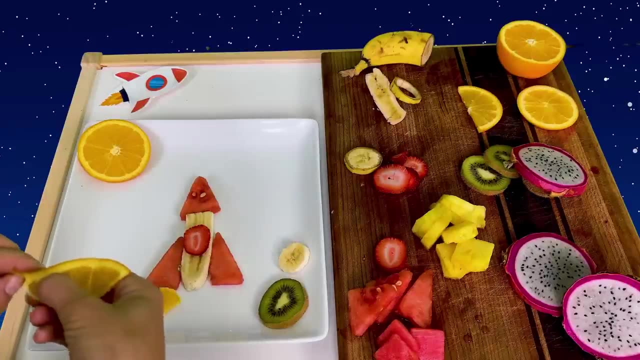 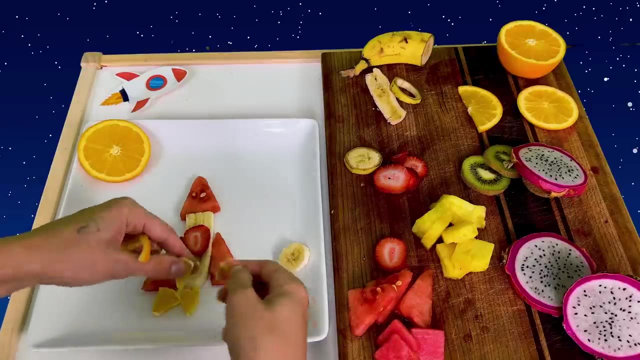 Now, when we go on, our blast off our rocket would have some fire And we can use these orange pieces as the flames. Here we go, Here we go, Let's add a few more flames, because our rocket is fast. Let's see. 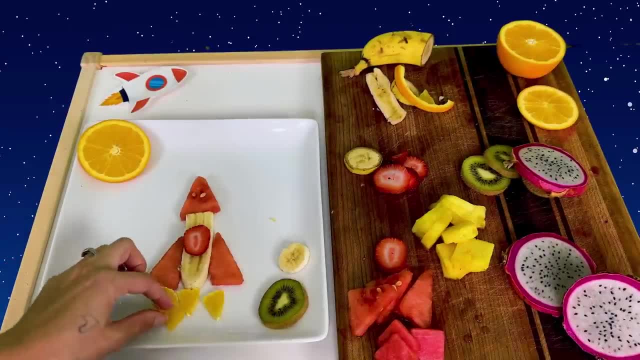 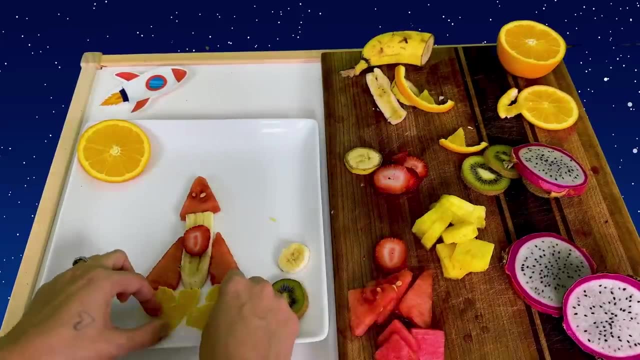 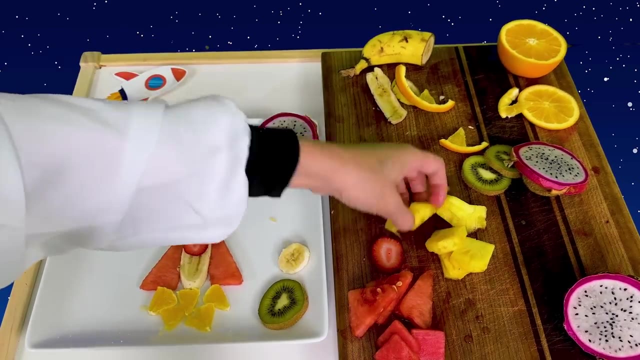 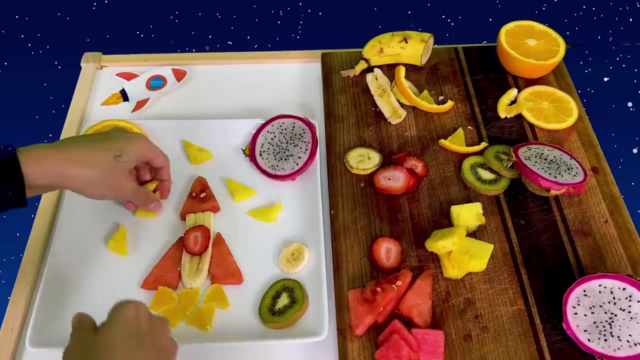 Here's a couple more triangles for our rocket. Here we go. We can also use this as a different planet out there, And we'll use our piece of pineapple as stars- Stars in the space. Here we go. Oh wow, Look at this rocket. 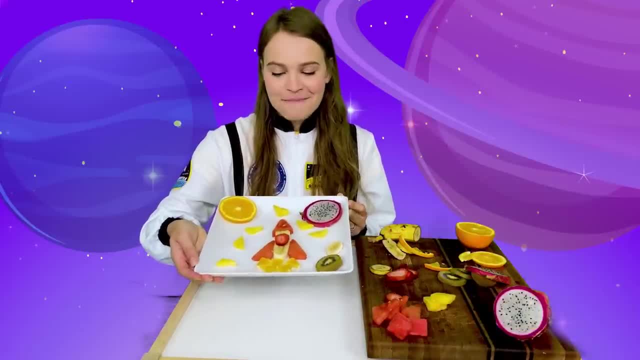 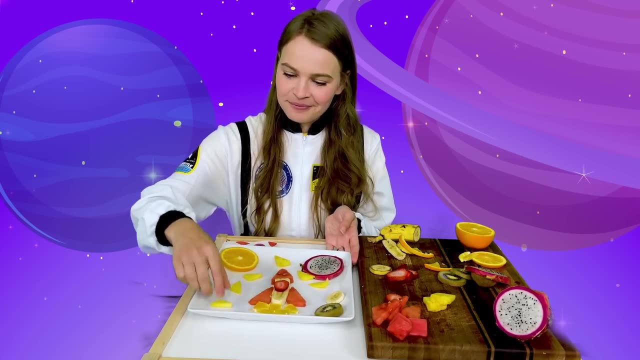 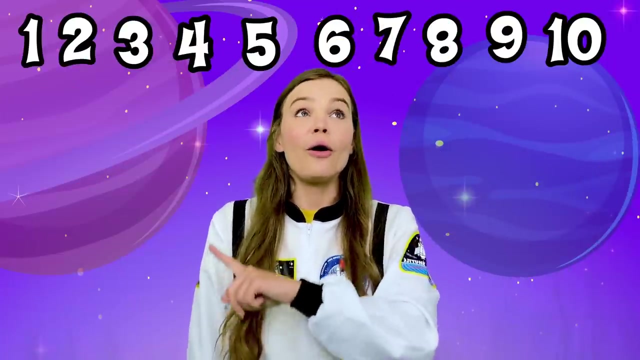 It's ready for blast off. Wow, Thank you so much for building this amazing rocket snack with me. That's going to be perfect, to give us lots of energy so we can play some more. Will you help me count to 10?? First, I want to count all the way to 10.. 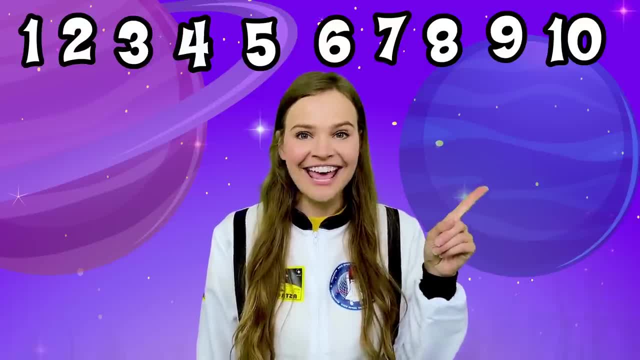 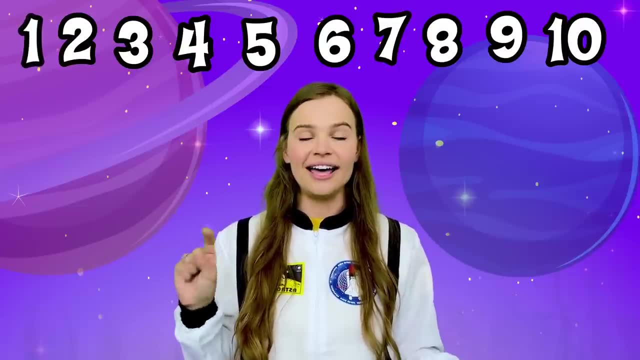 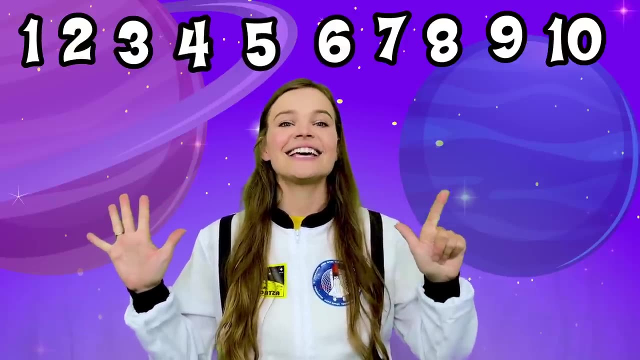 And then we're going to count backwards from 10 all the way to 1.. Let's do it. We can use our fingers on our hands: 1,, 2,, 3,, 4,, 5.. 6,, 7,, 8,, 9,, 10.. 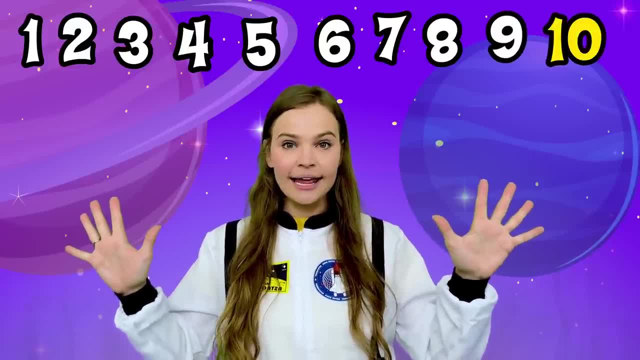 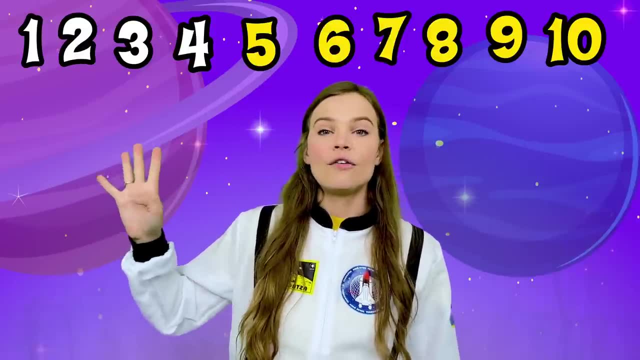 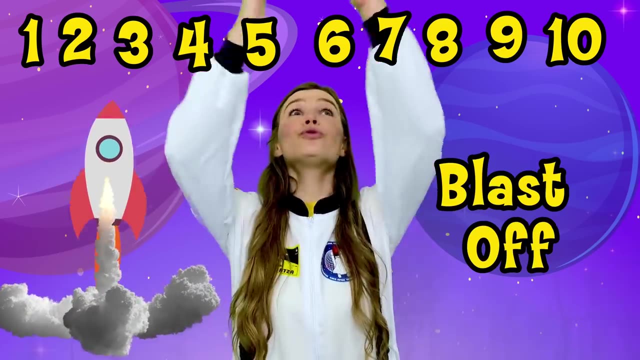 Now let's count backwards: 10, 9,, 8,, 7,, 6,, 5,, 4, 3, 2, 1.. Blast off, Let's make a rocket together out of these shapes. Let's see. 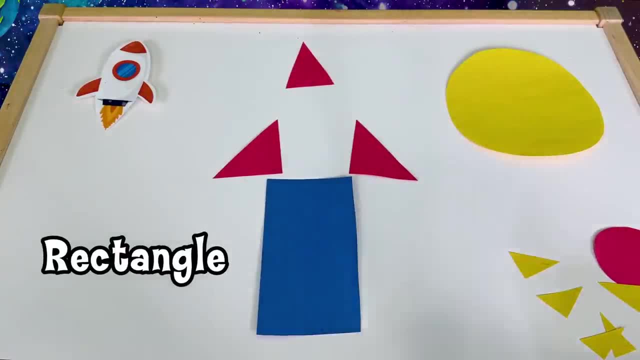 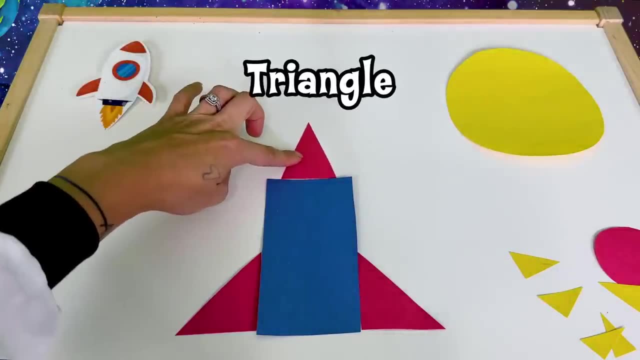 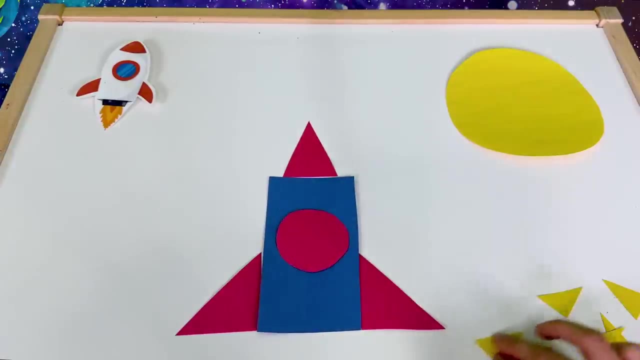 We'll make the main cabin out of a rectangle And I'll put two triangles on the side for the support. Here's another triangle to put at the top And we'll put a window right here. We can use these little yellow triangles as our fire that's coming off during blast off. 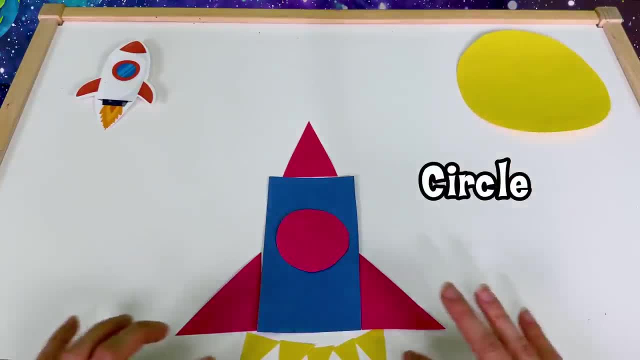 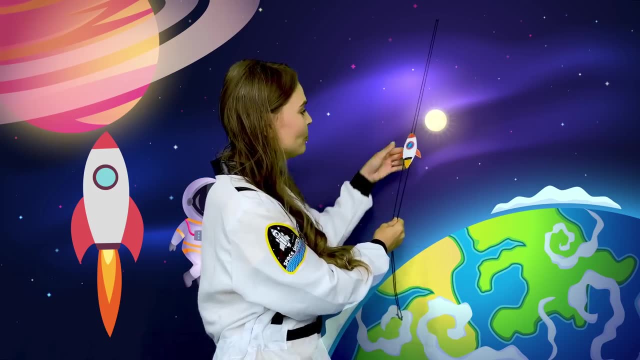 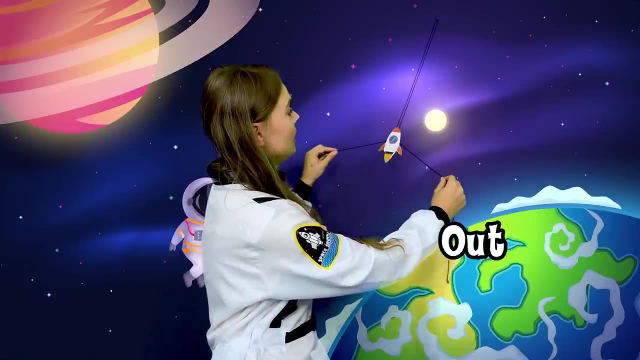 Here we go, And this big circle is the sun. We're ready to go. Thanks for helping me make a rocket. Here's a fun activity you can play at home. You just need a little rocket and some strings and straws, And as you pull the strings out, the rocket is climbing up. 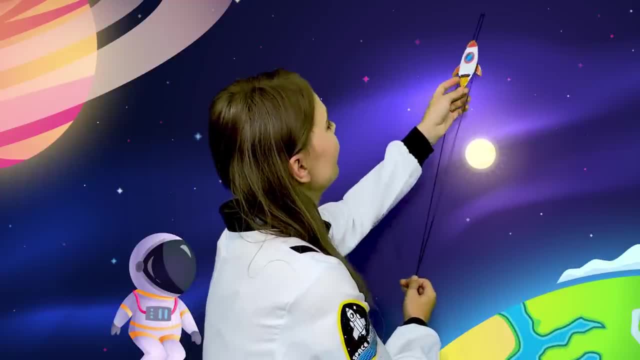 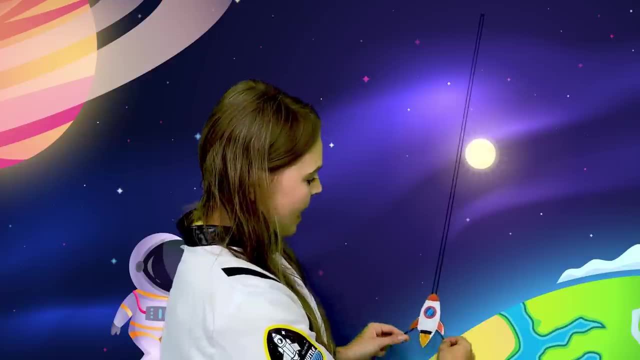 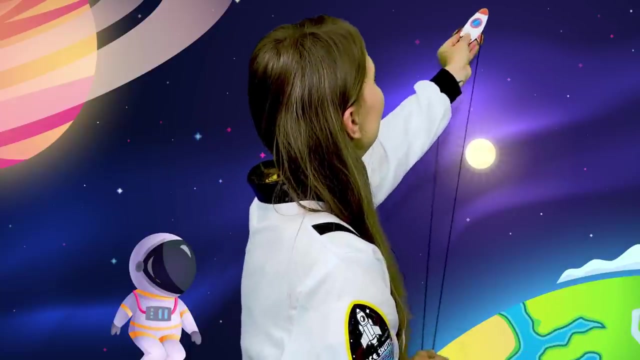 When you bring them together, here we go. your rocket will slide down. Let's do it again. Out and it climbs up. You got a little rocket, And here we go. When we put the strings together, it can slide down. 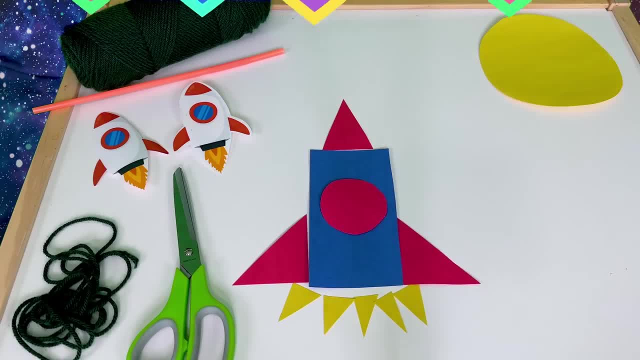 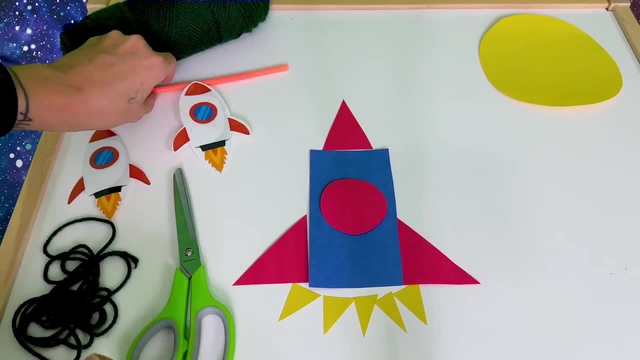 Let me show you how you can make this activity at home. Here's how to make that activity. You can use the rocket that you make or you can print one out. You'll also need straw and some string. We'll tape the straws on the back of our rocket ship. 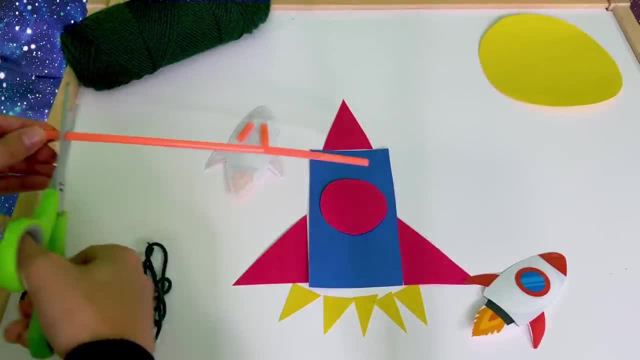 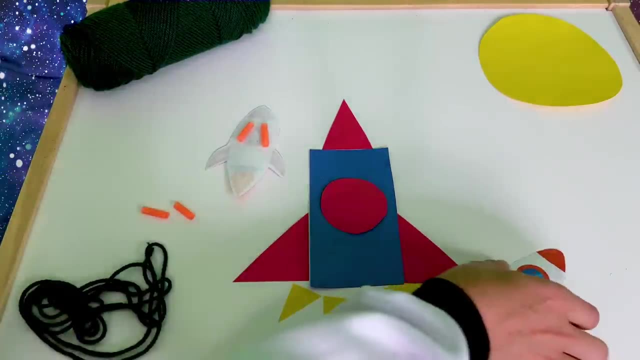 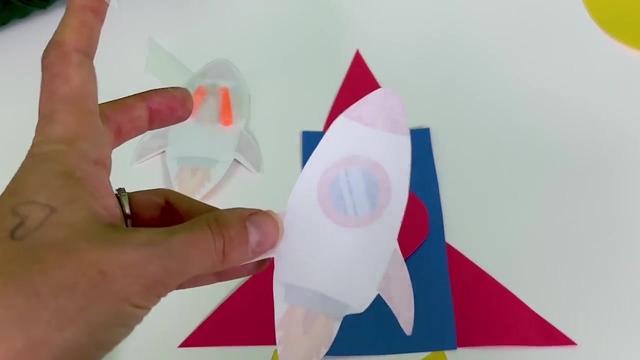 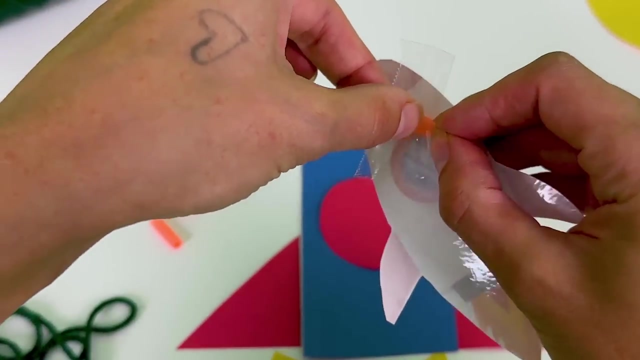 Let's make one cut, two cuts. Here we go. I want to put these straws and tape them to our rocket. Here we go. I'll put one piece of straw right here and tape it. We'll tape one piece of straw. 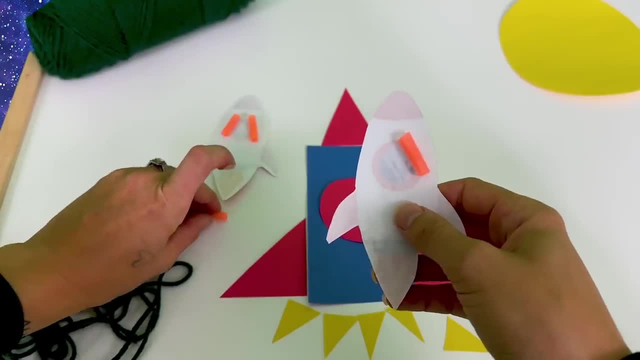 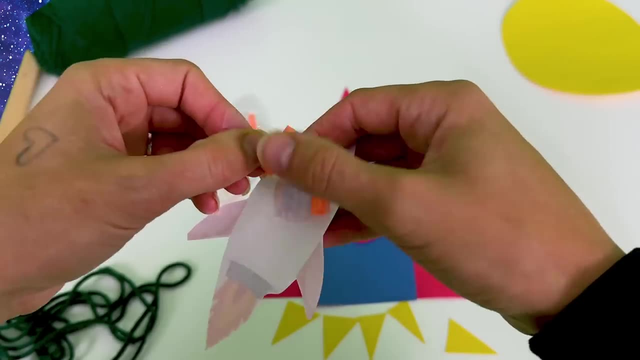 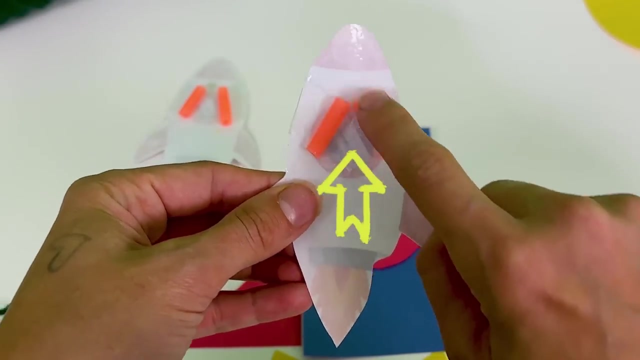 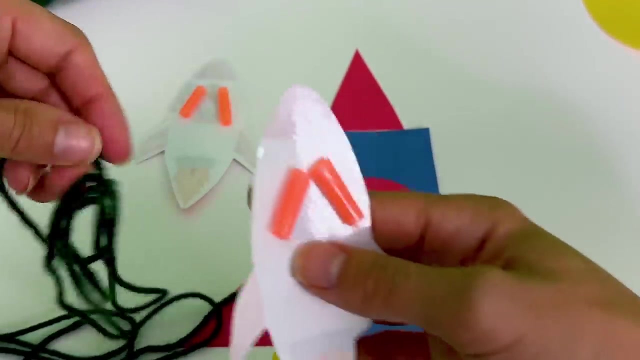 One piece of straw here and another piece of straw right here. When you tape the straw, you want to make sure they're pointing upwards toward each other, almost like a triangle would. Then you can cut a piece of string and thread it through the straw pieces. 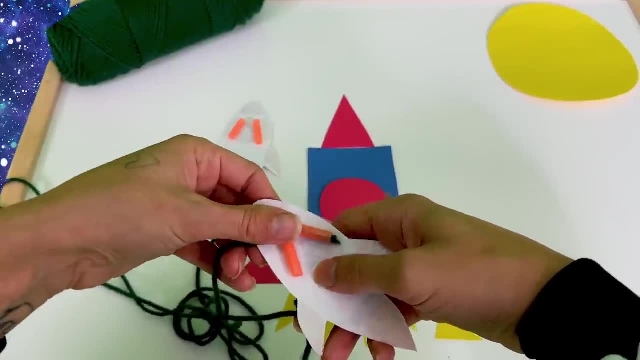 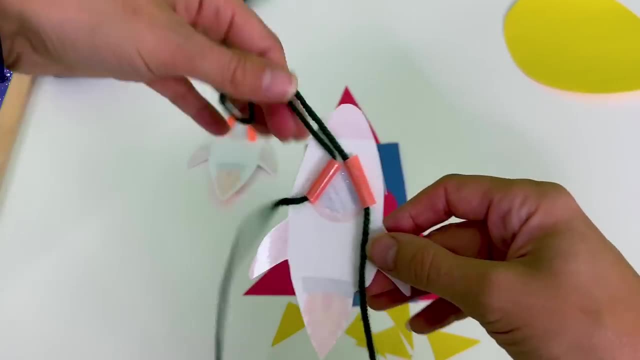 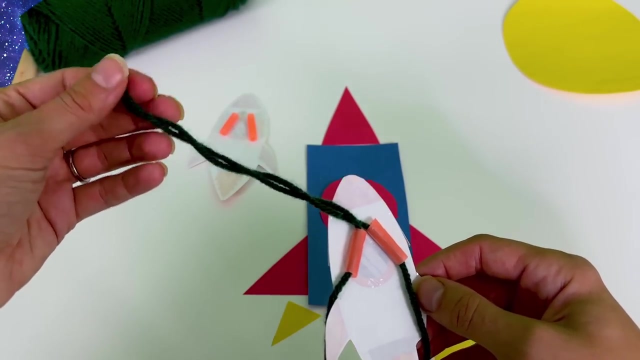 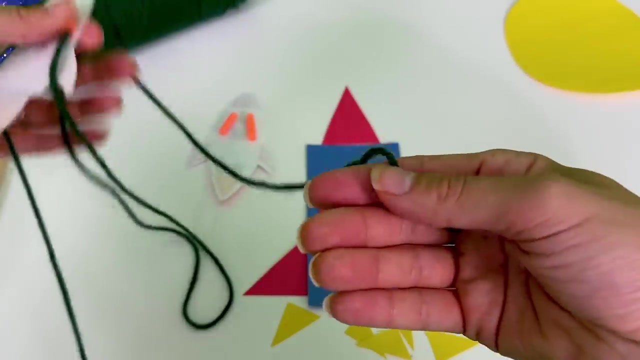 Here we go. Now we got our strings through This part. you can tie to any cabinet door or anything you can secure it to. You can even take this for a ride in your car And to make sure your ends don't come out, you can tie them up to create your little handles. 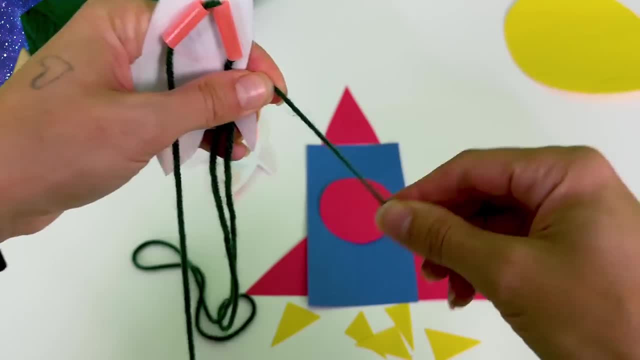 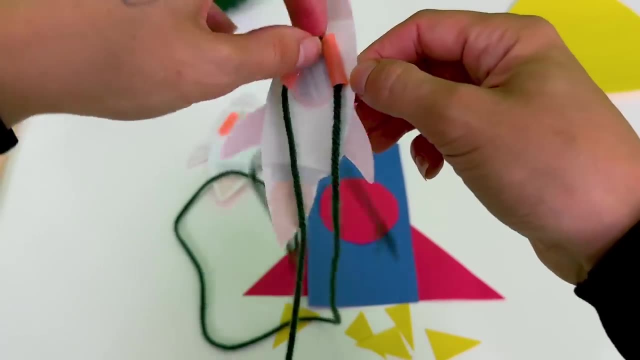 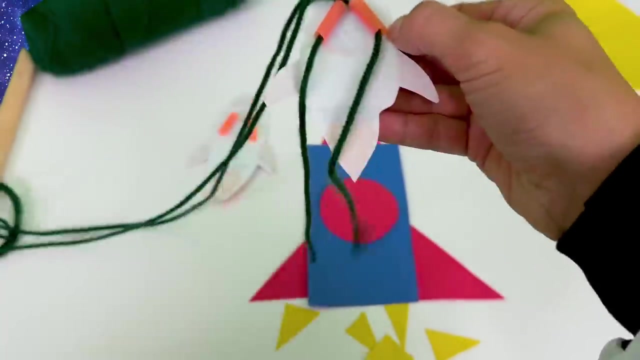 Or you can also tie something at the end of it, like a hair tie, something big enough that won't fit through when you're pulling it back. That way they don't come out for you. There we go. Now do the same thing on the other side and you'll be ready. 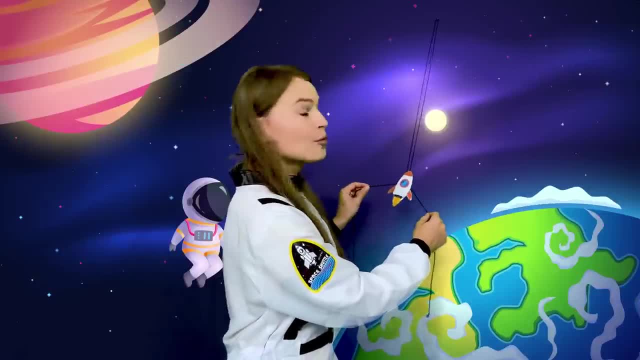 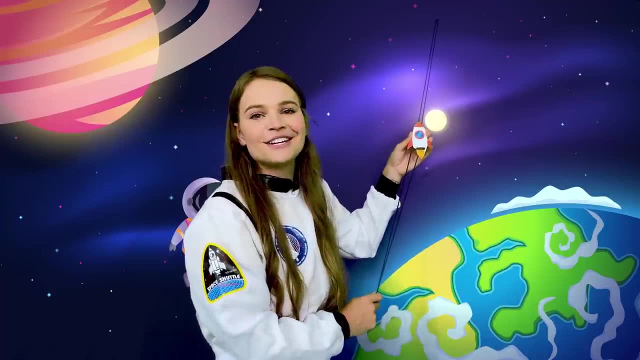 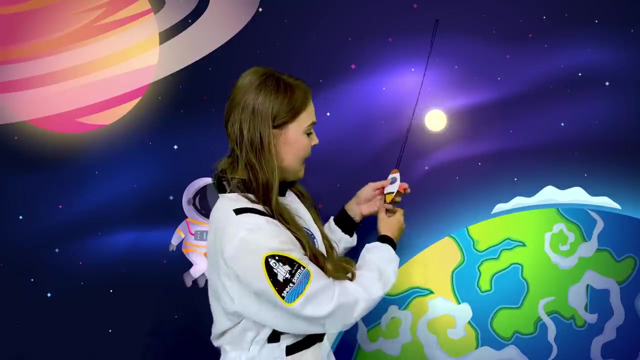 You can make tons of different rockets and then race them with your family or friends, And you can also do this with any other picture. You can use a picture Of an animal that goes up really fast, Or you can put a picture of yourself in this rocket and see yourself blast off. 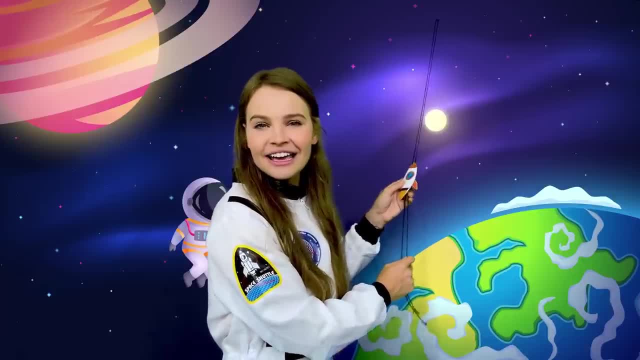 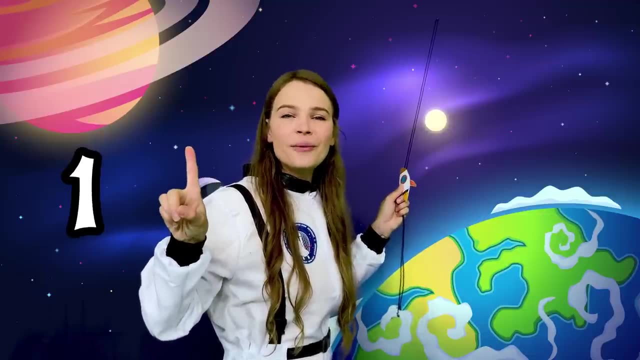 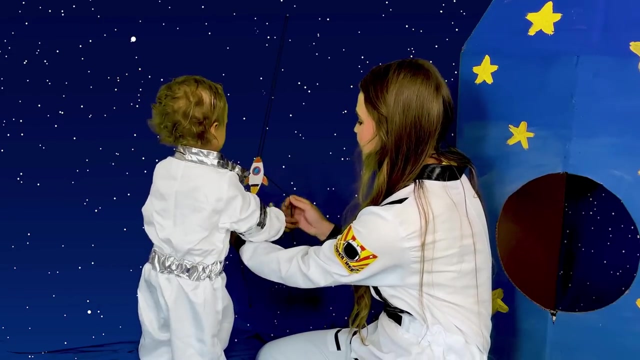 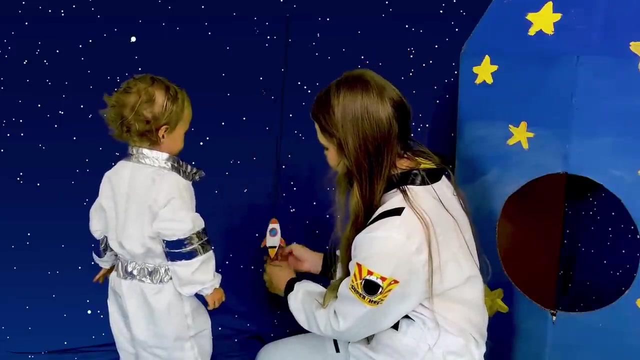 Let's count down from five and we'll make our rocket fly Ready. Five, Four, Three, Two, One Blast off. Wow, You remember it Ready. Pull them up. Wow, Rocket, Bring it together, Get ready. 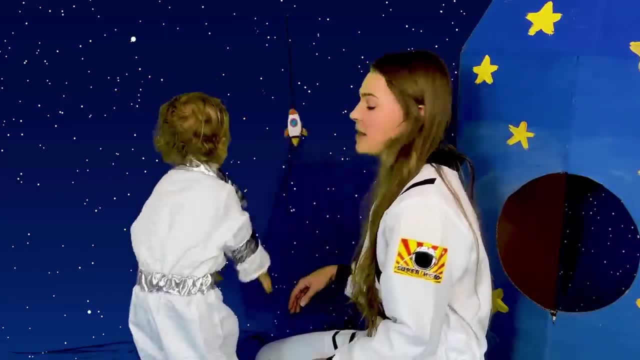 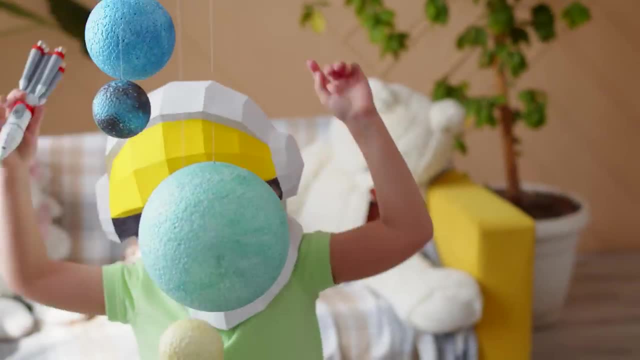 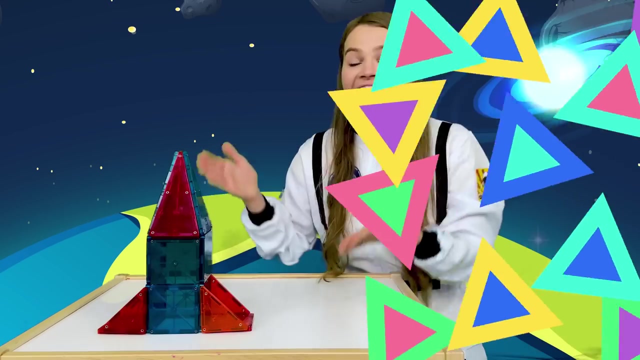 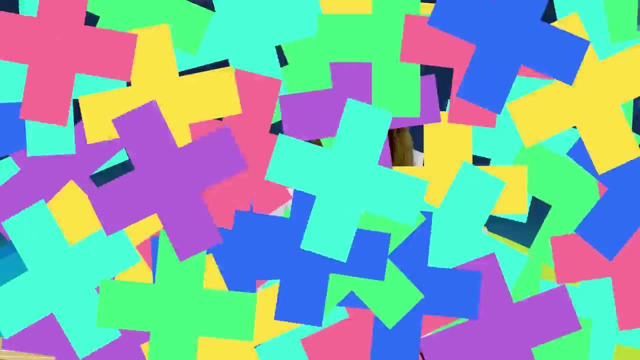 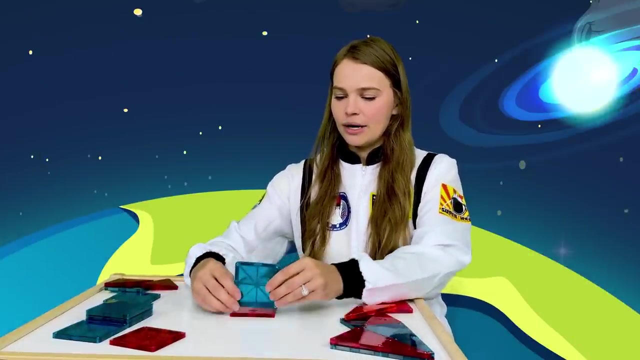 And pull it up again. Yay, You got a little rocket. How about this rocket? You can build a rocket like this at home if you have magnet tiles. Let's build it together. Let's build a rocket together. I'll put a square as our base and another square going up so it doesn't fall. 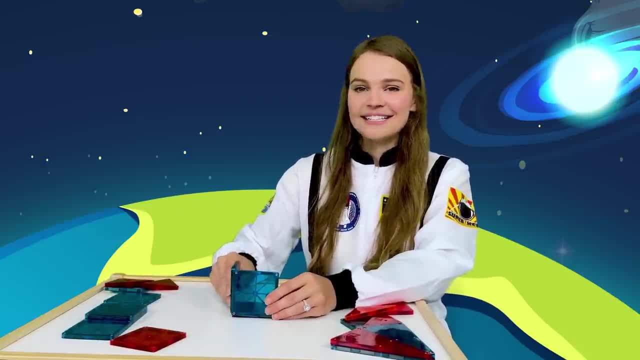 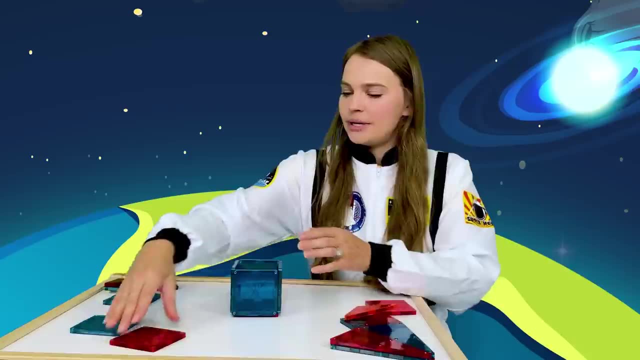 I'll use one more square to put on the side to support it. Let's add a few more squares, One on the side and one in the back. Let's put a top as our little roof and let's make it a little taller. 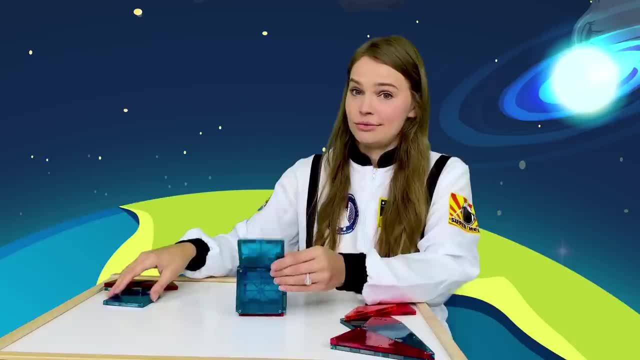 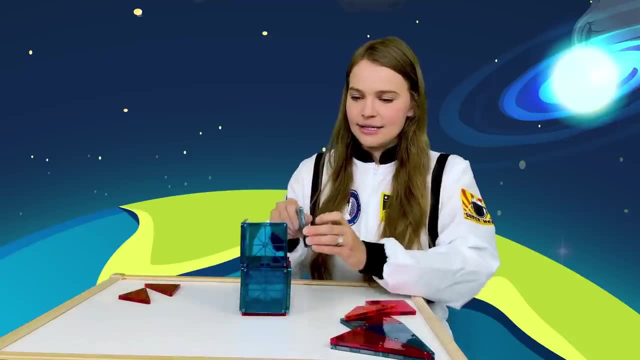 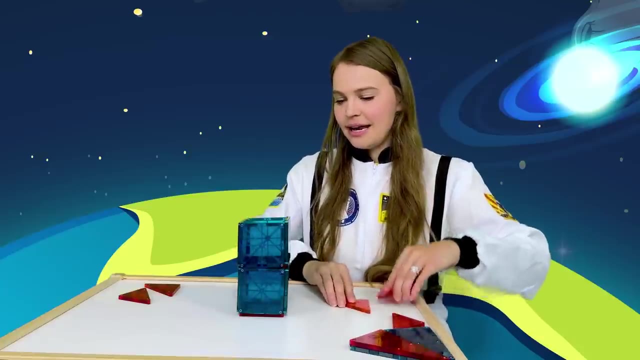 I'll add another square so it doesn't wobble or fall. I'll put one more square on the side. Let's see We'll need another square right here and one more square right there. Let's put another top on Next part we can add these triangles on the side. 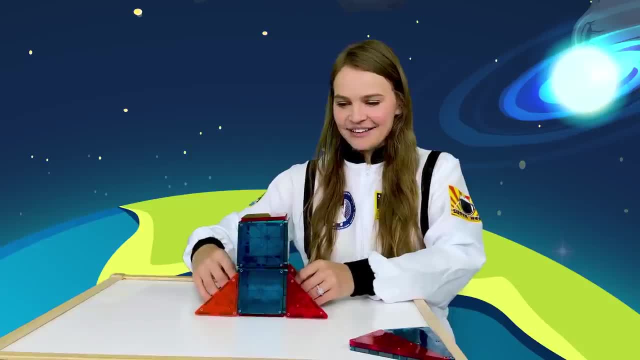 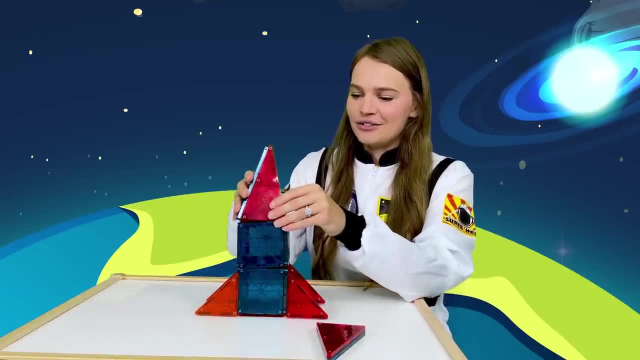 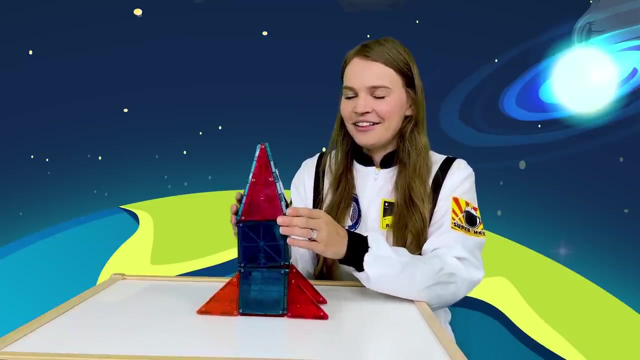 Let's do it in the front and in the back. We can also put a triangle up top here, Another triangle for support on the side, Another triangle on the side And another red triangle over here, And we've got a rocket. Where'd you go, little triangle? 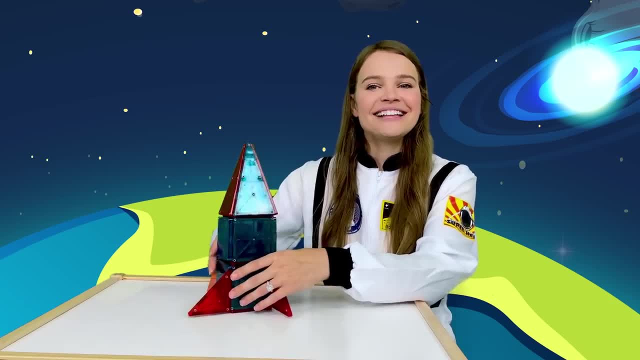 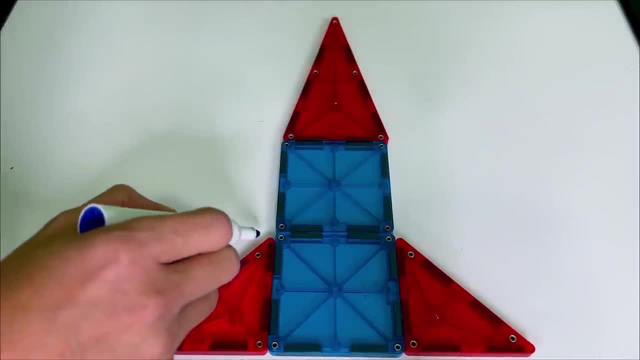 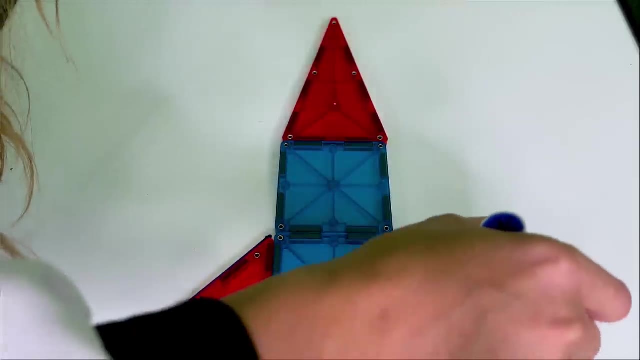 Here we go. Thank you for helping me build this. Here's another fun activity you can do at home. You can arrange your shapes into a puzzle of a rocket and then outline it with a marker To make your own puzzle. You can do this with any shapes. 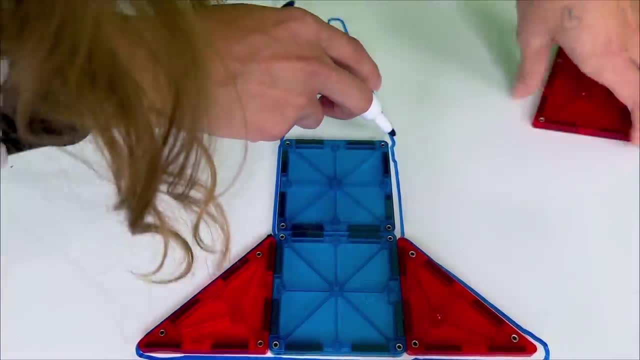 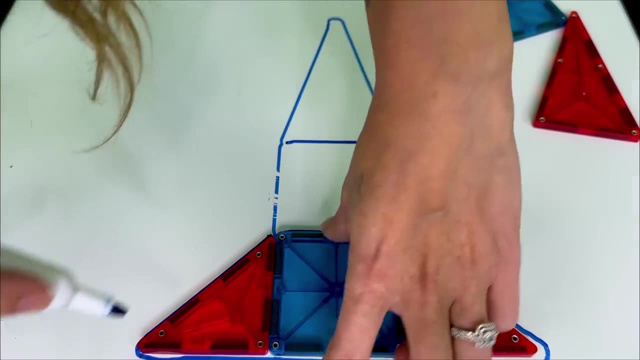 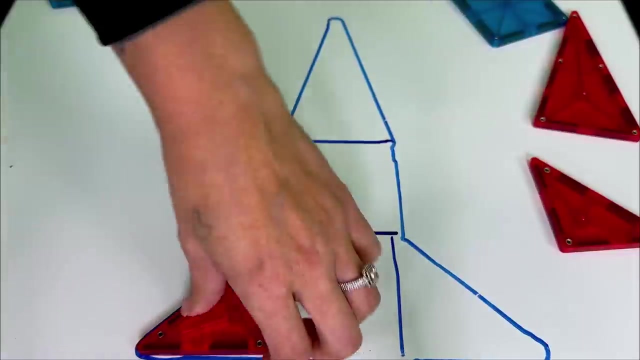 Today we're going to do it with a rocket. Here we go, Here we go. You can do this on paper or a whiteboard, so you can keep making more different shapes. Here you go. Now we made our own puzzle. Will you help me put it back together? 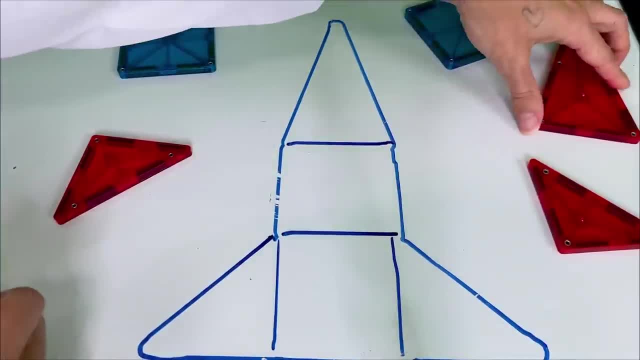 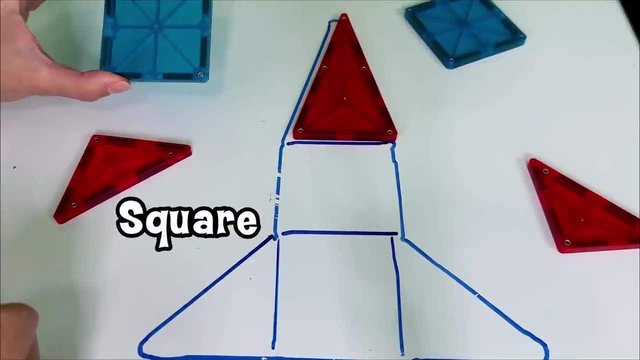 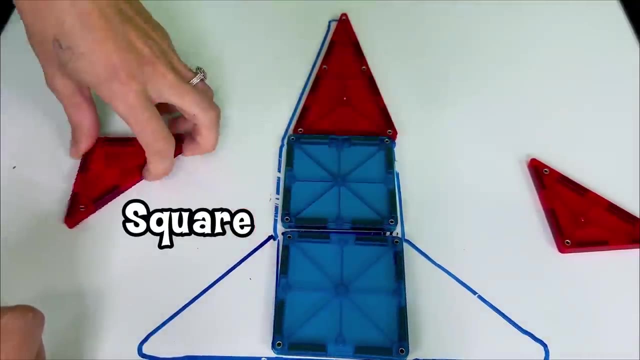 Let's see What goes up here. A triangle, All right, Here we go. And what about this spot? What should we put there? A square, Here we go. How about right here? Another square, How about over here? 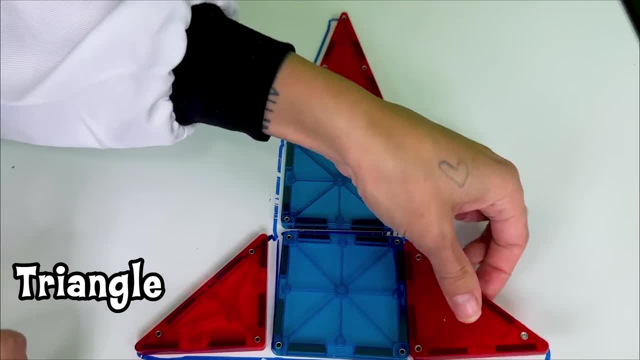 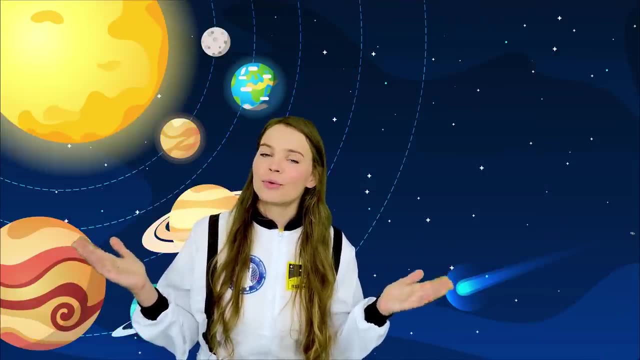 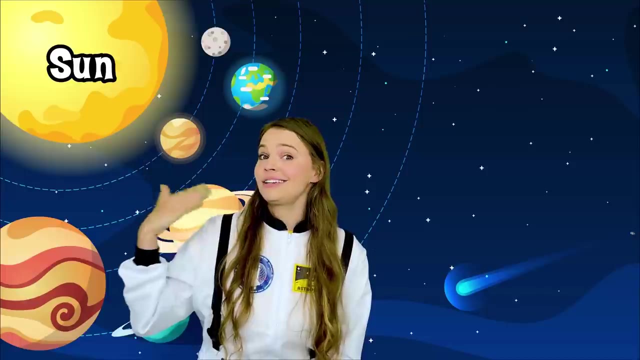 Triangle And we have one triangle left right here. Thank you for helping me with this puzzle. There are so many things out there in space. It's hard to see them when we're here on Earth. Our planet is called Earth. When we look up, we see the sun, and it makes it really hot during daytime. 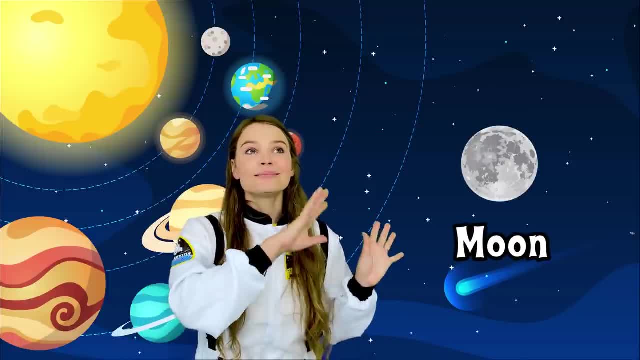 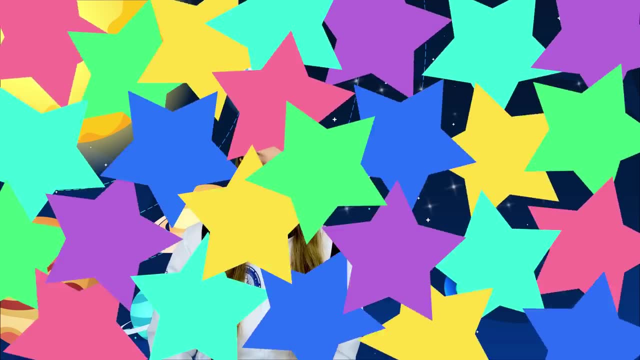 We also see the moon. when it's nighttime, The moon comes out and we can also see lots of little stars twinkling, twinkling. Let's sing twinkle little star together. Put your hands out and wiggle them around like twinkling little stars. 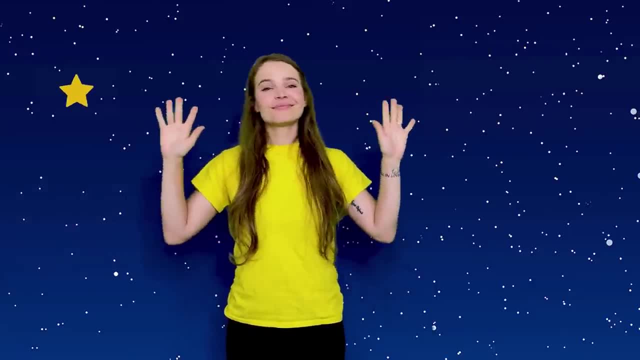 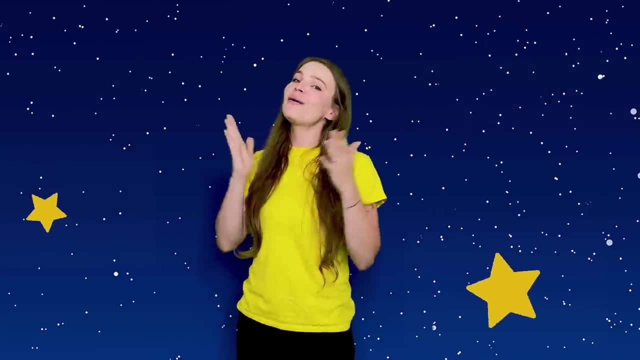 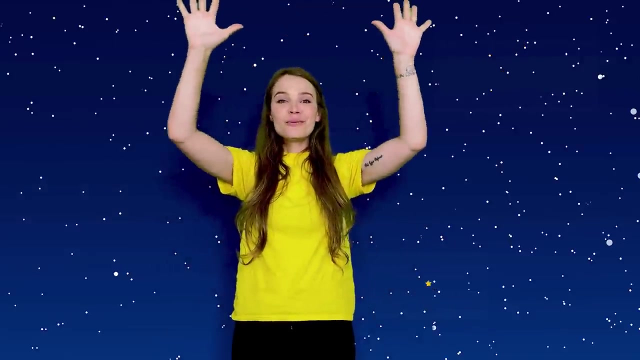 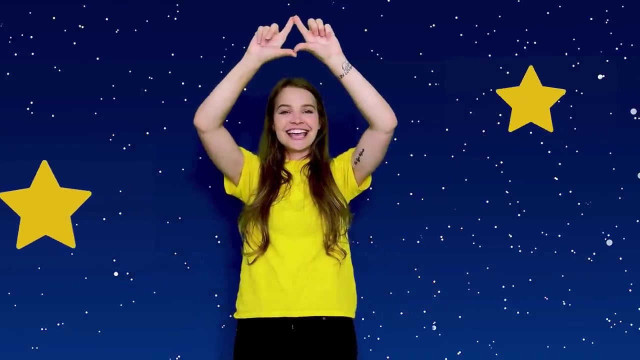 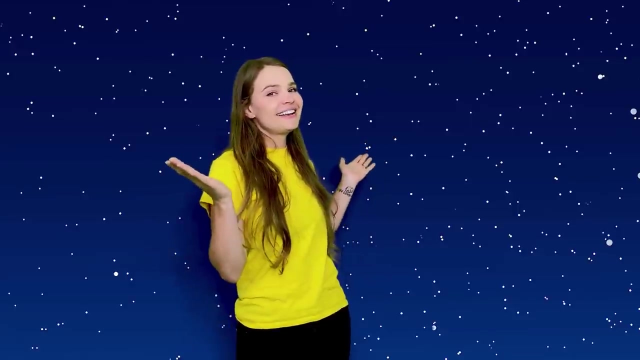 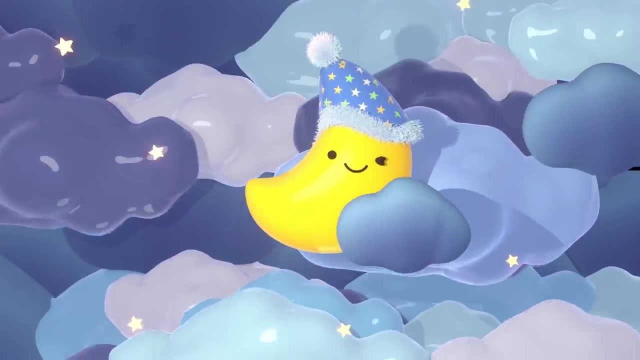 You ready? Twinkle, twinkle little star. How I wonder what you are, Up above the world, so high Like a diamond in the sky. Twinkle, twinkle, little star. How I wonder what you are. Among the stars, there are many different planets, including ours. 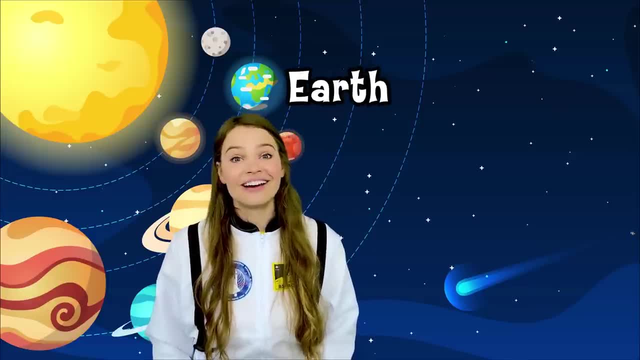 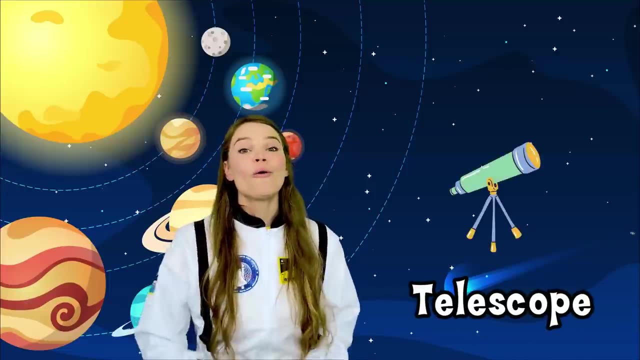 Our planet is called Earth, where we have water and land, But there are many more planets out there. To see other planets you would need a telescope. Or, if you become an astronaut, that's a person who goes up into space in rockets. 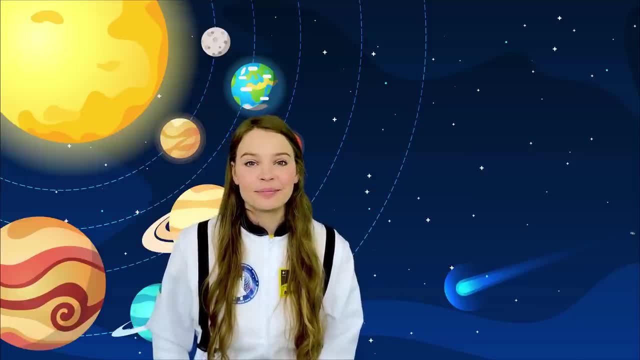 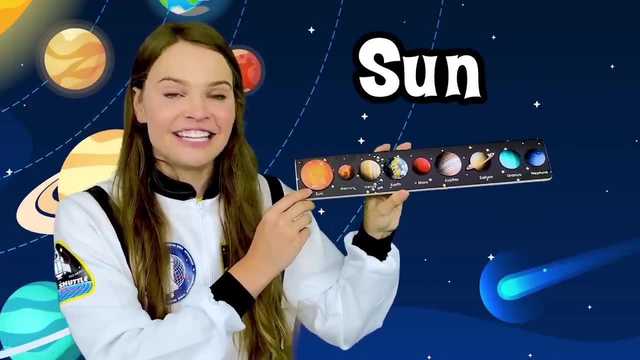 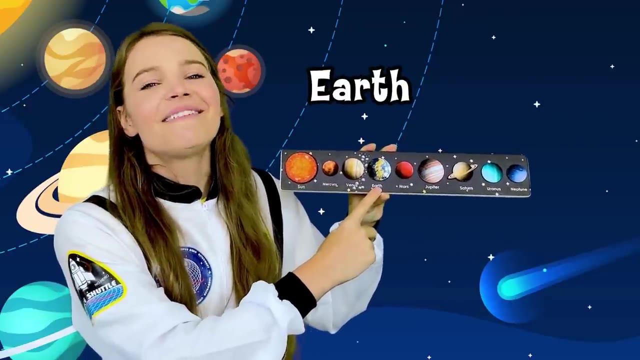 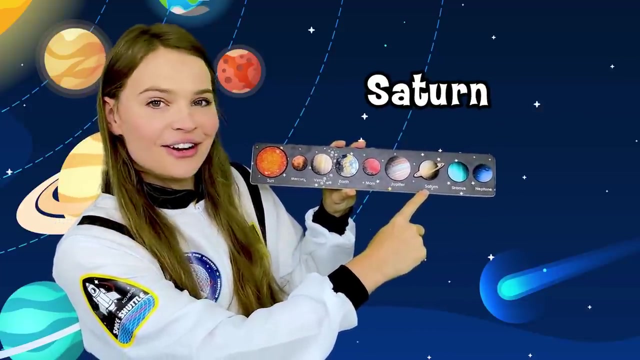 Then you can see other planets there in your rocket ship To learn about planets. I have this puzzle. Let's see. We have the sun, Mercury, Venus and Earth. That's the planet we're on. Then there's Mars, Jupiter, Saturn, Uranus and Neptune. 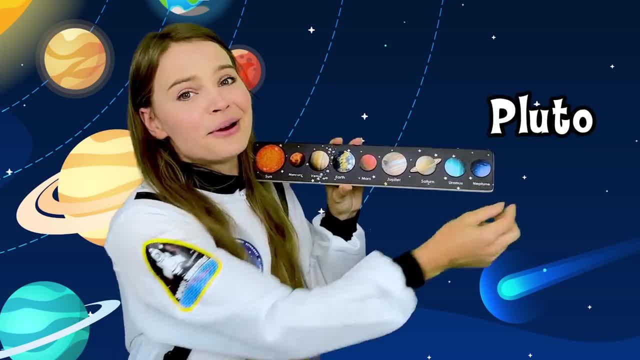 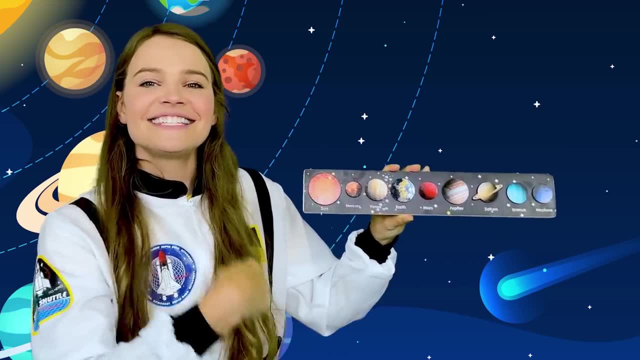 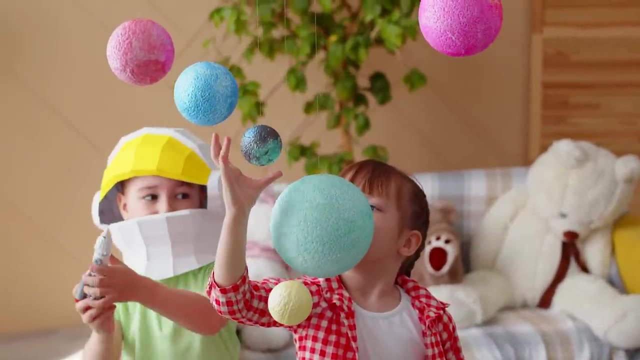 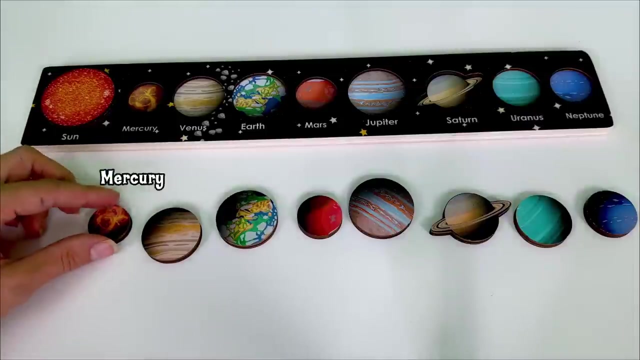 There's also a little planet, a dwarf planet, called Pluto, At the very end, But they're really far away And they all spin and rotate around the sun. Let's put this puzzle together. Here is the sun. Mercury is the closest to the sun. 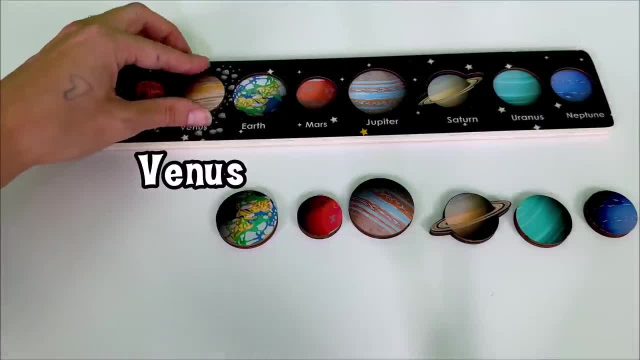 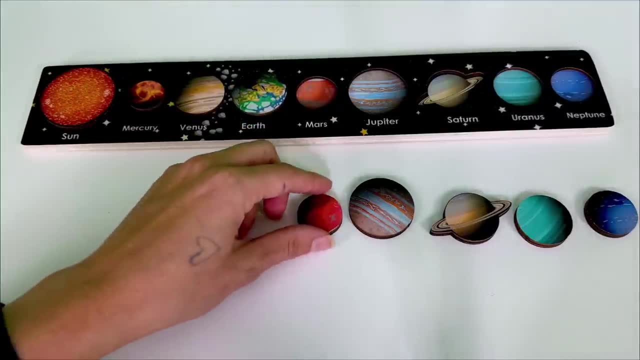 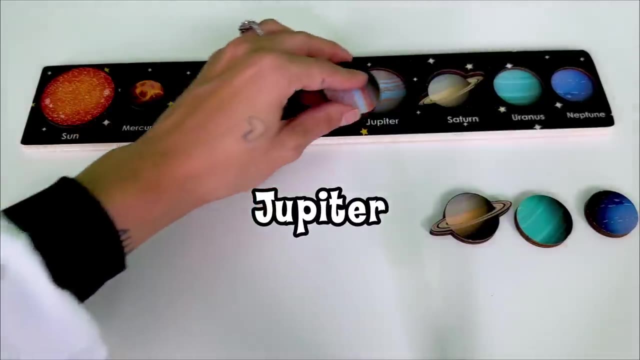 Next is Venus, It's the hottest one Here is Earth, The planet where we see amazing life that breathes. And then there's Mars nearby. It looks red in the sky. Whoa big. It's Jupiter, The giant planet made of gas. 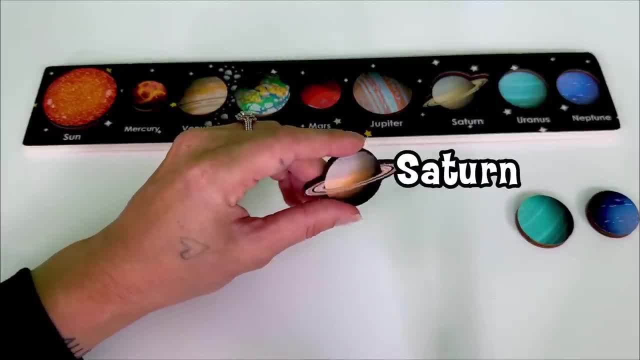 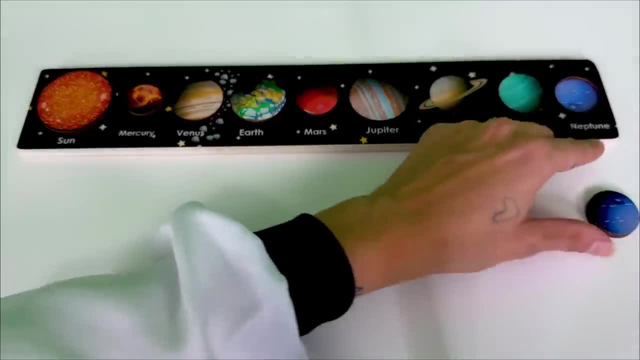 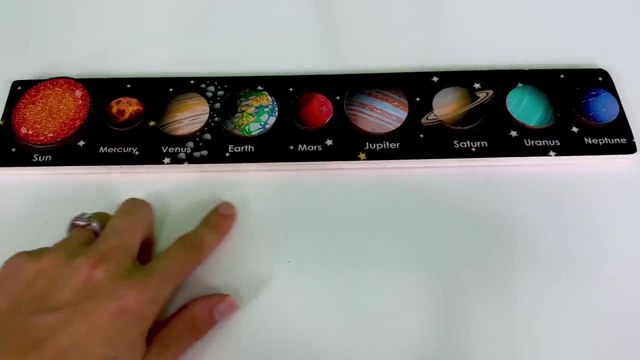 Next, Saturn is a planet that has rings that spin so fast, Brr. Uranus is so, so cold And Neptune is furthest from the sun. And now we're all done: Mercury, Venus, Earth, Mars, Jupiter, Saturn, Uranus, Neptune. 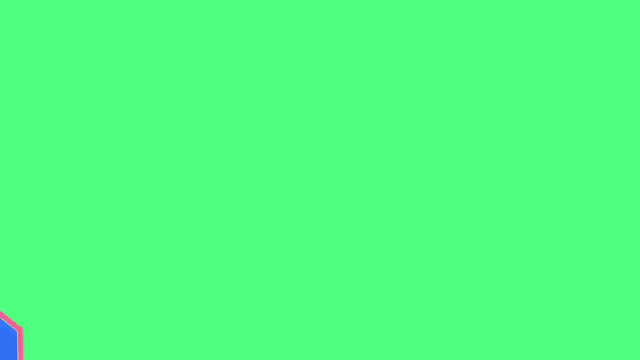 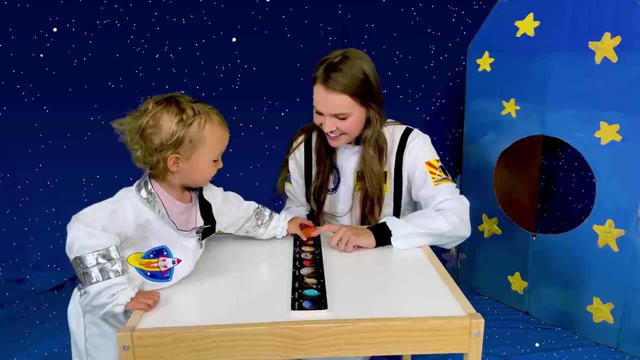 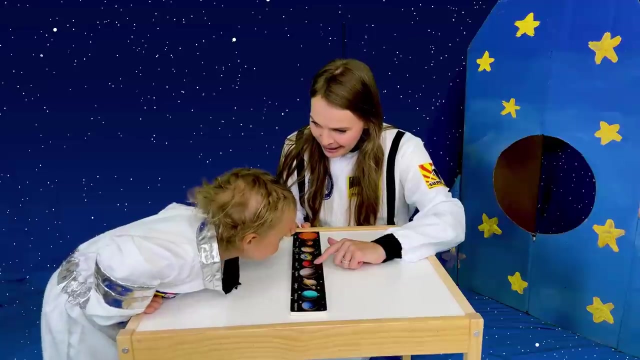 These are the planets of the solar system. First one is Sun. Sun. What's up to the sun? Mercury, Mercury, Then Venus, Venus. What's this one? Earth, Earth, What's this little red one? Mars? 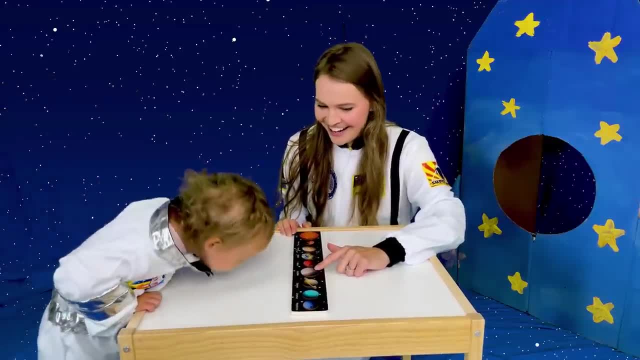 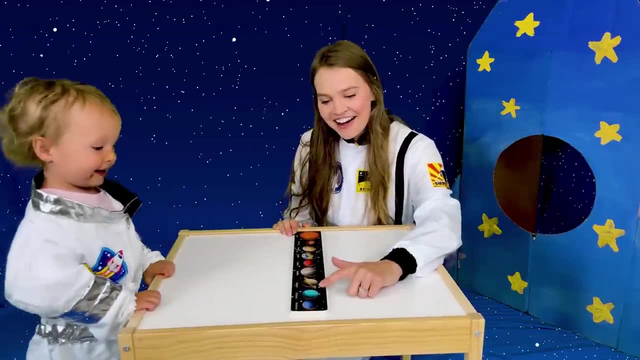 Mars? What about this one? Jupiter? Jupiter, What about this one, Saturn? What are the rings? Is it Saturn, Saturn, Saturn And Uranus, Uranus, And what's this blue one? Neptune, Neptune. Those are all the planets, isn't it? 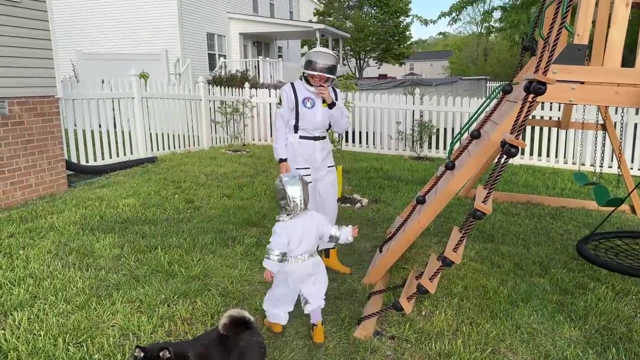 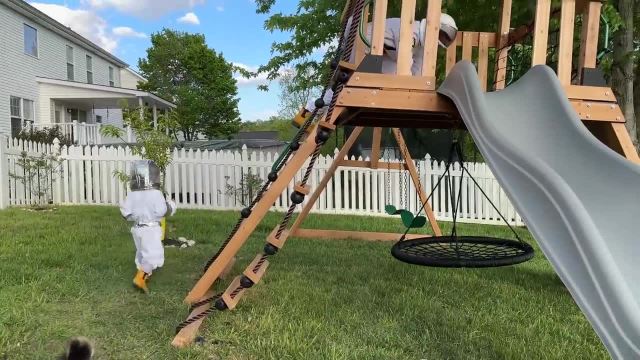 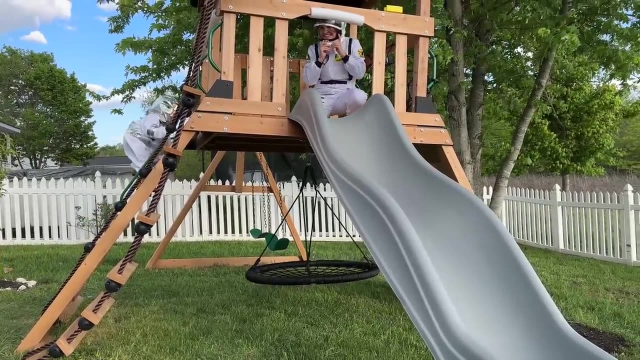 And we're all done. I'm going to blast off. We did a blast off, You did a blast off like that. I saw you. You want to do blast off with me? Yeah, I do. Do you want to go first? 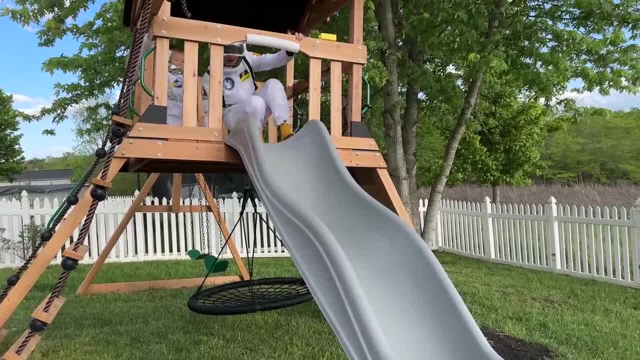 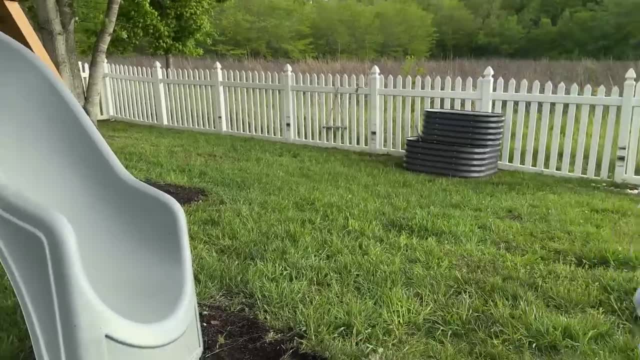 Yeah, One, two, three, Blast off. All right, Mommy, do you fly? You want me to go first. Okay, ready, Push, Blast off. One, two, three, Ready, Blast off. I fly more and more. 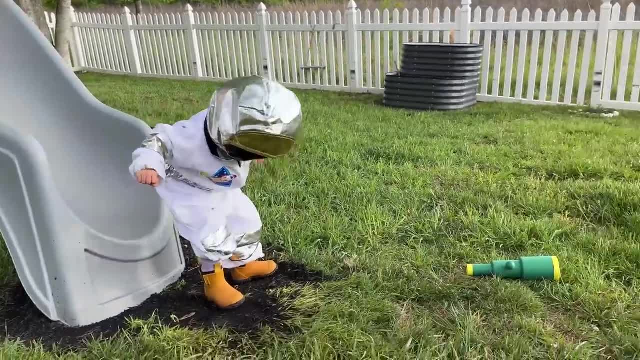 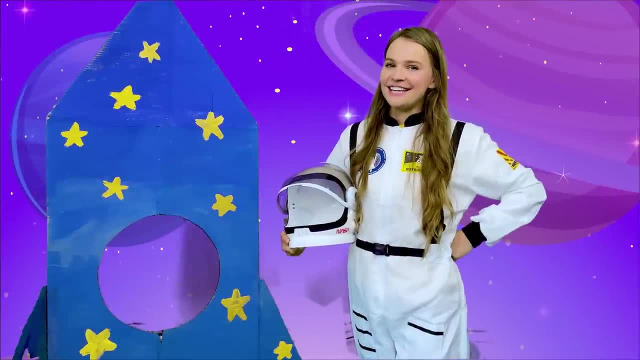 Exploring space is so much fun. Let's take a picture: Three, two, one Cheese. If you'd like, you can ask your grownup for help and print that picture out and cut your face and put it into another astronaut suit so you can take a picture of yourself and 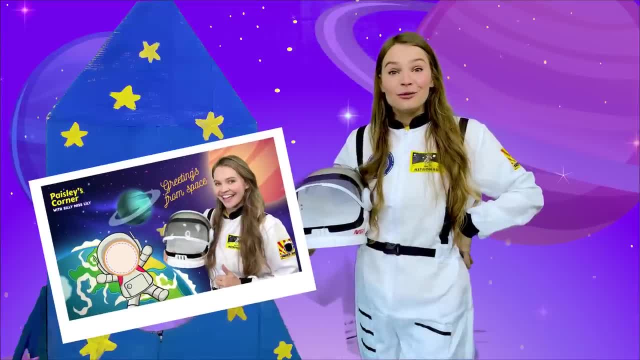 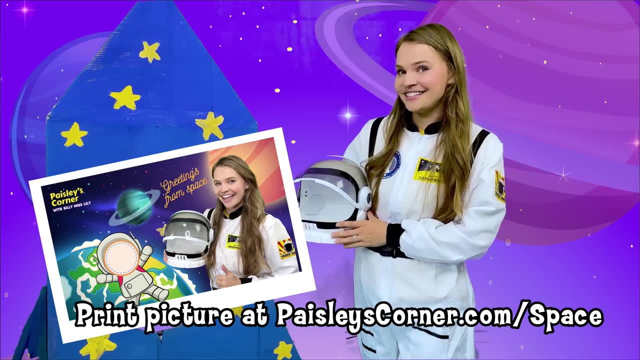 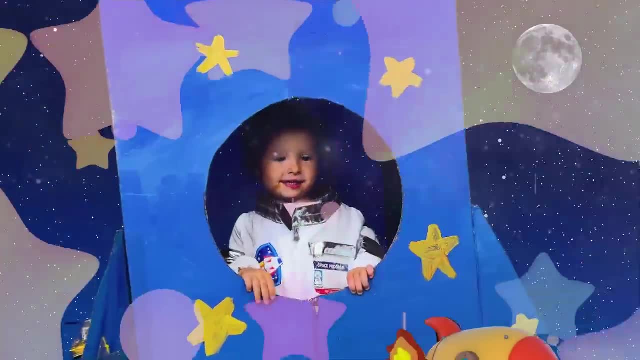 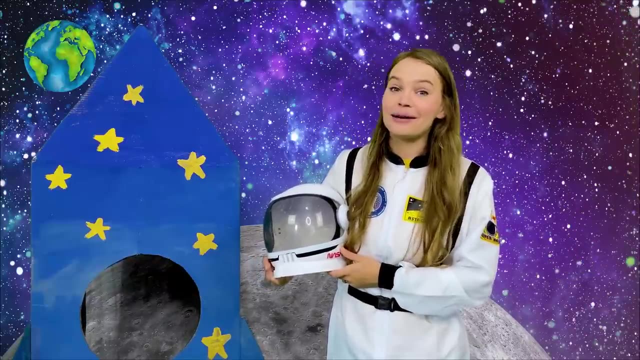 Now are you in space? Yeah, You are. Oh wow, This was so much fun. Thank you so much for playing with me. I loved learning all about space- the moon, planets, sun, stars- and making yummy snacks. 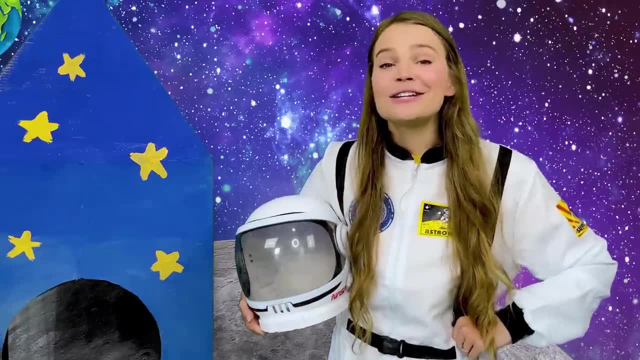 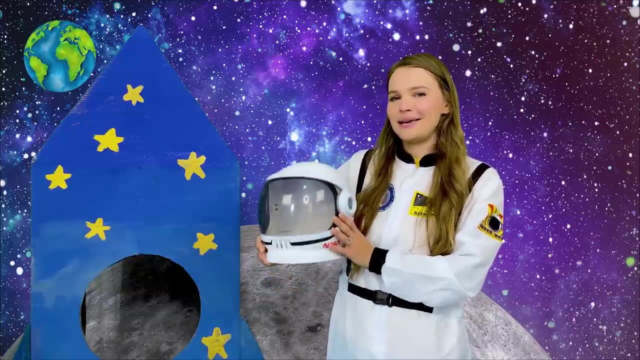 with you and freeze dancing on the moon. Thank you so much for playing with me. I love playing with you and I'm really proud of you. Well, it's the end of this video, So I'm gonna put on my space helmet. 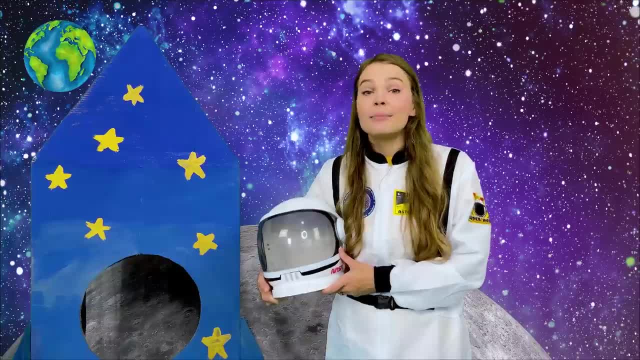 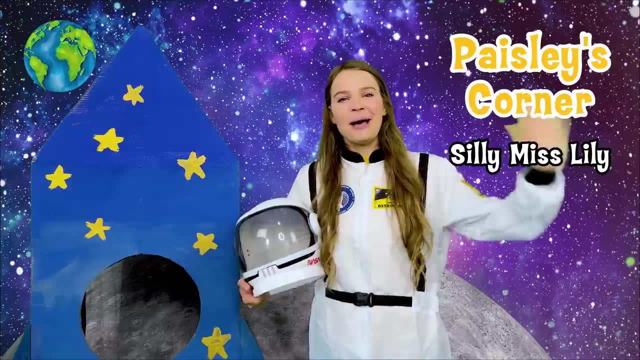 buckle up and get in my spaceship to go back to Earth, And if you're looking for more of our videos, make sure to stay for Paisley's Corner with Silly Miss Lily, And I'll see you then. Bye-bye. 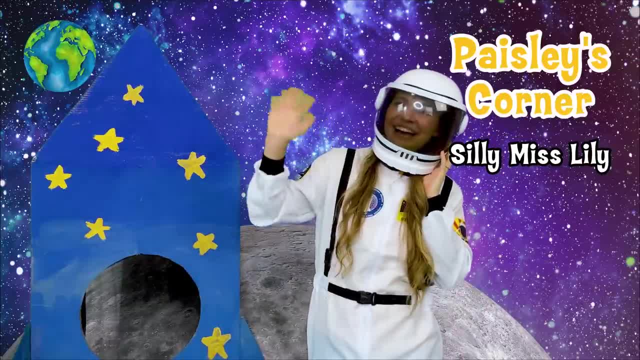 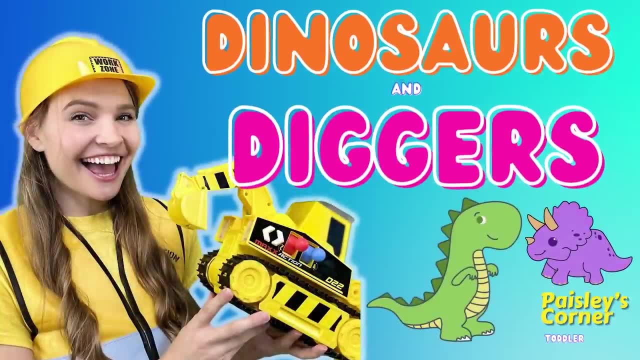 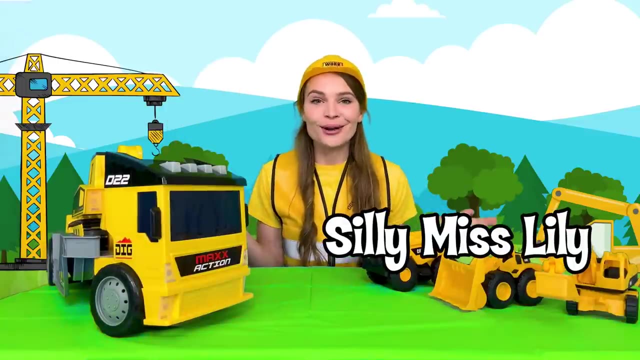 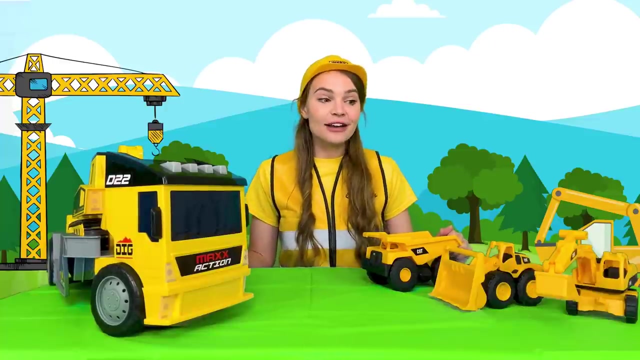 Hi friends, it's me Silly, Miss Lily, and I'm so excited to play with you today. Today I'm really gonna need your help, cause we gotta do some digging around here. I've got some construction vehicles who are gonna help me dig. 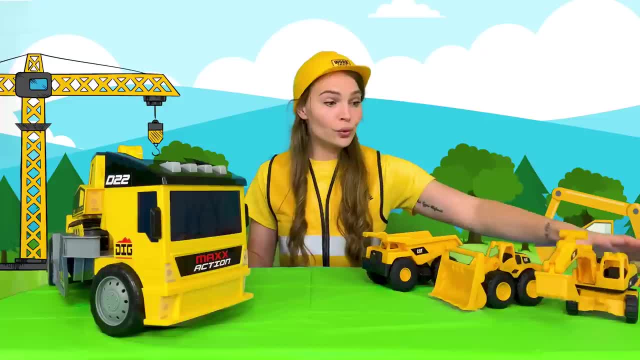 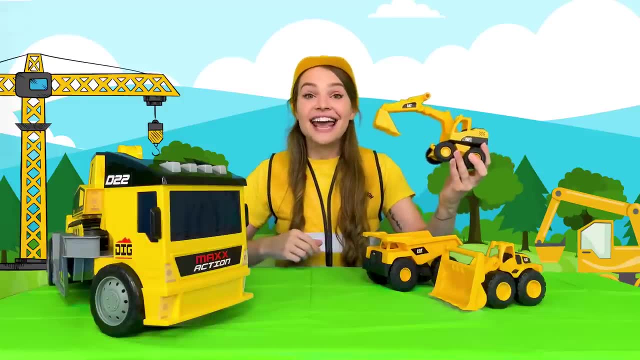 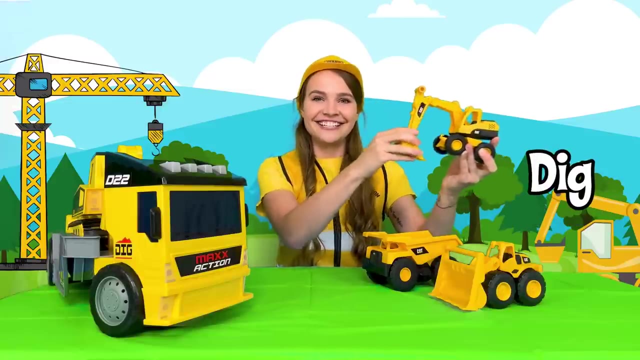 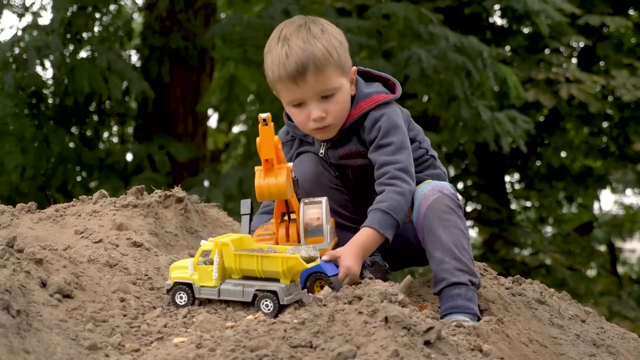 Let's see what we've got. Hmm, ooh, what about this one? Do you know this vehicle? This is an excavator. It's got a long arm and a bucket right here to go, dig, dig, dig. I've also got. 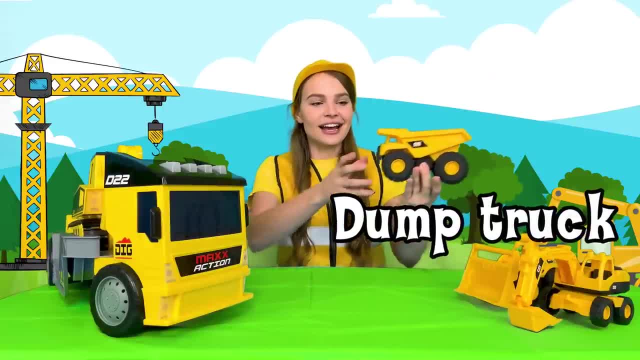 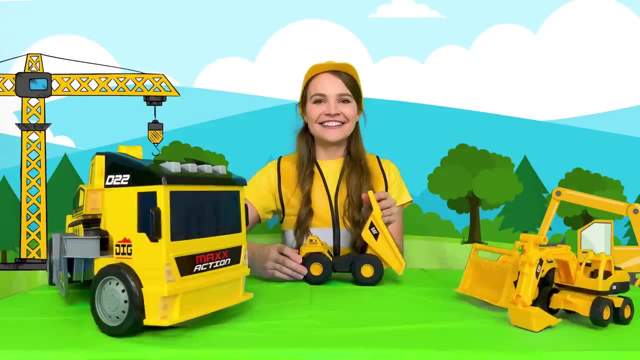 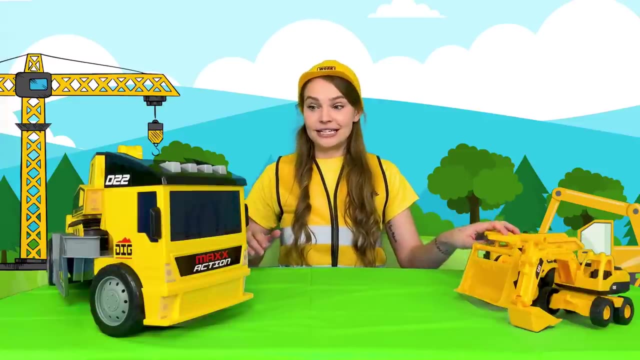 a dump truck. This is a dump truck. You can load the materials in, carry them over, drive, drive and then dump them out. Put them in, drive, drive and dump them out. We've got a big job to do today. 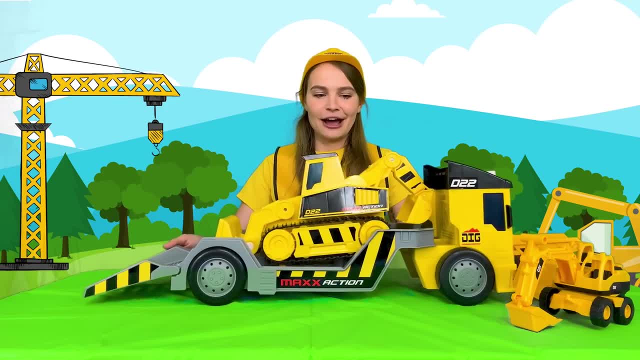 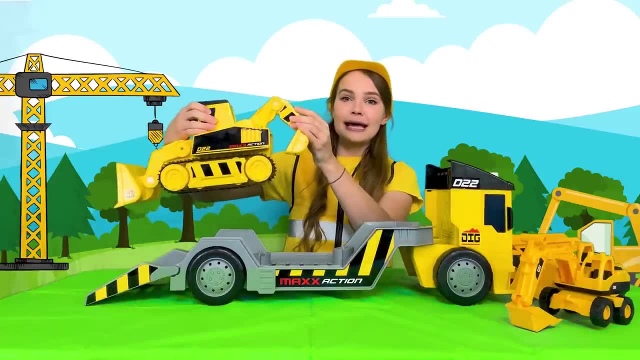 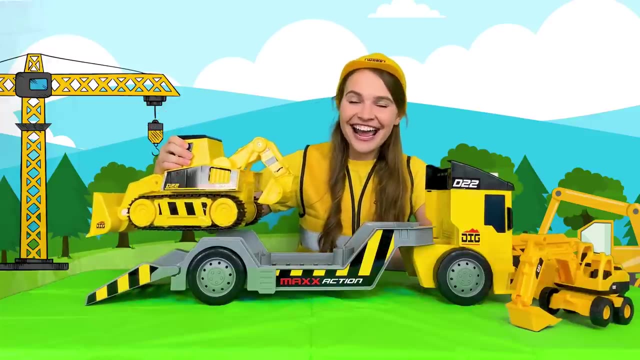 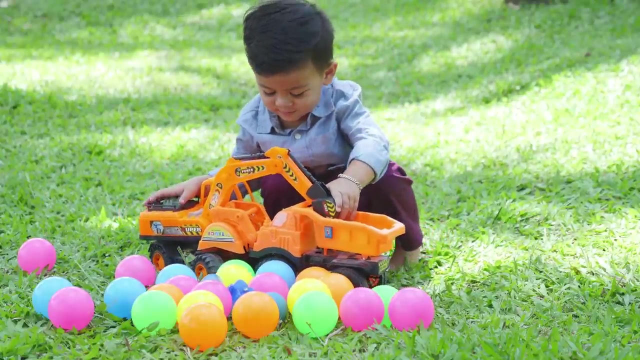 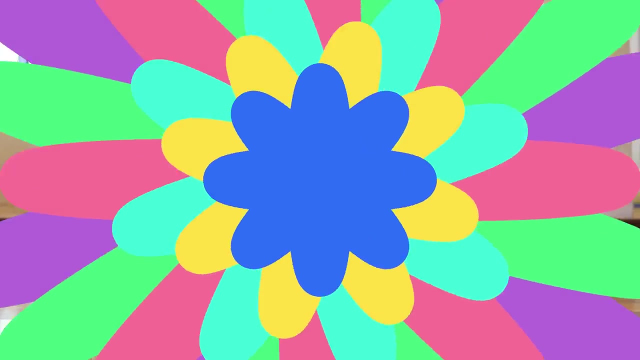 so I've got this big trailer to help us out with a bath hole loader that's gonna help us load things up and discover we've got hiding in the sand. Are you ready to help me? All right, come on. All right, look at ooh. 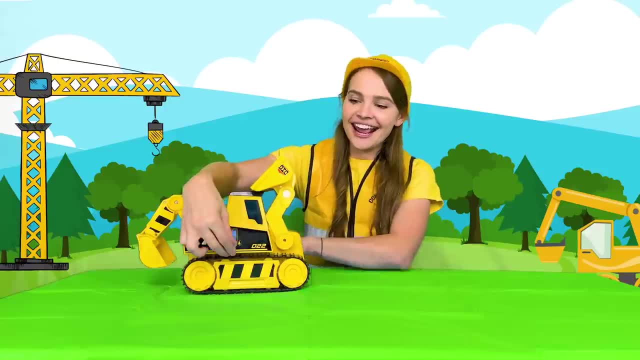 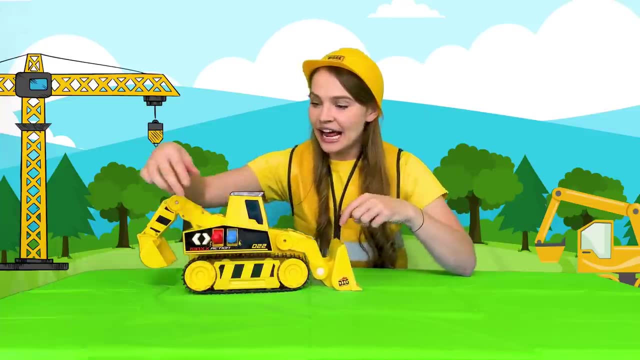 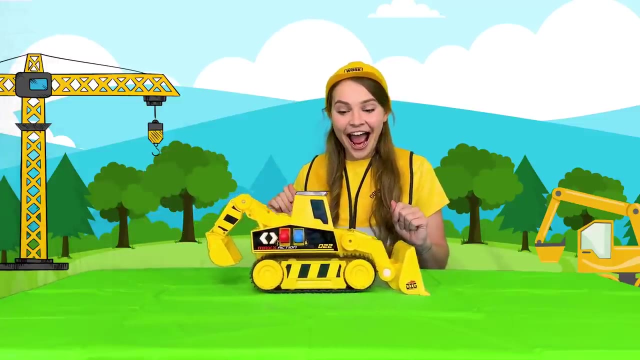 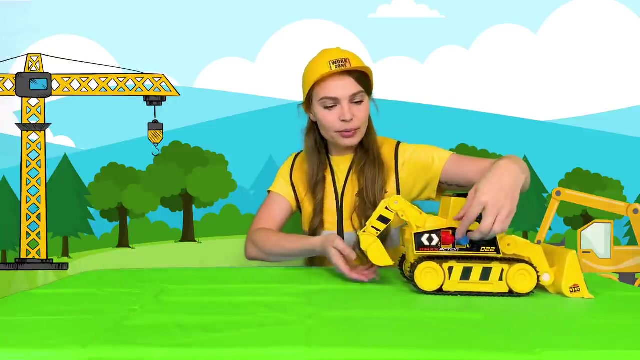 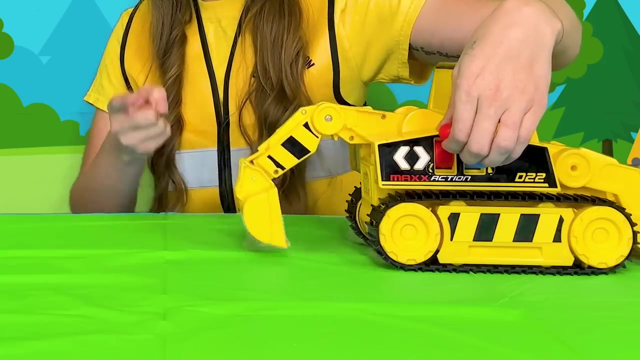 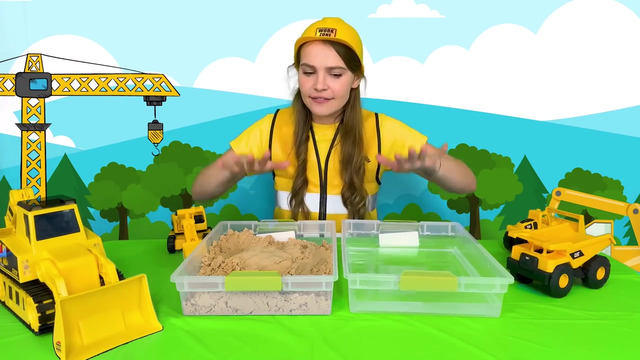 Up And down, Down. Let's see if we can drive it over. All right, Let's see if we can put this arm up, Down and up, Down and up. All right, I've got two bins, One, two. 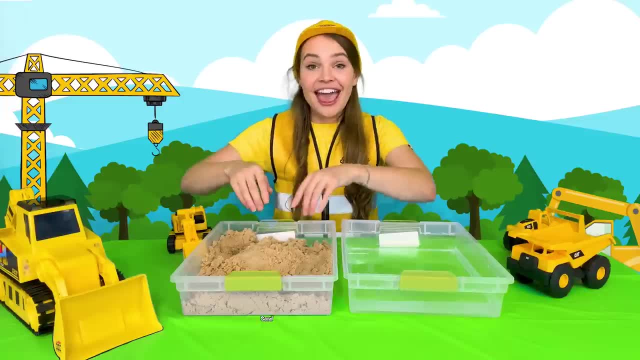 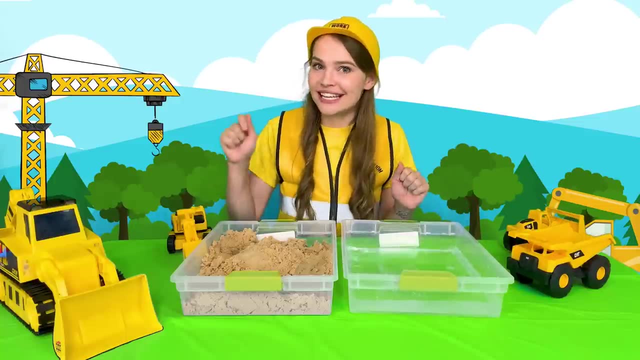 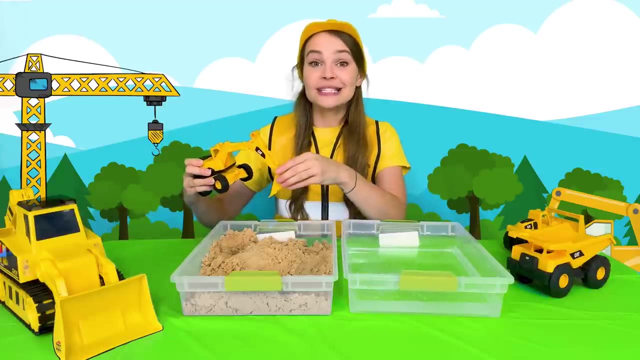 This one has sand in it and this one has water. This way, we're ready to discover what's in our sand bin and we can use the excavator to help us dig Ready. You say dig and I'll put the excavator arm in. 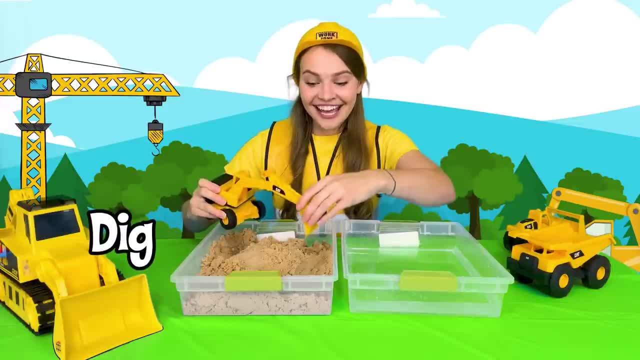 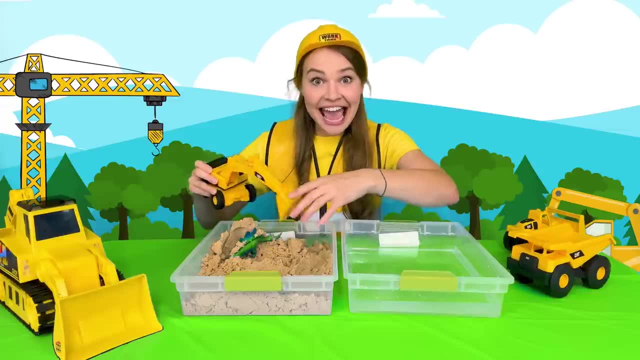 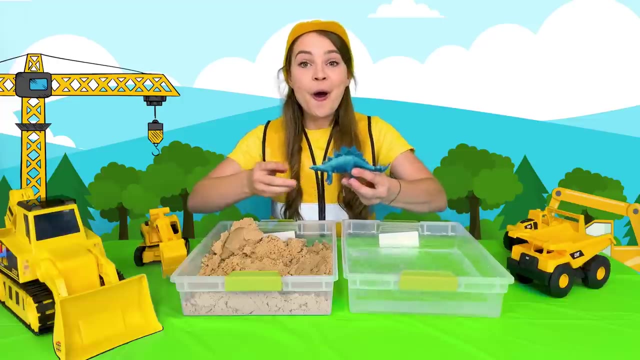 Ready Say dig, Dig, Dig. Hmm, Oh, wait a minute. Did you see that? What is that? Oh, let's take a look, Let's take a look. Let me wash this off. Oh look, Do you know what this is? 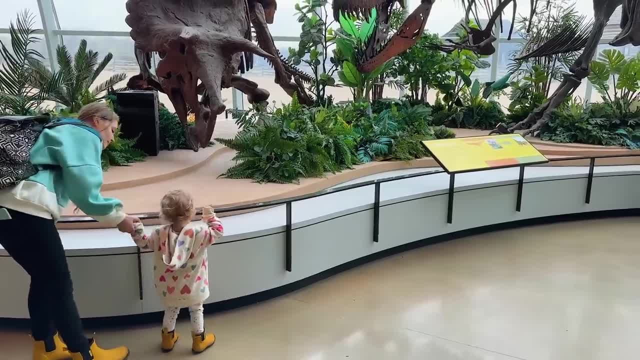 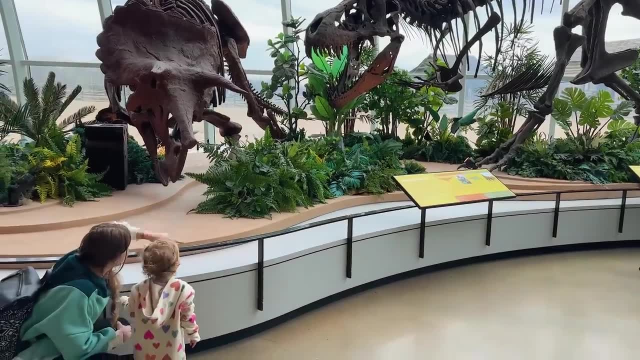 This is a dinosaur. Scientists believe dinosaurs lived a long time ago, but are now extinct and aren't around anymore. You might see dinosaurs on clothes games, big statues and museums, parks and toy dinosaurs, but they're not real dinosaurs, they're toy dinosaurs. 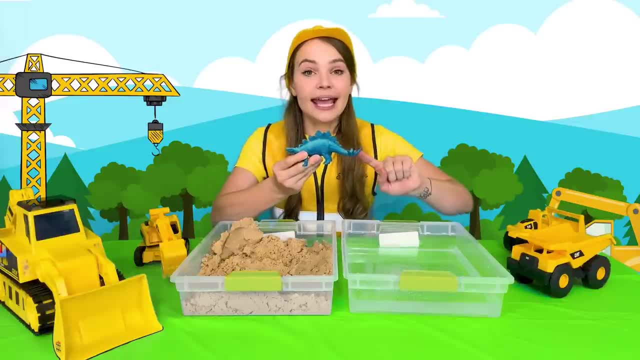 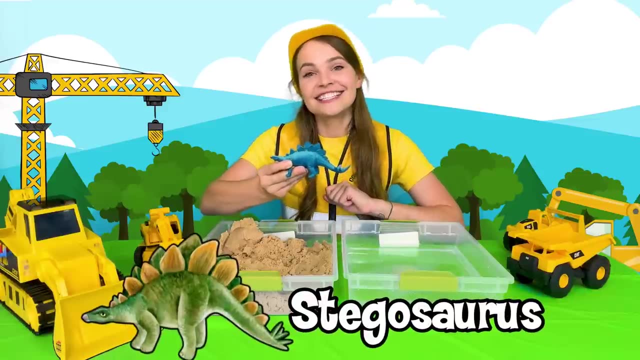 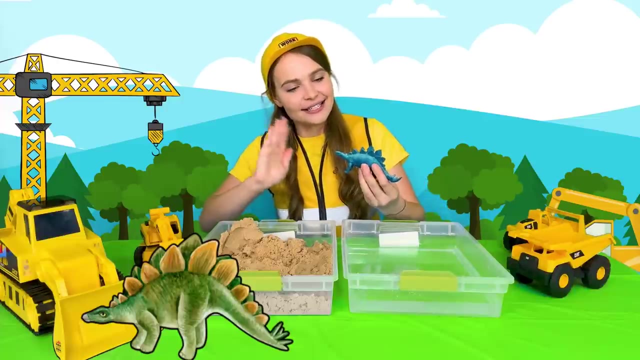 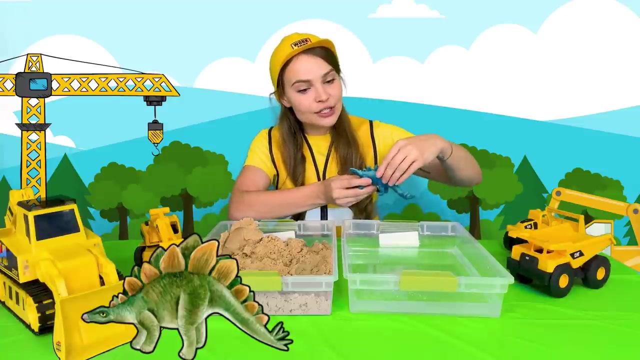 this dinosaur has spikes on its back and on its tail. this dinosaur is called a stegosaurus stegosaurus, the one with the spikes on its back, hi, stegosaurus. stegosaurus says hello, hello. thank you for digging me up. stegosaurus, would you like to swim in the water for now? 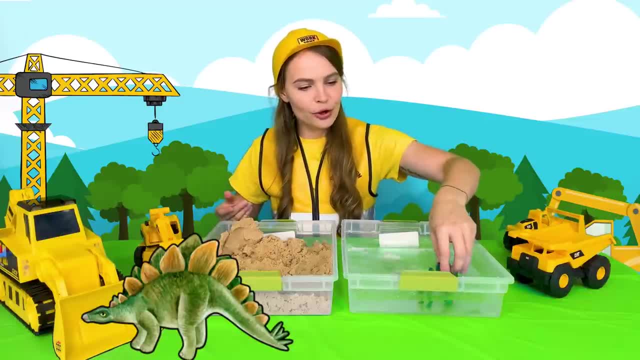 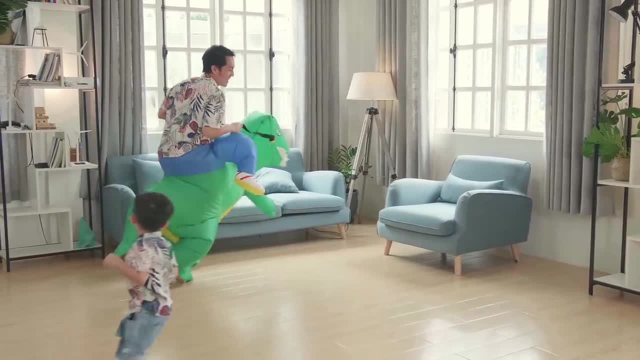 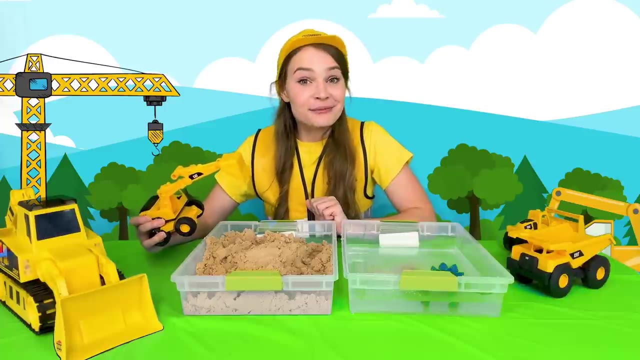 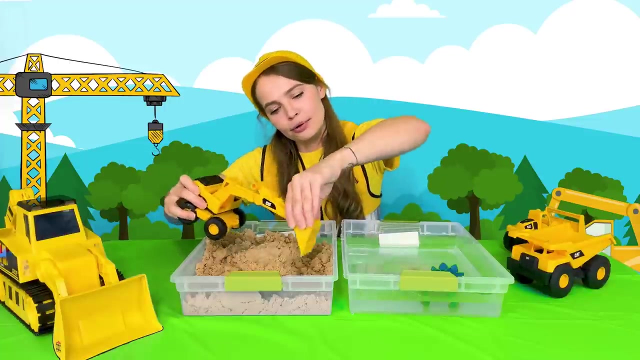 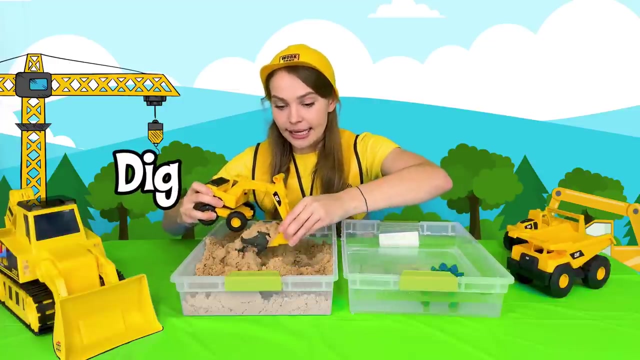 oh yeah, i'd love to swim. he says: bloop, bloop, bloop, have fun, let's dig some more and see what else we can find. come on, excavator, dig. i got some sand for it out. dig some more sand for it out, dig, i think we got something big. let's get it out. oh wow. 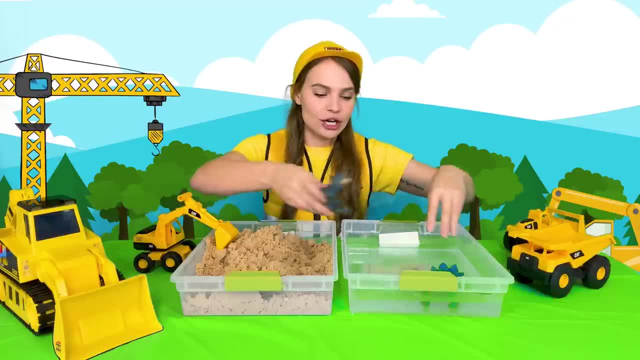 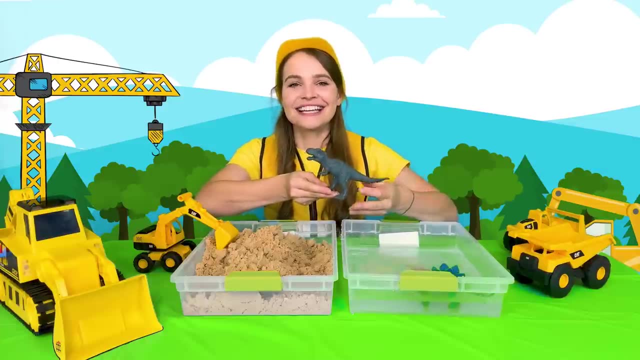 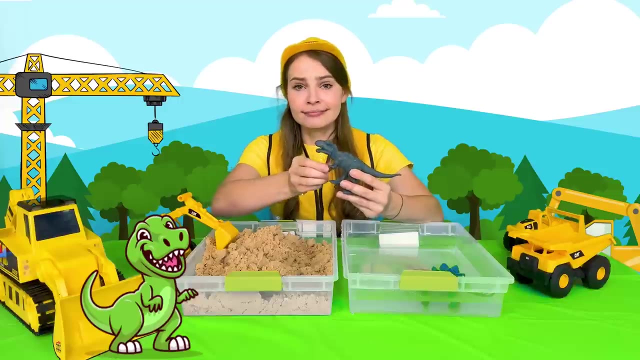 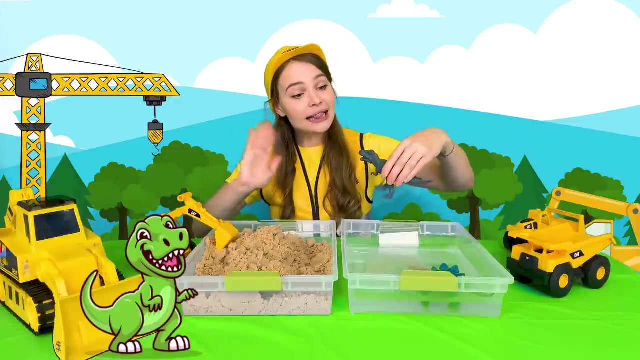 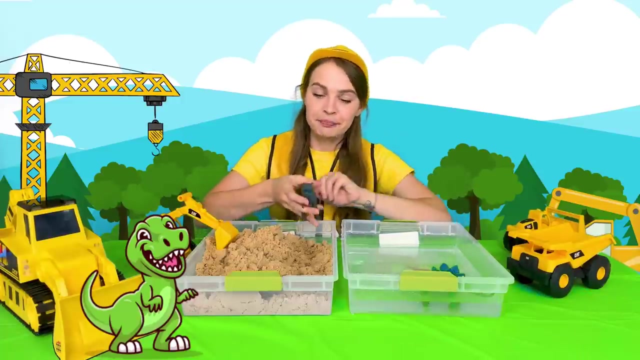 we got another dinosaur. let me wash him up. wash, wash, wash, wash, oh wow. this dinosaur is called tyrannosaurus rex, or t-rex for short. got a big head, small arms and strong big legs. says hello, hello, tyrannosaurus. tyrannosaurus, that's a big word. hello, it's very nice to meet you. hey, t-rex, you want to? 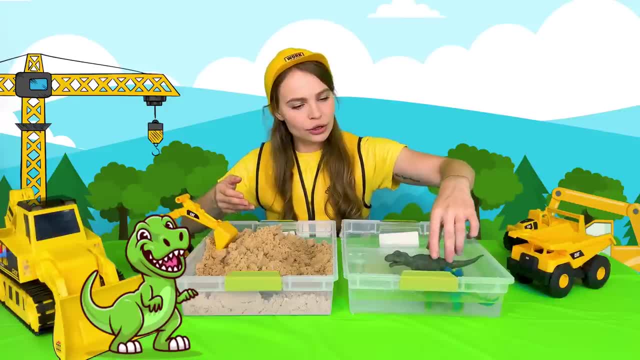 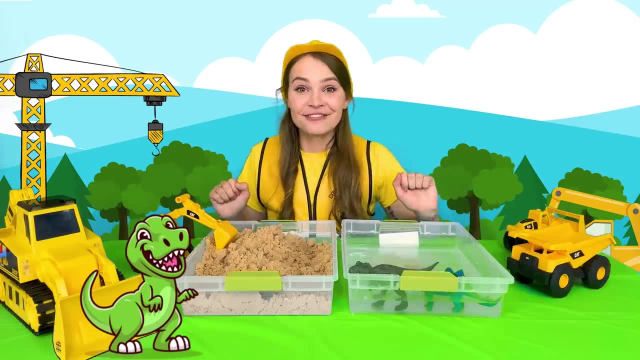 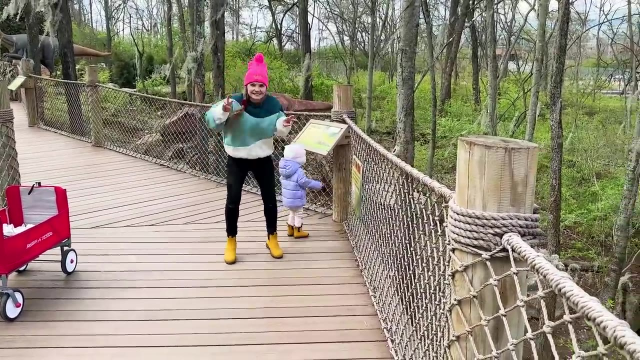 go in the water. oh yeah, i'd love to splash around there you go, there you go, little t-rex, and let's dig some more. i've am going up and down on my night watch and we can pop up here. there's one big fire, the any other guard? i need what to catch. 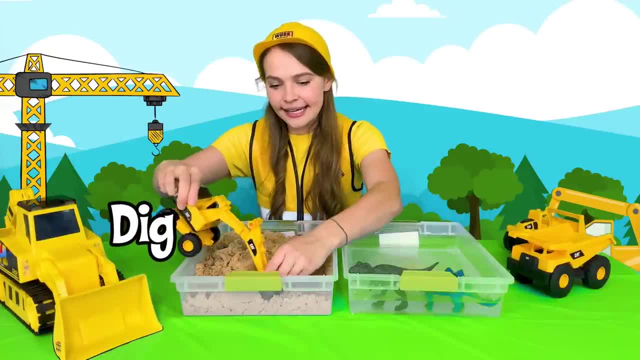 dig dig, dig, dig dig dig, digаж digg. displacement dig dig dig dig dig. old man, oh, i think i see something. dig dig dig dig. oh, i think i see something. 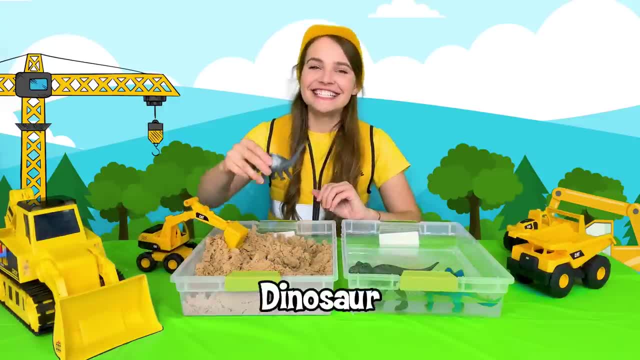 dig, dig, dig. oh, wow, we got another dinosaur. let's dig some more. i see that bone and stuff boy. oh, i want honey dadoo. dig, dig, dig, dig, dig, dig, dig. wow, we get a good dinosaur. 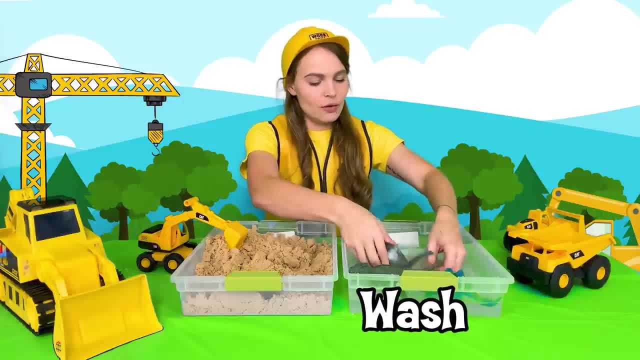 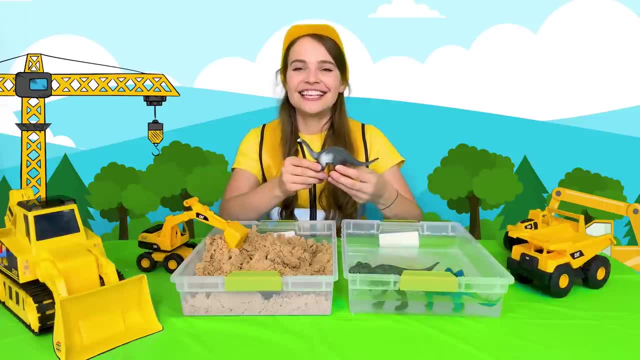 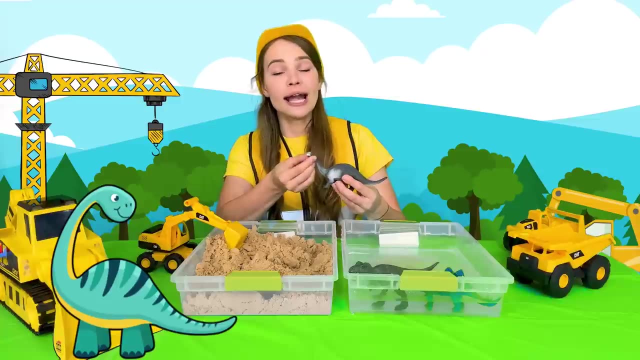 Let's wash it up. Here you go: wash wash, Wash wash dinosaur. Look at this dinosaur. It's got a long neck. This dinosaur is called Brontosaurus. Brontosaurus got a long neck, Kind of like giraffes, huh. 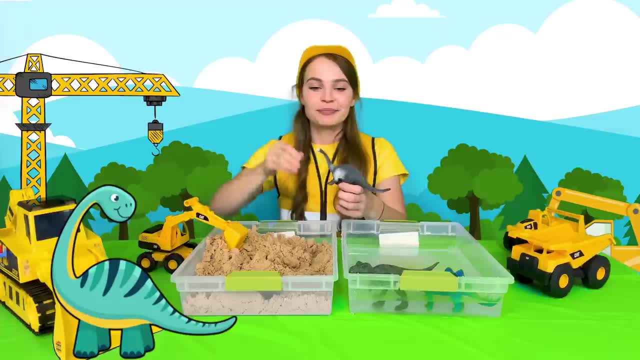 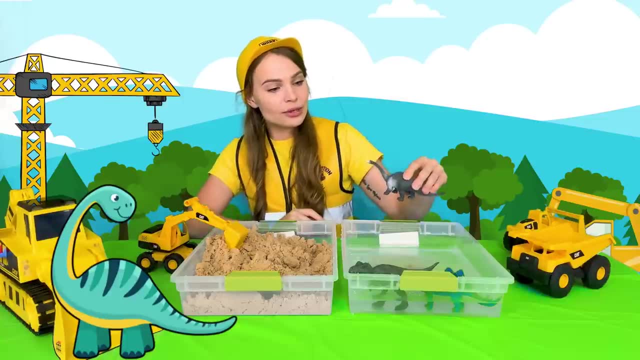 They like to reach up high and eat the leaves off the trees. I bet Brontosaurus love eating leaves off trees too. Hi Brontosaurus, Do you want to go swim with the rest of the dinos? Oh sure I'd love to, he says. 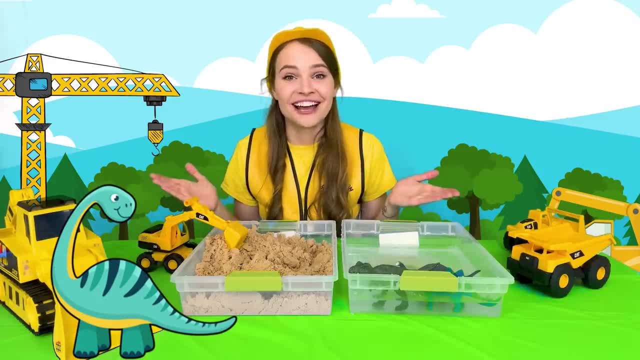 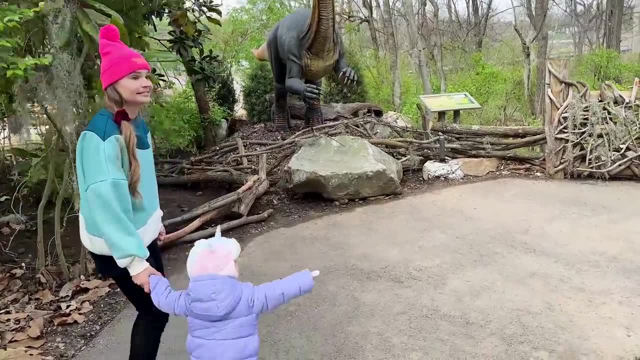 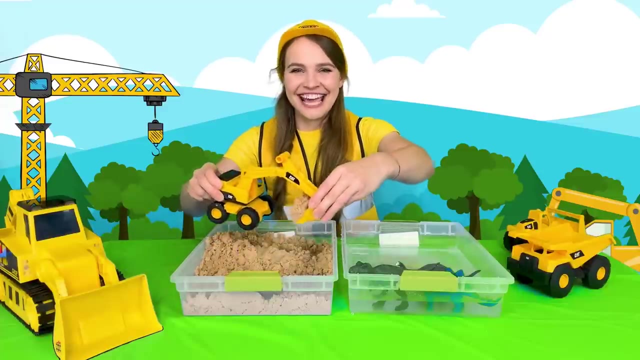 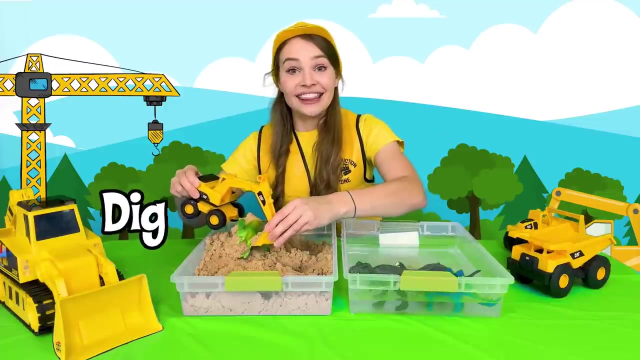 Bloop, bloop, bloop. Let's keep digging and see who else we can find. Dig some sand, empty it out. Dig. that's more sand. let's empty it out, Dig. oh, I think I see something. 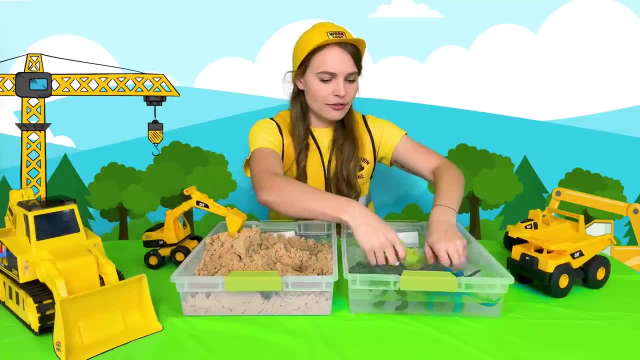 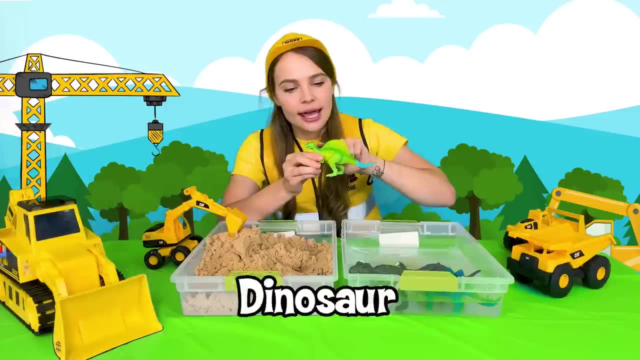 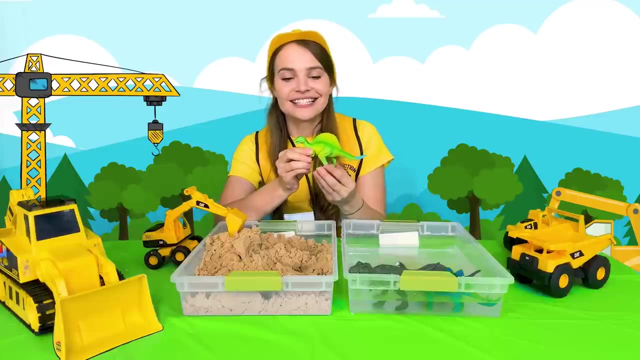 Let me catch it, Let me rinse them off. Wash wash, wash wash. Oh look, it's another dinosaur. This dinosaur has a little kind of sail on top of the back, almost like a rainbow going over it, and it's called Spinosaurus. 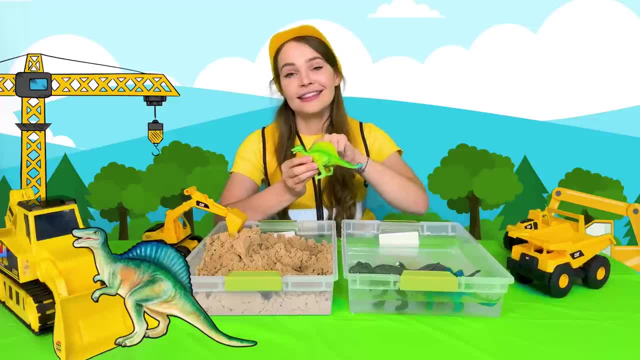 This part of our back is called our spine and this dinosaur is called Spinosaurus. Hi, Spinosaurus, it's very nice to meet you. Hi, Spinosaurus, it's very nice to meet you. Hi, Spinosaurus, it's very nice to meet you. 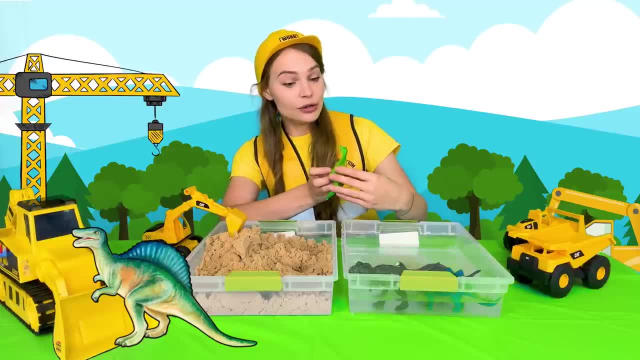 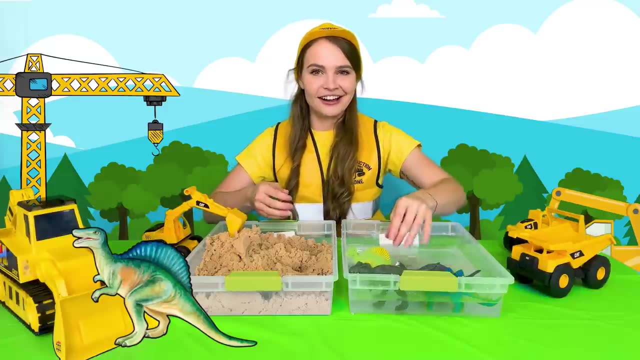 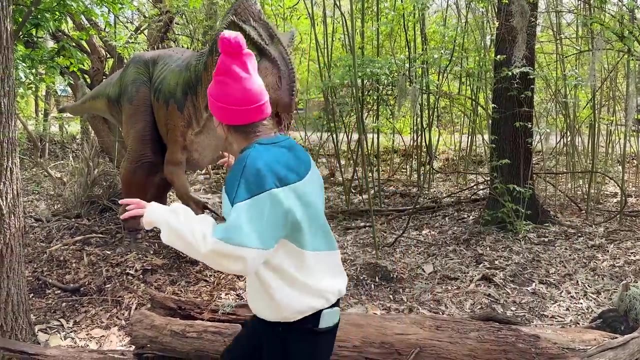 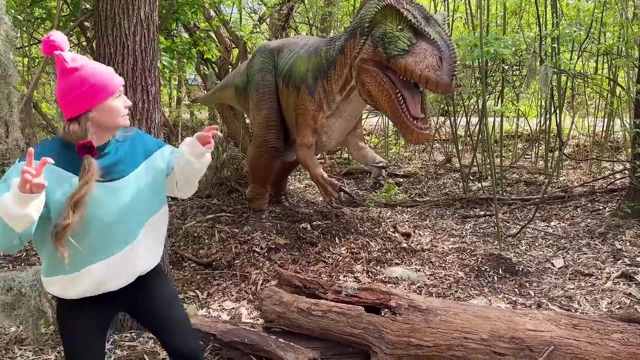 Spinosaurus says: hello, Would you like to go wash up with the other dinos? Spinosaurus says: okay, wash, wash, There you go, have fun. Let's dig for some more dinosaurs. Let's keep digging. 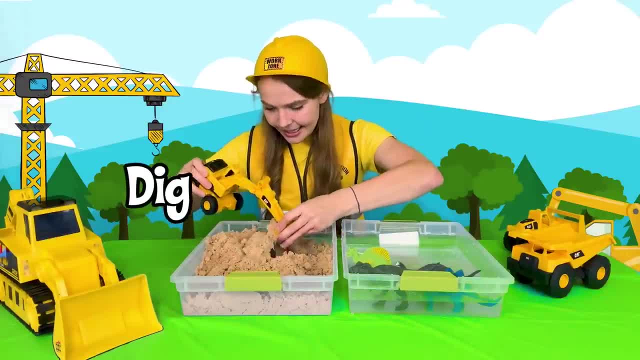 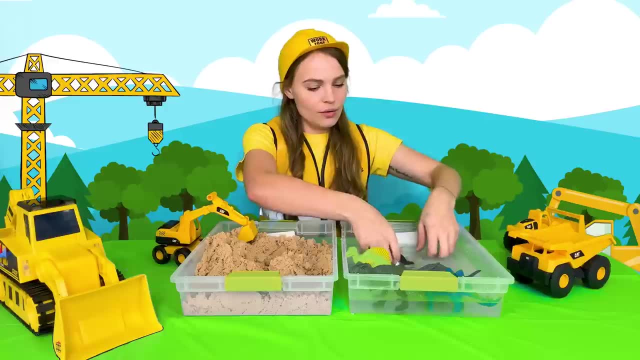 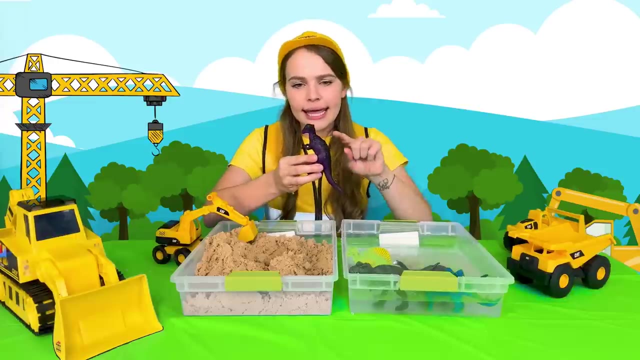 Dig, dig. Oh, I think I see something. Oh wow, let's wash this dino up. Wash wash dino, Wash wash dino. Look at this dinosaur. It looks like he's almost wearing a helmet. 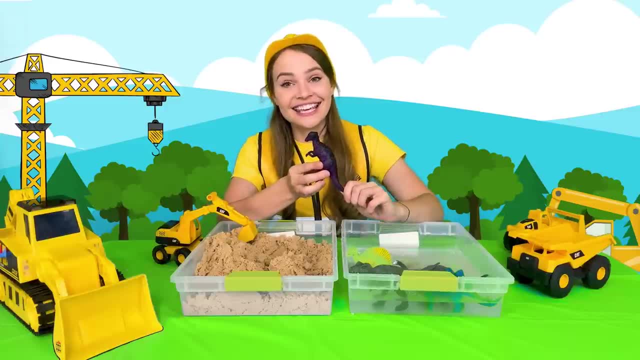 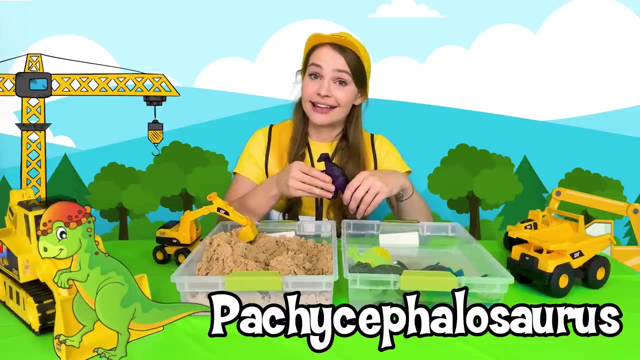 like an egg-shaped helmet almost. I think this is a Pachycephalosaurus. A Pachycephalosaurus, That's a big word: Pachycephalosaurus, Pachycephalosaurus. 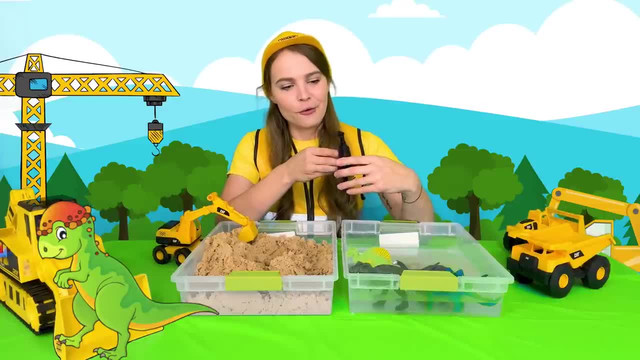 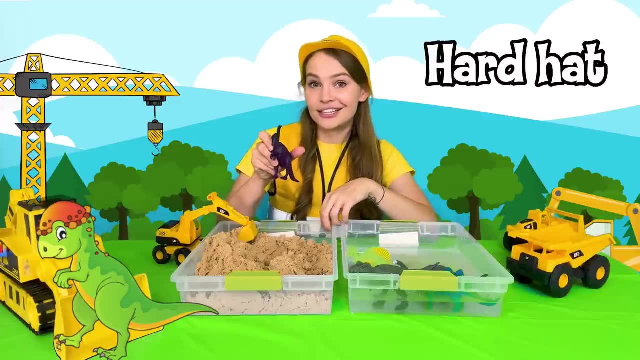 Pachycephalosaurus. Oh wow, I like the way his head looks like he's almost wearing a helmet or a hard hat. I bet he'd like to do construction too, huh Well, it's very nice to meet you. 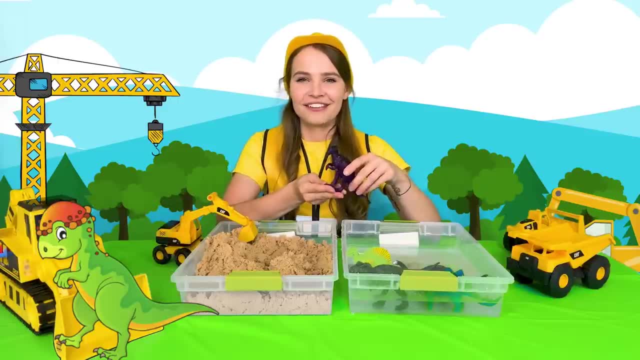 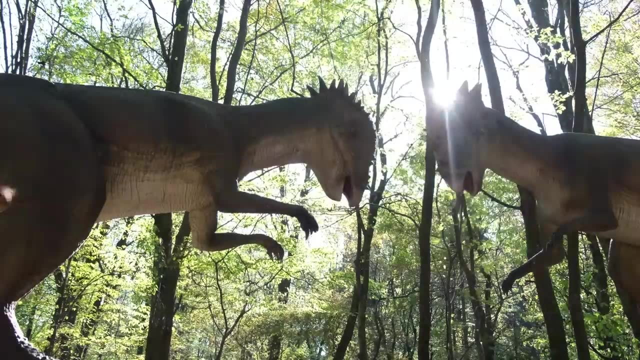 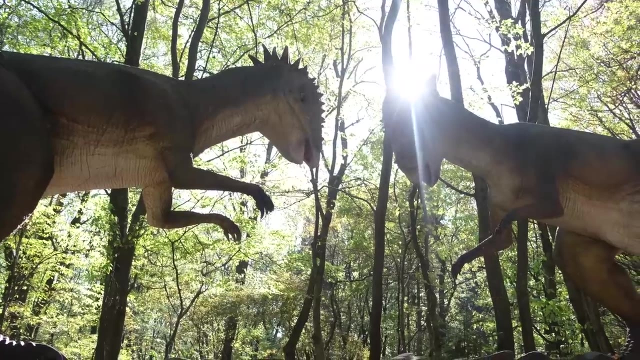 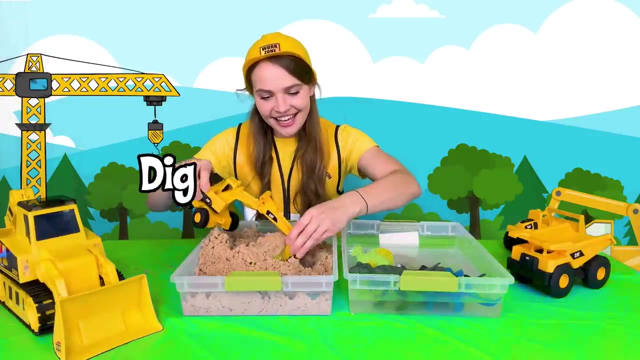 Would you like to go swim with our other dinosaurs? Pachycephalosaurus says: sure, Here you go. enjoy, Let's dig some more. Let's keep digging, Dig, Dig. I think I got something, Let's bring it out. 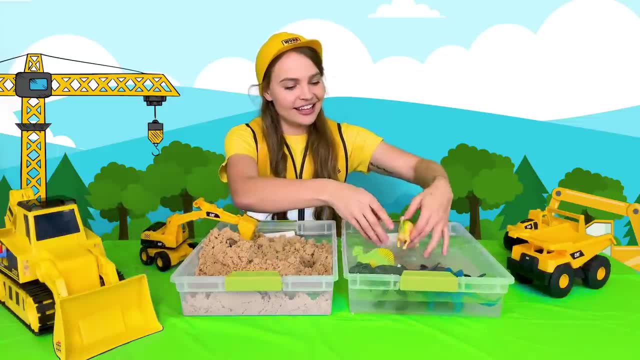 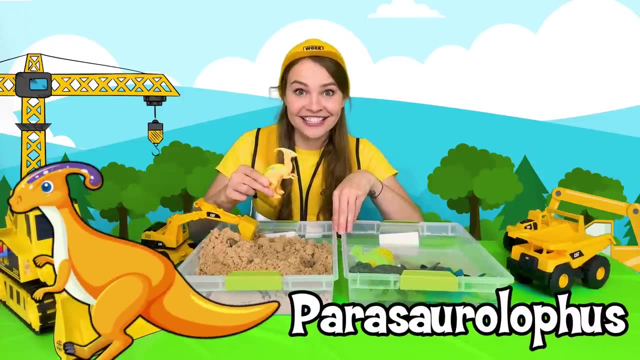 Give him a little wash. Look at this dinosaur. This dinosaur is called Parasaurolophus. That's another big one, Parasaurolophus- Parasaurolophus- Parasaurolophus- Parasaurolophus. 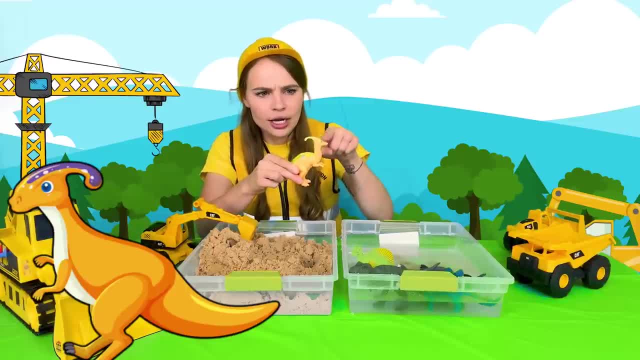 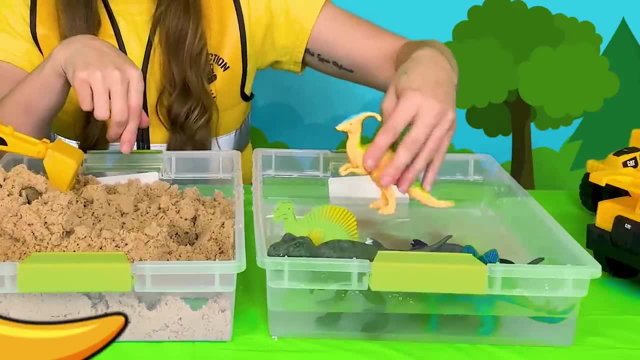 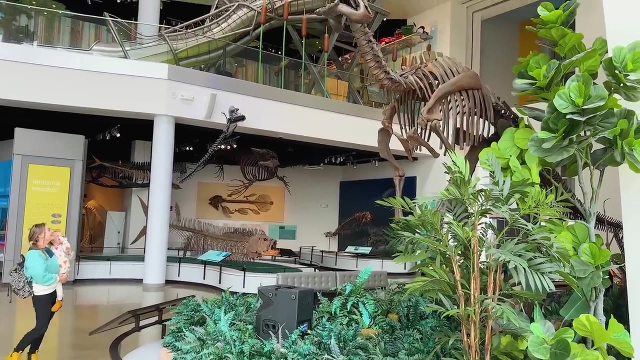 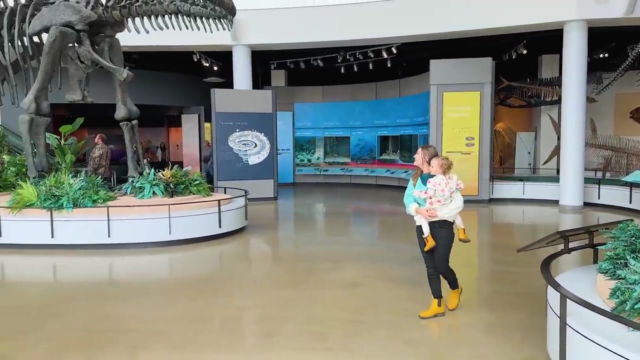 Parasaurolophus. It's got a really interesting head. Almost looks like a hook on its head. Wow, Very nice to meet you. I'll go swimming with the other dinos. Okay, Have fun, Let's keep exploring. 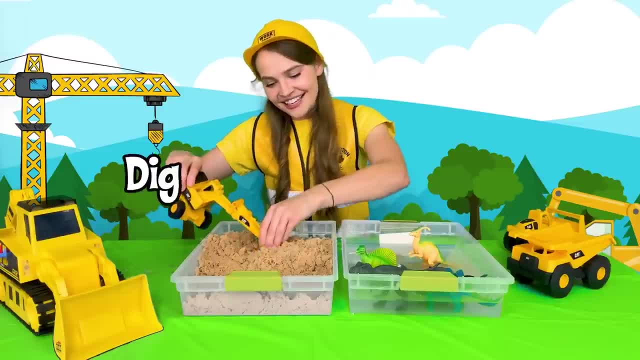 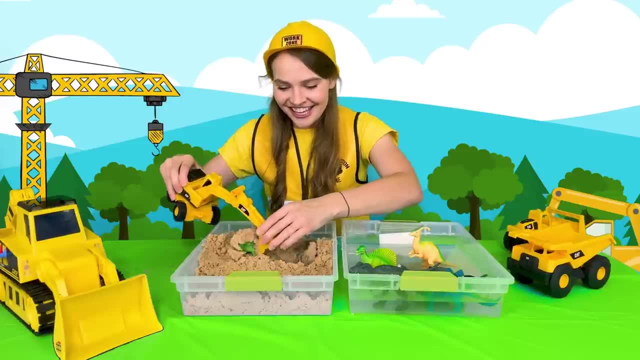 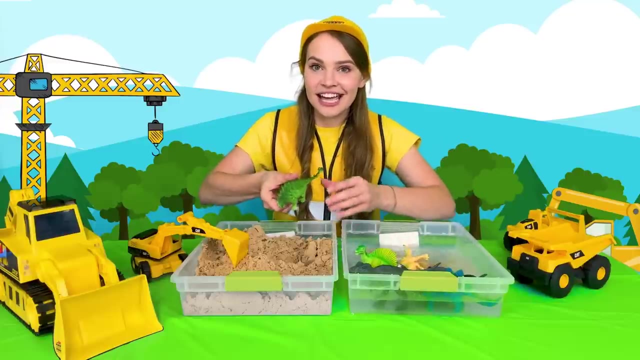 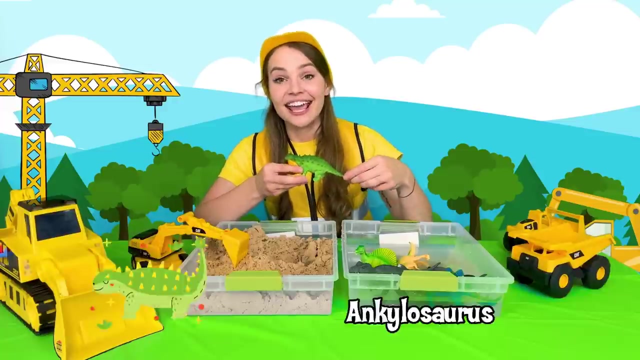 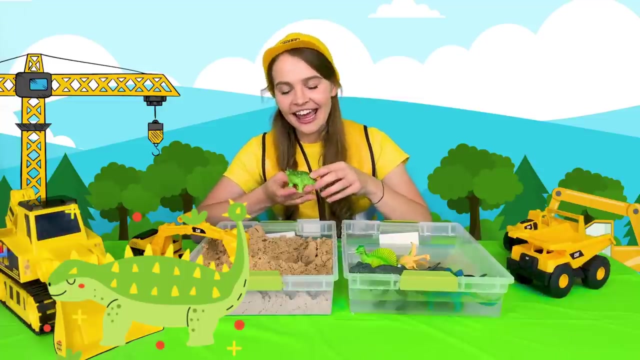 let's keep digging, dig, dig, dig. I think I got something. let's see what we've got. oh, let me wash them up. oh, look at this dinosaur. it's got spike spikes all over his back and his tail. this dinosaur is called ankylosaurus. hi ankylosaurus. ankylosaurus says hello, hello. he kind of looks. 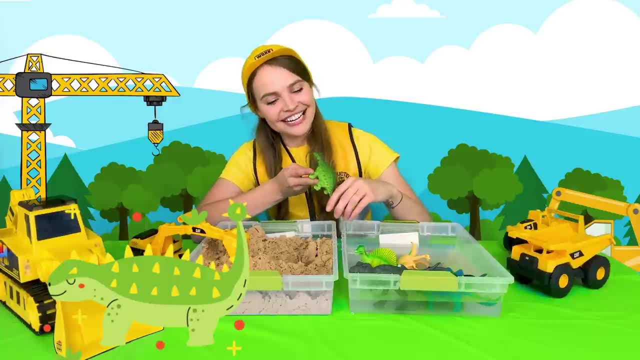 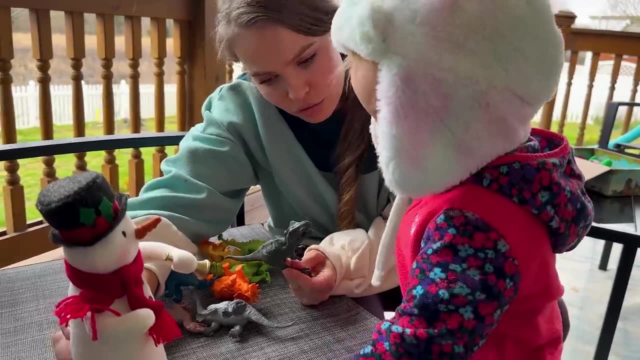 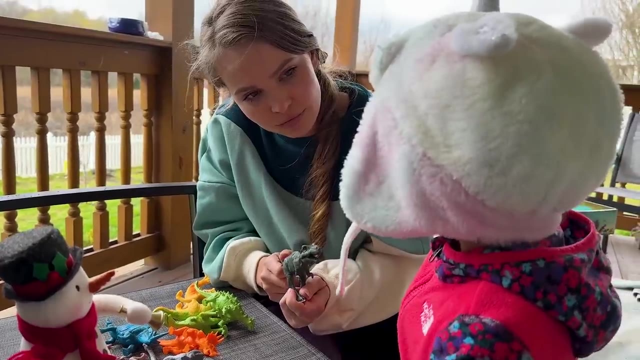 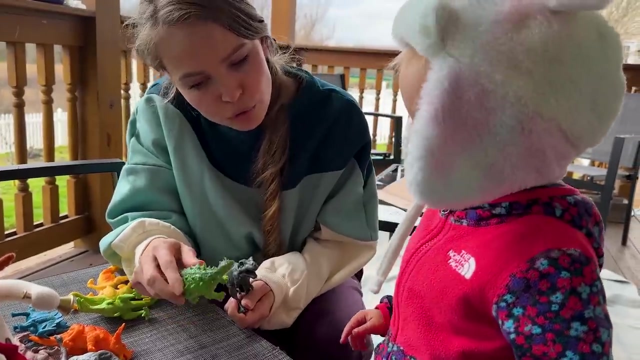 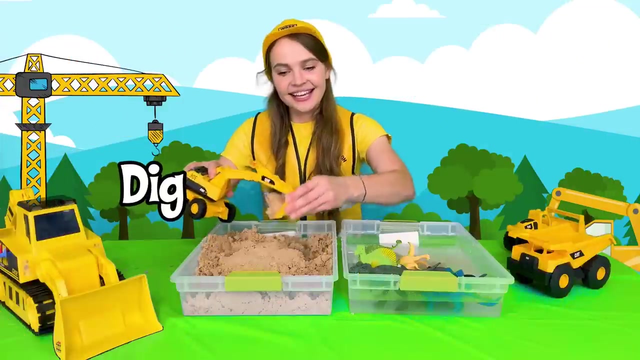 like an alligator with the spikes. very nice to meet you. I'll go swimming with the others. have fun, let's see who else we can find. oh, ankylosaurus, hello, hello. will you press my button? ankylosaurus dig did. oh, I think I got something. 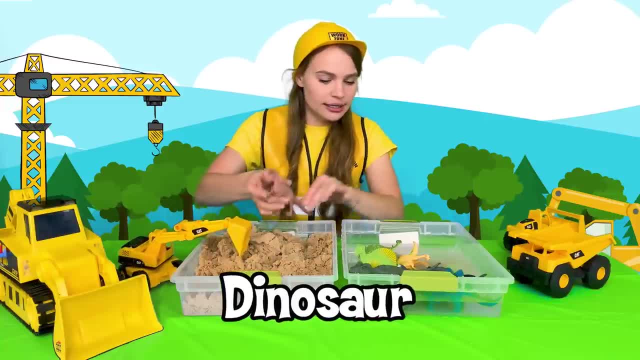 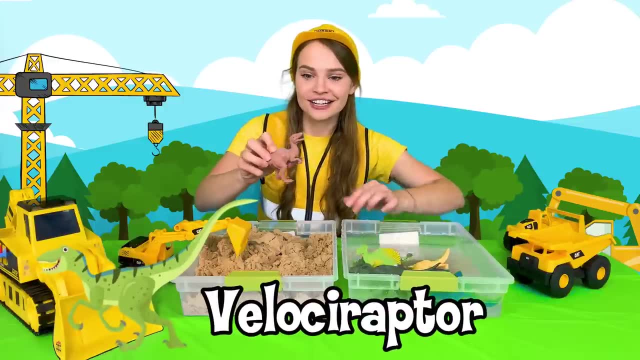 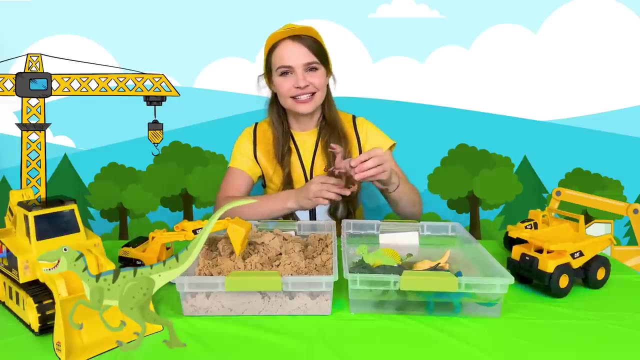 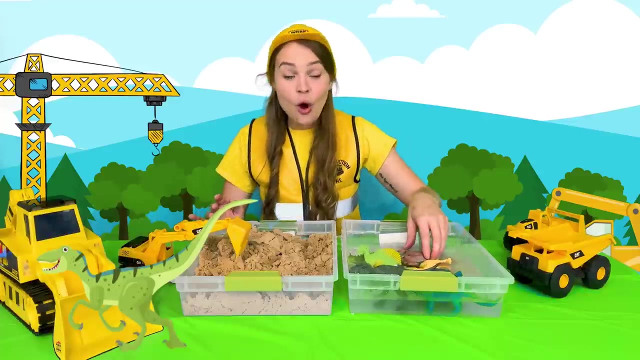 oh look another dinosaur, let's wash him up. oh look, this dinosaur is called velociraptor. they kind of look like T-Rex, but with smaller heads. very nice to meet you. velociraptor says: hello, I'll go swim with the other dinosaurs, have fun. wow, can you believe all the dinosaur that we? 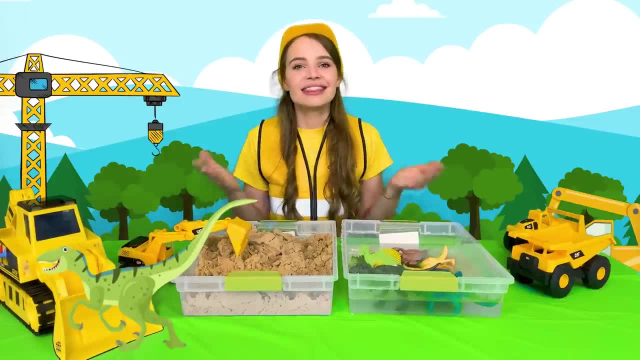 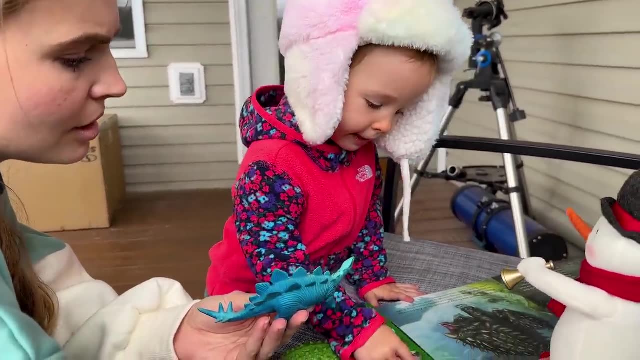 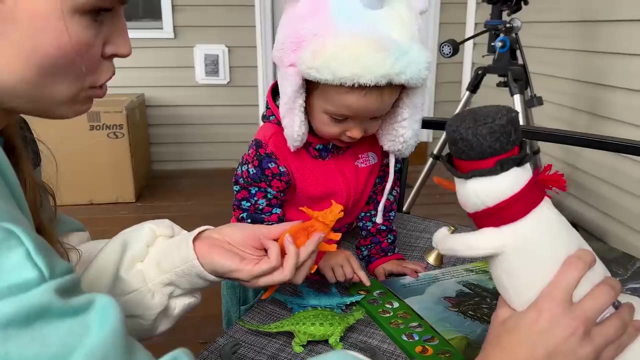 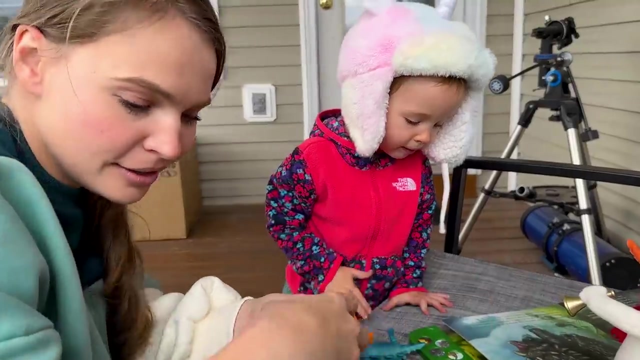 found in the sand. that was really fun. thank you so much for digging with me. what's this dinosaur called? that's right. what's the name on Paisley? what's this one called monoclonius, right? monoclonius, monoclonius, Paisley, Paisley. what's this dinosaur called? 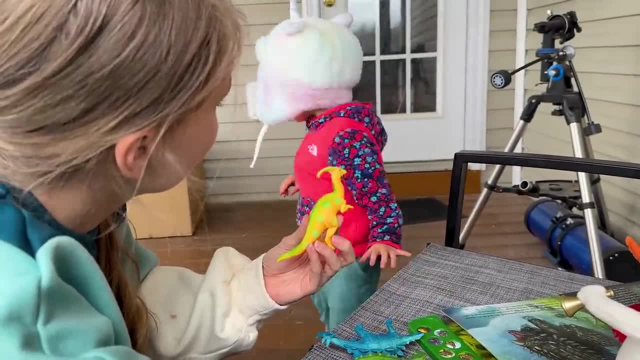 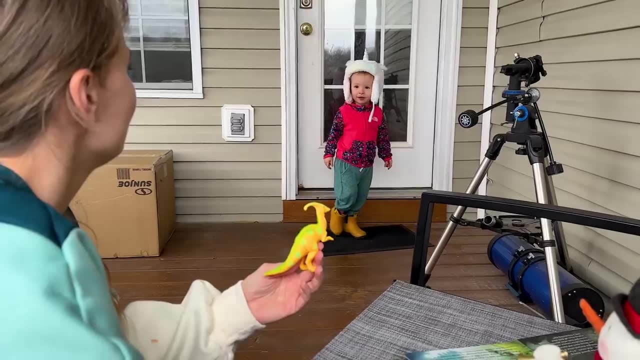 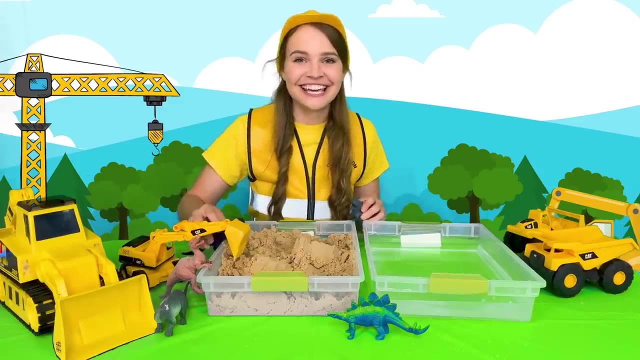 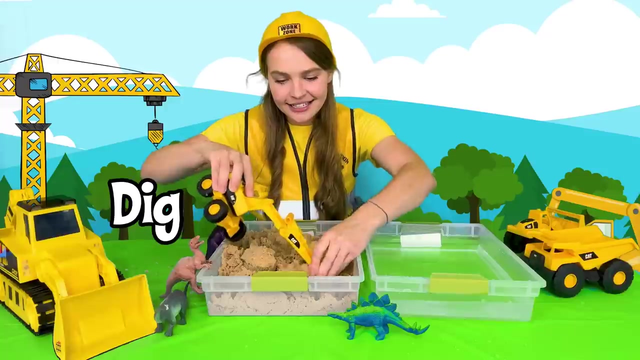 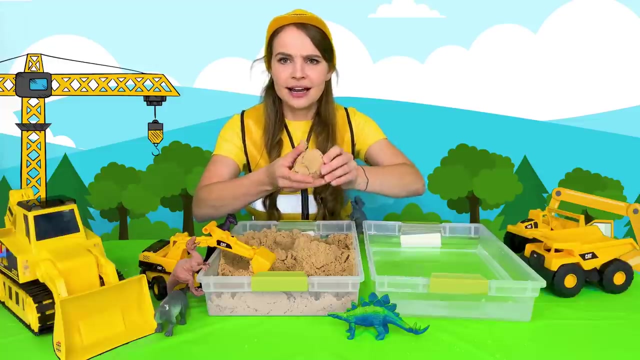 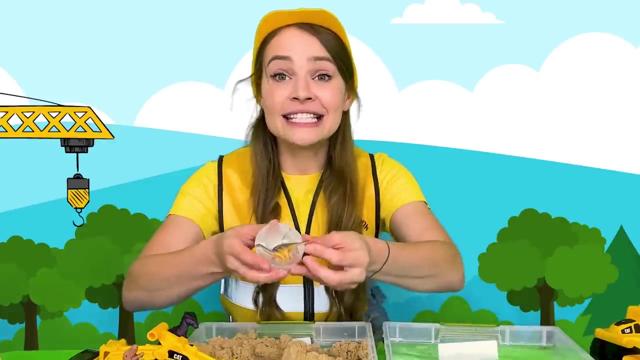 parasaurolophus- good one. what about parasol? parasaurolophus- good one. parasolophus: good one. let's dig together. ready, dig, dig. oh. I think I found something. oh, it's hard to tell. I'm gonna wash it off. wash, wash, wash wash. oh look, it's another dinosaur. but 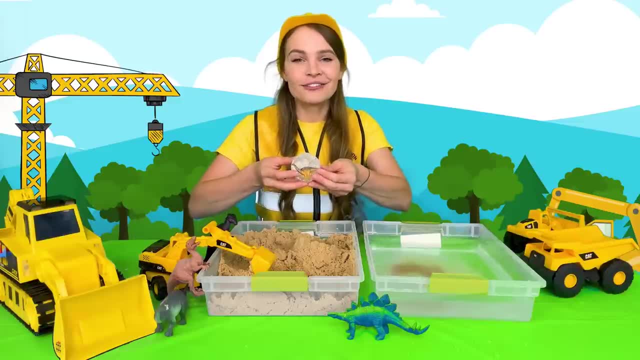 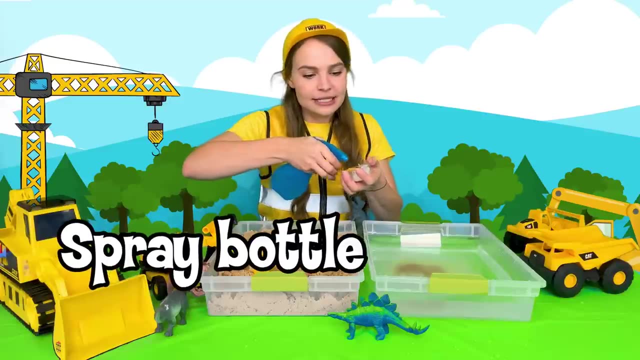 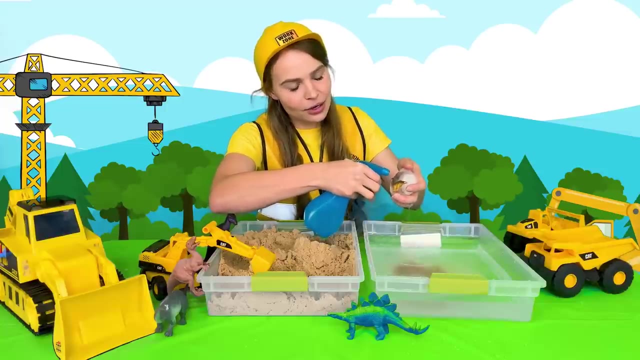 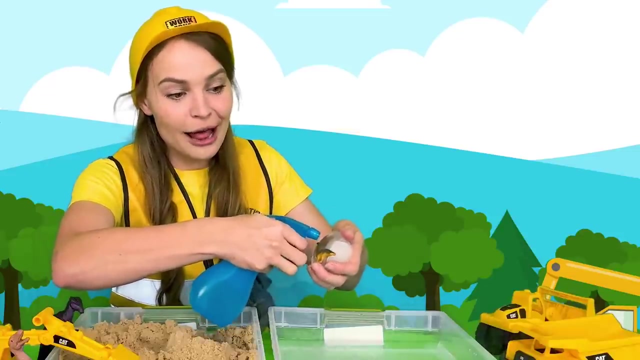 this one is frozen resin. let's help rescue this dinosaur from the ice. I've got a spraying bottle. let's see if we can spray the dinosaur and help him get out of the ice. spraying the dinosaur, we have something cold like eyes. putting warm water on it will help defrost it–. 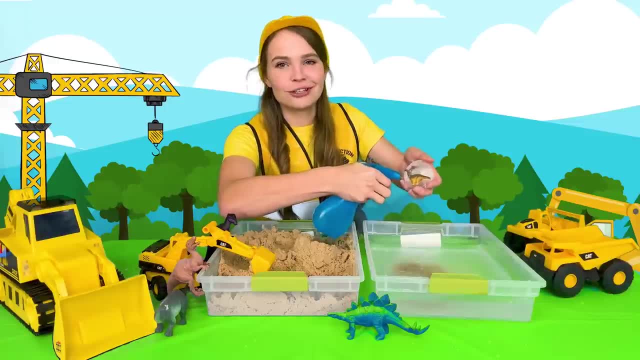 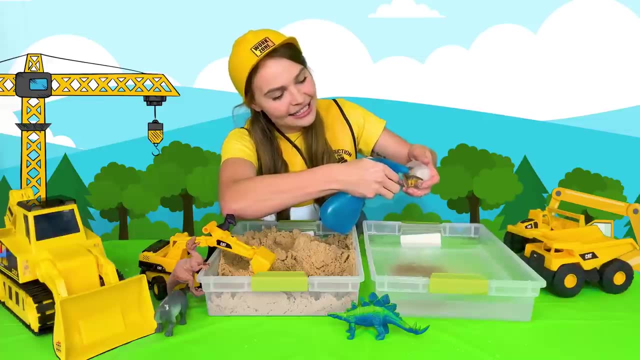 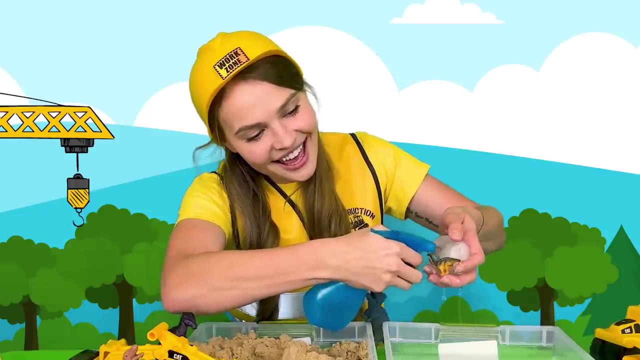 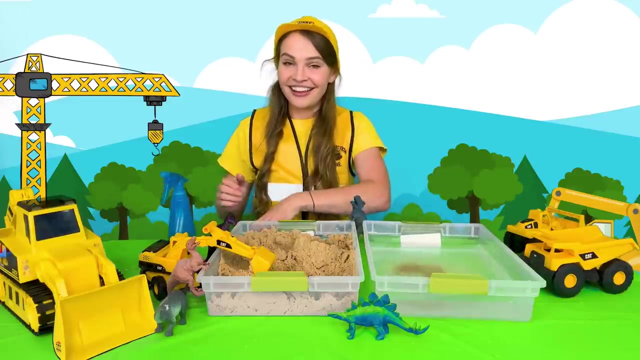 look at that. Look at that. We almost got you little dinosaur. Let's keep spraying. I think he's almost out of the ice Spraying the dinosaur. Look at that. You can play this fun activity at home if you ask your grownup for help. 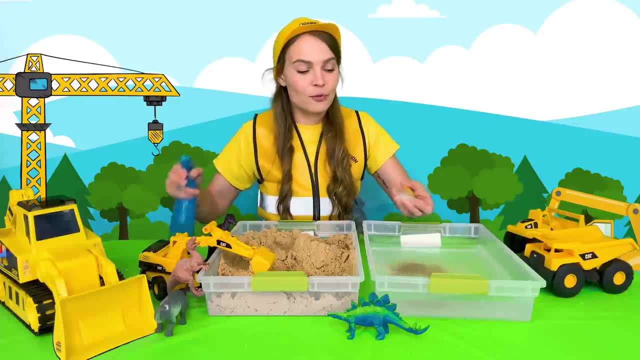 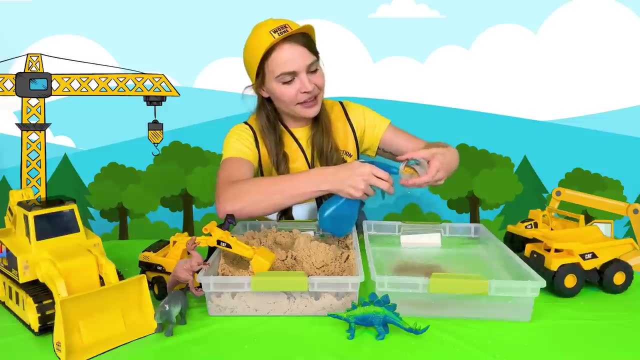 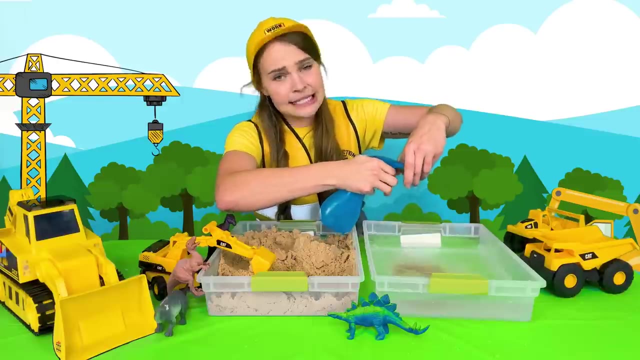 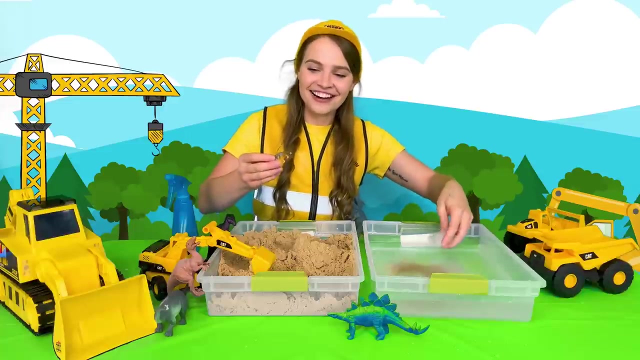 You get some little dinosaurs, put them in some water in a muffin pan and freeze them up. Then you can help her rescue them with a spray bottle. We got you dinosaur, We got him out. All right, Here you go dinosaur. 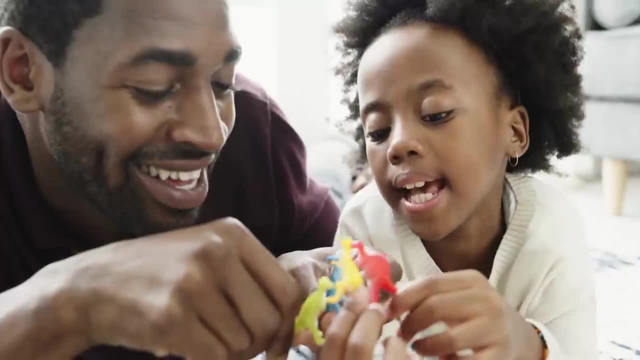 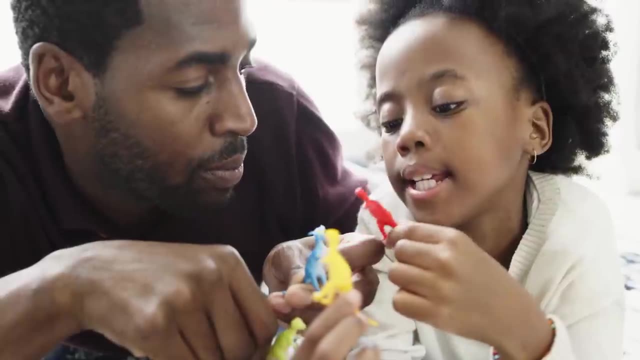 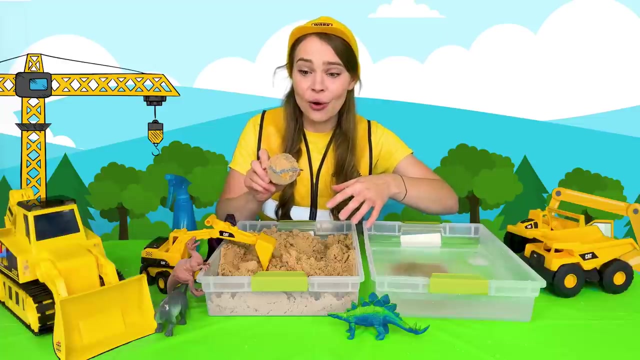 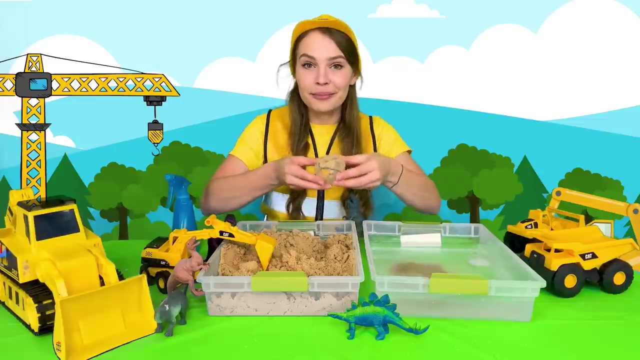 Go swimming. Let's see who else we can find. Dig, dig, oh wow, I think I found another frozen dinosaur. We can use a spray bottle again, or another fun activity is: if you have another bin of water, you can put the ice in the water. 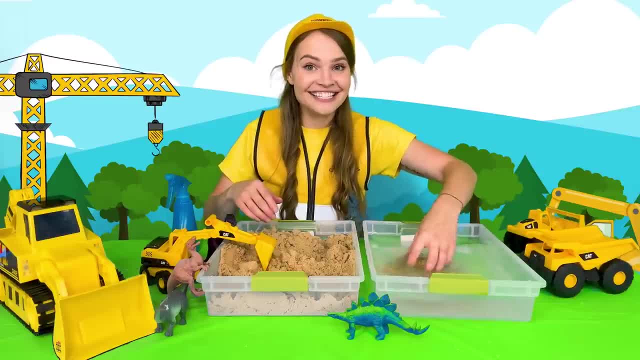 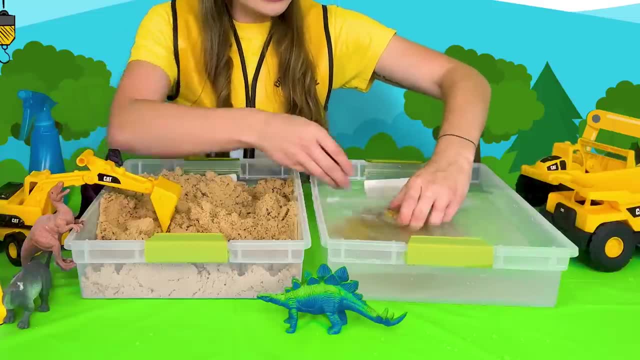 and that's gonna help melt the ice around the dinosaur. Melt it, melt it, melt it so he can come out, Melt, melt ice. Let's help him out a little more with a spray bottle. Here you go, dinosaur. 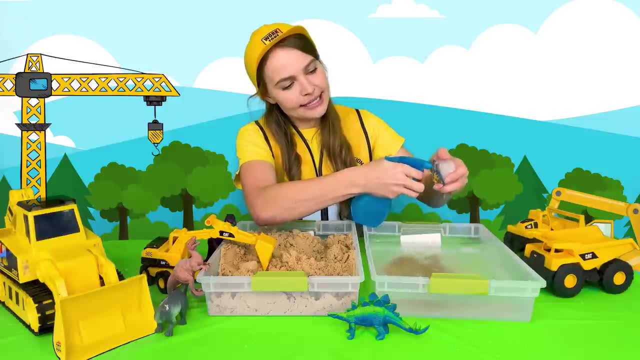 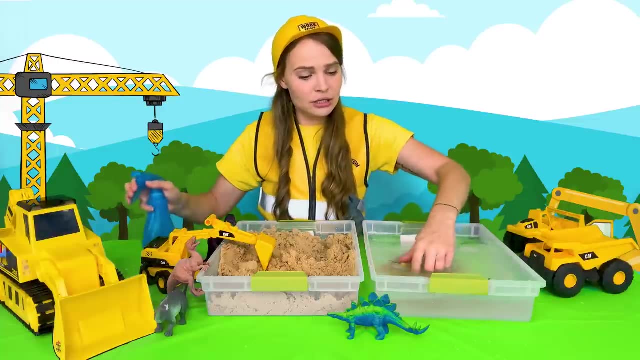 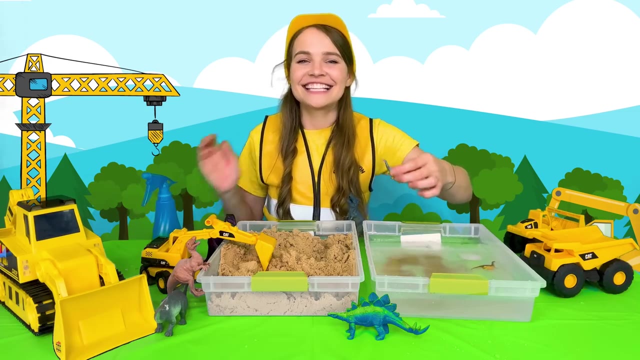 We got you All right. I think he's almost out. See if we can let him swim some more. Swim, swim dinosaur. And we got him out of the ice. Thank you for helping me. OK, ready, You want to spray it? 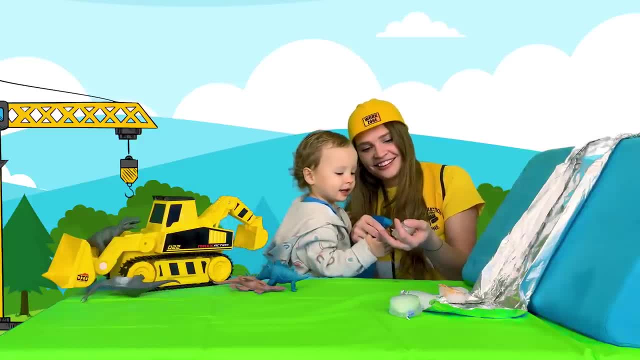 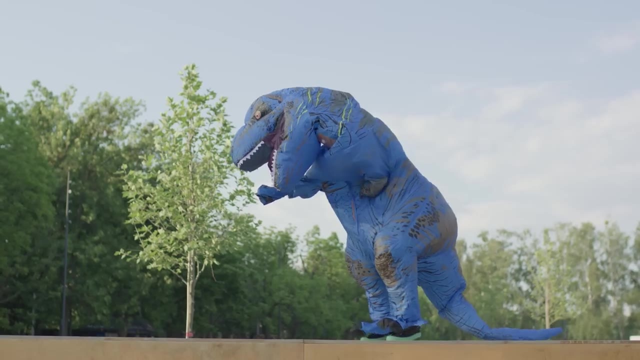 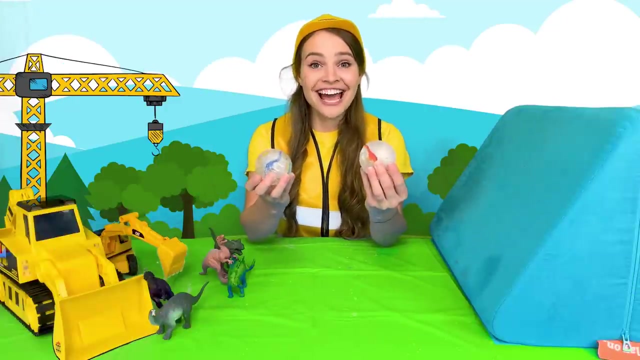 I'll hold it for you, Keep going, keep going, Spray, spray, spray. Oh, You see ice coming out of the ice. Looks like our dinosaur friends found two more frozen dinosaurs: One, two, One, two, One, two. You're gonna". 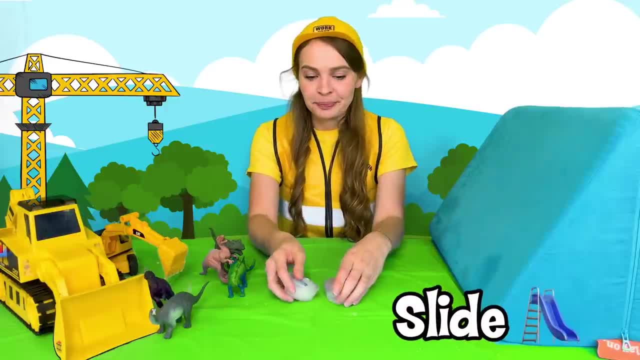 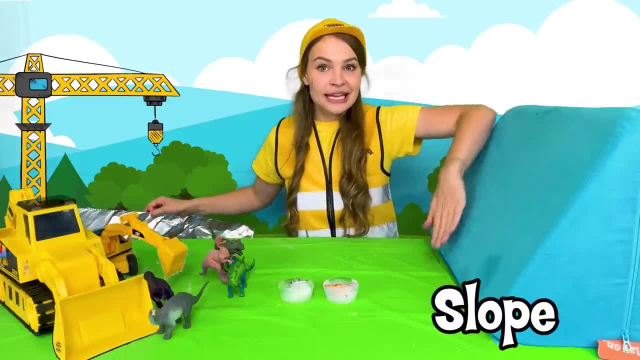 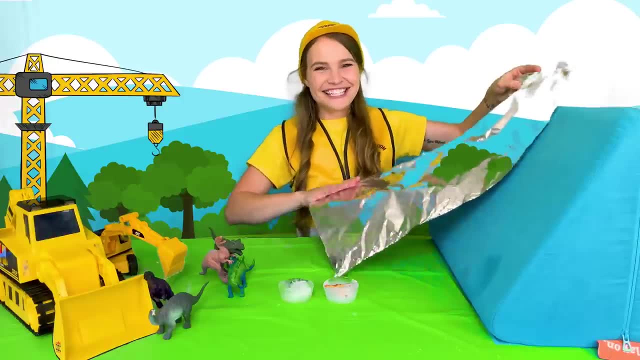 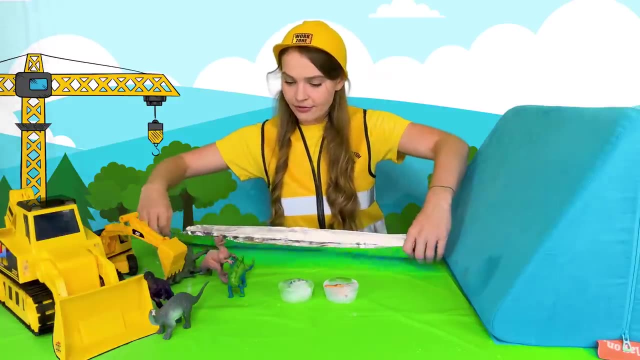 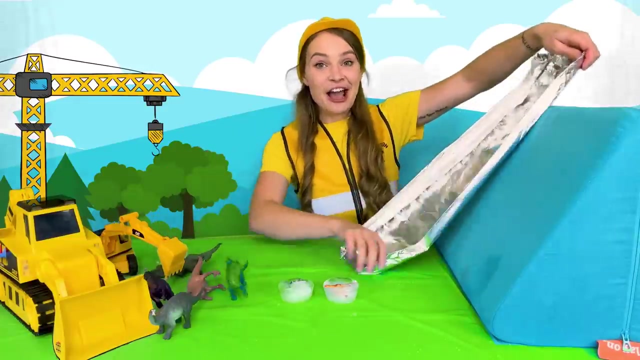 you can make a slide with a slope, something that's tilting down, and if you have some foil, you can make a little tunnel. Let's do it together. I'll fold up the sides, Fold, Fold, All right, And now we've got a little slide. 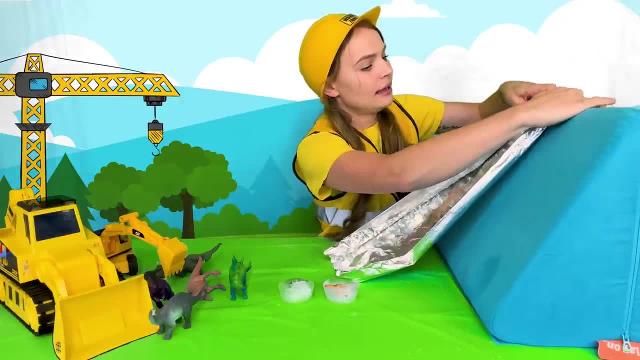 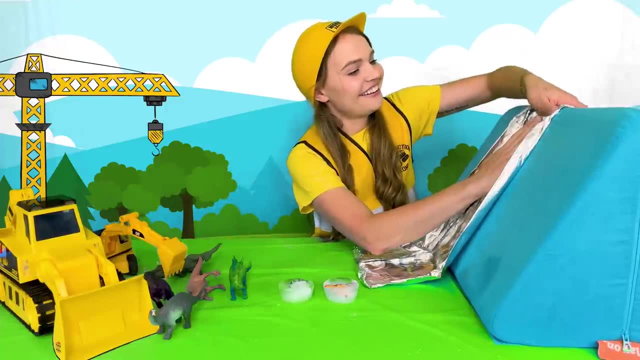 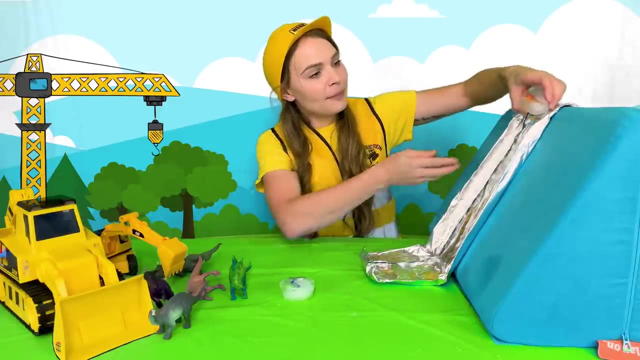 I'll bend it over this side. Keep our edges up All right, Ready. First, we're gonna put this dinosaur up and watch it slide down. Ready, Let's let it go on. three, One, two, three Slide. 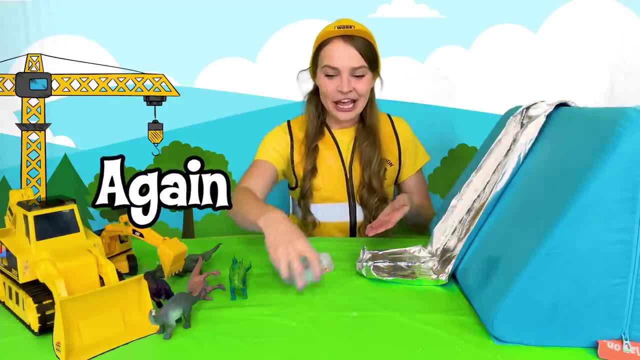 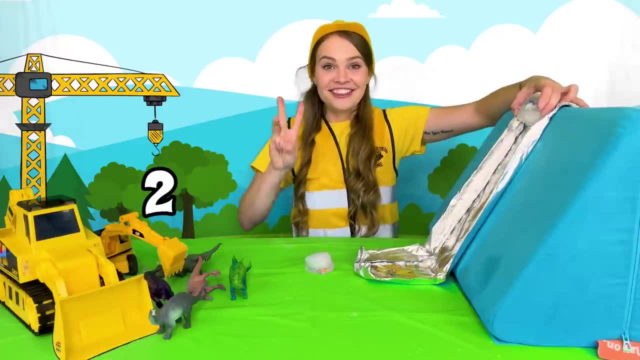 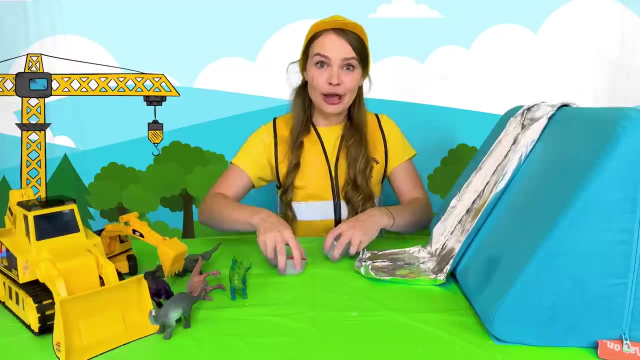 Good sliding. Let's do it again. Now we'll use this blue dinosaur. You're ready to slide? Let's let him go on. three, One, two, three, Slide. Let's do it again. Ooh, let's put him on there at the same time. 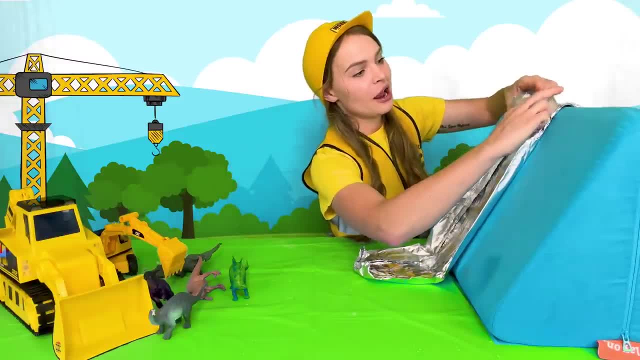 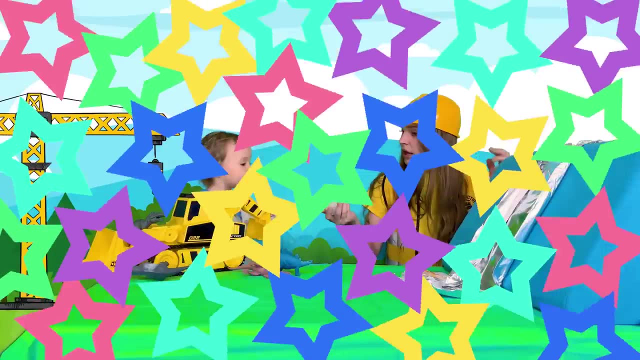 and see which dino goes down fastest Ready: One, two, three Slide- Great job. This one's frozen, but look, they can go sliding like this. This one's frozen, but look, they can go sliding like this. 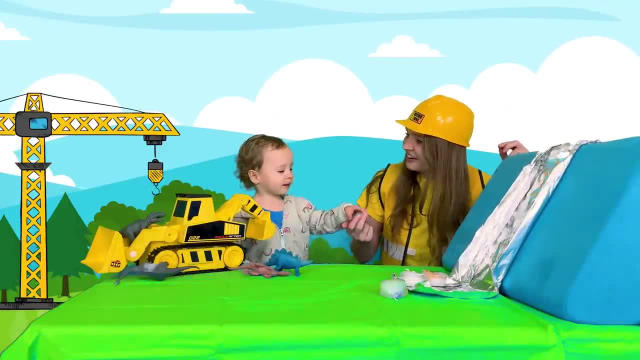 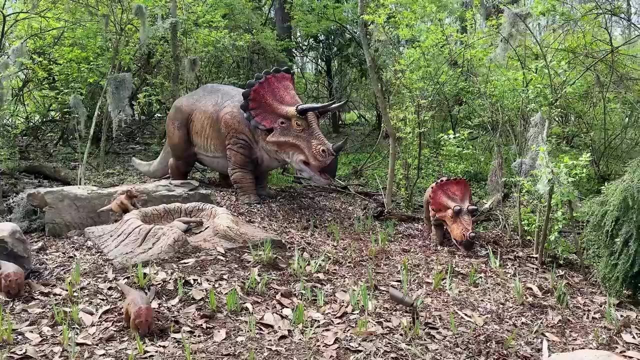 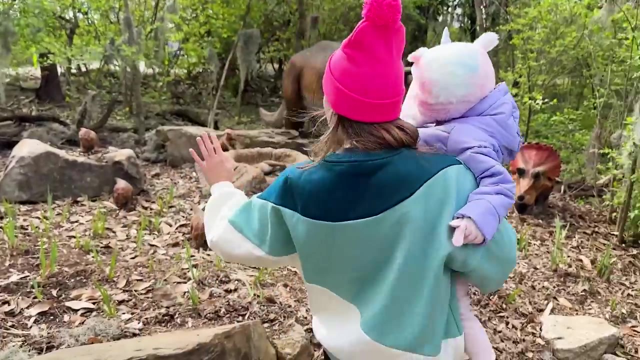 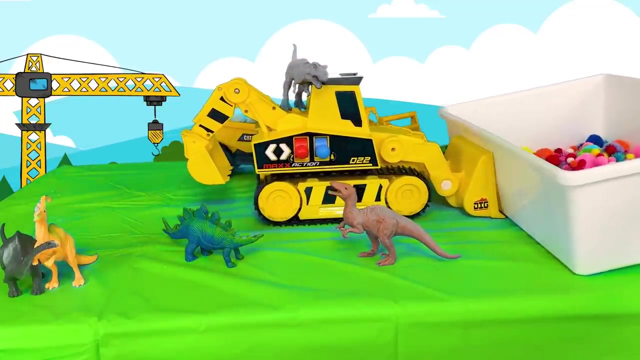 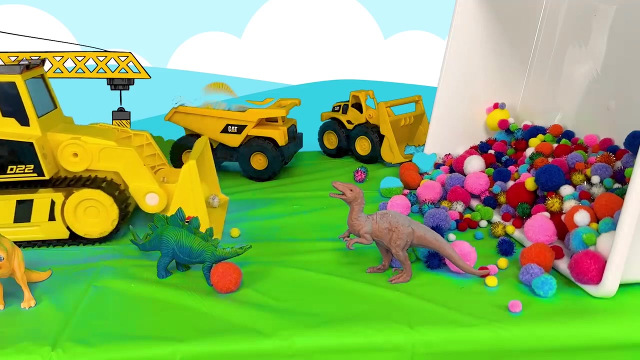 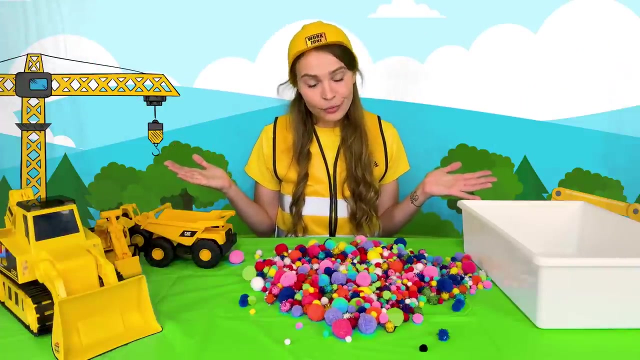 Ready Slide. You wanna do it? Yeah Yeah, It was cold, Mine was cold. Okay, ready Slide. Oh wow, look at this. Oh wow, look at this. It looks like our dinosaurs were playing and made a little bit of a mess. 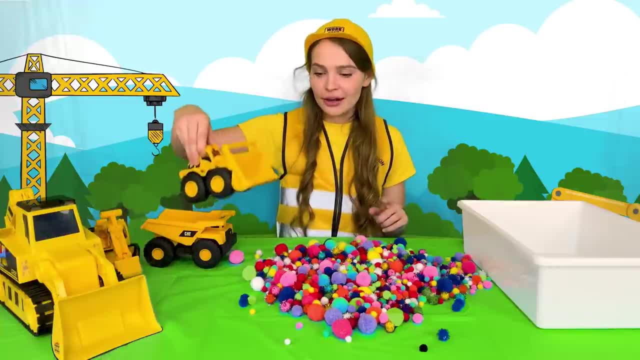 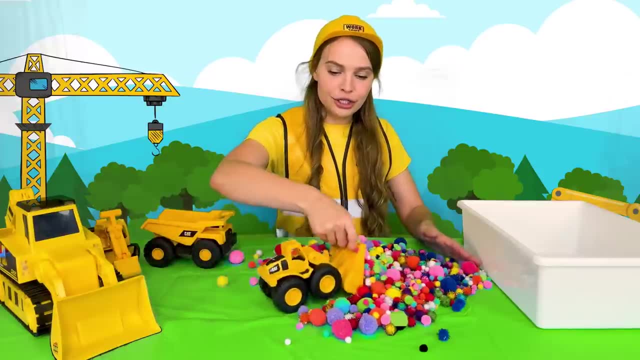 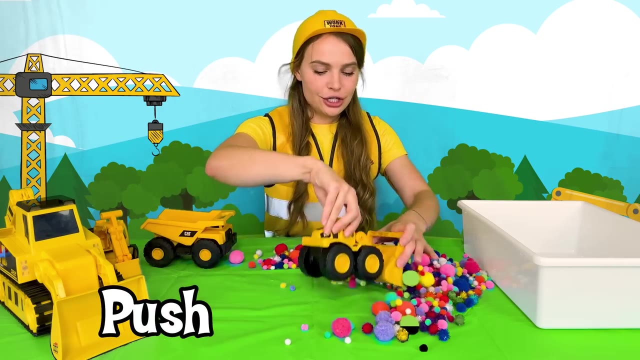 Let's clean it up. Hmm, ooh, here we go, We can push the pom-poms all in together. Here we go, We'll make a pile, Push, Drive, drive, Push them together, Push, Push, Push. 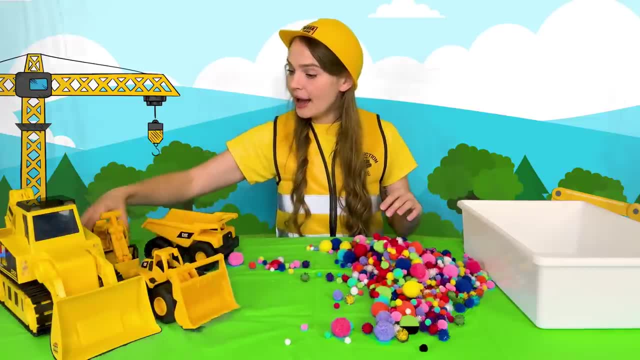 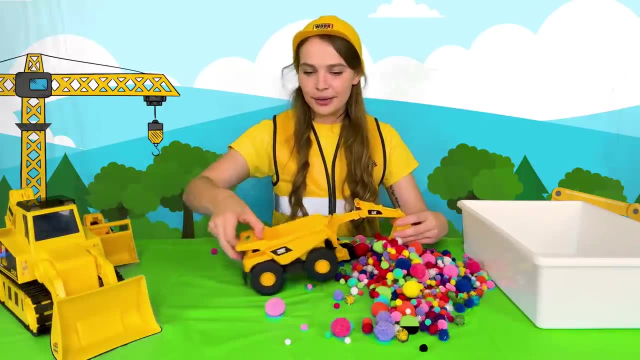 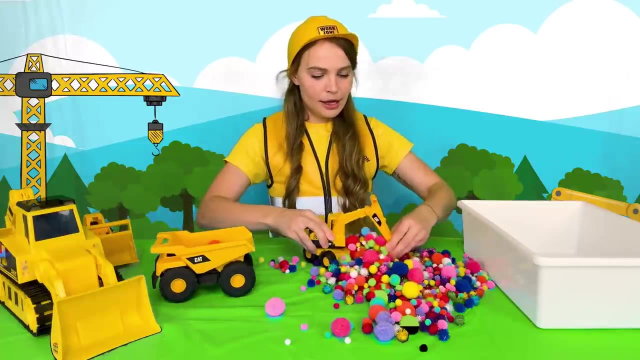 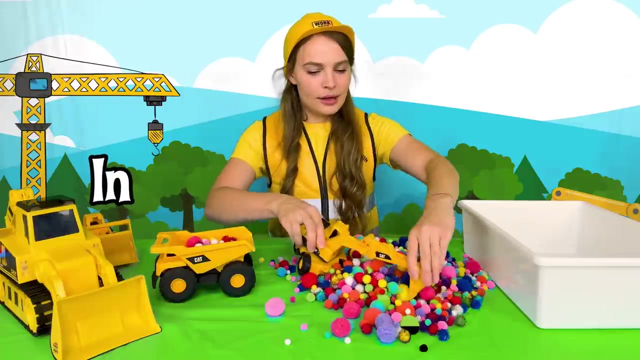 Push. All right, Now we can use the excavator to pick them all up and load up our dump truck. Here we go: Pick some up, put them in. Pick them up, put them in, Pick them up, put them in. 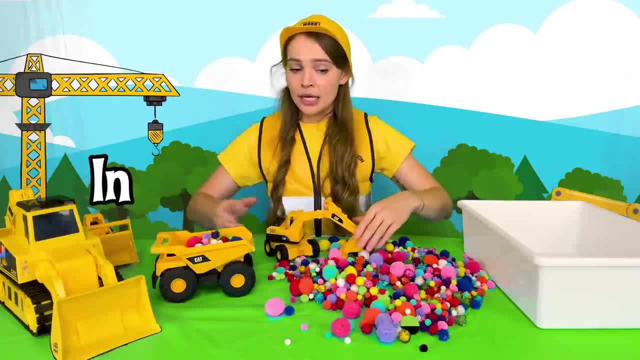 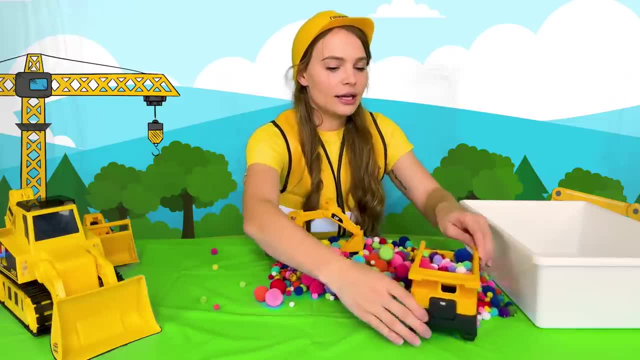 Pick some up, put them in. Pick some up, put them in. Pick some up, put them in. Okay, I'm full, Let's go drop them off in the bin Drive. drive Here we go And out. 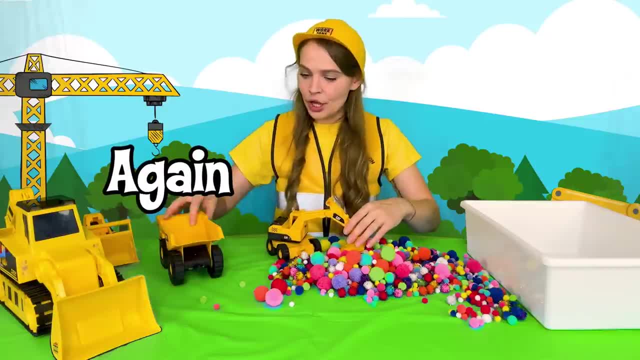 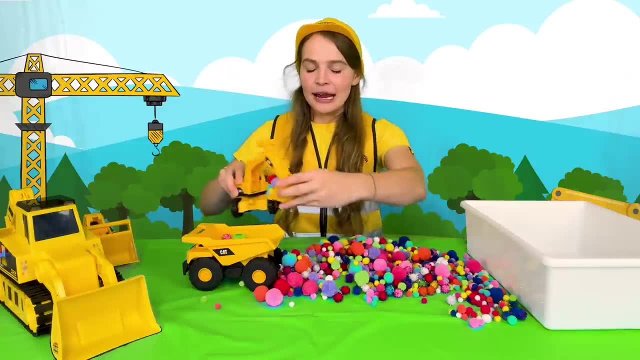 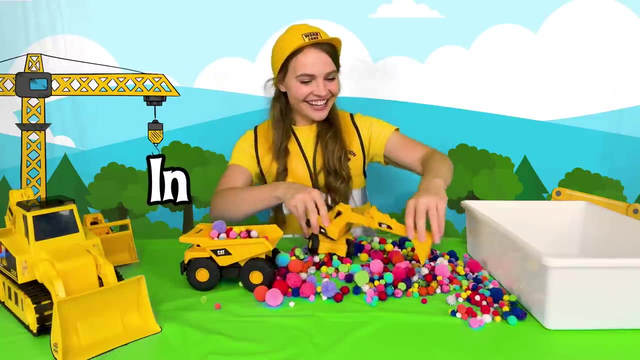 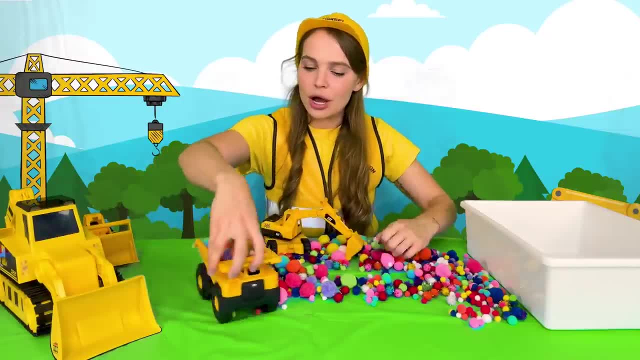 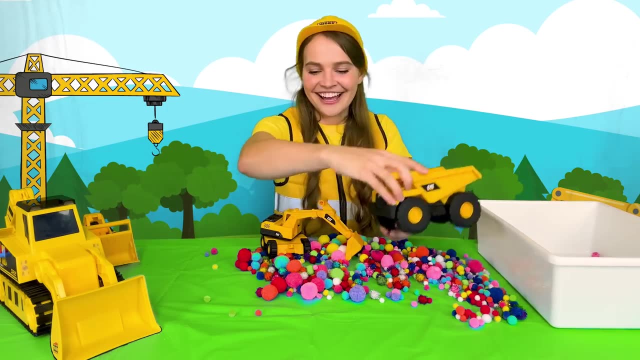 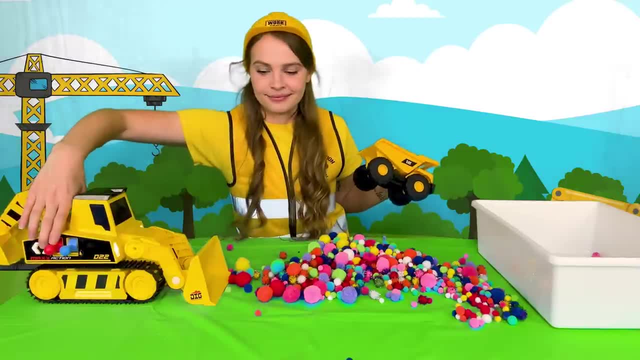 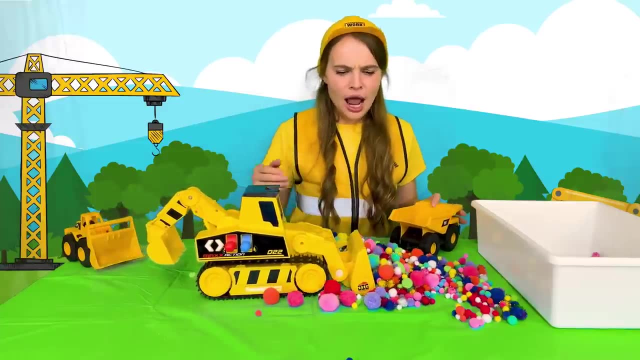 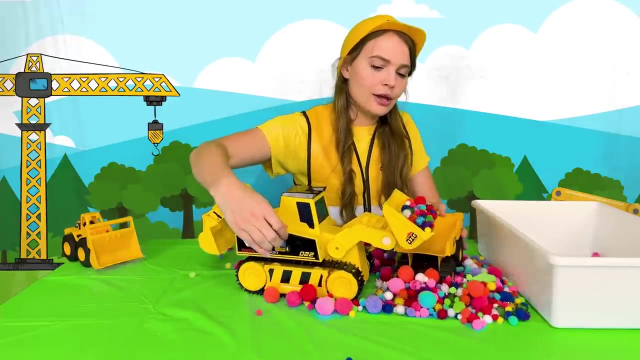 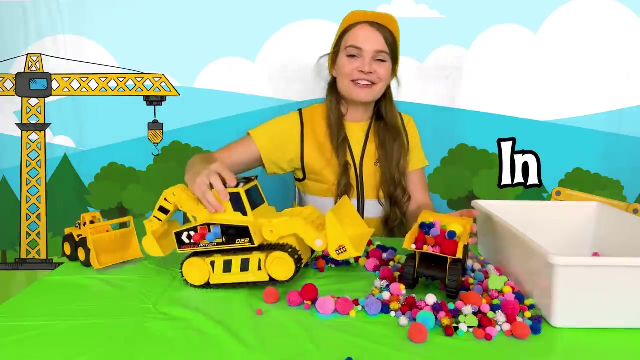 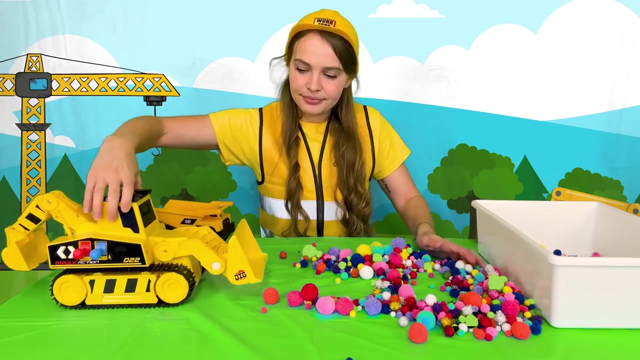 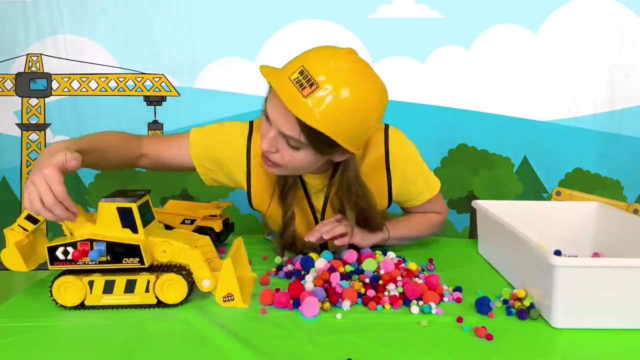 Let's turn it on, Scoop them up, all right, and let's put them up and load them up in the dump truck and we'll put it in in the bin. all right, let's do that again. let's lower this there. y'all go, pick them all up. 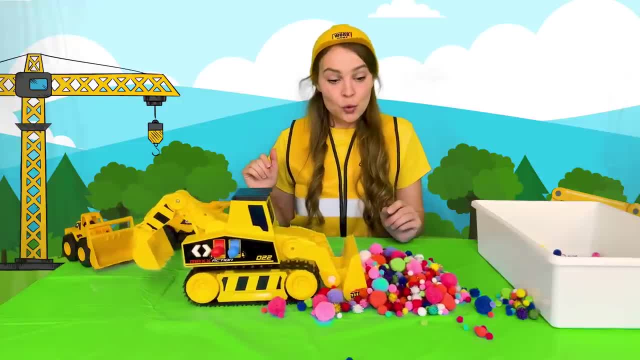 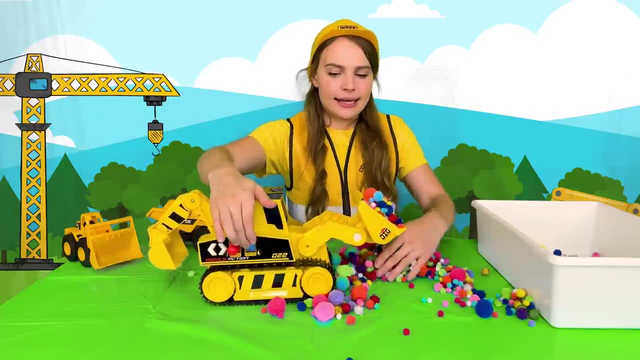 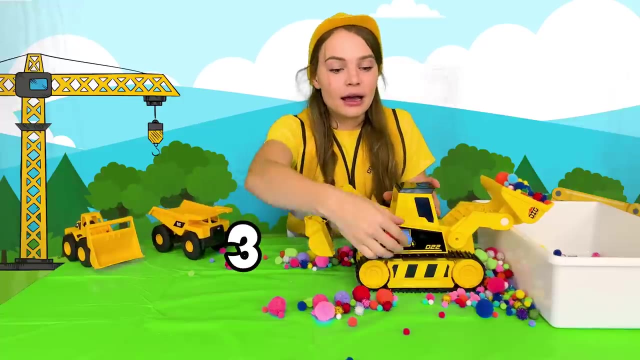 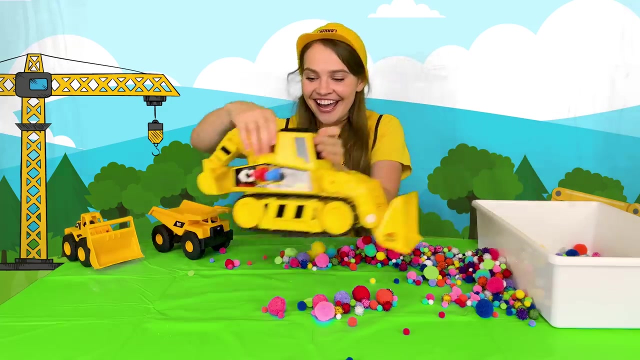 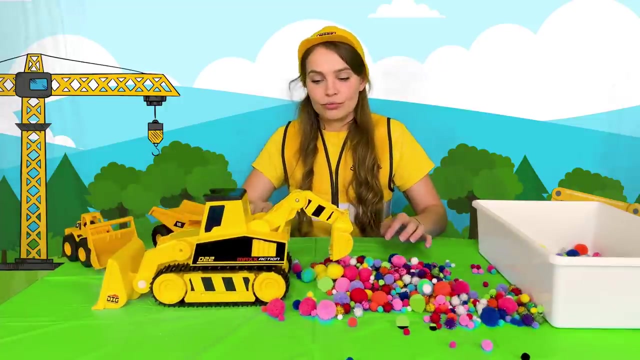 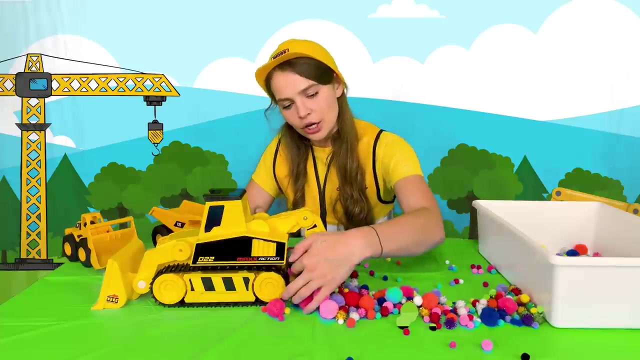 all right, load them up. we'll pick it up and let's just drive over to our bin and we'll put it out on three. one, two, three. all right, let's see if we can use this side. here we go. oh, we picked up a few, let's try it again. there you go. oh, now we got many, let's go. 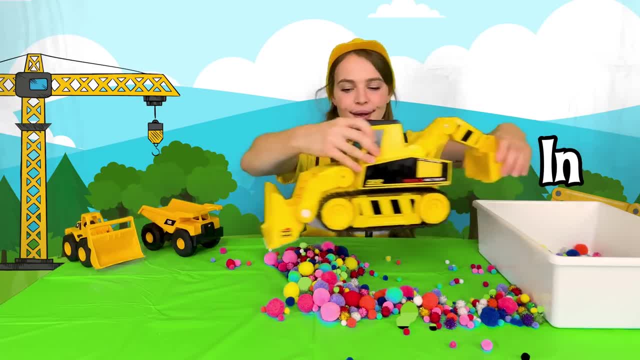 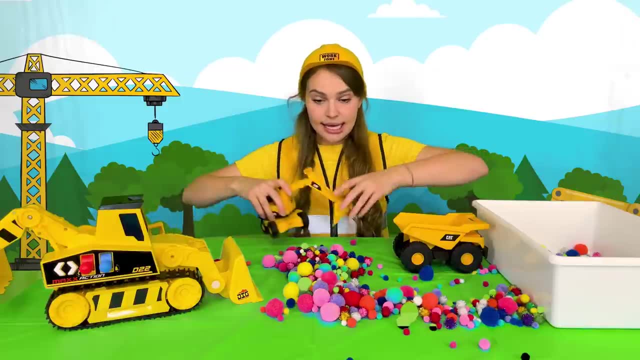 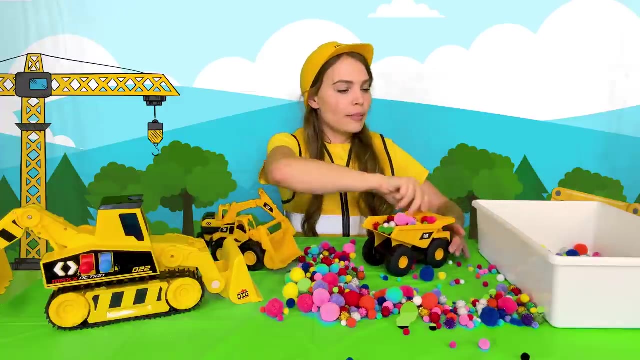 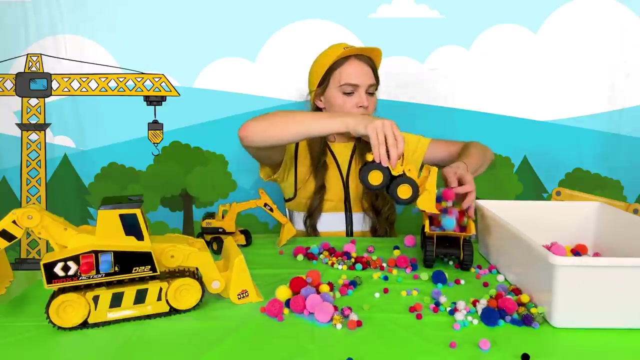 drop them off, drive, drive and let's load up some more. here I am, says the dump truck, load it up. here's the excavator too. I'll help put them together in the dump truck. I'll drop them off. down we go, let's load up some more. load them up in the dump truck, drive, drive. 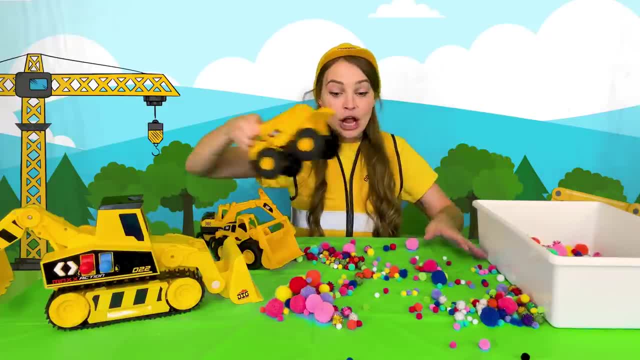 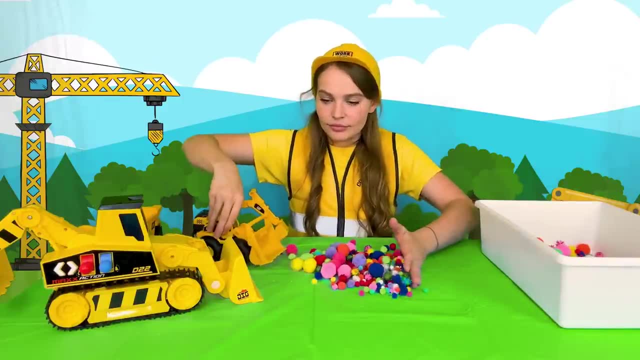 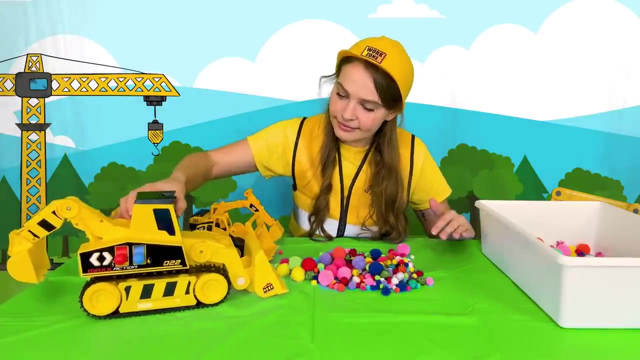 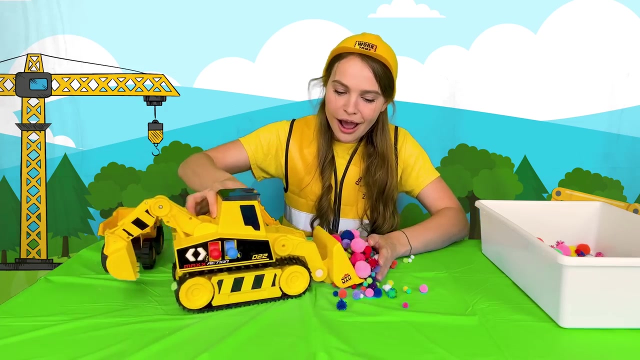 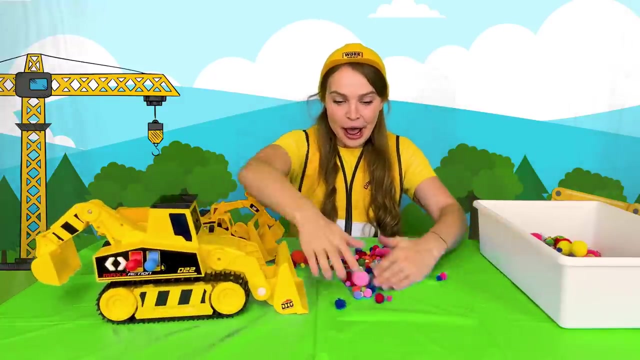 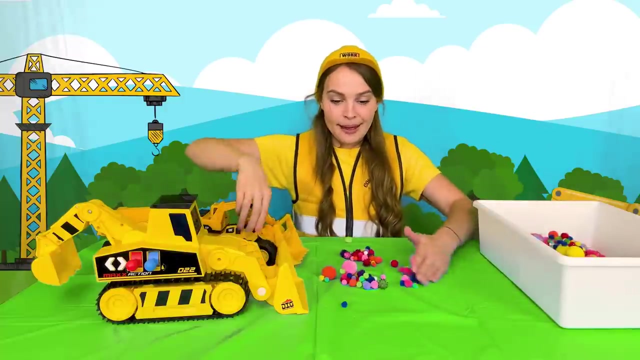 drop them off. look at this, we almost cleaned it all up. let's put them all together. here we go. here we go. here we go, pick them up and dump them in. great job, we have a little bit more. I'll help. I'll help pick them all up, drop them in, pick them all up. 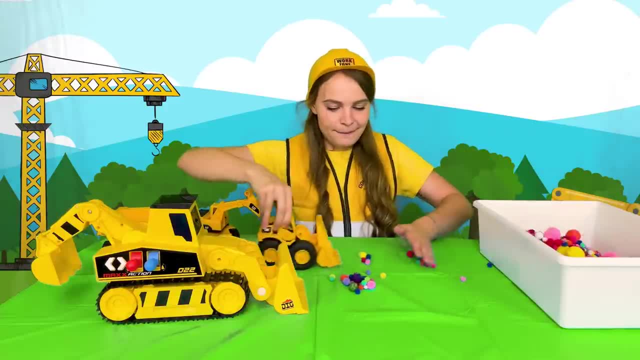 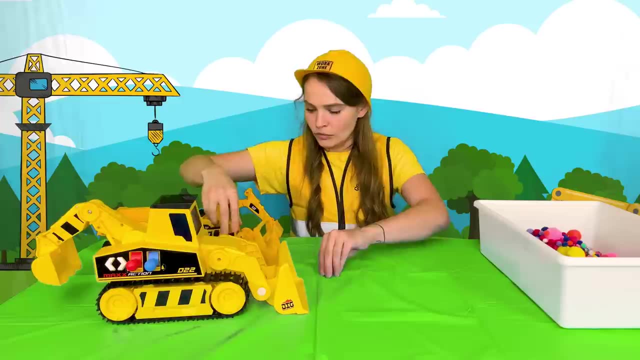 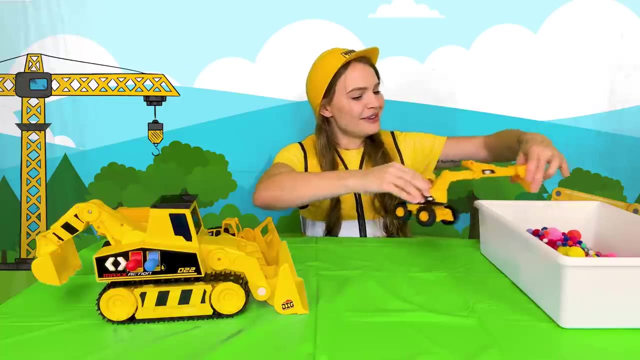 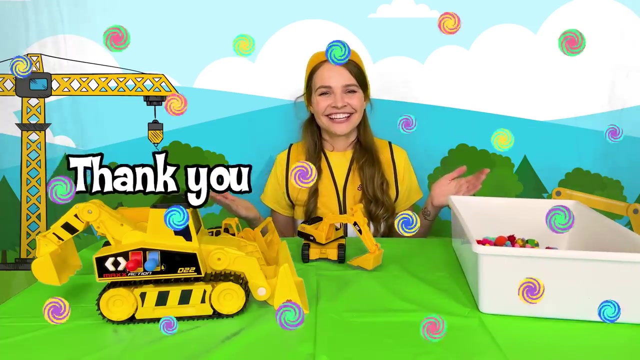 drop them in. pick them all up and we'll drop them in. there's three left. I'll get them, says the excavator. put them in my bucket drive, drive, dump them in. all right, look at that. we got all of the pom-poms back in the bin. thank you for helping me. 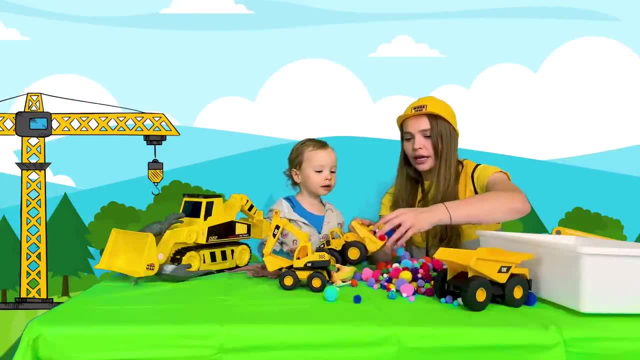 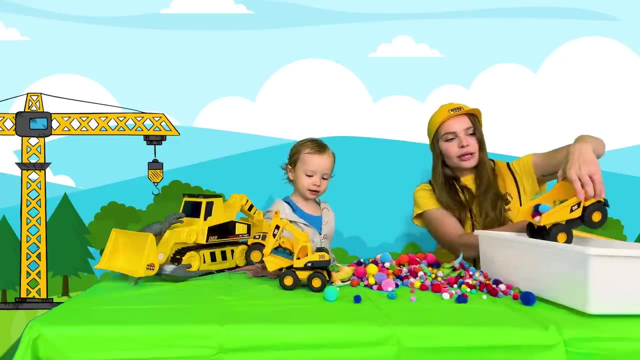 and they spilled. so I was going: okay, put it in here. will you hold me? put it in here, put it in here. will you hold me? put it in here, put it in here. will you hold me? put it in here in the dump truck? Hey Well, the dinos were playing. I'm going to dump it in. The dinos were playing. 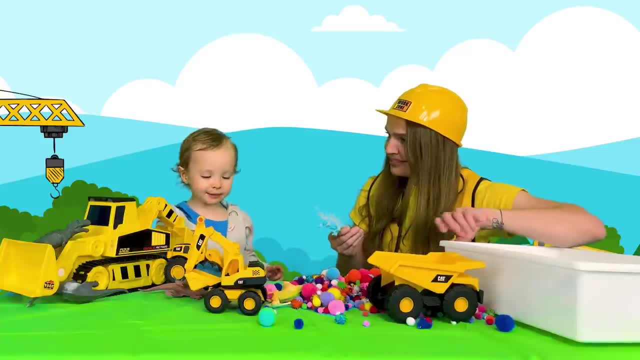 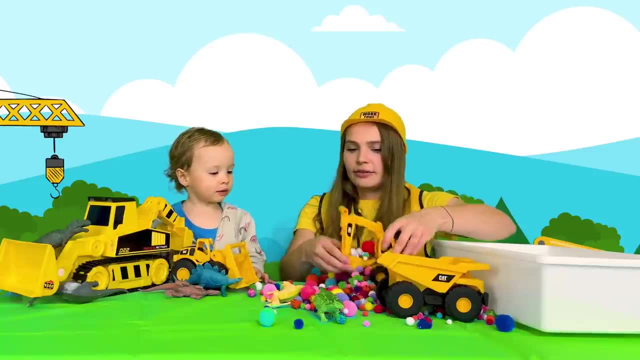 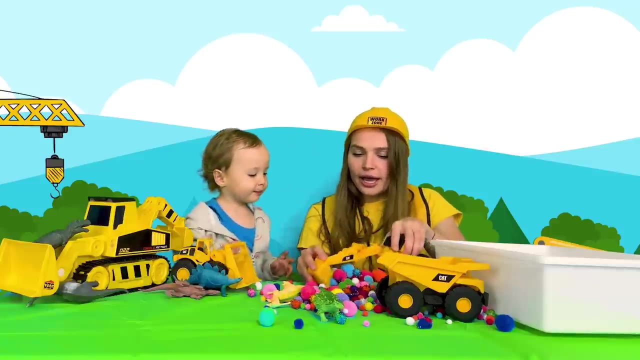 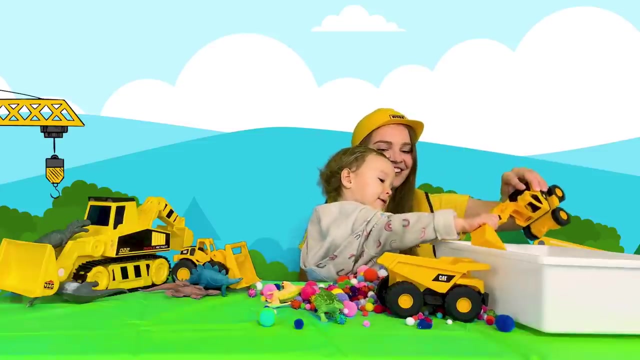 They got pom-poms everywhere. I was playing with these dinos and they made a mess. So I said: here, dinos, we can help clean up the excavator. Where should I put this Paisley In the bin? Here we go, Okay, Thank you. Thank you All right, Perfect, Want to do it again. 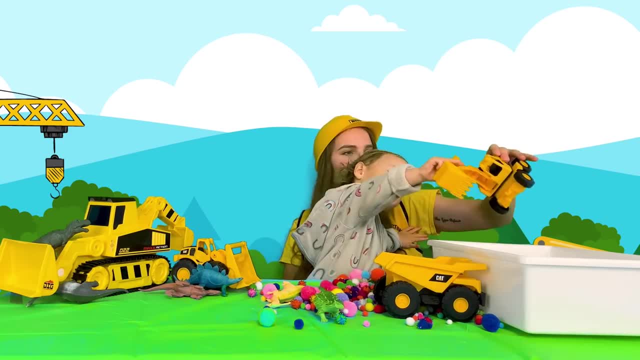 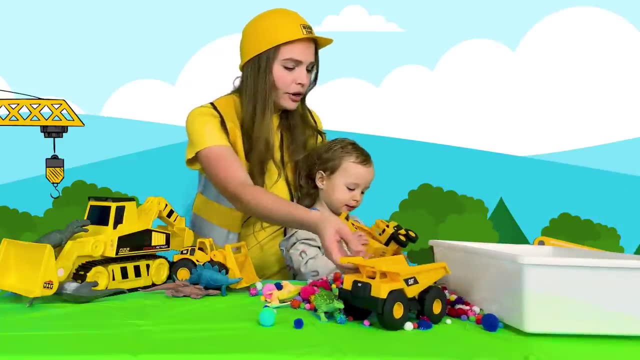 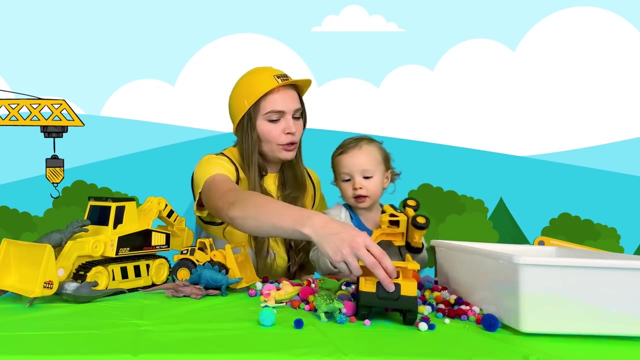 Good scooping, Perfect Drive, drive. Oops, I got stuck on the tire. Here we go, Drive, drive. Put those pom-poms in. girl Nice, I'll help you load it up. Beep, beep. 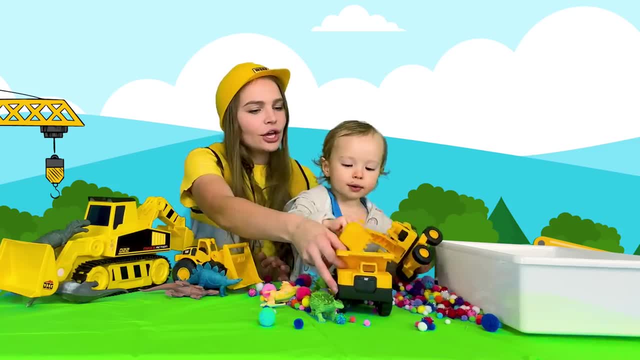 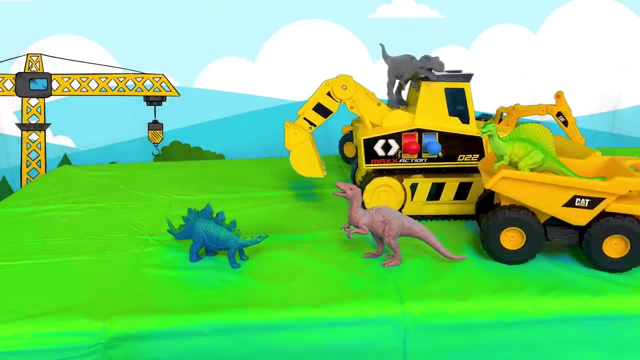 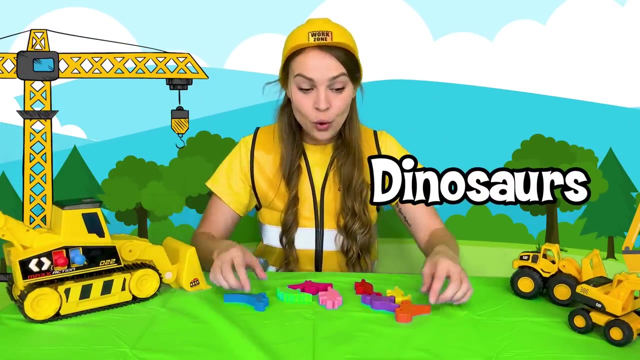 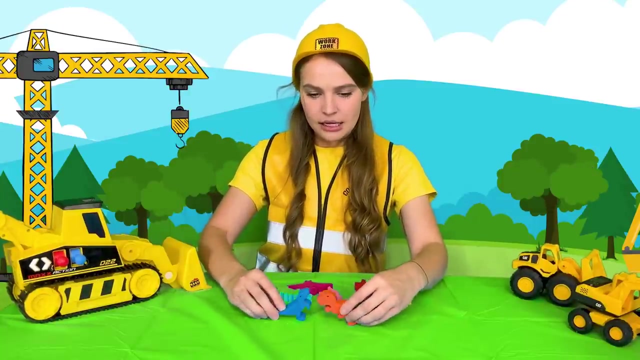 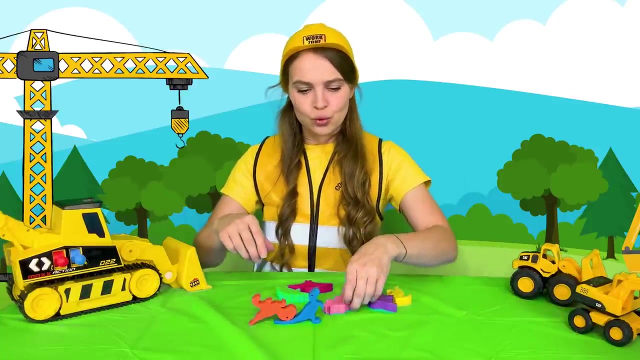 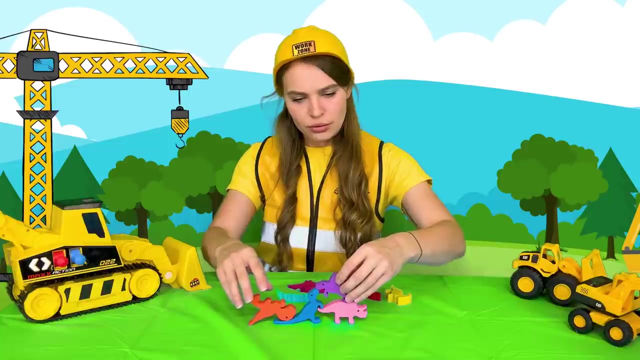 Skip, Here you go, Thank you. Thank you, I've got some more dinosaurs. Will you help me stack them? All right, See, we'll start with one, two, three, Maybe this way: Ooh, We've got Triceratops. Here we go, Ooh. 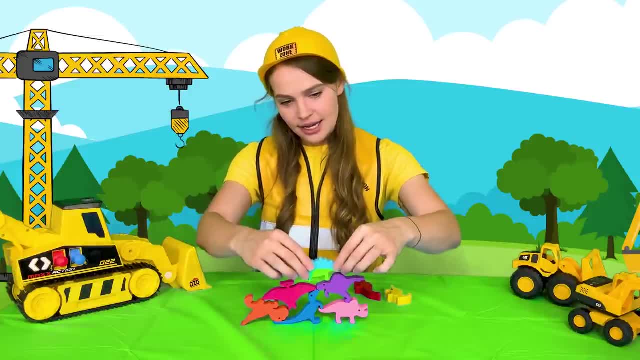 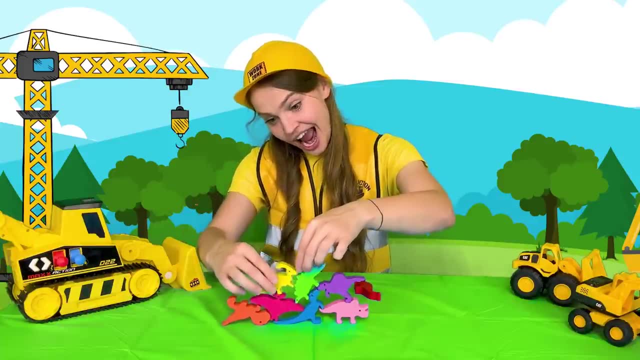 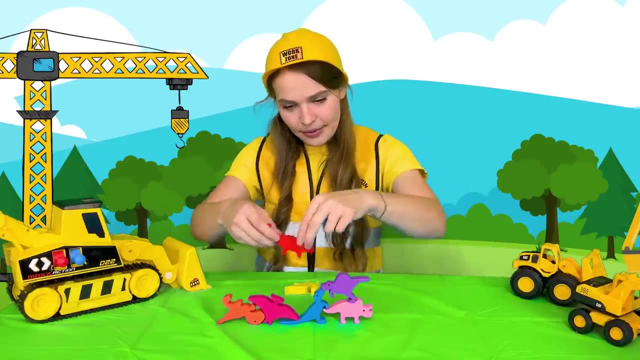 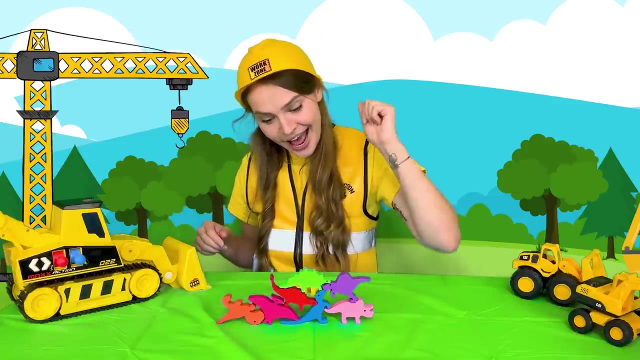 On. Let's put this one on. Ready On This one. Oh no, My dinosaurs fell down. Let's try it again. Let's see, Maybe we'll put this on here. Ooh, Let's stack this one on top. 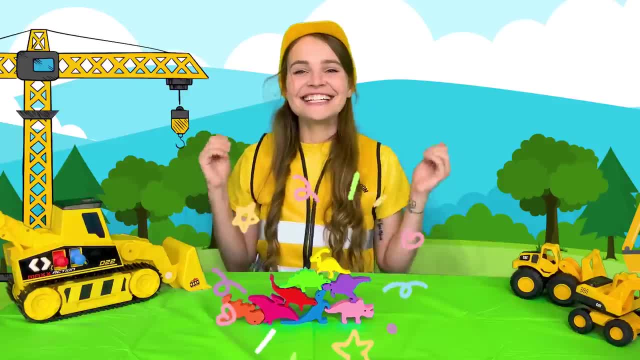 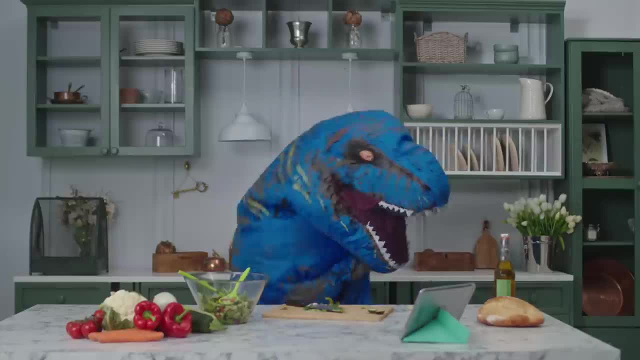 Let's see if we can put this one here. We did it, Yay, Thank you for helping me. Thank you, Stay tuned. We found a dinosaur. It's Triceratops. Stay tuned, Stay tuned, Stay tuned. 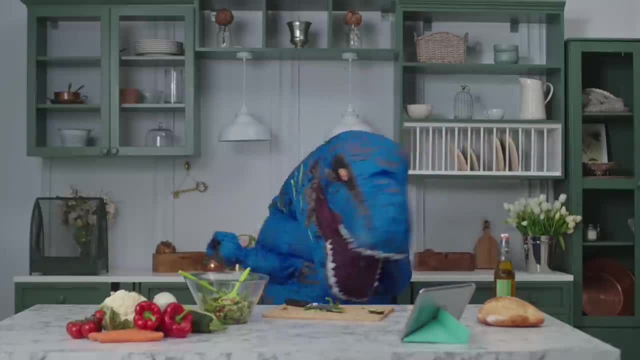 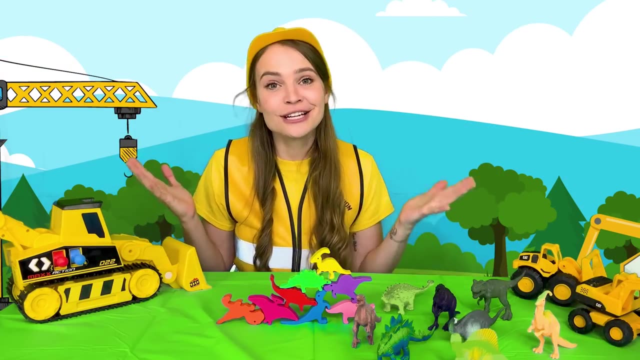 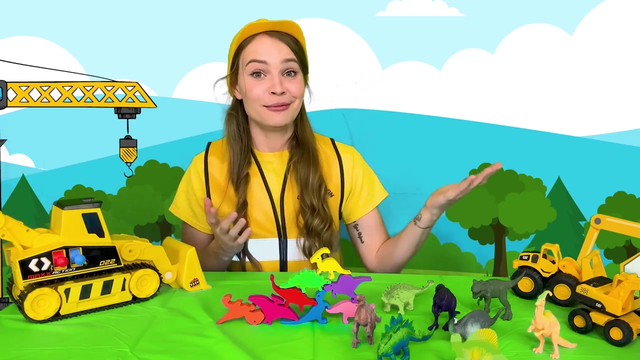 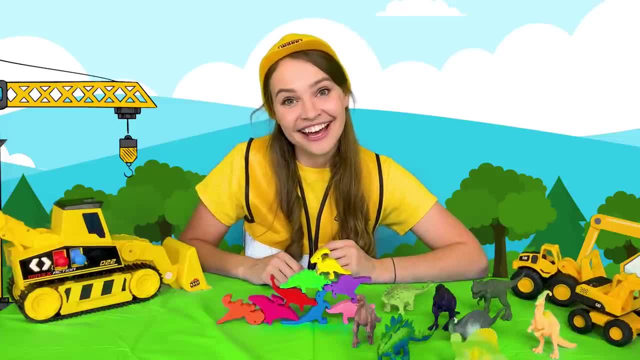 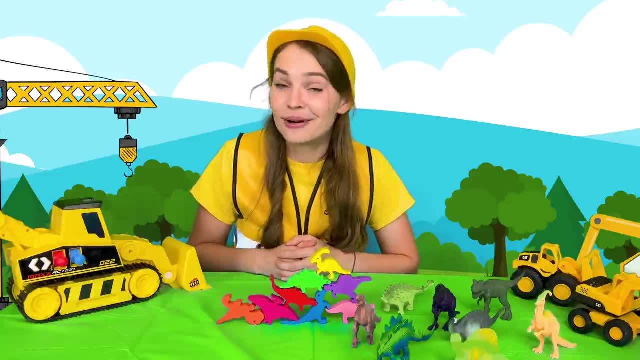 to dump out all of our pom poms. That was really fun. Thank you so much for playing with me. I love playing with you and I'm really proud of you. Well, that's the end of this video, but if you're looking for more of our videos, make sure you search for Teezy's Corner. 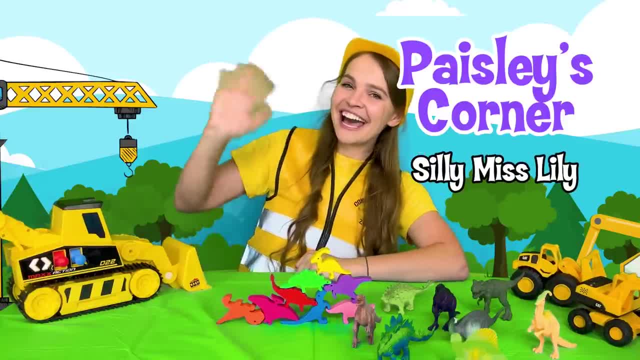 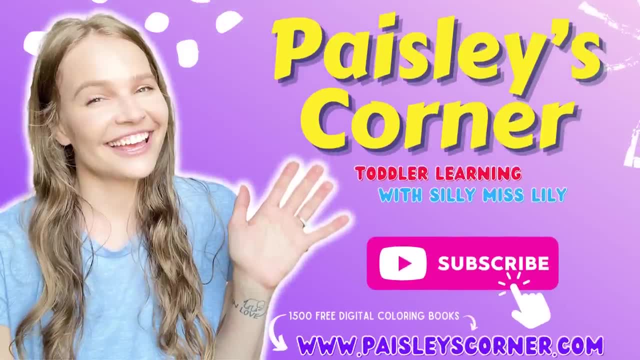 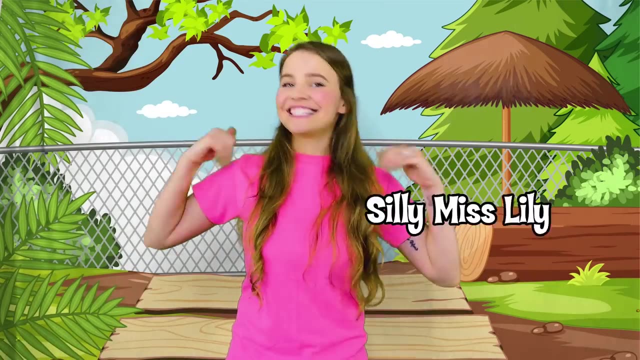 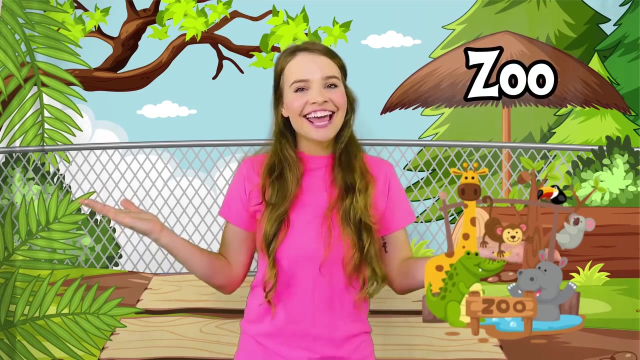 with Silly Miss Lily and I'll see you then. Bye-bye, Bye-bye, Hi friends, It's me, Silly Miss Lily, and I'm so excited to play with you today. Today we're going to take a trip to the zoo and learn about animals and our ABCs. I'm so excited. 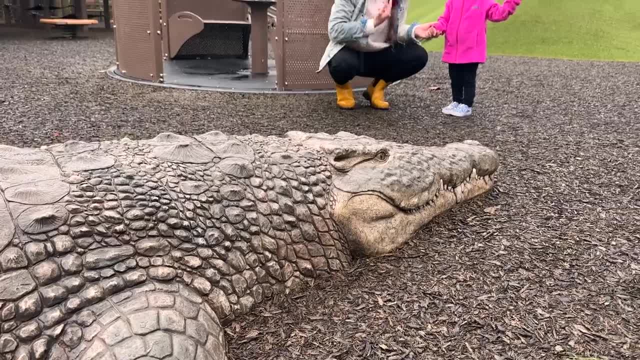 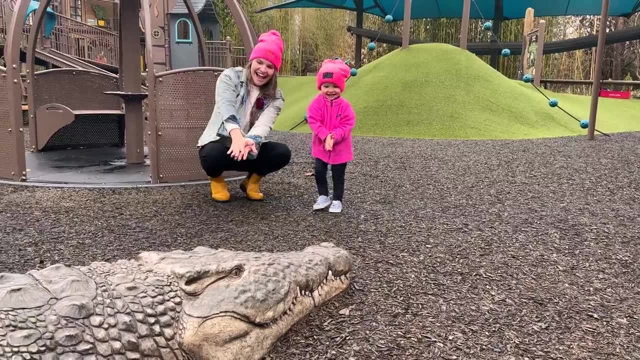 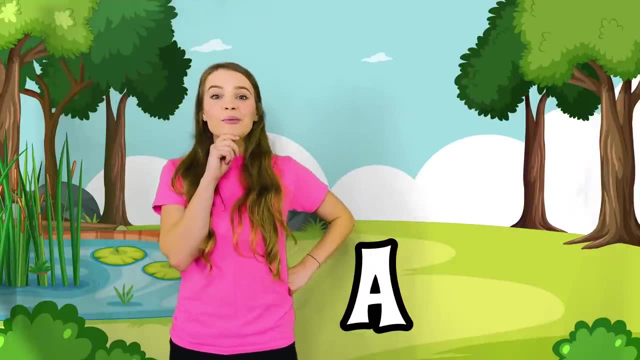 to play with you and explore. Come on, How about this alligator? How do they chomp Chomp, Chomp, Chomp, Chomp, Chomp? Hi alligator, How are you Walking, walking through the zoo? Hmm, Let's see who we find first. Oh, 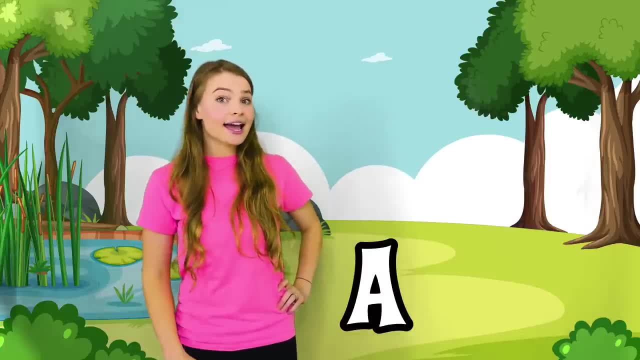 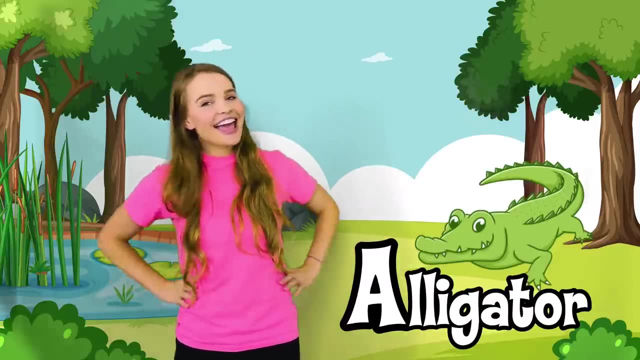 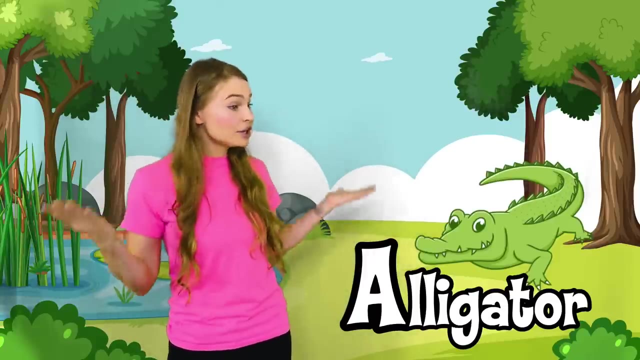 look, Here's letter A and oh wow, An alligator. Hi alligator. Alligator, That's a big word and a fun one. Hi alligator, How are you today? Alligator says hello, Say hi, alligator. 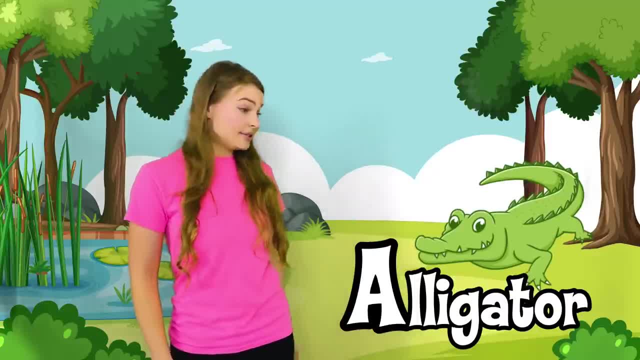 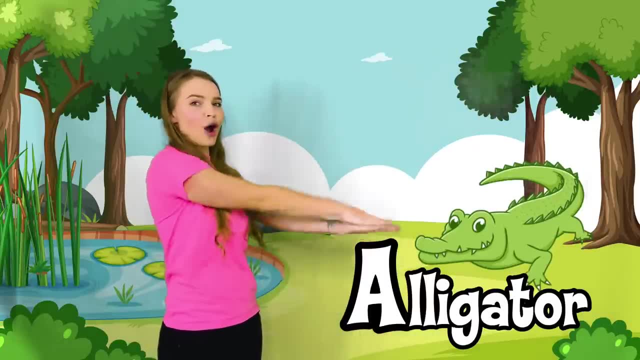 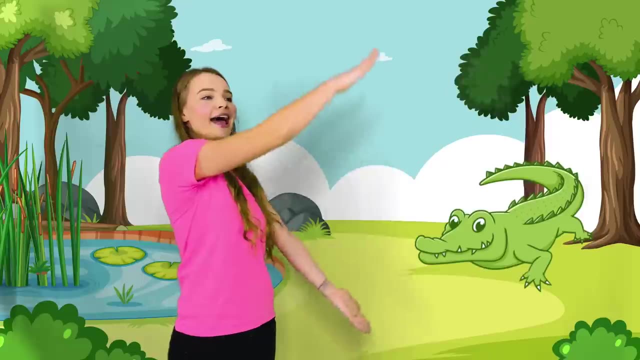 You've got a really pretty green color. How about alligators Go like this: Hello, Chomp, chomp, chomp, Alligator, Will you act like an alligator with me? Alligator, Wow, Hey, alligator. 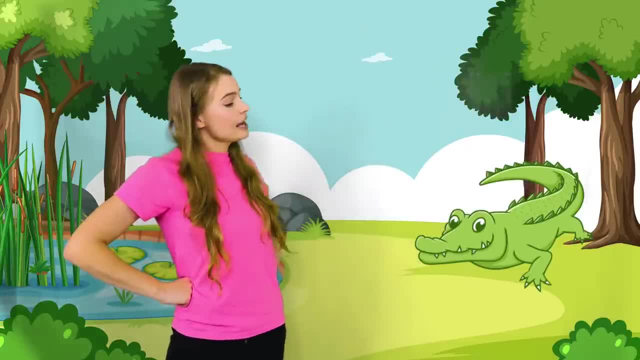 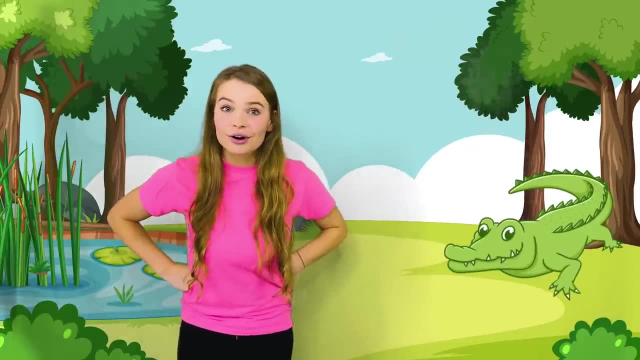 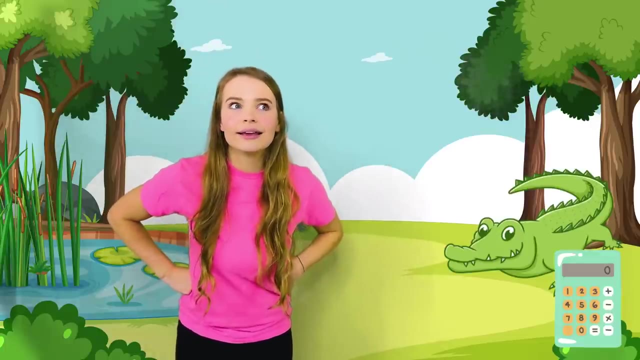 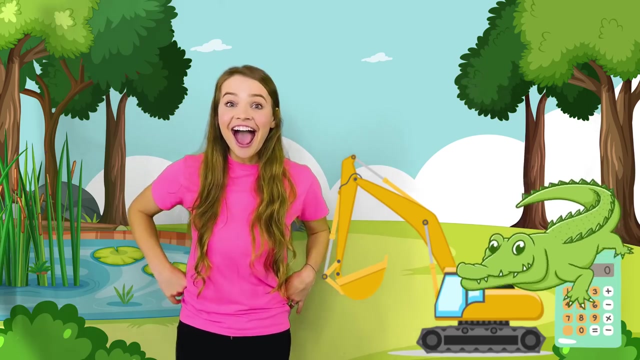 Oh hi, How you doing Alligator. do you like rhymes? Well, you're just. yeah, Okay. how about an alligator who likes a calculator in an excavator, saying: see you later. What Alligator with a calculator? 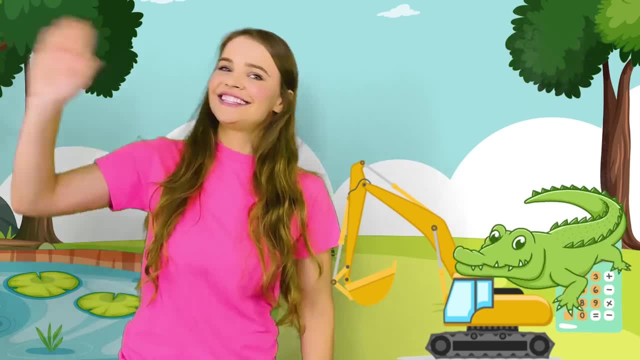 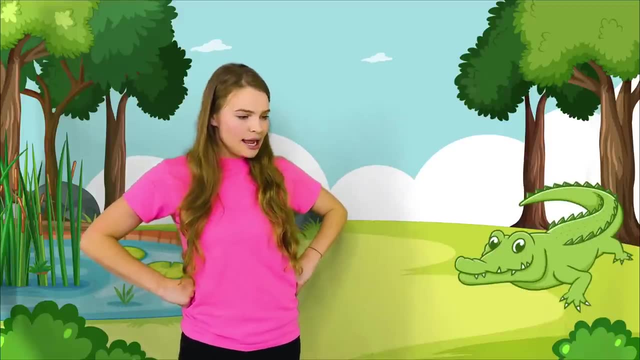 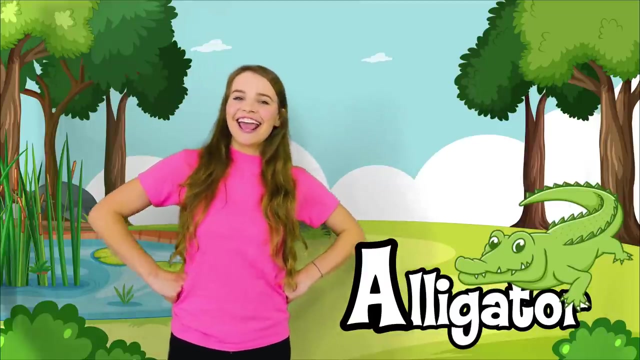 in an excavator saying: see you later. How silly Alligator, it was very nice to meet you. And you start with the letter A. A makes the ah sound, ah, ah, alligator. A makes the ah sound, ah, ah, alligator. 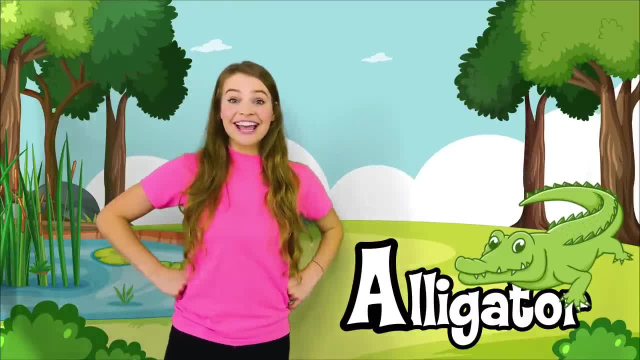 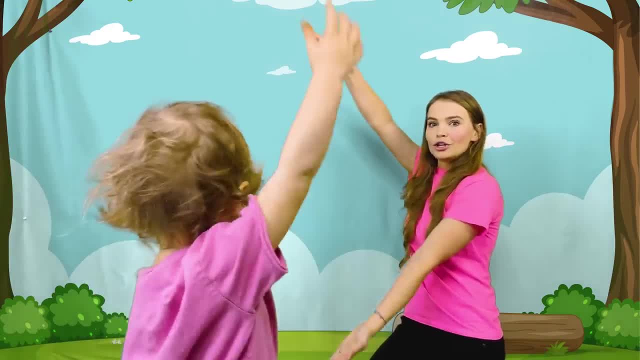 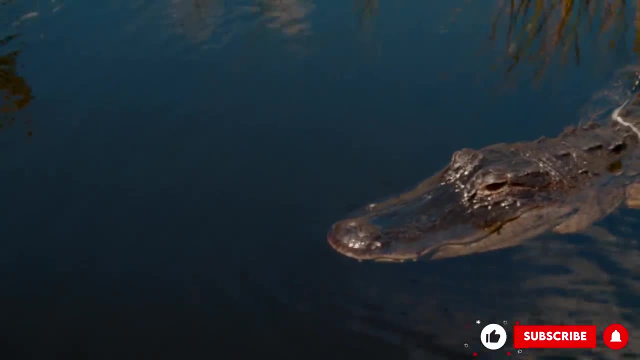 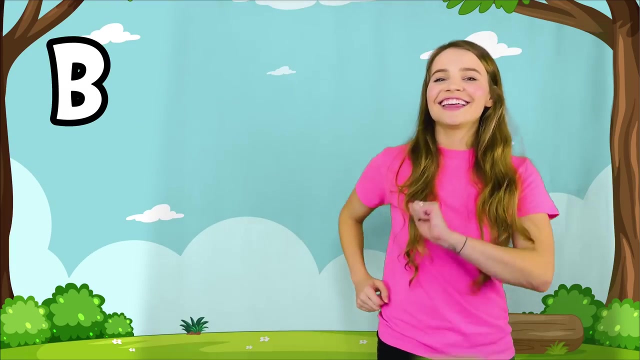 So nice to meet you. We're gonna go see some more animals. come on, What about alligators? go like this chomp. Yeah, How do you do with your arms? Chomp, chomp, chomp, Walking, walking through the zoo. 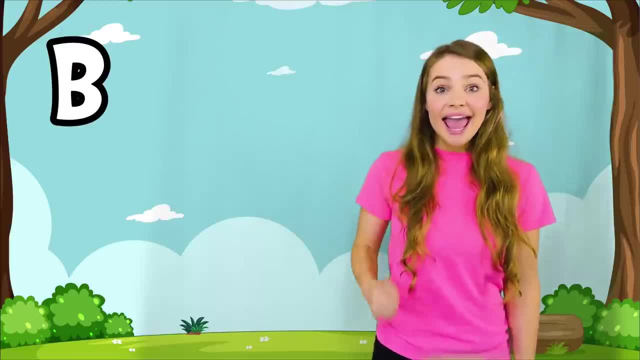 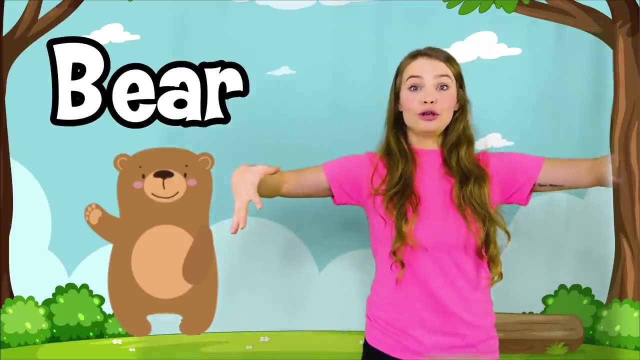 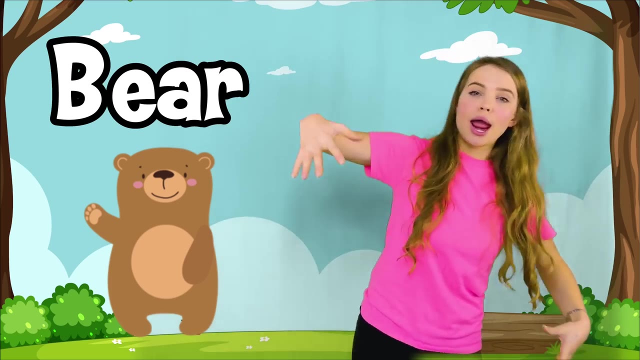 and look there's a letter B and a bear. Hi, bear Bears can be really big. Let's walk around like a bear together. Bear walking, walking, Bear b b, bear Bear. start with the letter B. 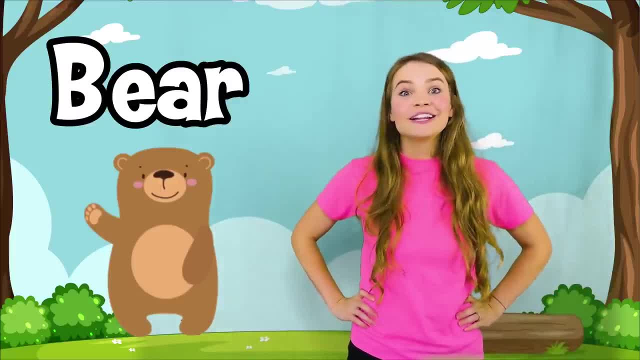 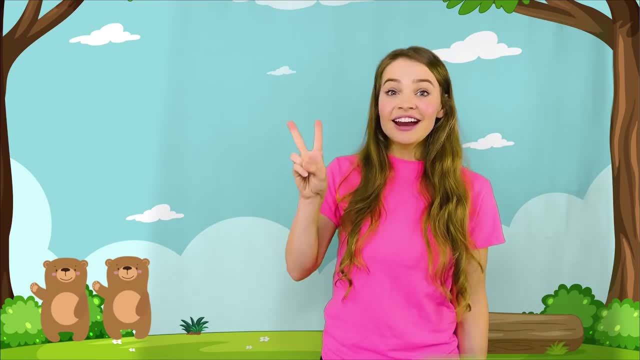 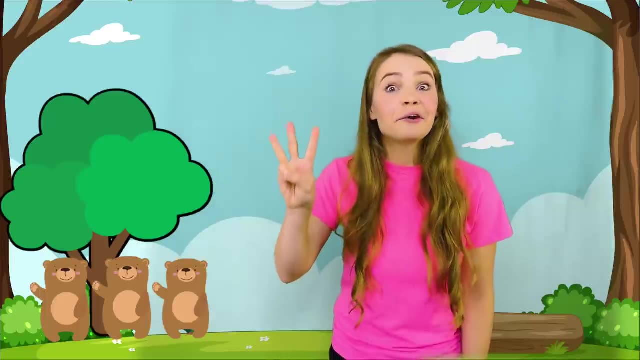 B b bear. Let's do a fun little nursery rhyme about bears together. One little bear wondering what to do, Then came another, and then there were two. Two little bears climbing up a tree, Then came another, and then there were three. 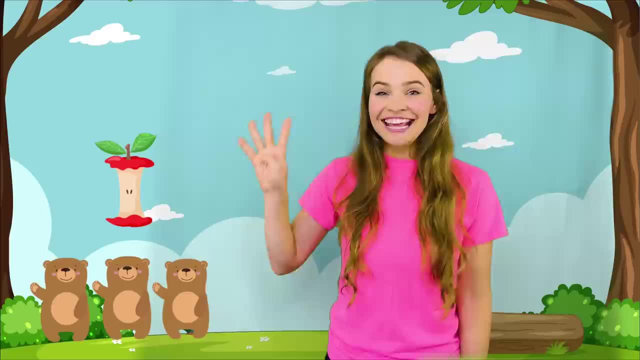 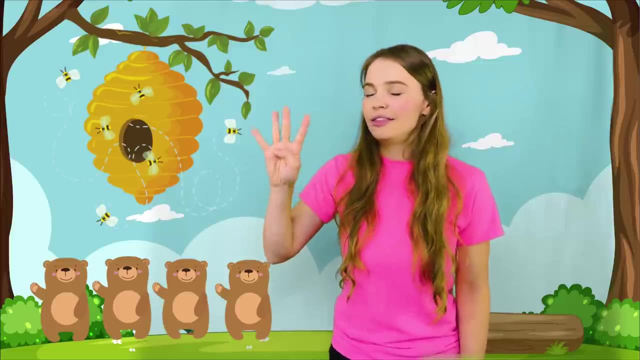 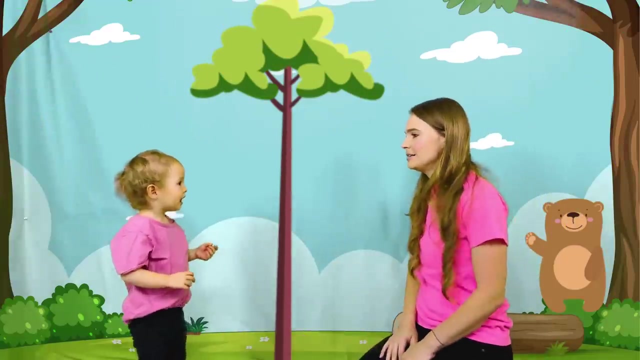 Three little bears eating an apple core. Then came another, and then there were four, Four little bears looking for honey in a hive. Then came another, and then there were five, Five little bears. How would the bear climb it? Ah, bop, bop, bop. 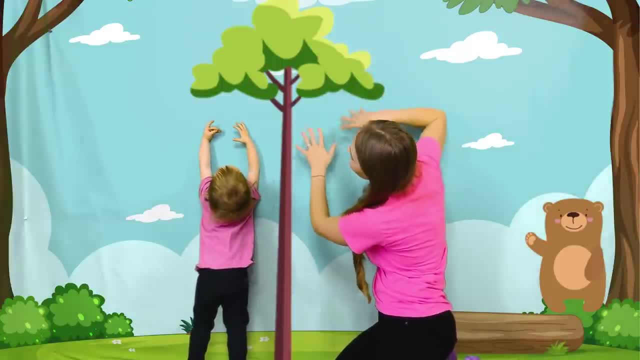 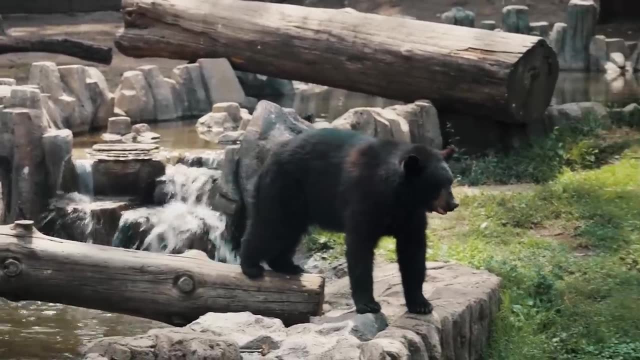 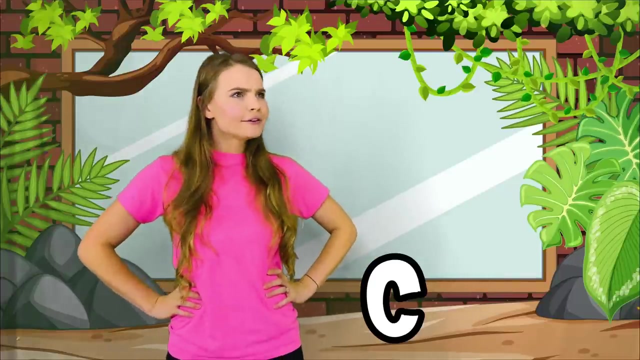 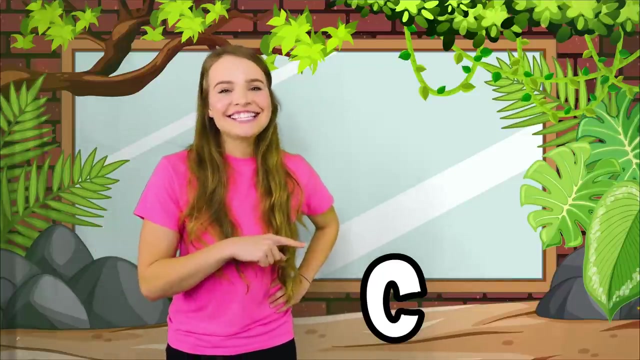 Climb, climb, climb, climb, climb the tree bear. Go climbing, Walking, walking at the zoo. I'm looking around looking for another letter. Do you see a letter anywhere Where? Oh right, This is the letter C. C makes the ck sound. 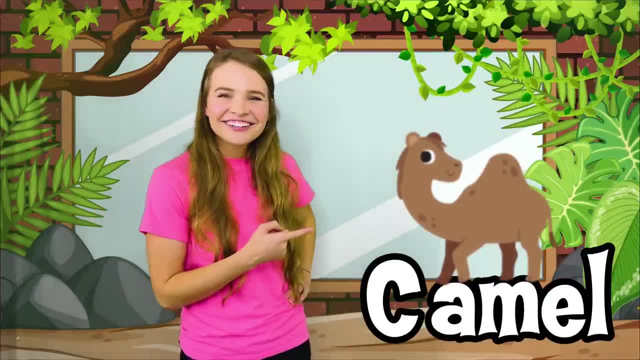 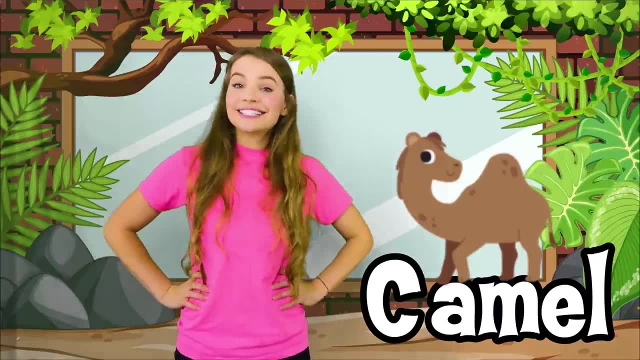 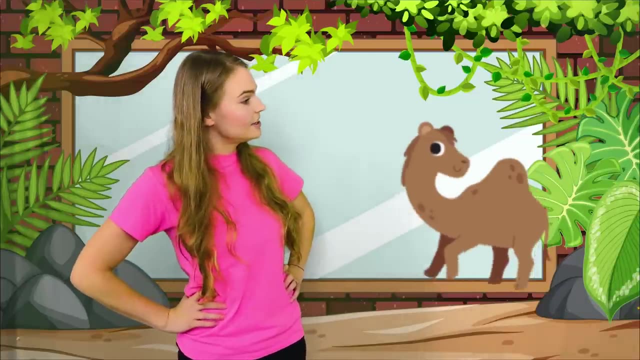 C for ck, ck, Camel. Hi camel, I like your hops. Camel, your name starts with the letter C. That's right, Camel. That's really interesting. I really like that Camel. do you know how to bend your knees? 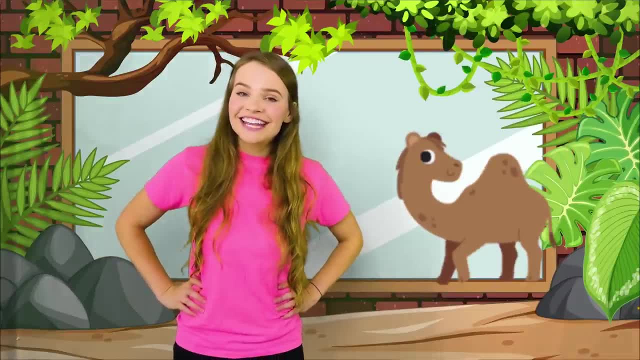 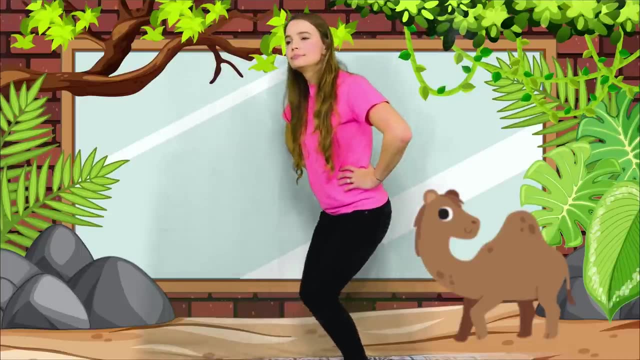 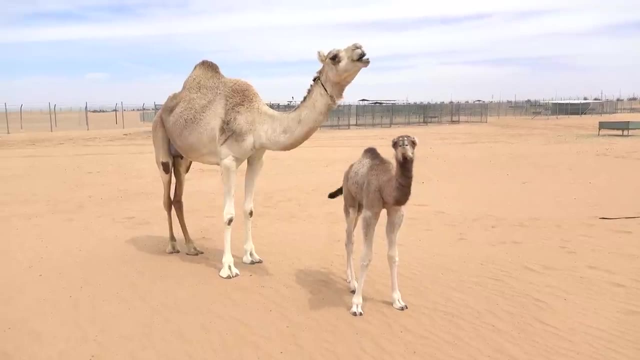 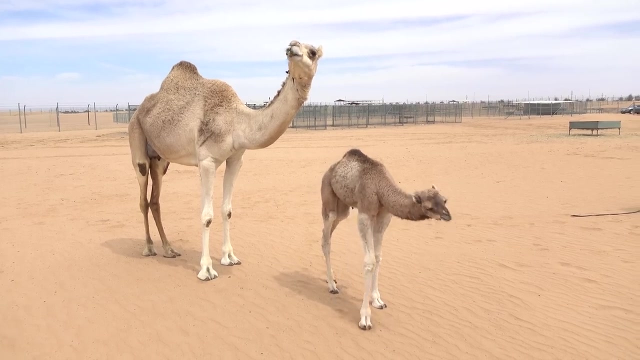 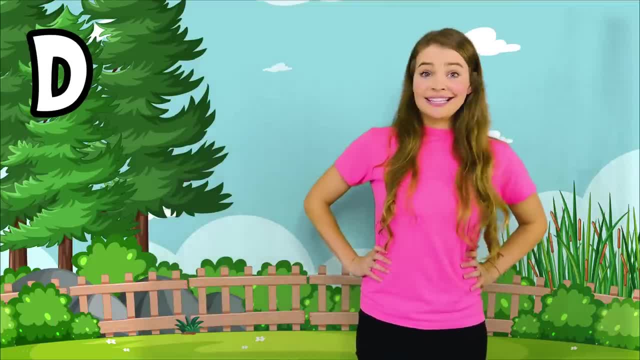 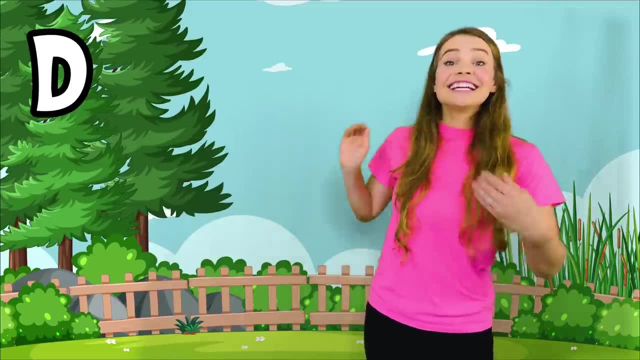 Good job. Now I'm looking for the letter D. Do you see a letter D anywhere? D d There it is. Thank you, D D for donkey. Hi, donkey. Donkey says hello. Should we make donkey sounds together? 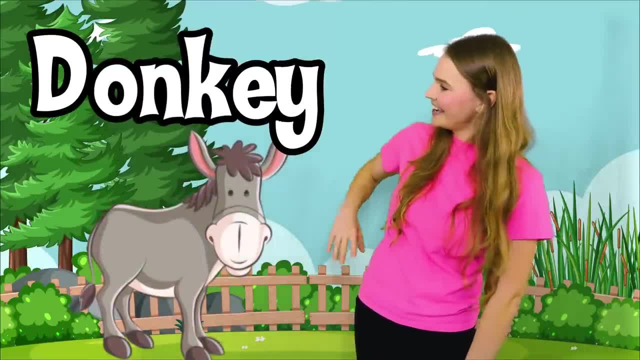 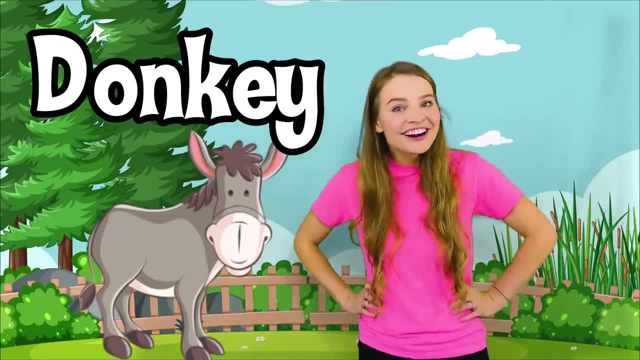 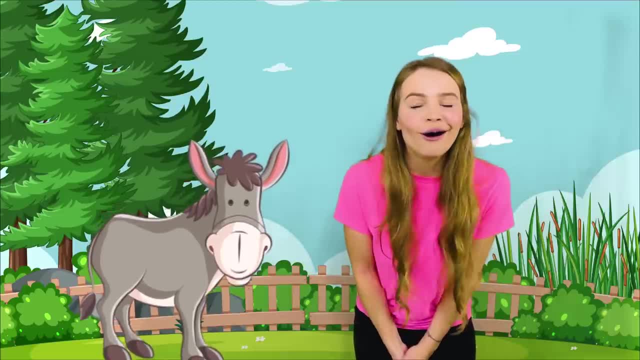 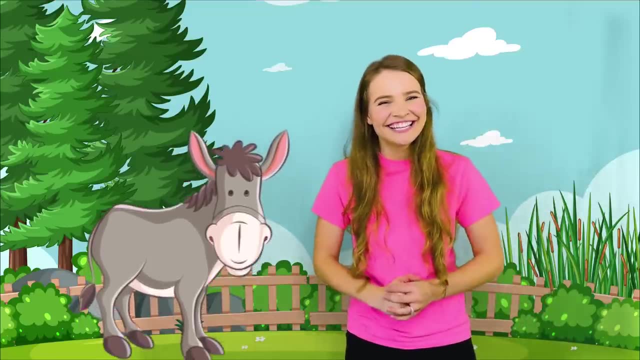 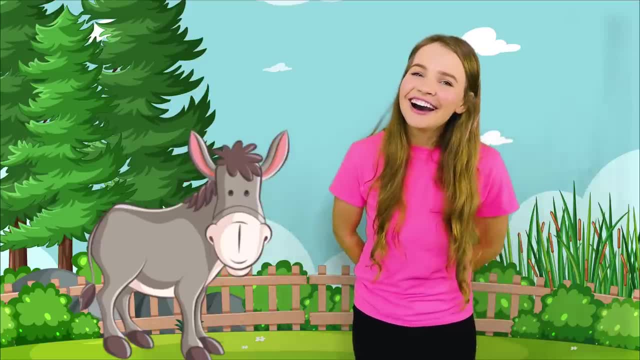 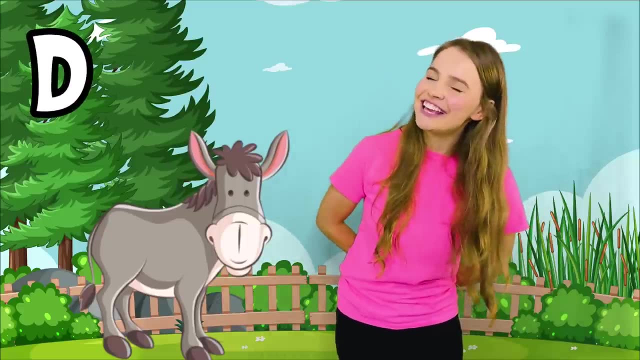 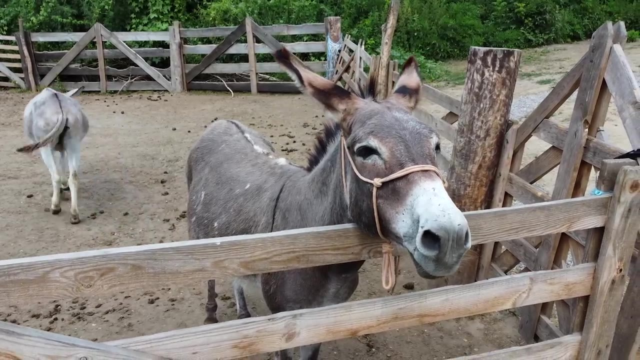 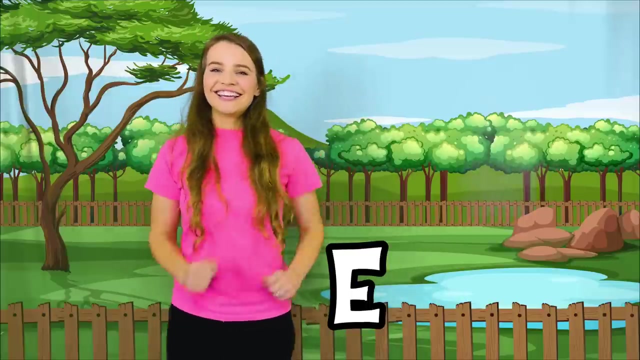 Donkey, donkey, I love you. Oh, that's really sweet, Donkey. we really like meeting you and we like it that your name starts with the letter D for d d, donkey, Walking, walking through the zoo, and now I'm looking for the letter E. Do you see a? 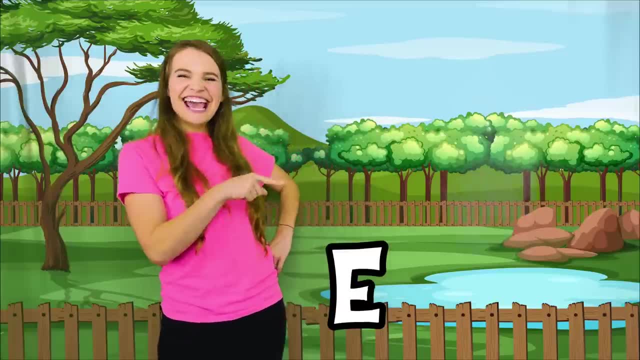 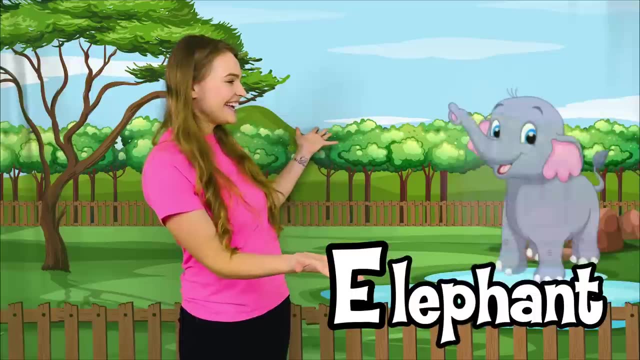 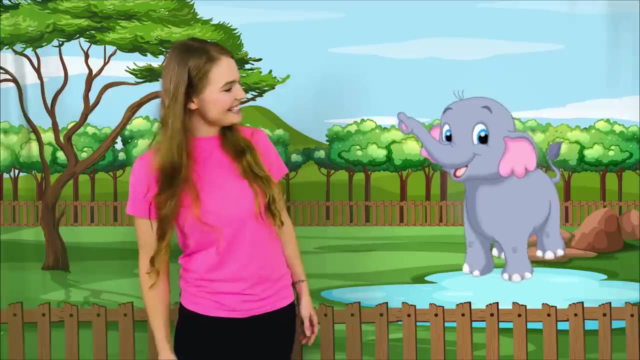 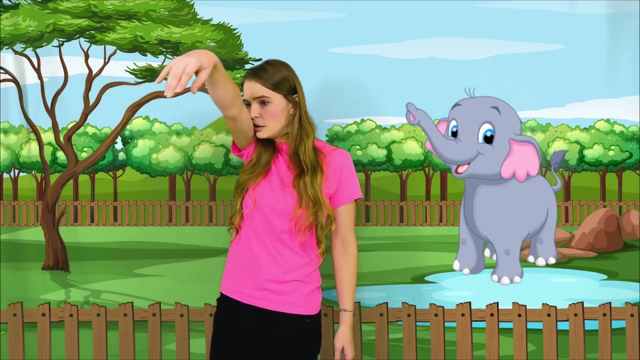 letter anywhere. Oh, yeah, right there, That's the letter E. that makes the eh, eh, eh sound for elephant. Hi, elephant, How are you? Elephant says: hello, nice to meet you. Should we stomp around like elephants? Okay, we'll get a trunk out, Pretend this arm is a trunk And we'll 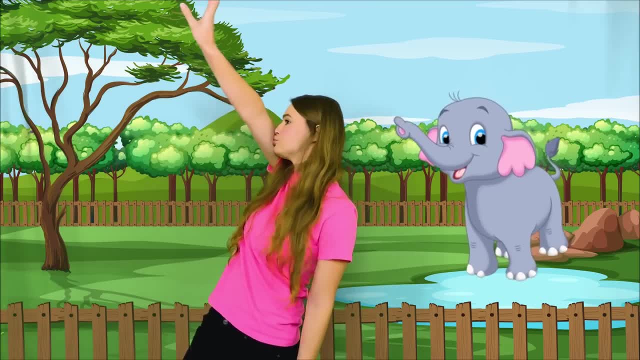 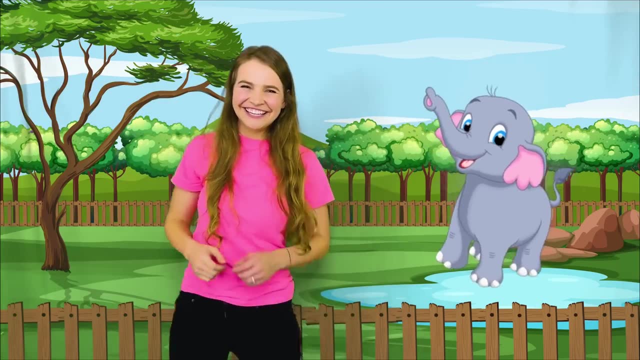 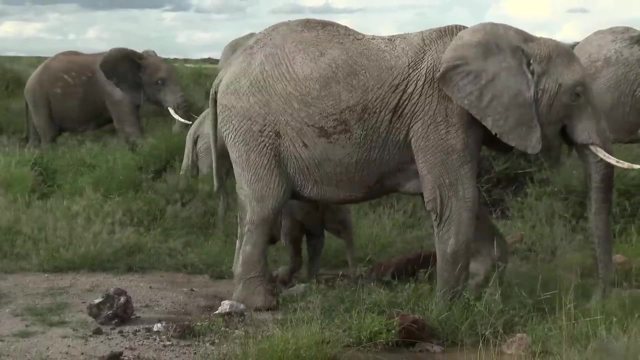 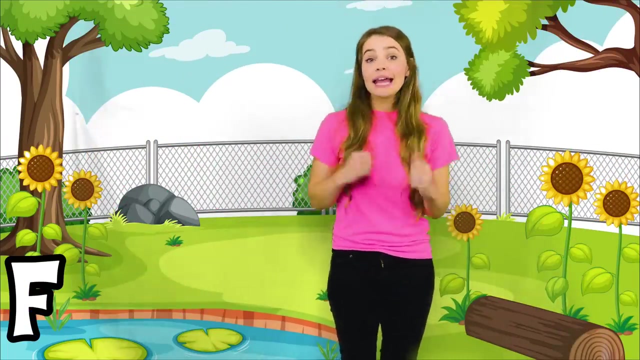 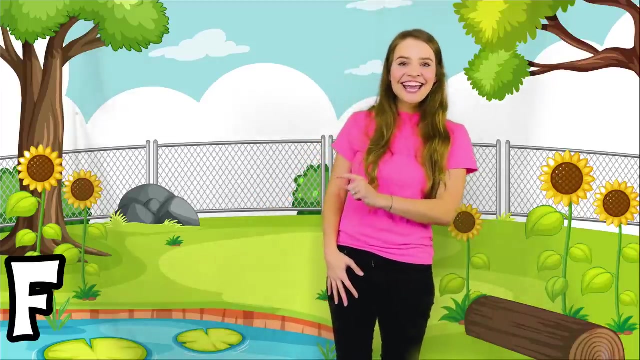 stomp, stomp, stomp, stomp, stomp, stomp, stomp. How silly. Now I'm walking, walking through the zoo And I'm looking for the letter F. Do you see the letter F Where? Oh yeah, right there. 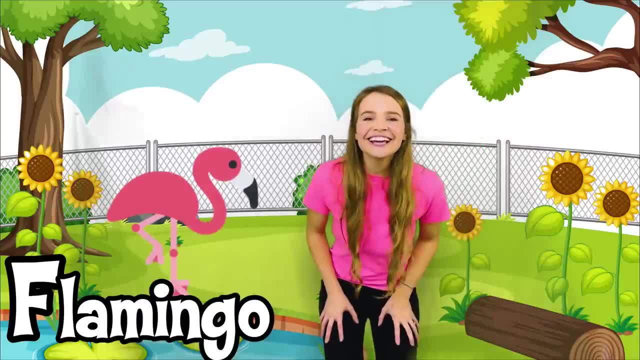 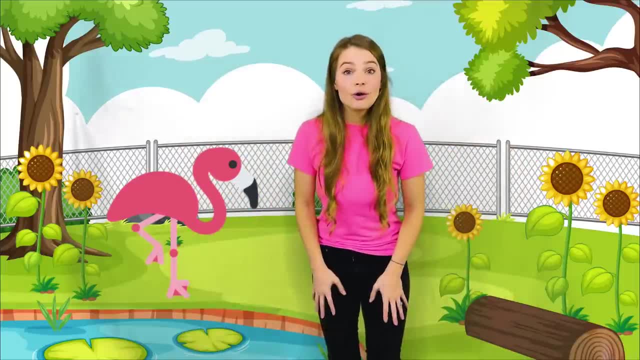 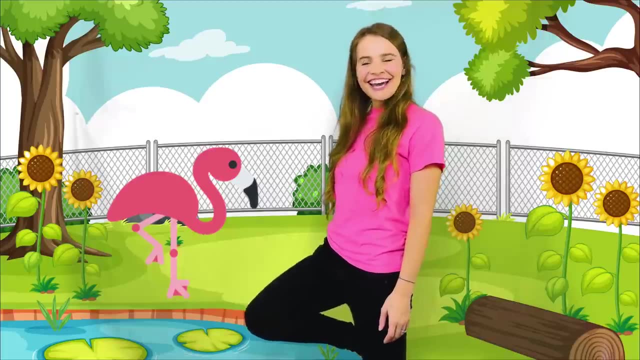 F for flamingos. Flamingos are really big birds And they got big pink wings. And did you know that they go to sleep standing on one leg like a flamingo? Isn't that silly? Hi, flamingo, it's really nice to meet you. 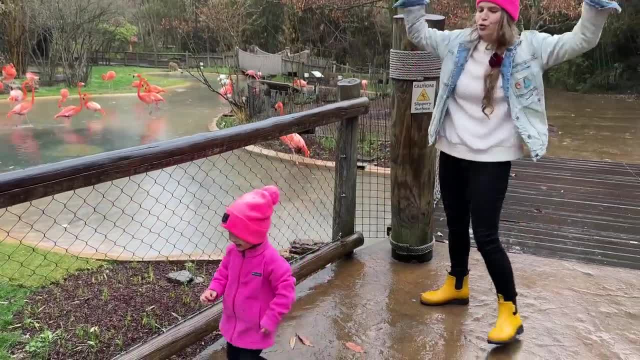 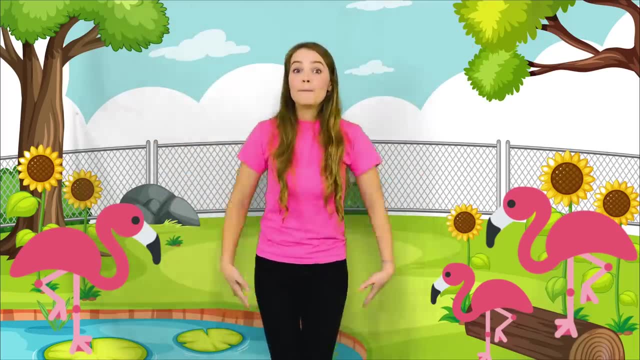 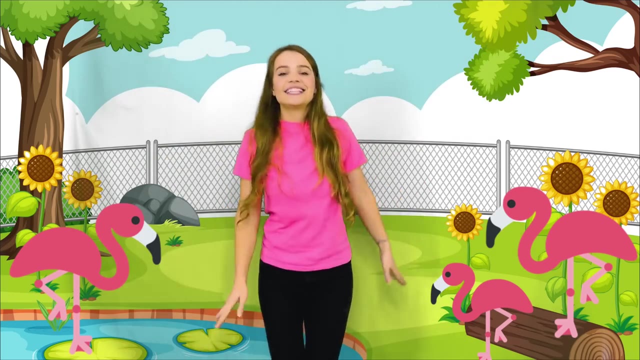 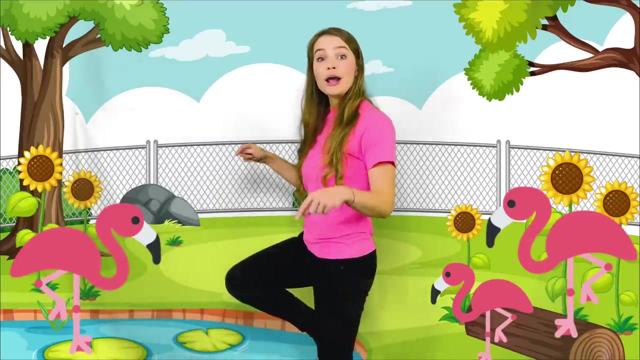 Flamingo's flapping, Flamingo's flapping Big pink wings, Big pink wings Flying through the sky, Flying through the sky. Time to land, Time to land Flamingo's standing. Flamingo's standing on one leg, On one leg, Sleeping while they're standing, Sleeping while they're. 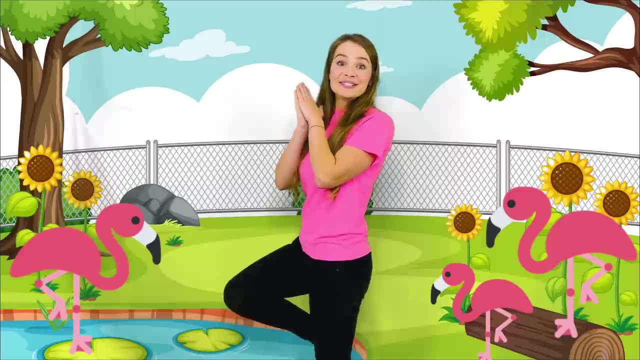 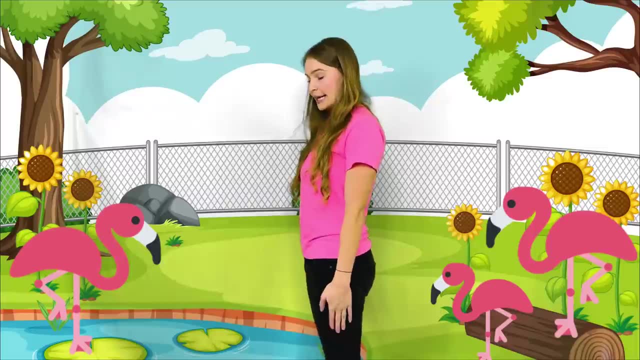 standing. Time to wake. Time to wake. Do you want to stand on one leg with me like a flamingo? All right, here we go. We're going to stand on two feet, Find our balance And then pick one leg up. 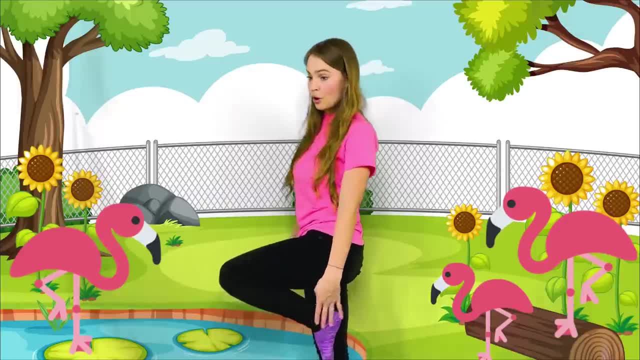 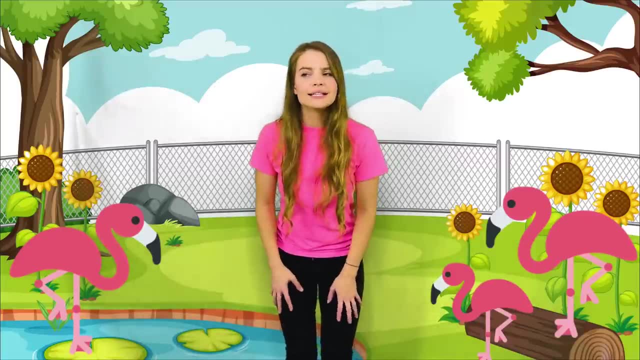 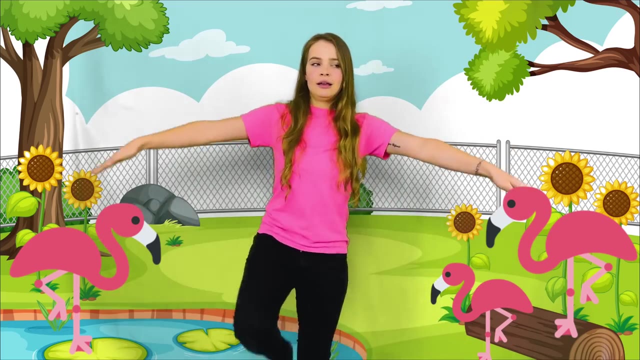 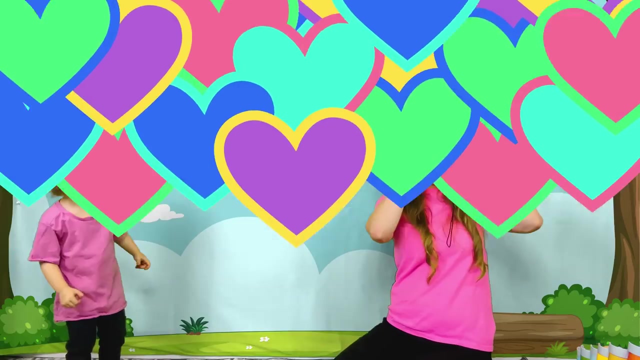 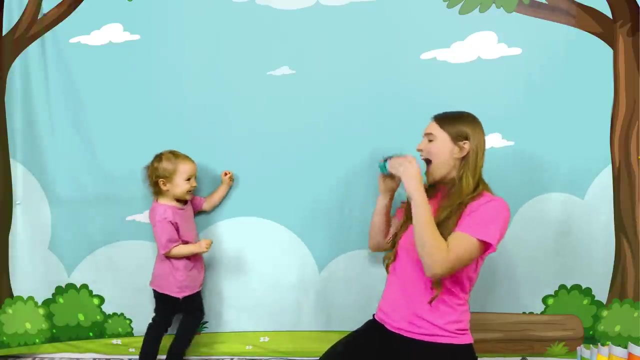 Wow, we're flamingos together. Whoa, whoa. sometimes it's hard to balance Whoa. Flamingos must have really good balance because they can balance on one leg. huh, Whoa whoa, Can you do it? It's kind of tricky. Whoa Whoa, Wow, Thank you. Oh, is that a flamingo? Hi, flamingo. 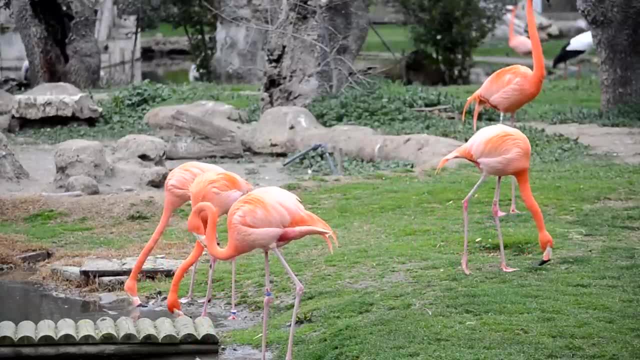 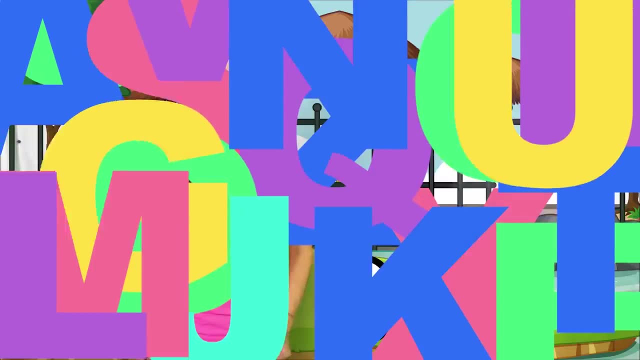 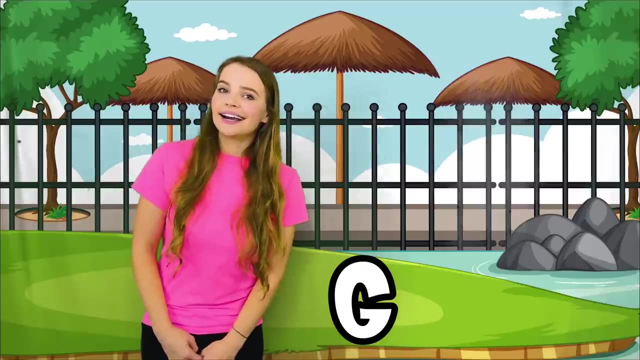 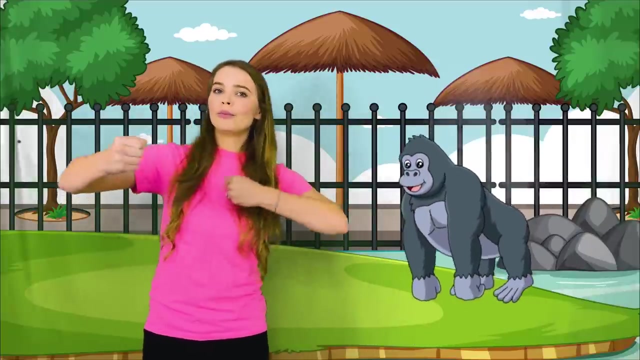 I'm walking, walking through the zoo and now I'm looking for the letter G. G makes the g-g-g sound like g-g-gorilla. Gorillas can thump their chest like this: Thump thump, thump, thump. We don't want to hit our chest too hard, but we can pretend we're thumping. 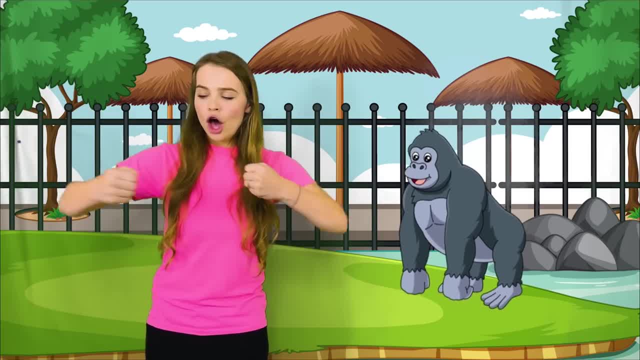 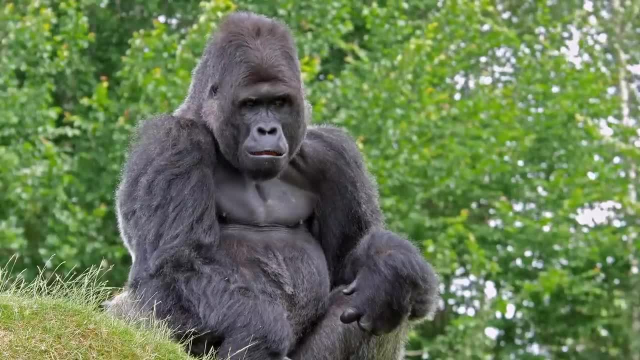 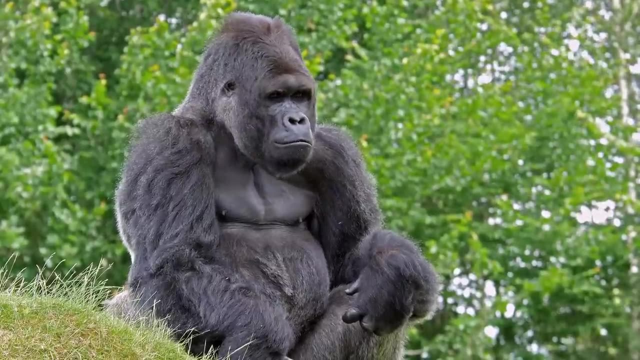 it Really hard. like a gorilla. You want to do it with me? Thump thump, thump, thump thump. That's very silly. Letter G can also make a softer sound like g-g-giraffe Look. 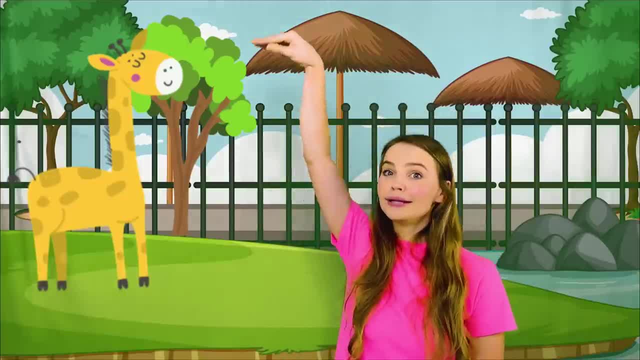 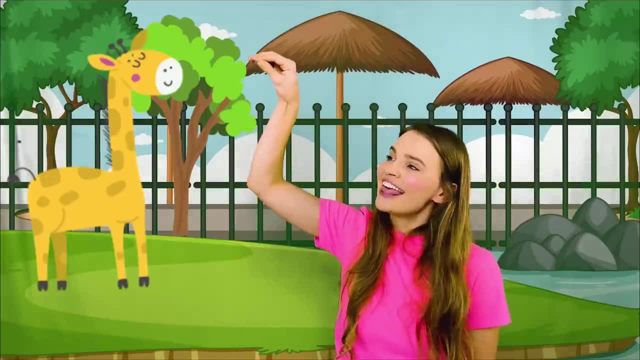 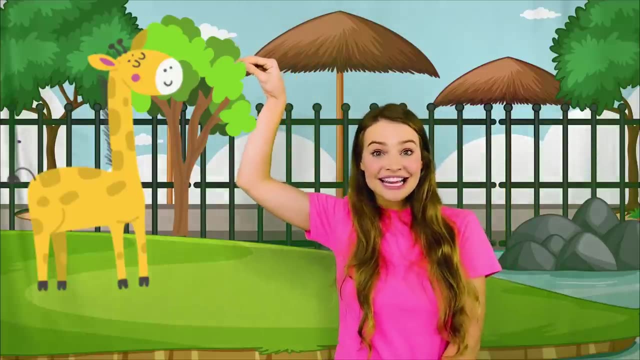 at this giraffe. Giraffes have really long necks and they go. ooh, I can't reach the top of this tree and eat some leaves. They also have spots on them. huh, A little spotted giraffe. Hey, giraffe, are you eating some leaves? Do you want to pretend to be? 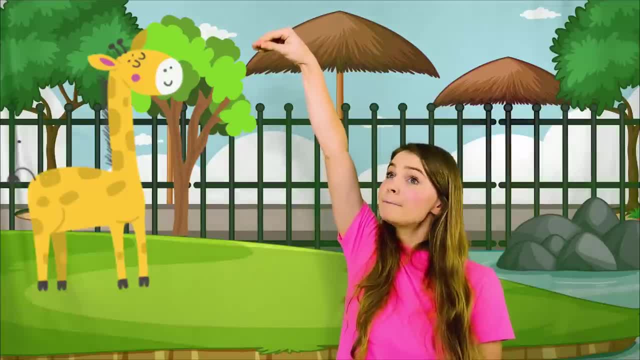 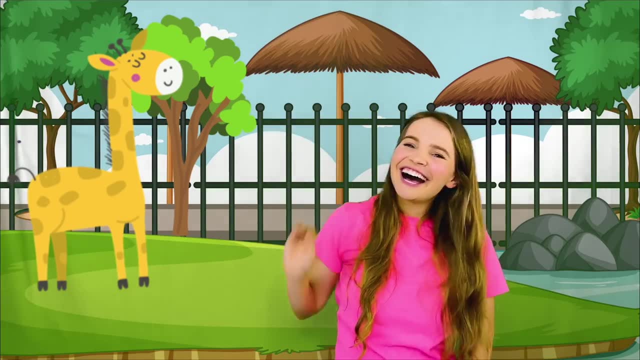 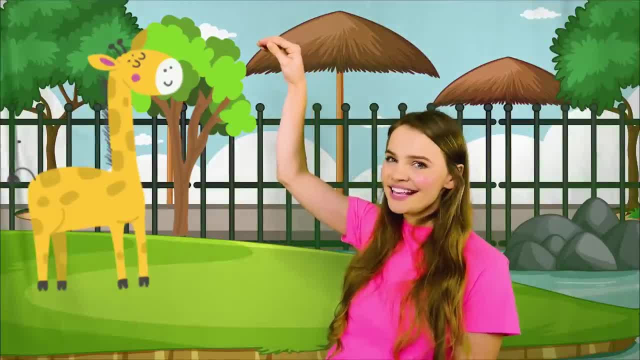 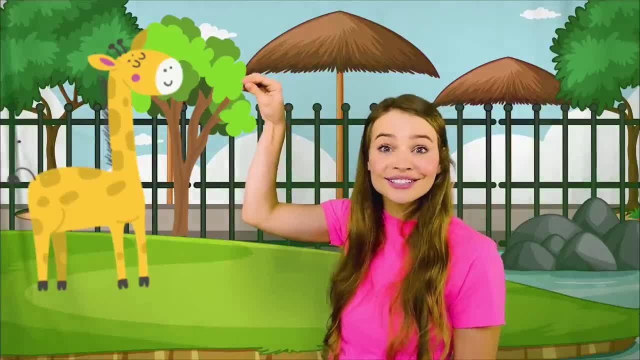 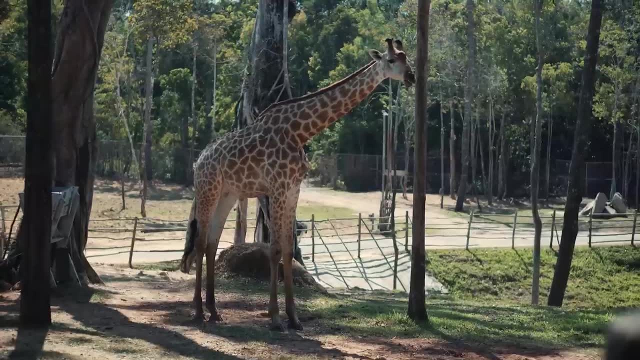 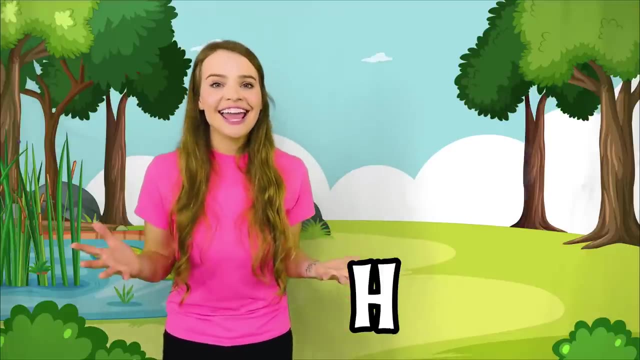 יו, you do good, Hippo parti and du ui gated, but it's a bunch of leaves on a tree. His neck's really long and his legs are long too, and he can be faster than his friends. 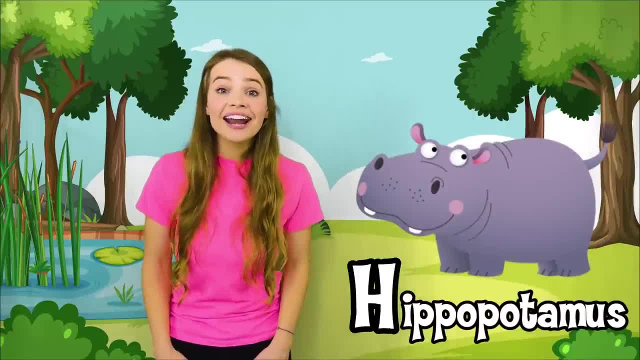 at the zoo. Now I'm walking, walking through the zoo and I'm looking for the letter H for a hippopotamus. That's a big word: Hippo-potamus, Hippo-potamus, Hippo-potamus. 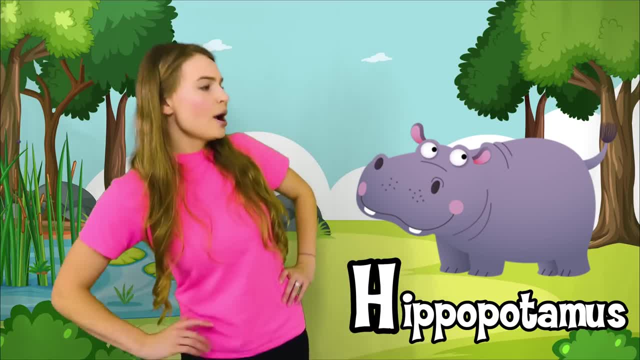 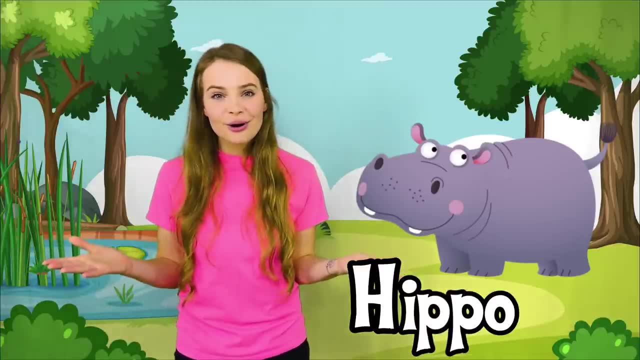 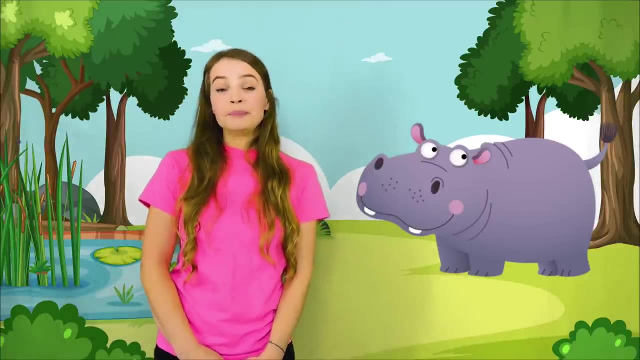 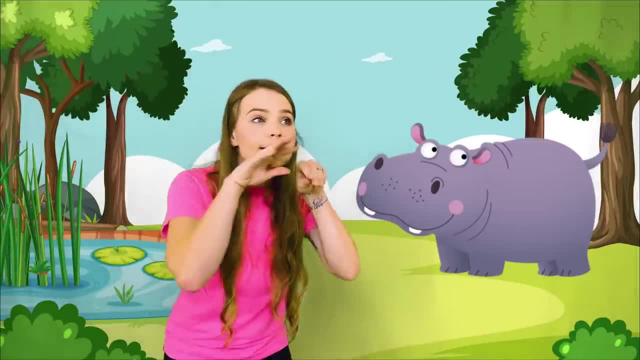 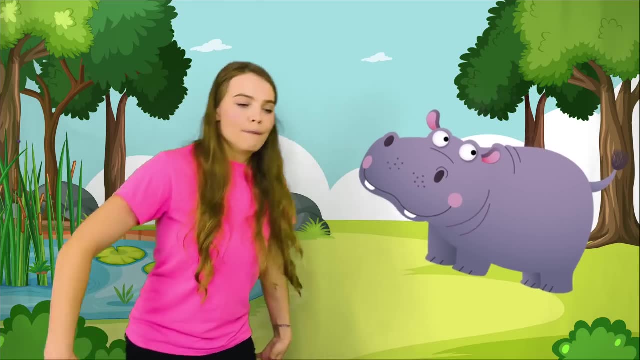 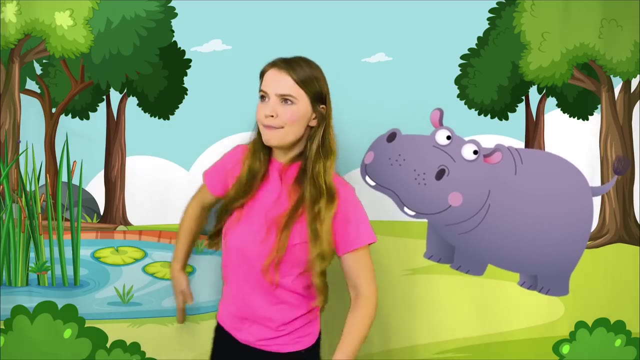 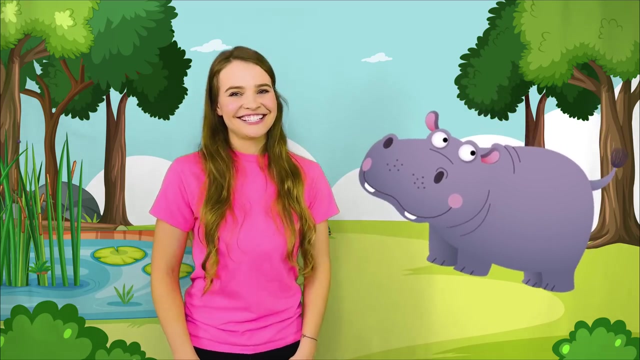 and still look up and see stuff and eat and drink. they're pretty big. you want to walk around like a hippo with me. hippopotamus, hippopotamus, hippopotamus. hey, hippo, hippopotamus, hippo, hippo. that's very silly. what about hippopotamus hippopotamus? 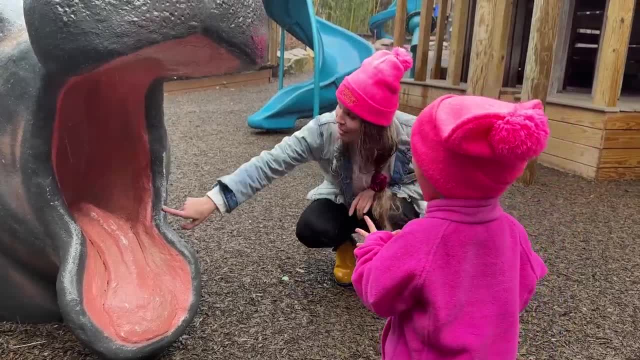 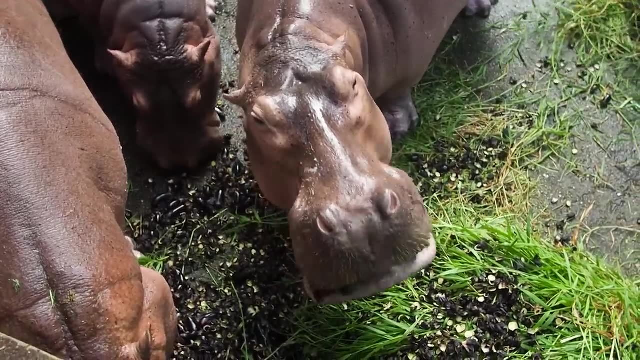 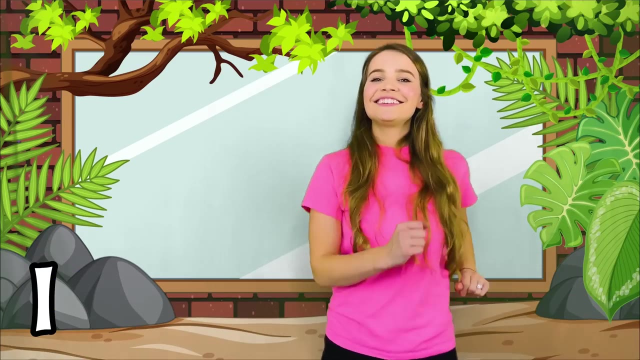 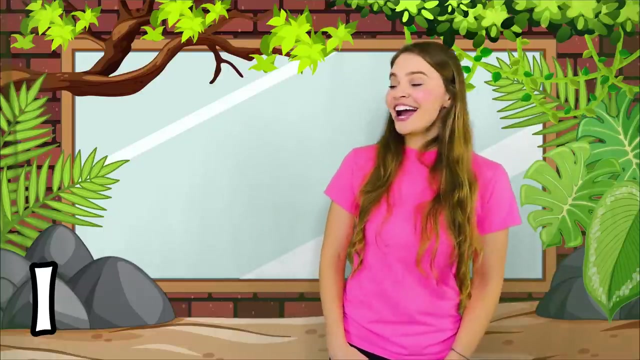 that's his mouth. he's going like this: ah, maybe he's gonna brush his teeth. hippopotamus- hippopotamus- hippopotamus hippopotamus. walking, walking through the zoo and I'm looking for the letter I. that makes that it it. it sounds for iguana. iguanas are big lizards and they love sitting on. 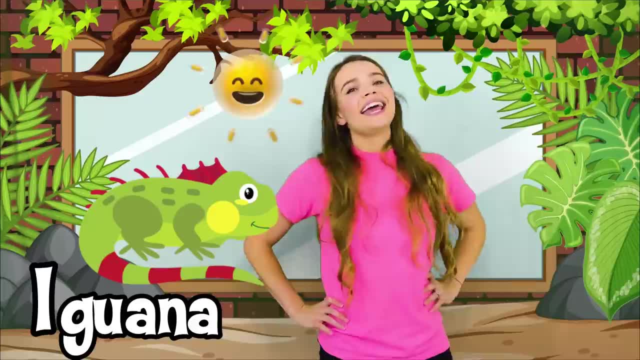 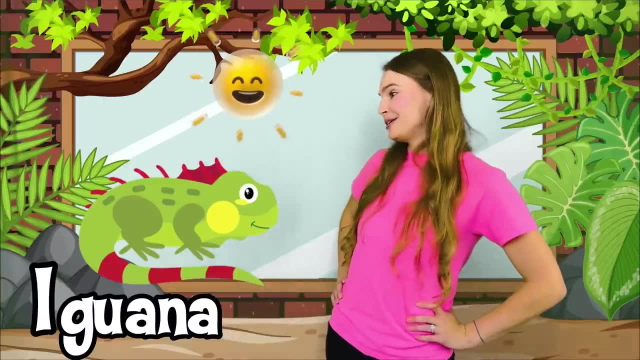 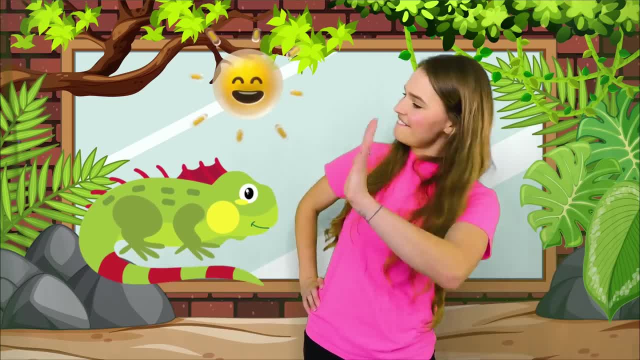 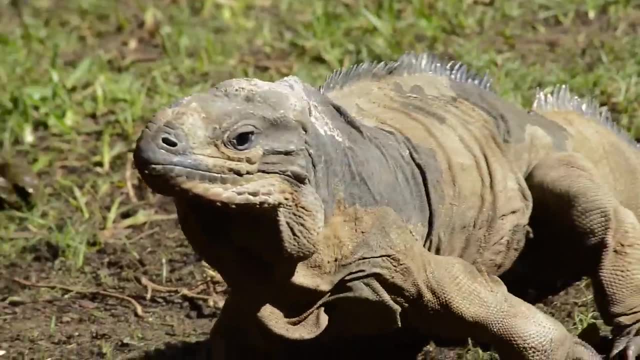 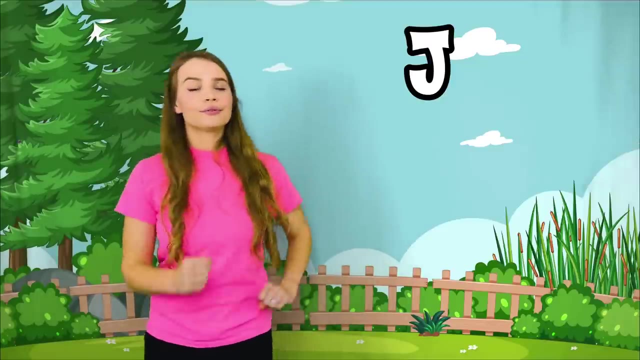 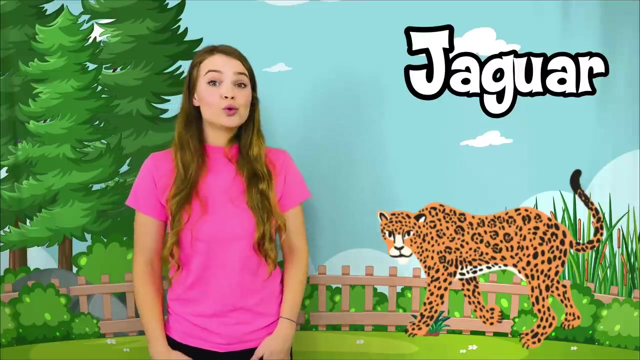 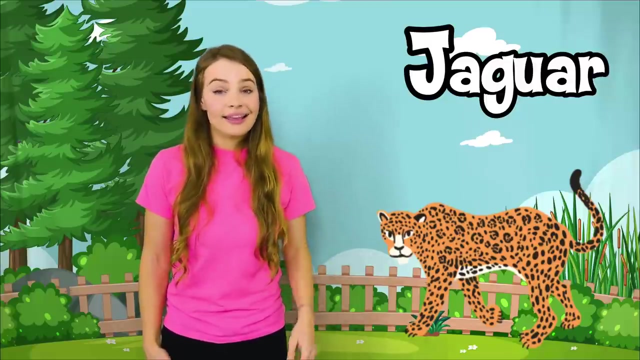 nice and warm. oh, we're happy to hear that. have fun. we're off to explore and find more animals. now I'm walking through the zoo and I'm looking for the letter J, J for giant jaguar. jaguars are really big cats, kind of like a tiger, a lion or a cheetah, and they can 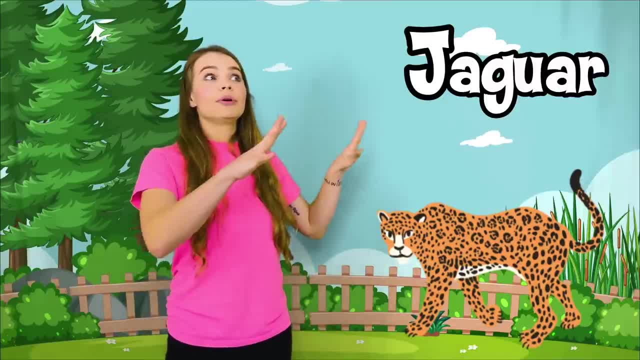 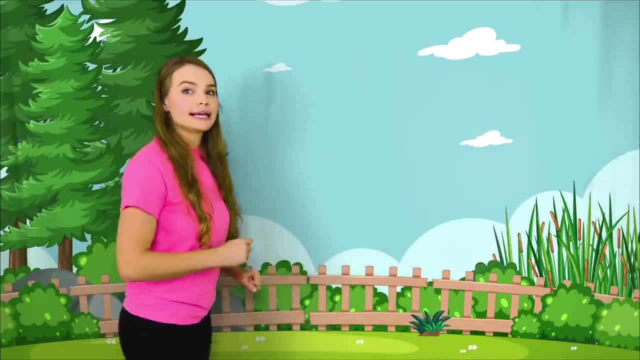 run really fast and they can leap. they can leave really far. should we do some jumps and leaves together, all right? all right, we'll start on this side and I'm gonna leap over there. you want to do with me? come on, let's stand up. we'll. 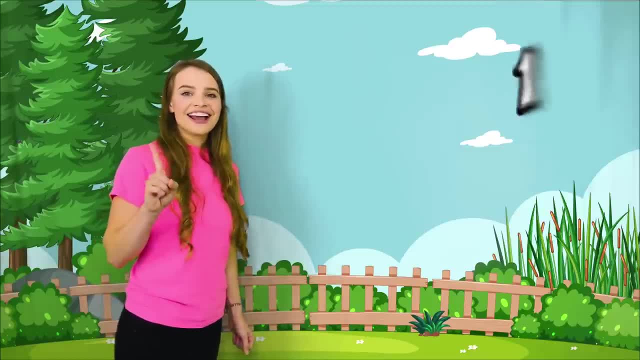 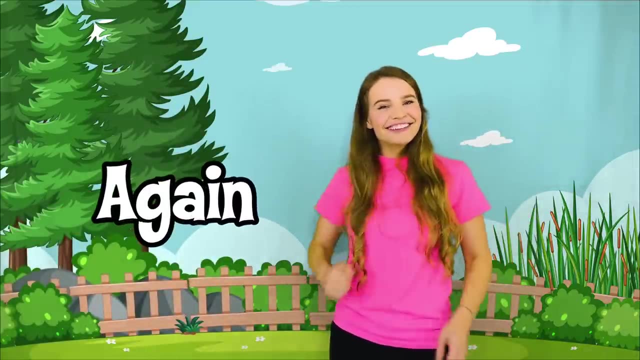 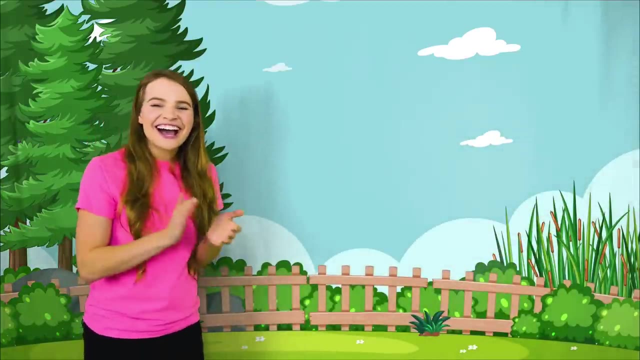 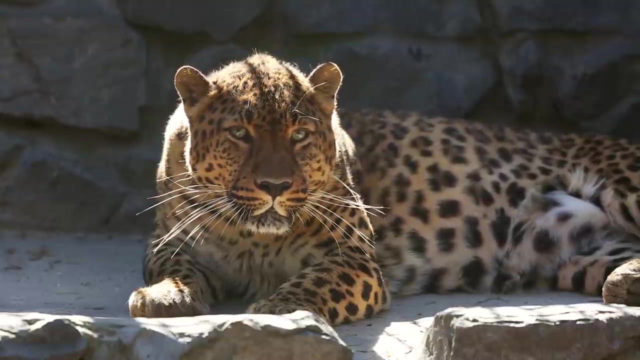 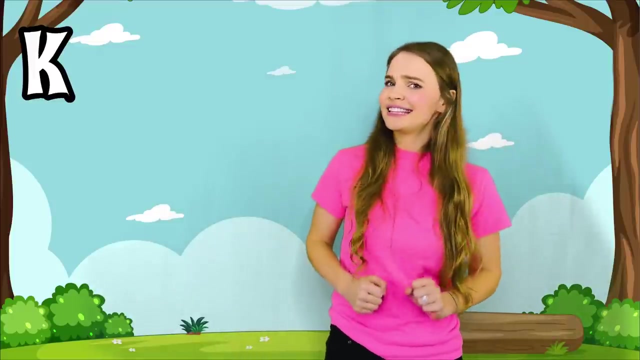 count to three and then we'll leap like a big jump. okay, one, two, three, all right, three and leap. Wow, Should we do it again? All right, Ready. One, two, three and leap, All right. I'm walking through the zoo and I'm looking for the letter K K. that means the k k k sound for kangaroo. 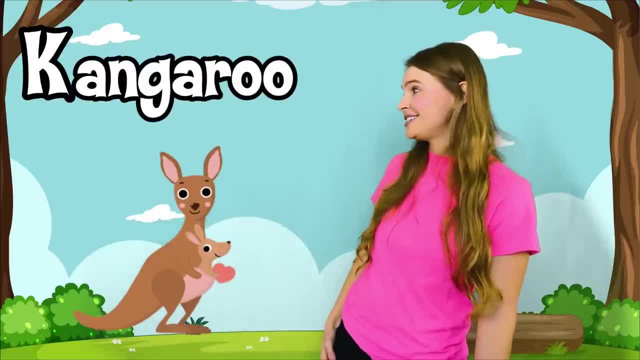 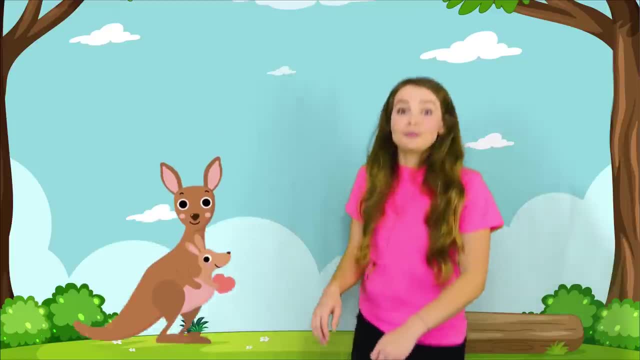 Hi, kangaroo, It's very nice to meet you. Did you know that kangaroos are really good at jumping? They have strong legs and they go boing, Boing, boing, boing, boing, boing. 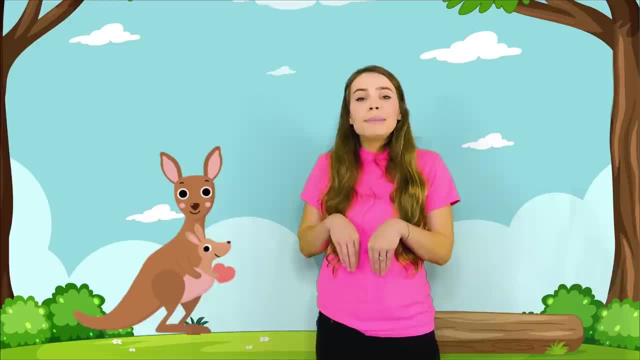 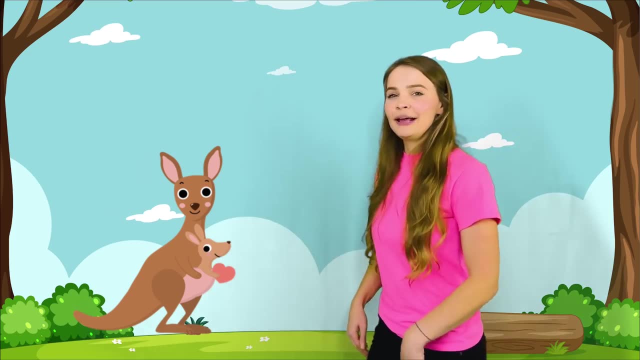 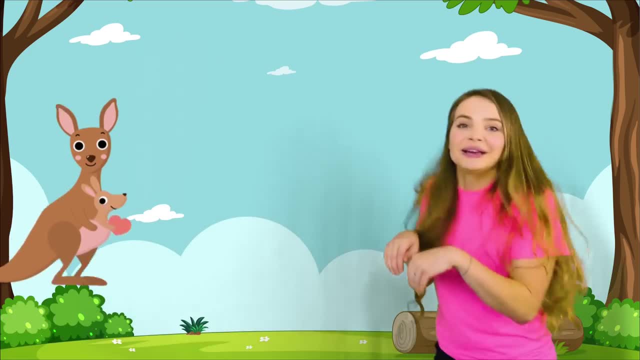 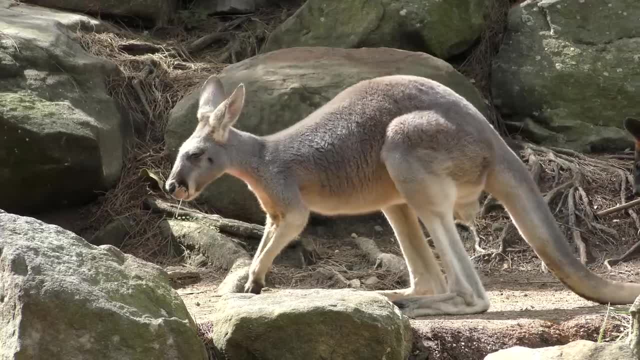 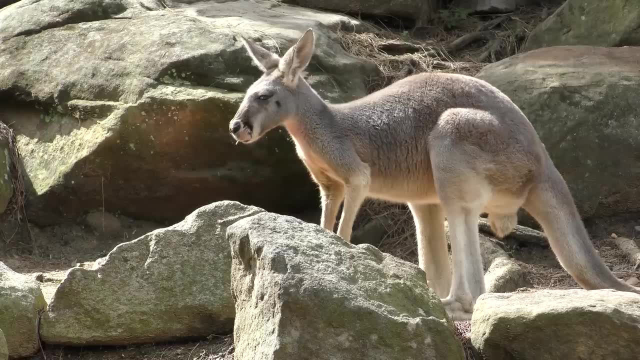 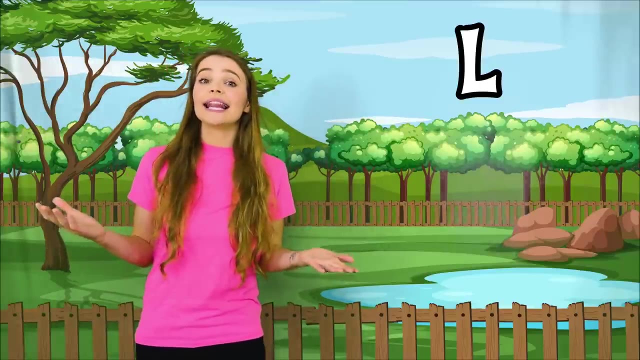 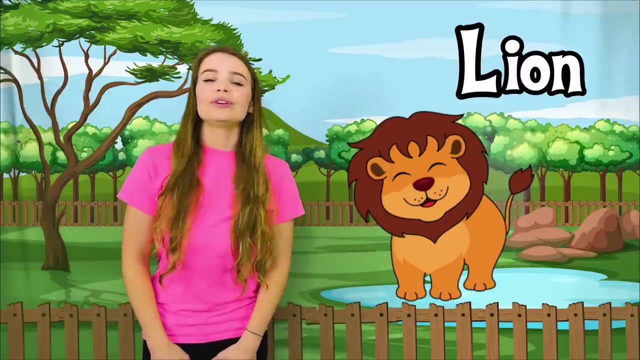 How silly. Thank you for jumping. Now I'm walking, walking through the zoo and I'm looking for the letter L for lion Lions are really big and they like to roar really loud. Do you want to roar with me? Oh, go, roar. That was pretty loud. 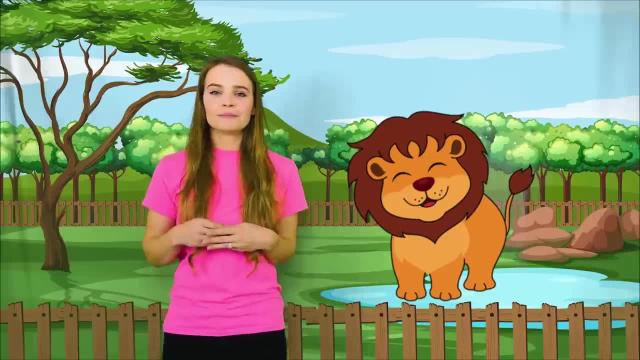 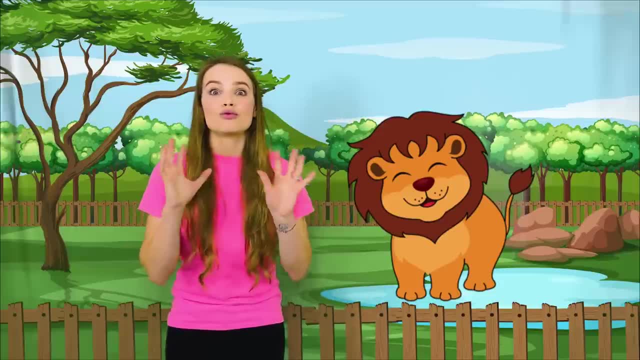 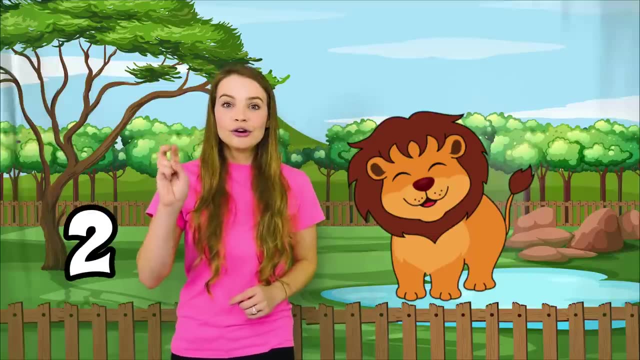 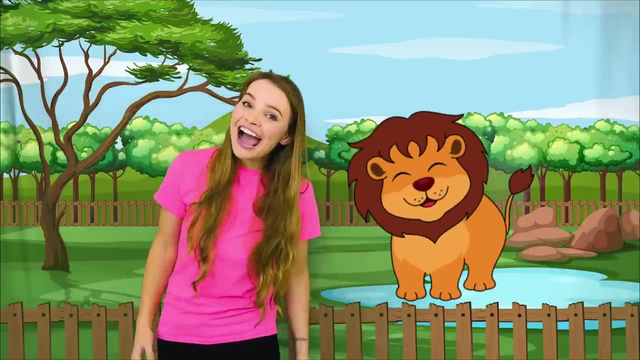 Ooh, that was pretty loud too. Okay, let's do a really big roar. Are you ready? You gonna do it with me? Okay, ready, One, two, three Roar. Wow, that was really big and really loud. 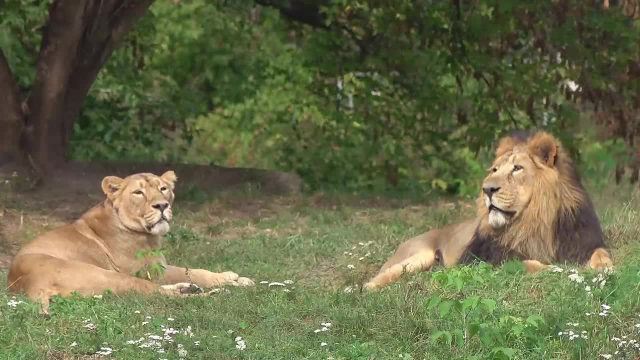 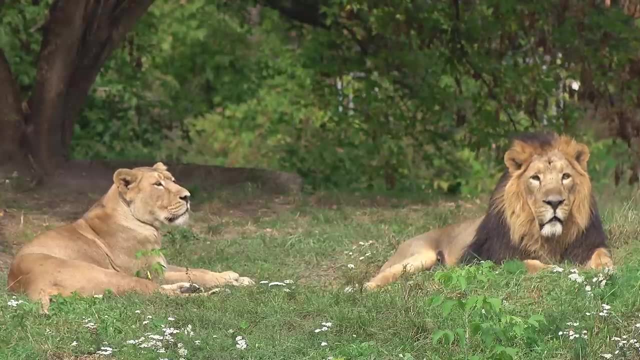 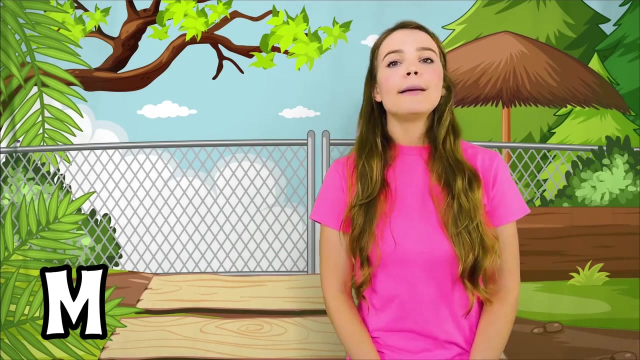 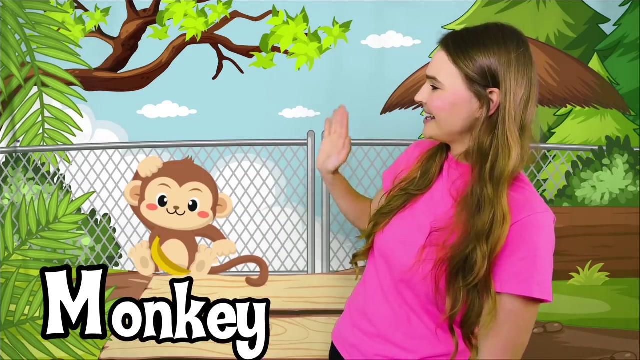 You make a great lion. Now I'm walking, walking through the zoo and I'm looking for the letter. M? M makes the mm, mm, mm sound for monkeys. Hi, monkeys, Monkeys like to jump around. go, ooh, ooh, ah, ah. 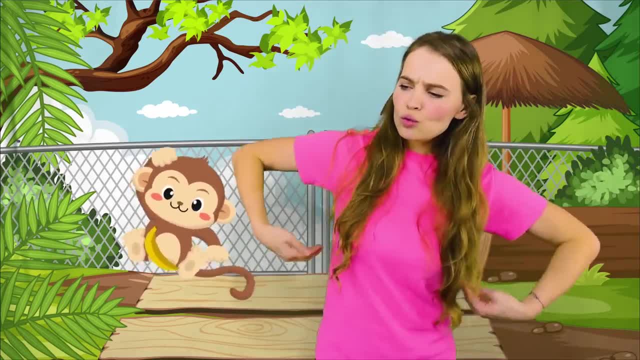 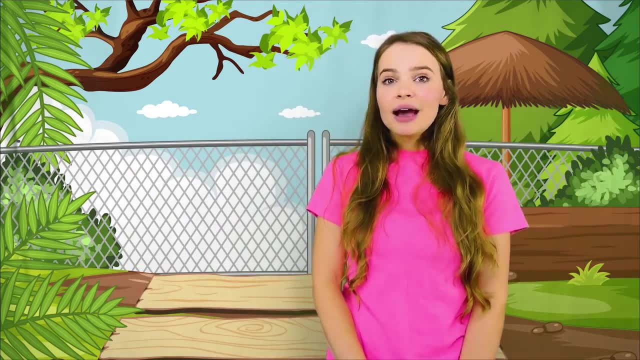 Ooh, ooh, ah ah. Let's act like monkeys together. Ooh, ooh, ah, ah, ooh, ooh, ah, ah, ooh, ooh, ah, ah. How silly. Let's do the little rhyme. 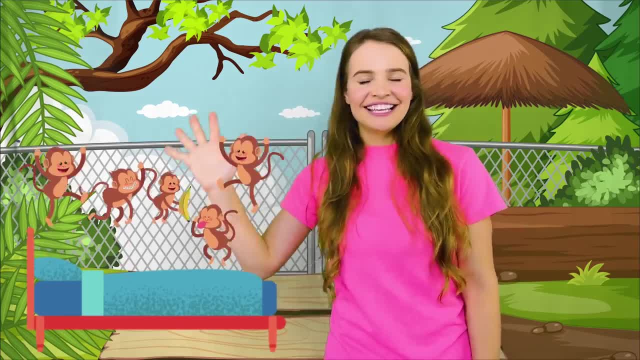 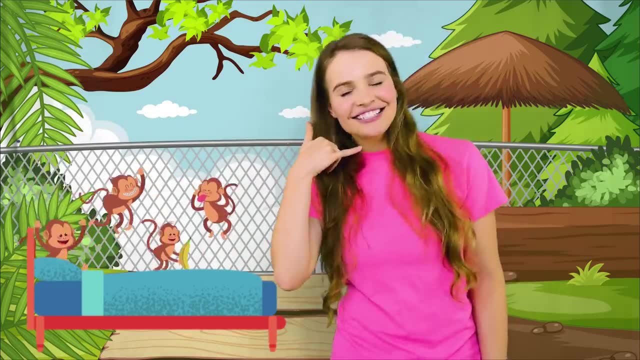 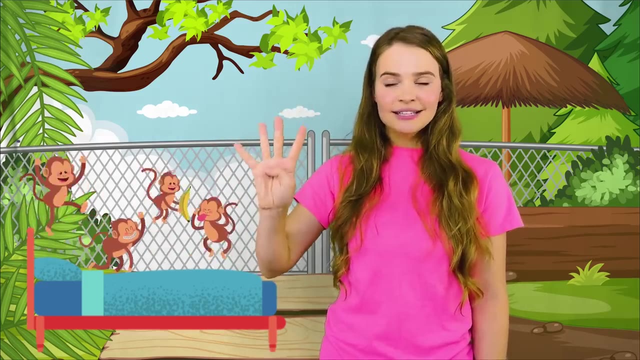 About five little monkeys. Five little monkeys jumping on the bed. One fell off and bumped his head. Mama called the doctor and the doctor said: no more monkeys jumping on the bed. Now we've got four little monkeys, Four little monkeys jumping on the bed. 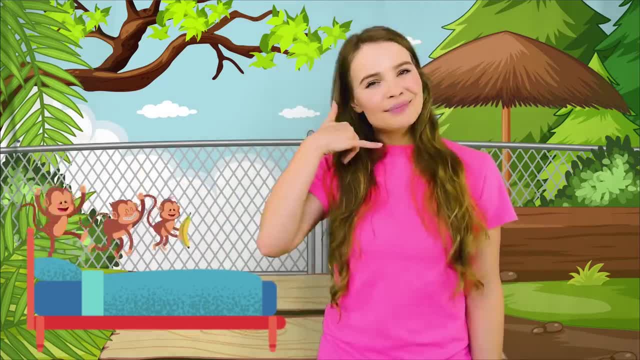 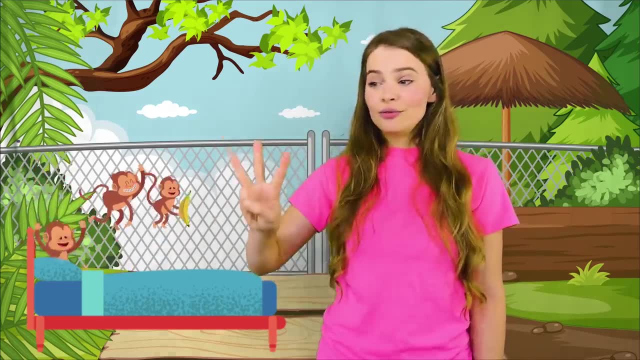 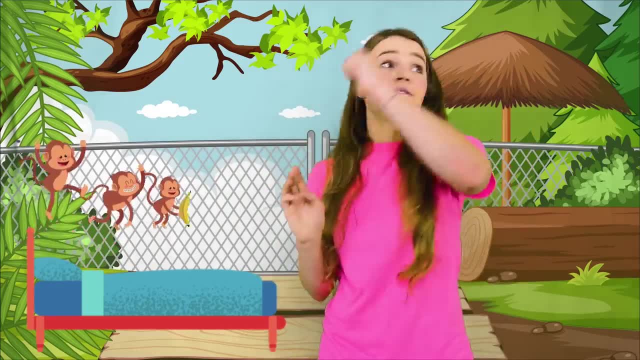 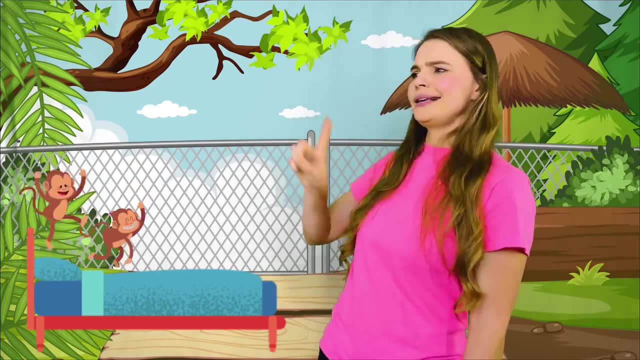 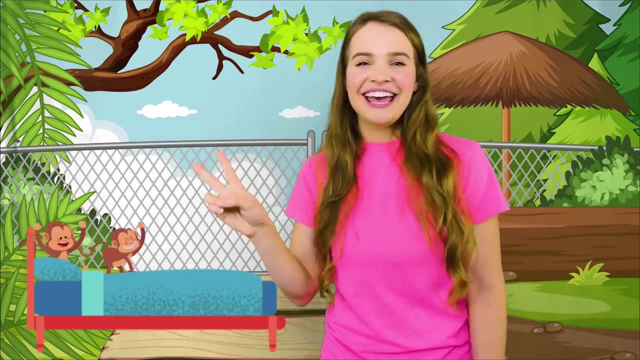 Three little monkeys jumping on the bed. One fell off and bumped his head. Mama called the doctor and the doctor said: no more monkeys jumping on the bed. Now there's two monkeys left. Two little monkeys jumping on the bed. One fell off and bumped his head. 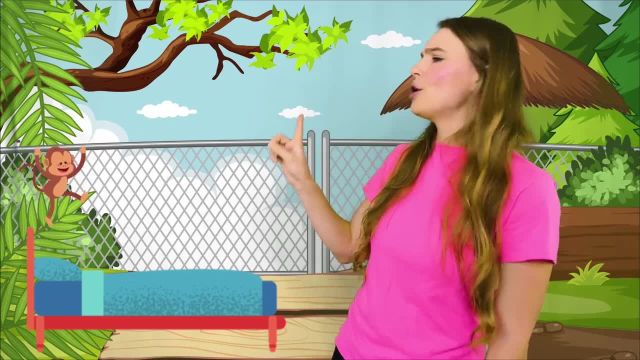 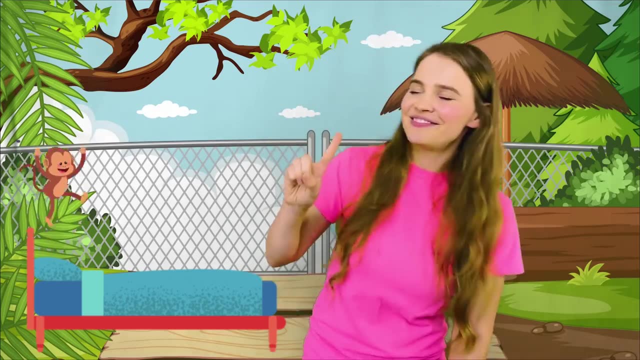 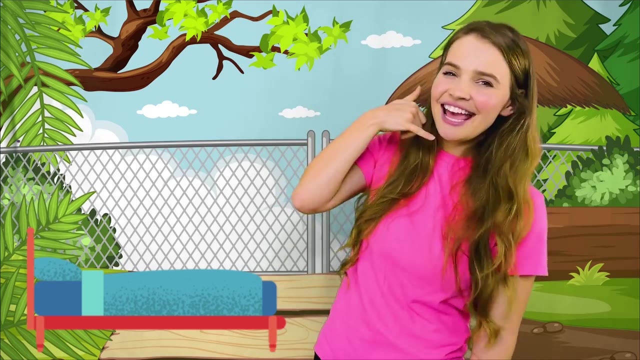 Mama called the doctor and the doctor said: no more monkeys jumping on the bed. We've got one monkey left, One little monkey jumping on the bed. He fell off and bumped his head. Mama called the doctor and the doctor said: no more monkeys jumping on the bed. 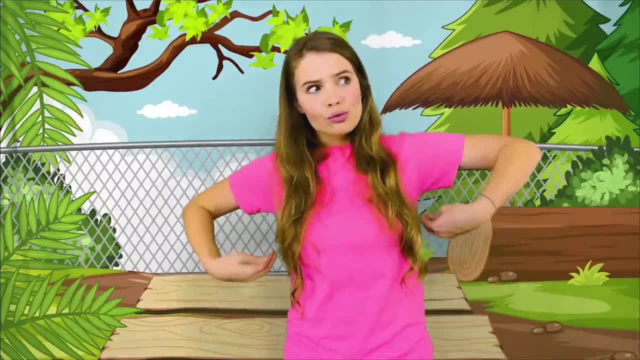 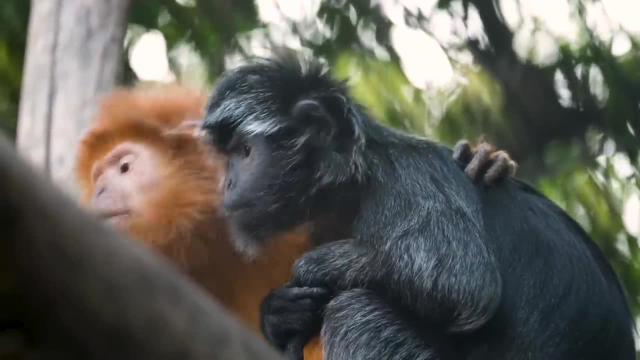 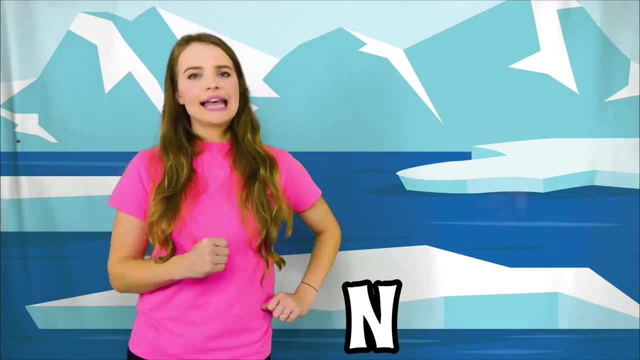 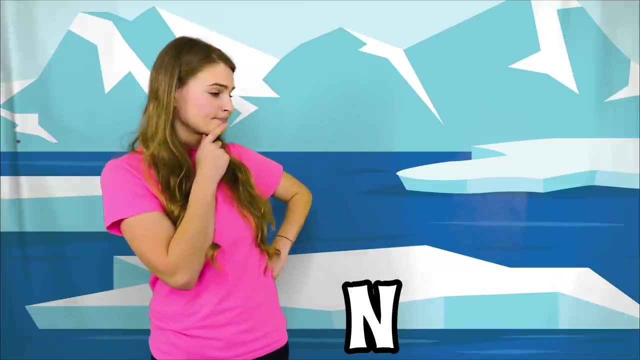 Wow, silly monkeys. Now I'm walking through the zoo and I'm looking for the letter N. It makes a N N N sound. Do you see the letter N? Hmm, Oh yeah, right there, N for a narwhal. 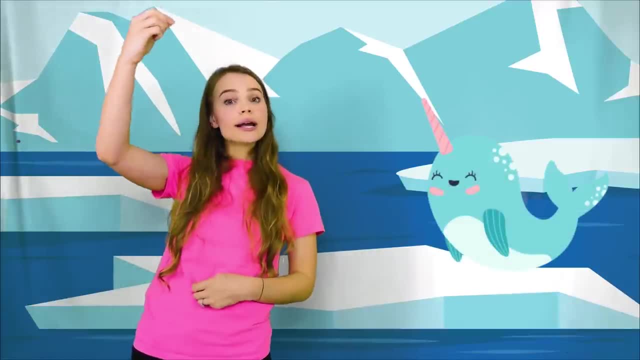 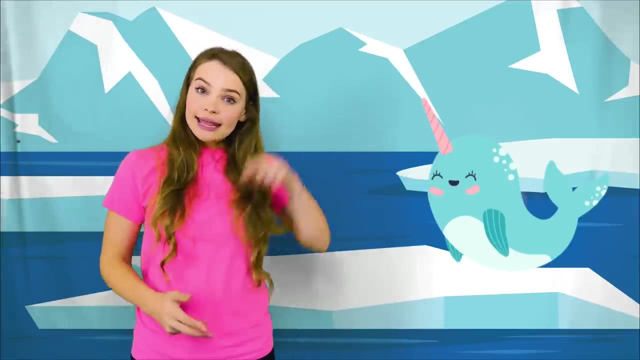 A narwhal looks like a whale with a horn on top of its head, Like a unicorn in the sea. That's pretty silly. They love to be in cold waters and they use their horn to break up the ice if they need to. 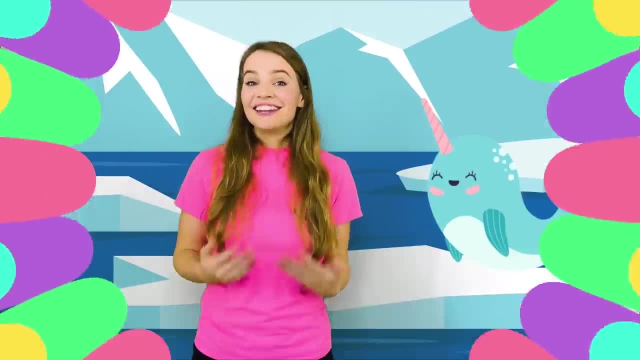 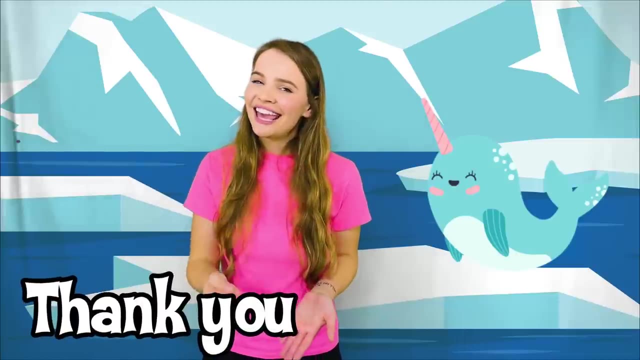 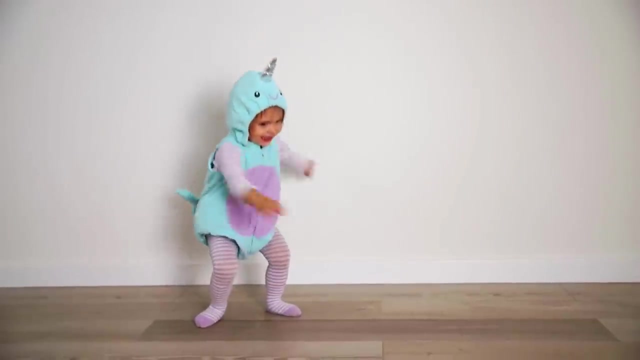 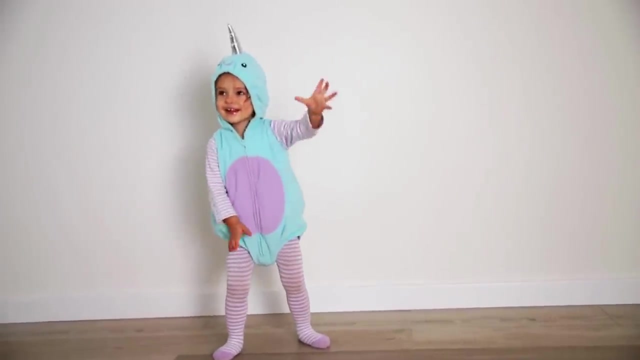 And swim around. The narwhal is the unicorn of the icy Arctic seas. He likes to say: excuse me, thank you and please, How kind. That's very nice, narwhal. Now I'm walking through the zoo and I'm looking for the letter O. 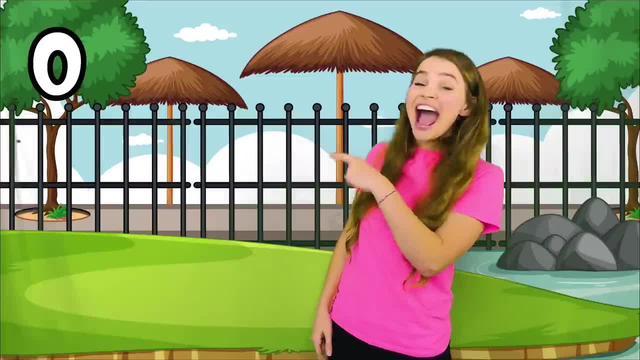 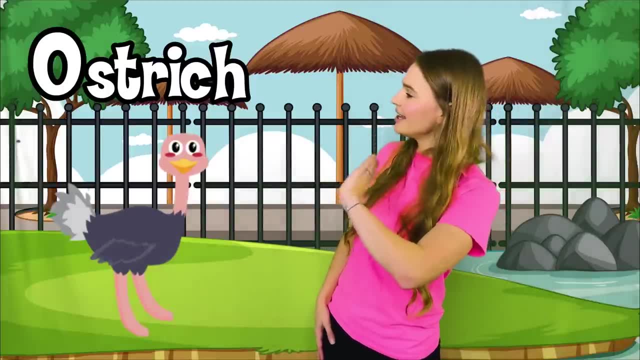 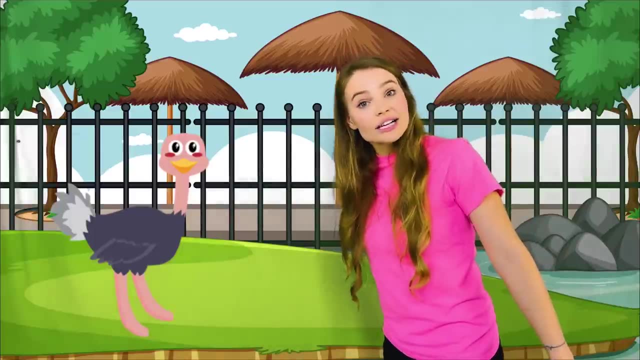 Do you see the letter? O? Hmm, Oh, yeah, right there O for an ostrich. Hi ostrich, how are you? Ostriches can run really fast. They open up their wings and they run really fast. You wanna run like an ostrich with me? 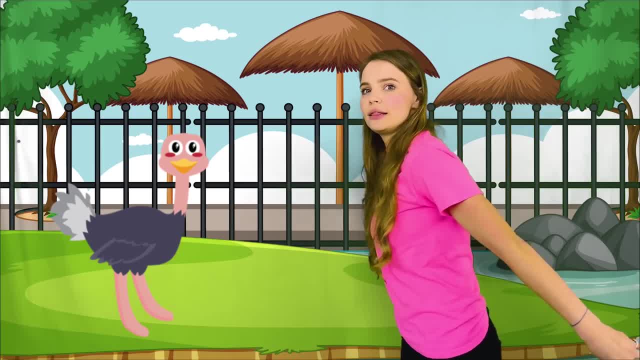 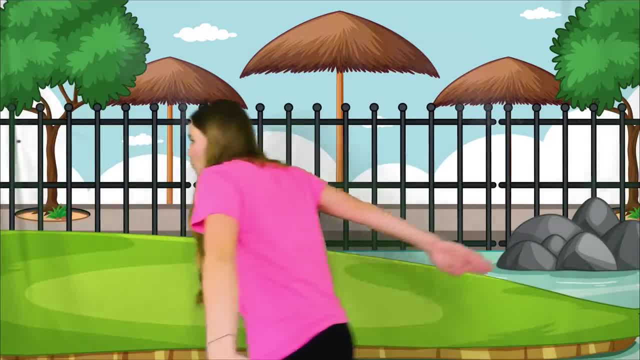 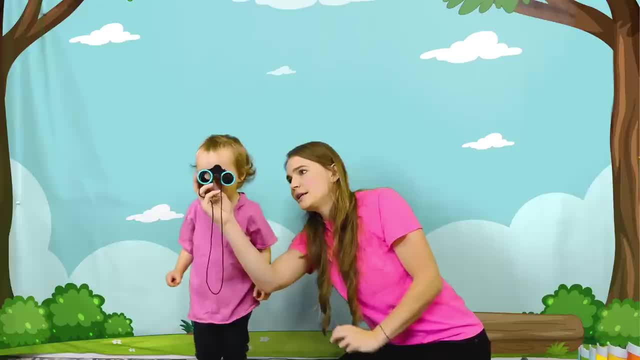 Whoa, so fast. Whoa, ostrich, whoa, You make a great ostrich. You wanna see. if you see an ostrich, Yeah, Come look. do you see an ostrich? Yeah, Where You see one. 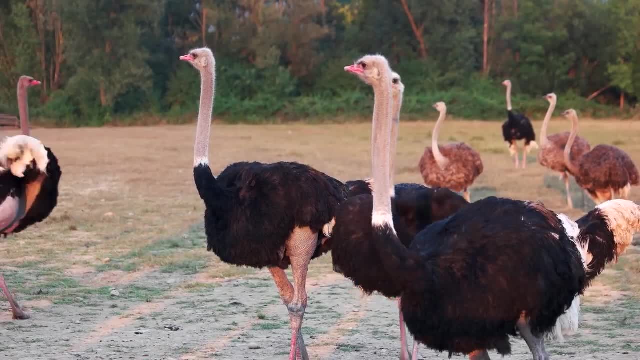 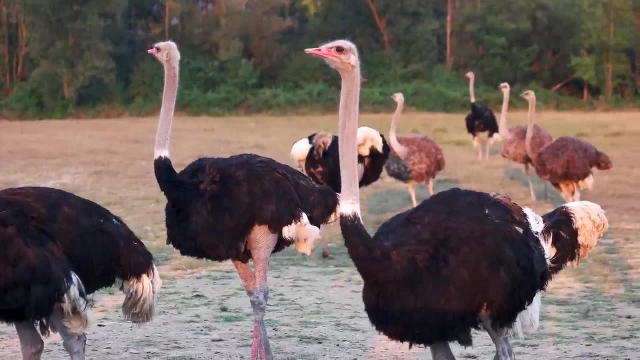 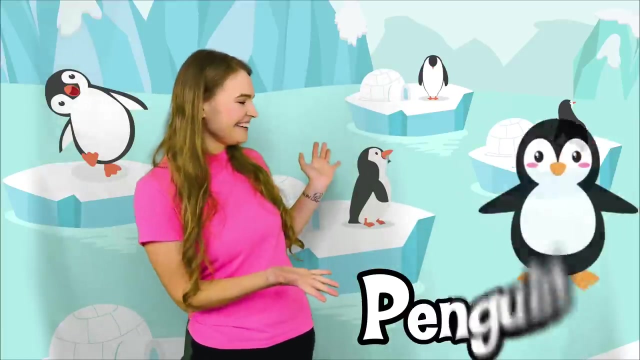 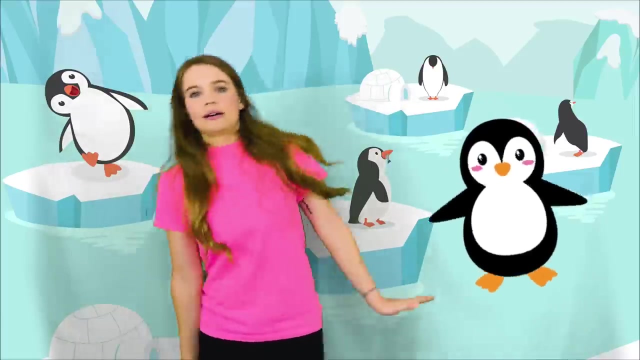 Right there, Hi ostrich, Walking, walking through the zoo and looking for the letter P for p, p penguin, Hi penguin, Nice to meet you. Penguins like to waddle, like this: Waddle, waddle, waddle, waddle, waddle. 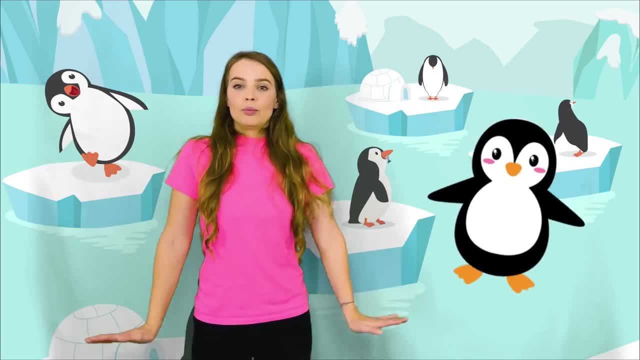 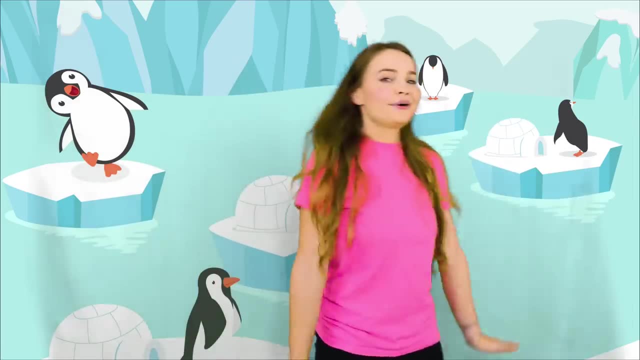 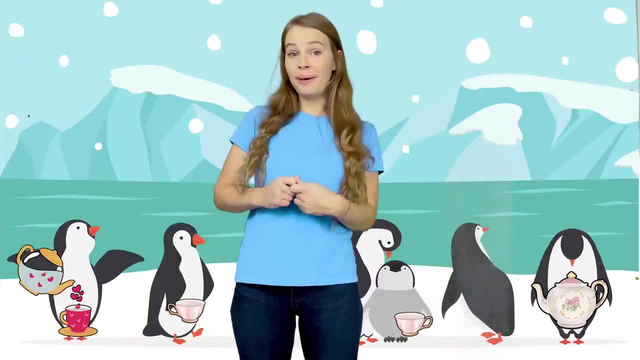 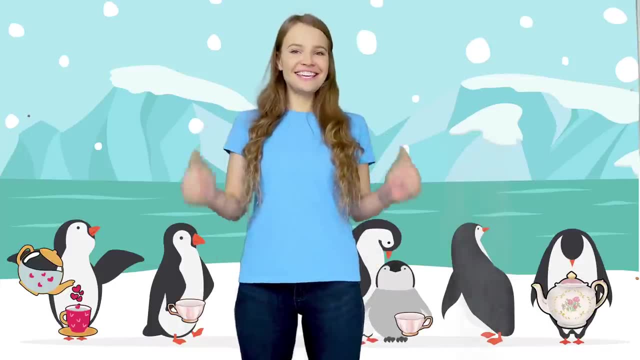 How silly. This is a silly song about a penguin who likes to drink some tea. Have you ever seen a penguin drinking tea? Take a look at me, A penguin, you will see Penguins. attention, Penguins. unite Right arm. 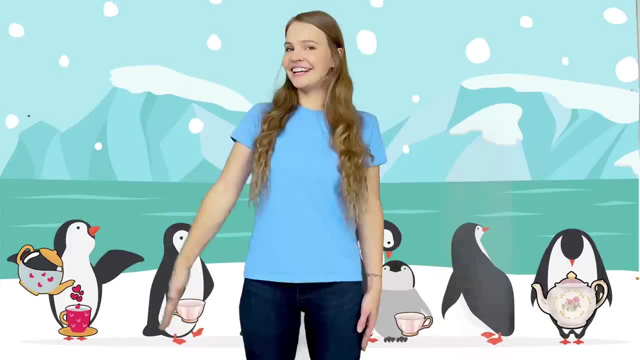 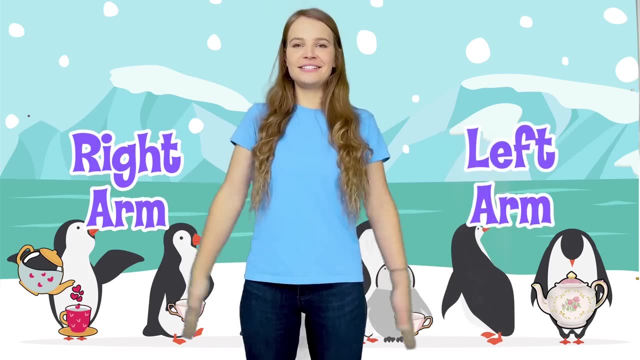 Have you ever seen a penguin drinking tea? Take a look at me. A penguin, you will see Penguins. attention, Penguins unite Right arm, left arm. Have you ever seen a penguin drinking tea? Take a look at me. 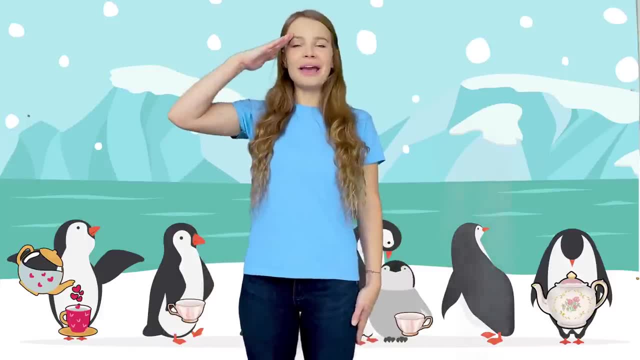 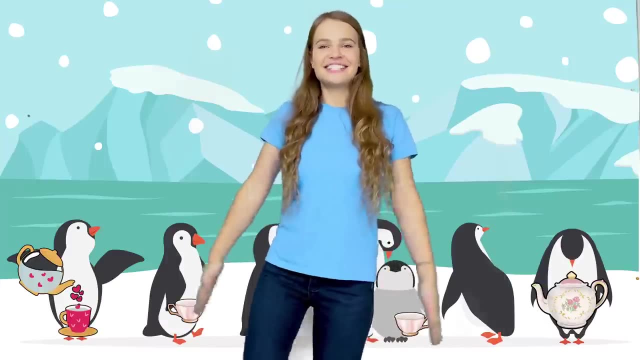 A penguin. you will see Penguins. attention Penguins unite. Right arm, left arm, right leg. Have you ever seen a penguin drinking tea? Take a look at me. A penguin, you will see Penguins. attention Penguins unite. 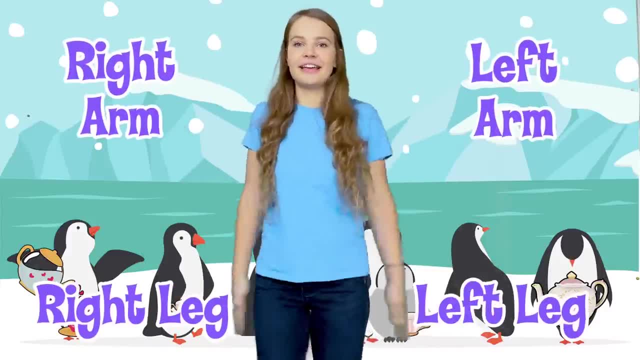 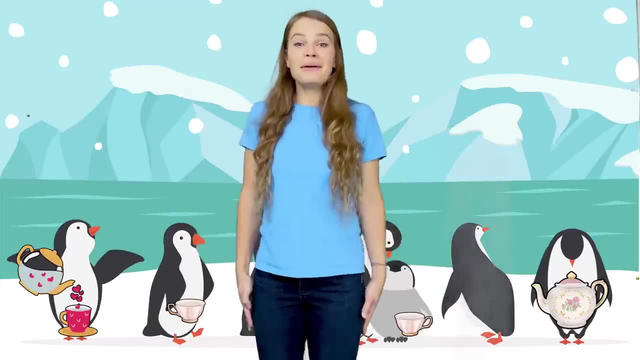 Right arm, left arm, right leg, left leg. Have you ever seen a penguin drinking tea? Take a look at me, A penguin, you will see Penguins. attention, Penguins unite. Right arm, left arm, right leg, left leg, head bow. 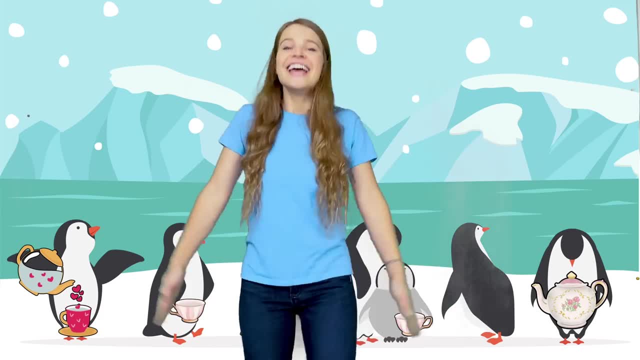 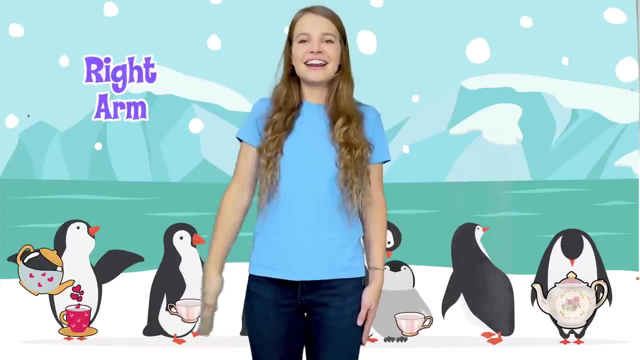 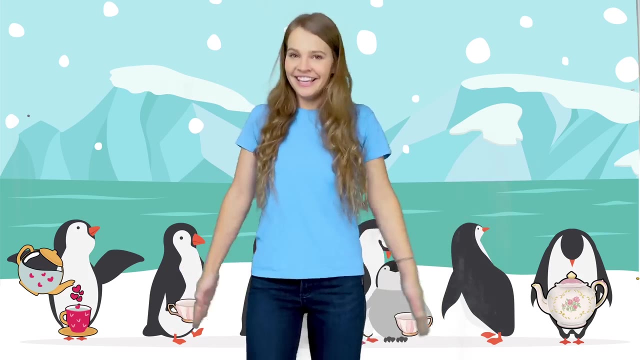 Have you ever seen a penguin drinking tea? Take a look at me, A penguin, you will see Penguins. attention, Penguins unite: Right arm, left arm, right leg, left leg, head, bow, Turn around. Have you ever seen a penguin drinking tea? 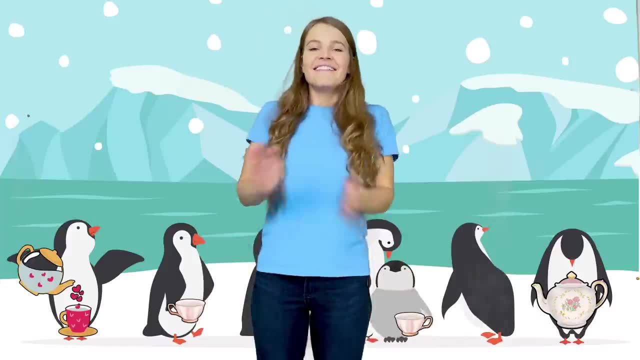 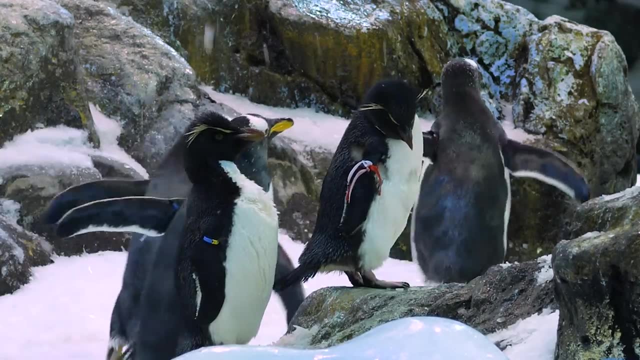 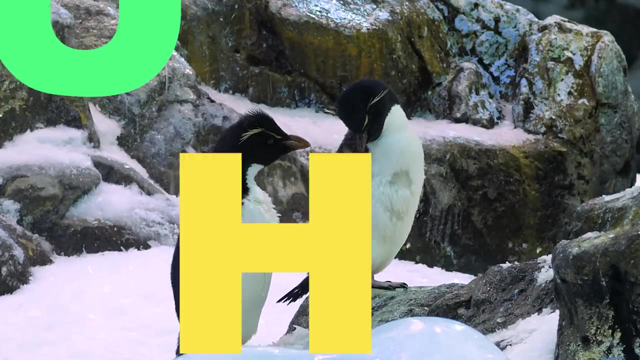 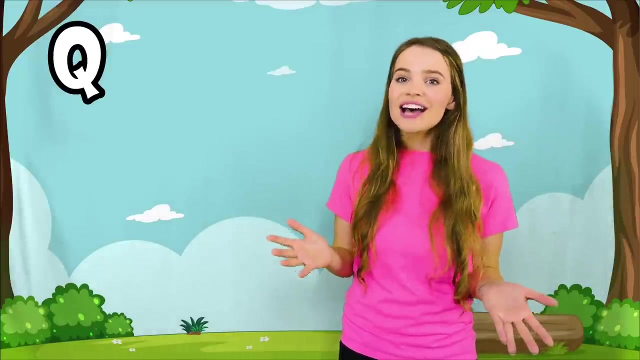 Take a look at me- A penguin, you will see. Wow, You make a great penguin. Thank you for playing with me. I'm walking through the zoo and now I'm looking for the letter Q. Q makes the kwa kwa kwa sound for quail. 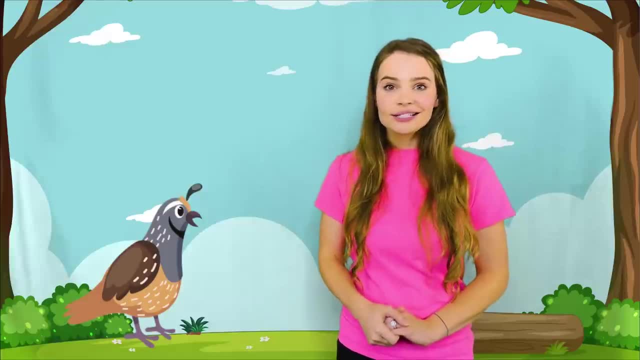 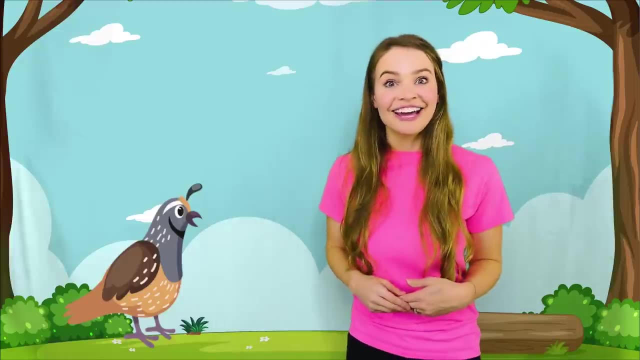 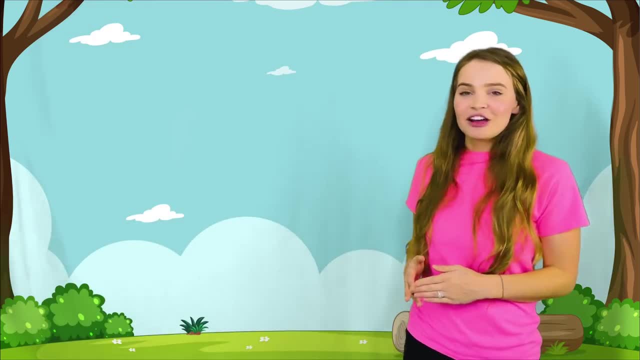 Wow, Vroom, vroom, vroom, vroom, vroom, vroom, vroom. Whoa. Okay, let's do it one more time. ready Vroom, vroom, vroom vroom, vroom, vroom, vroom. 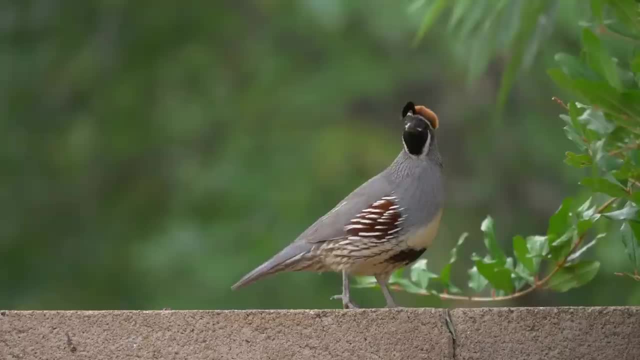 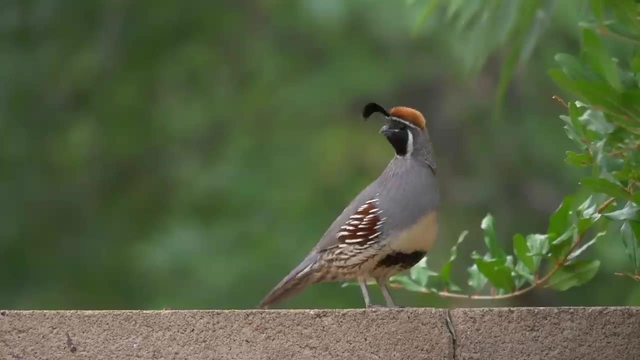 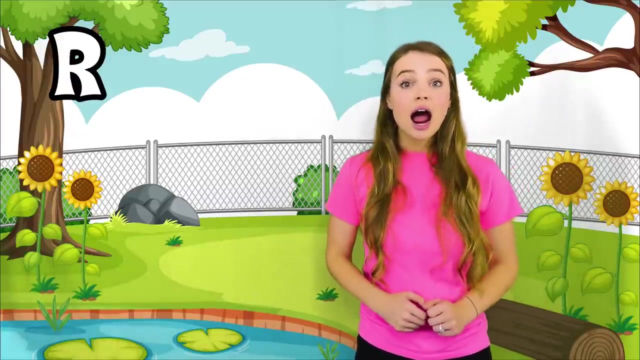 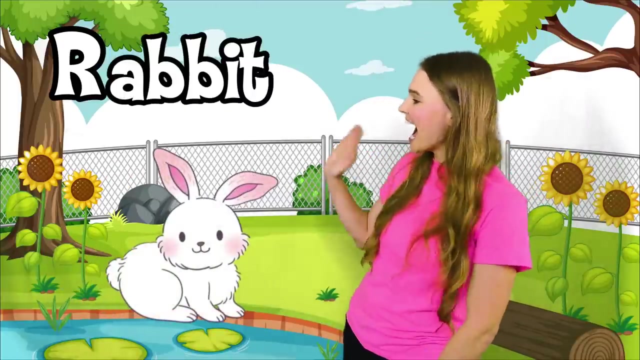 Wow, You make a great quick quail Woo. I'm walking through the zoo and I'm looking for the letter R that makes the r r r sound for rabbit. Hi rabbit, It's so nice to meet you. 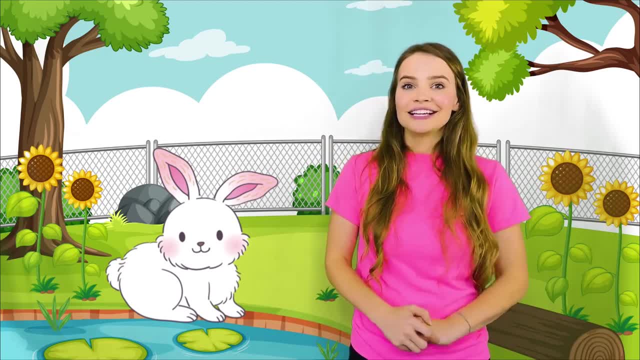 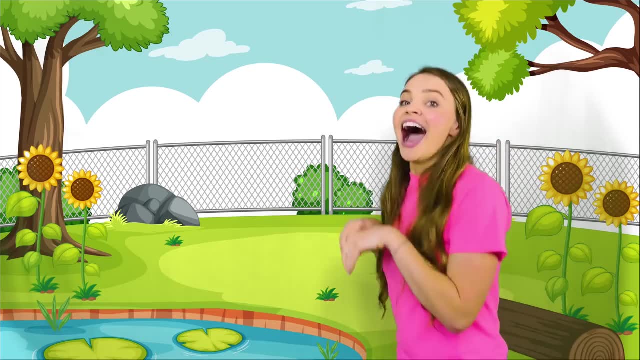 I like your two ears and I like how you like to go. hop, hop, hop. Should we hop like bunnies? Okay, I'm gonna hop from this side to that one Ready Hop, hop, hop, hop, hop. 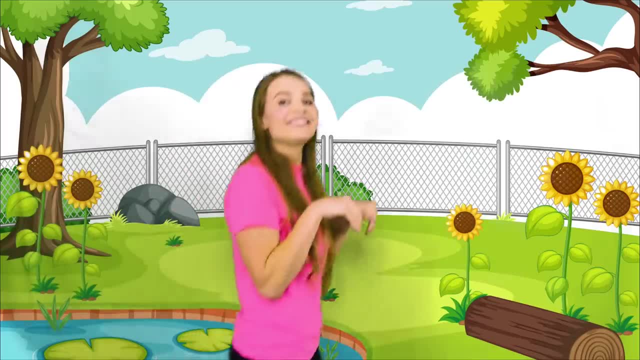 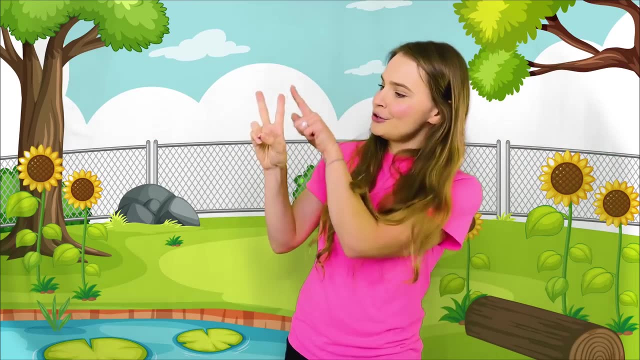 Now let's go back Ready. Hop, hop, hop, hop. This is my friend rabbit, or a bunny. He's got two ears and he likes to go hop, hop, hop, hop, hop. Bunny says hello. It's nice to meet you. 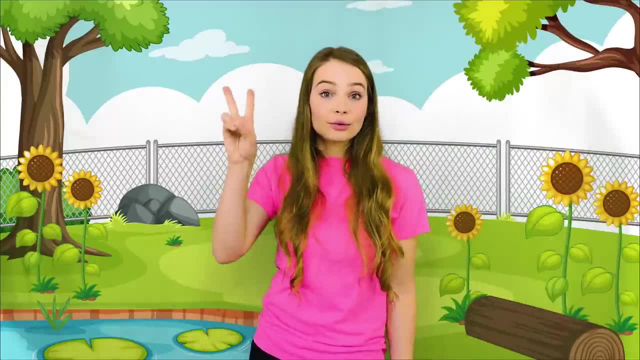 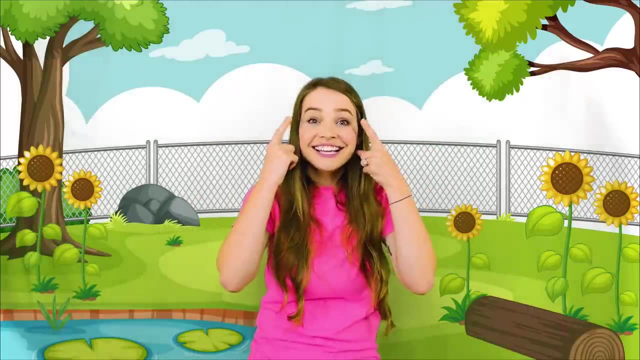 Hop, hop, hop. I saw a little rabbit go hop, hop, hop. I saw his little ears go flap, flap, flap. I saw his little eyes go blink, blink, blink. I saw his little nose go twink, twink, twink. 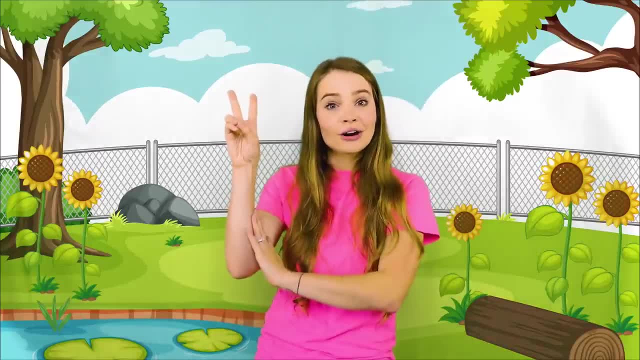 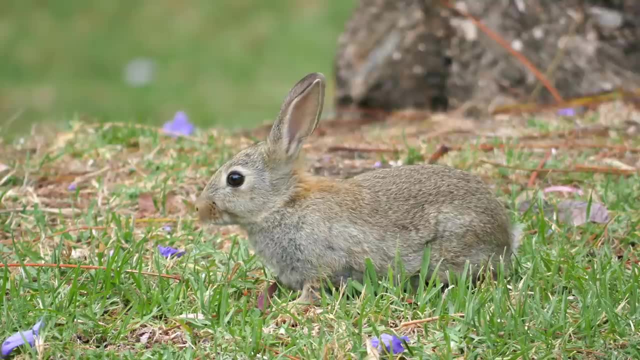 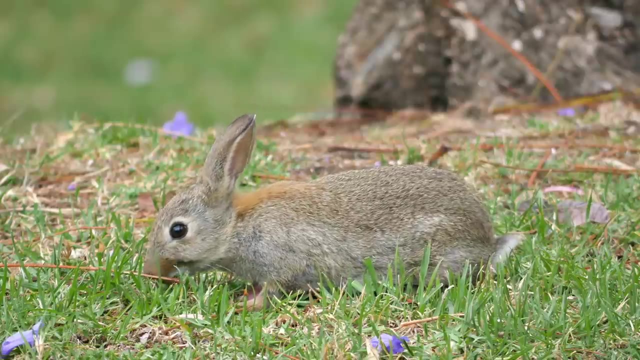 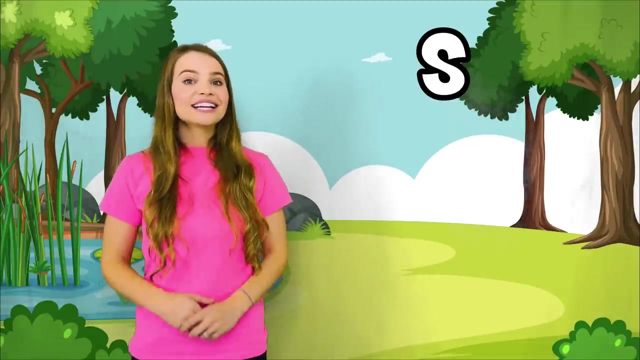 You see his little fur, so soft and furry, And now let's watch him hop away in a hurry Bye rabbit. I'm walking through the zoo and I'm looking for the letter S that makes a sound for sloth, Hi, sloth. 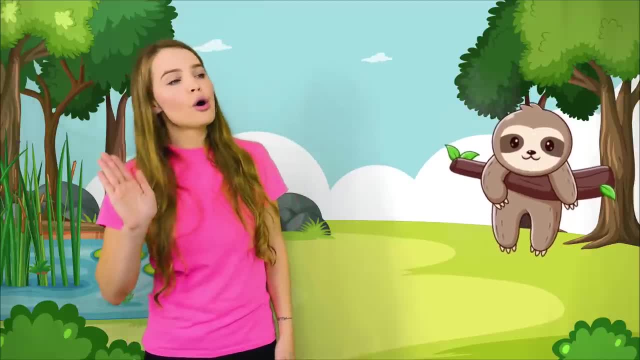 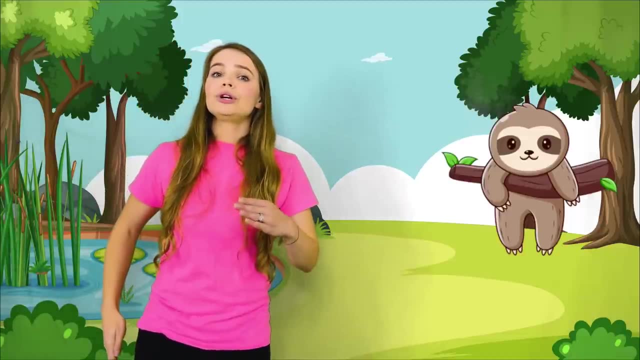 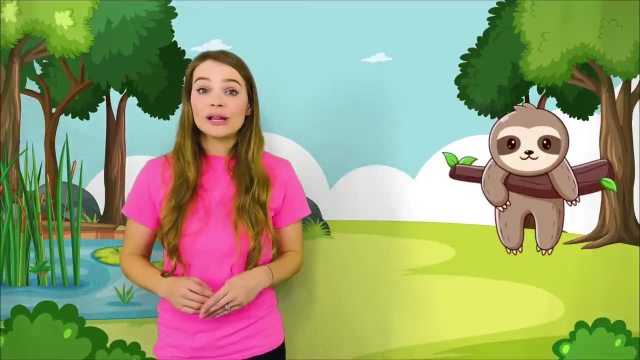 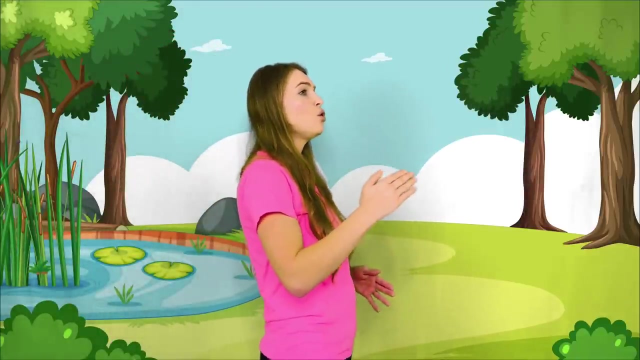 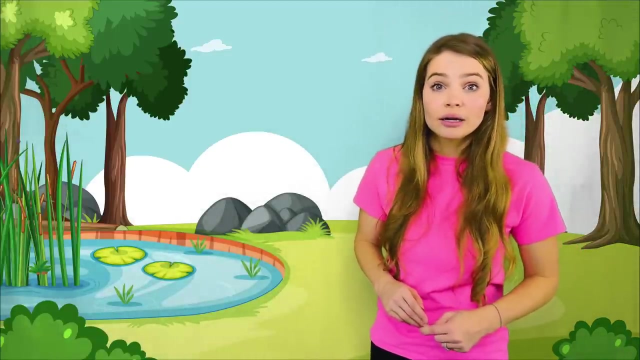 Sloth says hello, Hi, sloth, It's very nice to meet you. Sloths can really slow down and slow. Let's move really slow like a sloth: Slow, slow, slow. But sloths can actually swim really fast in water. 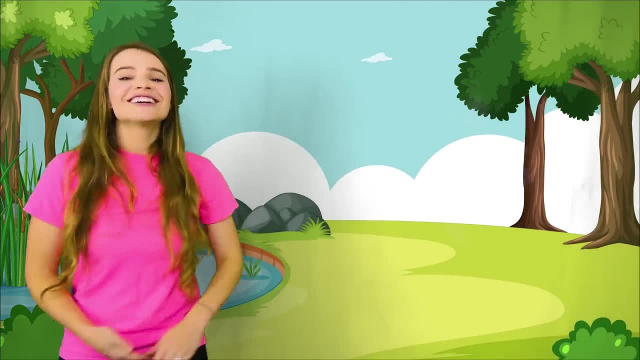 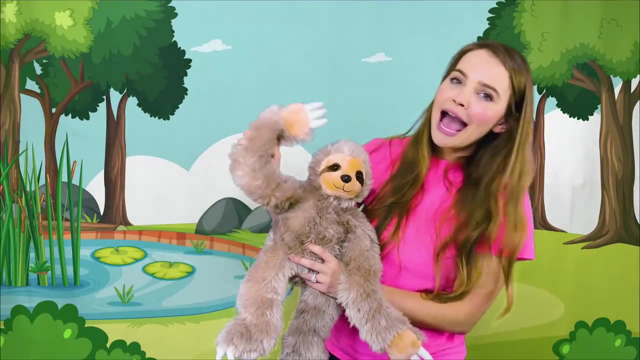 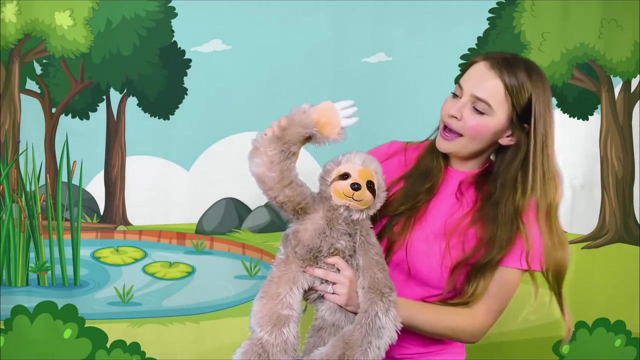 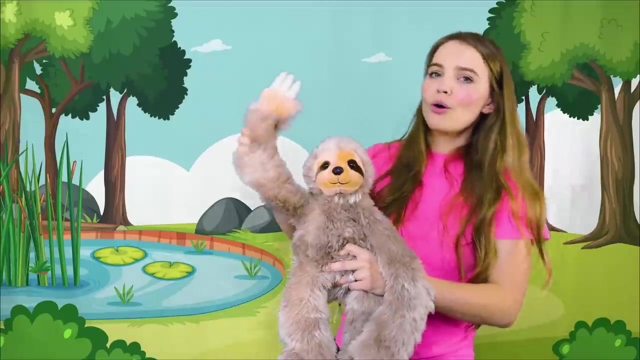 Let's swim really fast, Ready Whoo, whoo, whoo, whoo, Great swimming. This sloth says: hello, Hello, Hello. How are you? Hello, How are you, Hello, How are you? How are you this morning? 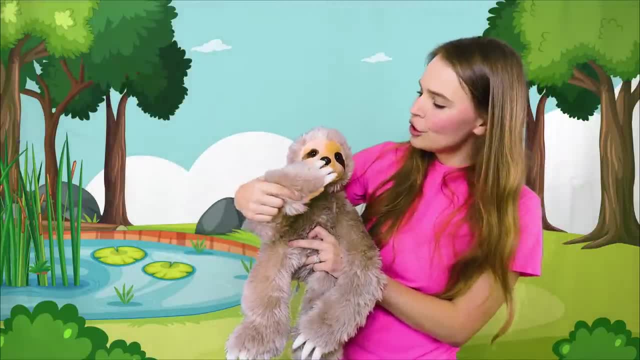 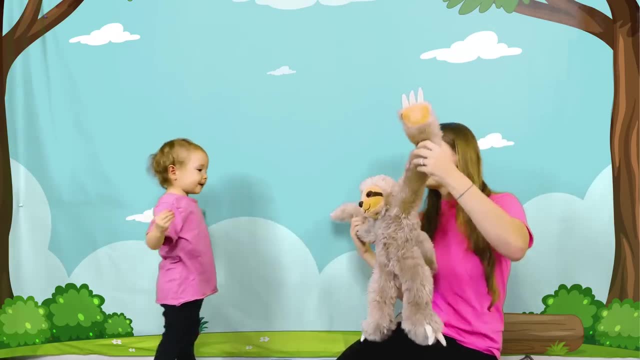 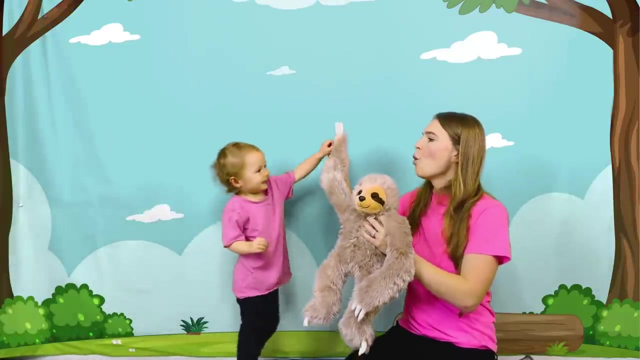 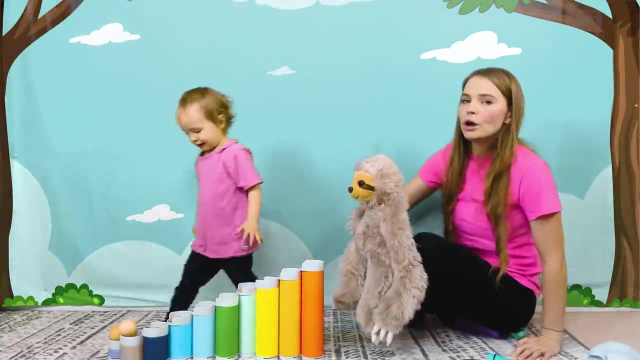 Oh, that was a beautiful song, Sloth. Thank you, Sloth. A really slow high five, Sloth, Thank you. Thank you. Why Will you show me how you do that again? I grab a ball. You did, Let me see. 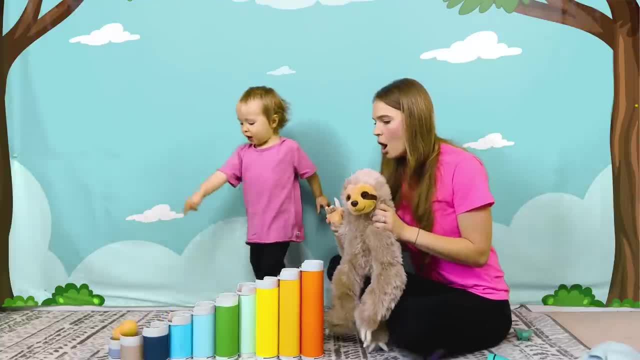 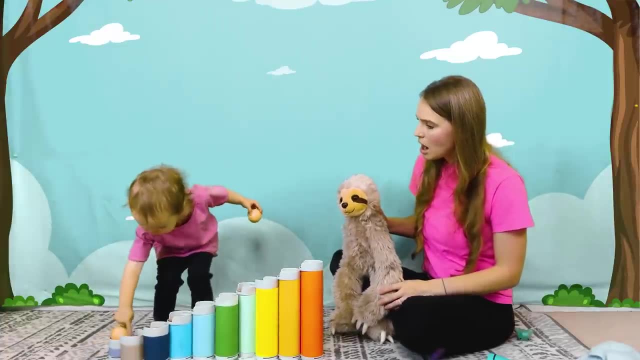 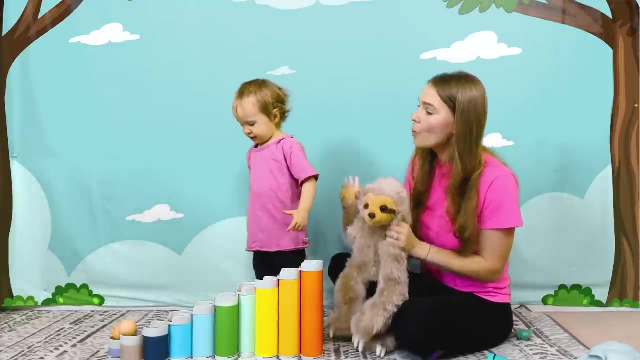 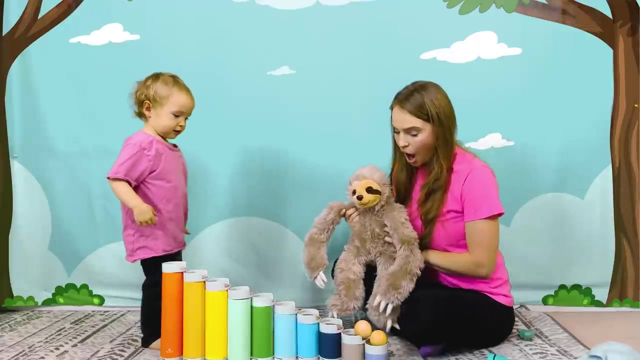 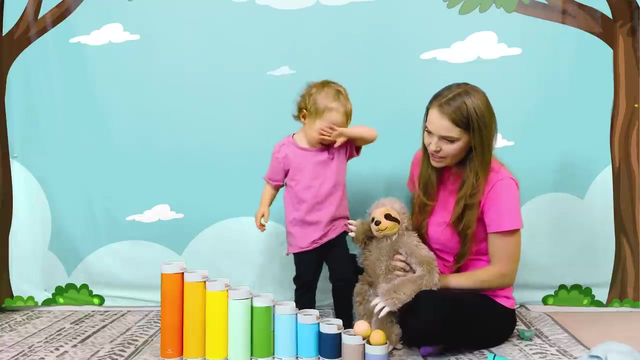 And put it up here, Right, and then what? And then pull an elbow, Oh wow. And then down down, Wow, will you show me yours? Yes, Wow, It rolls down like that, Wow, Wow, that's really great. 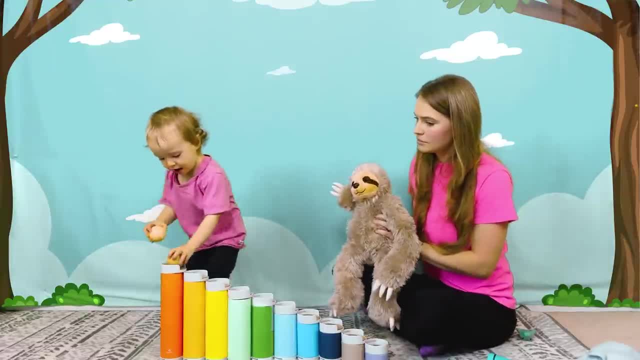 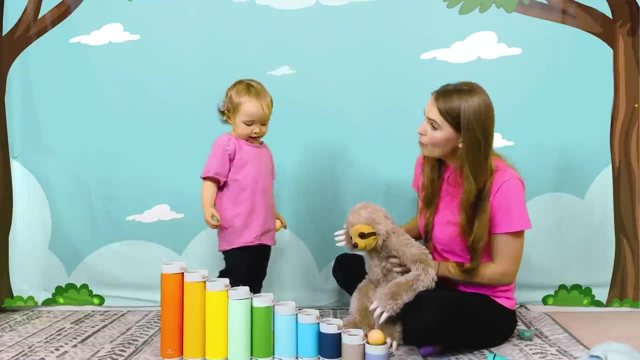 Okay, One right here, One down here, One down here: Oh wow, Wow. I got a donk. Oh wow, I got a donk. Swoosh Oh wow, Swoosh, Oh wow. 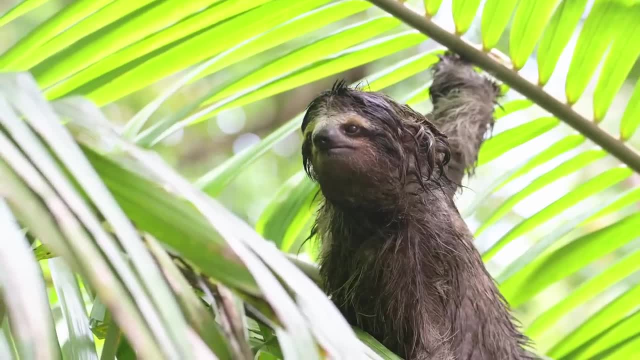 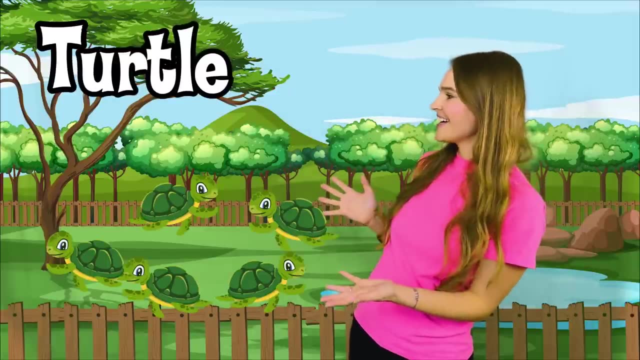 Swoosh, Oh wow, Swoosh, Swoosh, Swoosh, Swoosh, Oh wow, Swoosh. Oh wow, There's a turtle set. Now let's find the letter T for T, T, T, Turtle. 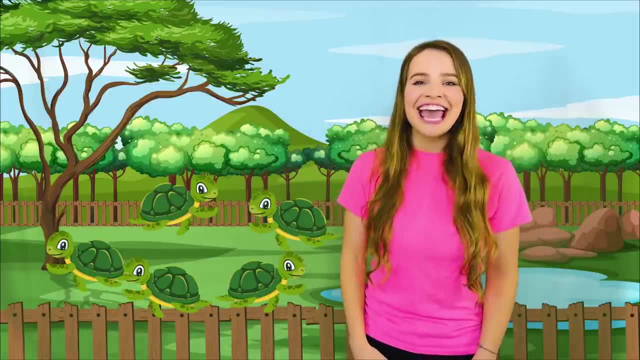 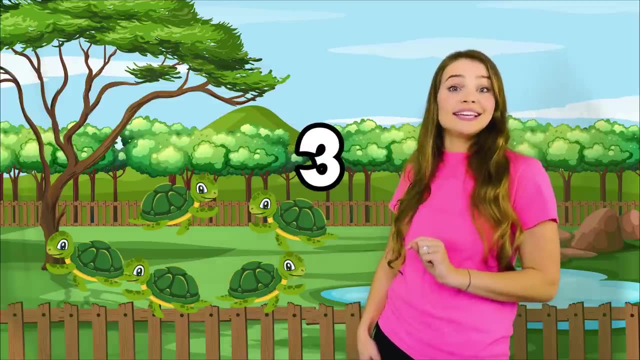 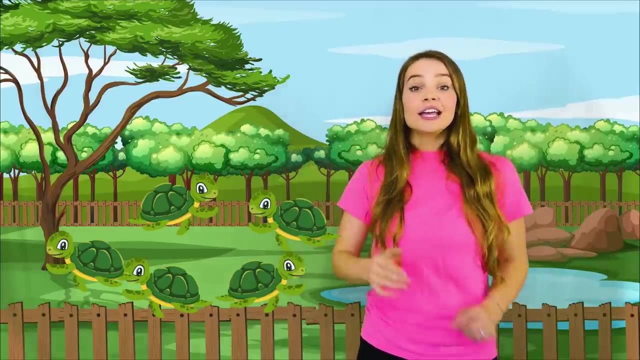 Oh wow, There's many turtles here. Let's count them. One turtle, Two turtle. Oh wow, One turtle, Two turtles, three turtles, four turtles, five turtles, five turtles. Turtles also move really slow like this. 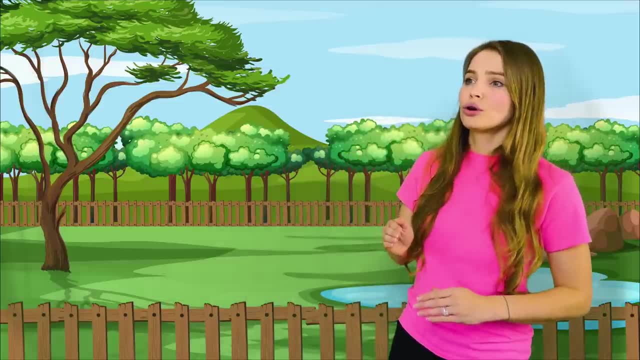 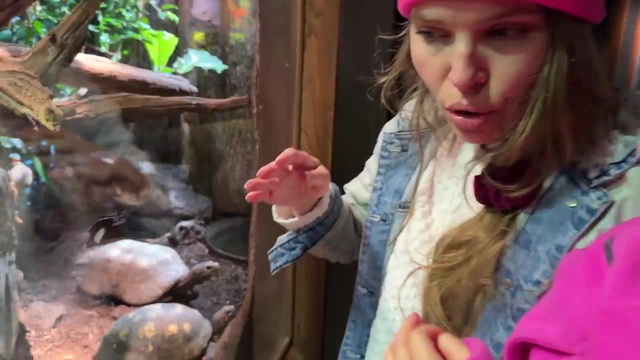 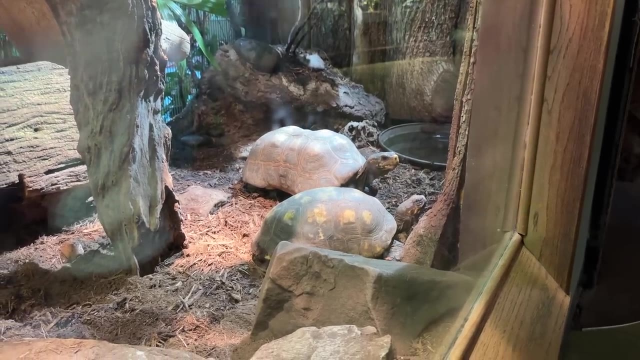 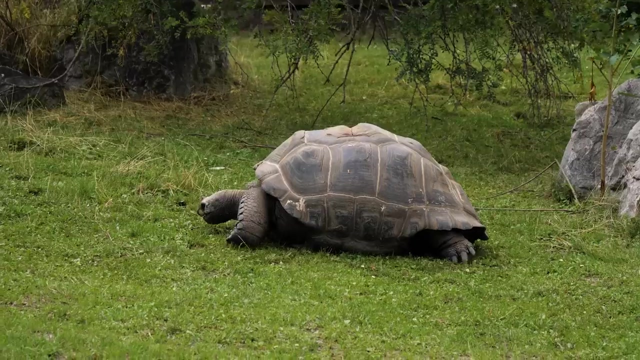 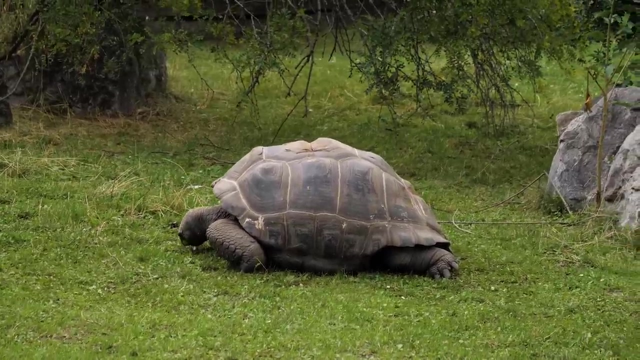 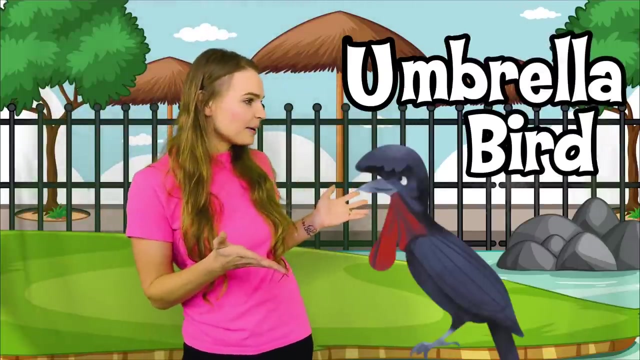 Slow turtle. That's very silly, Slow turtle. Hello turtle, How are you today? You see their eyes. Where's he going? Blink, blink, Blink, blink, blink. I'm walking through the zoo and I'm looking for the letter U for a, a, a umbrella bird. 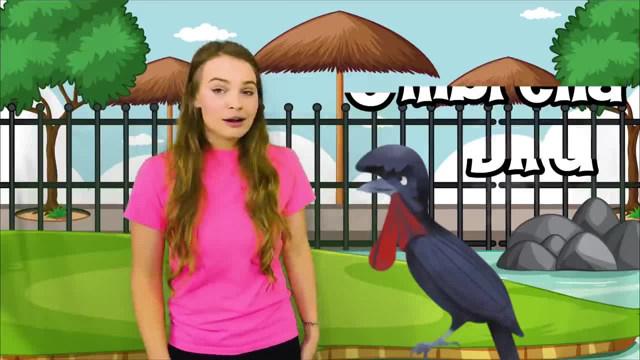 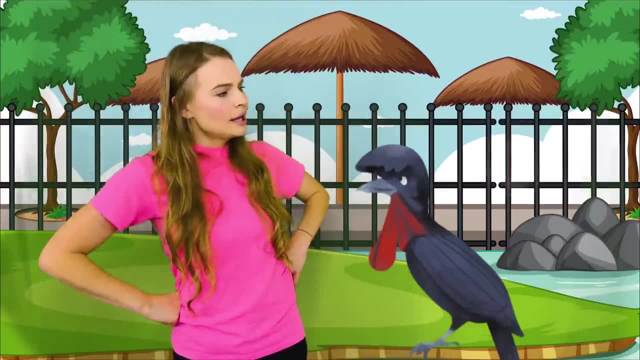 Oh, Wow, hey there, umbrella bird. Umbrella birds look like they have an umbrella on their head. I bet they don't get wet in the rain. Umbrella bird, you like being in the rain because you don't get wet. 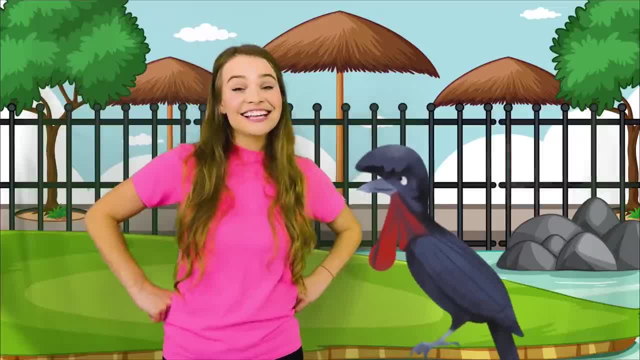 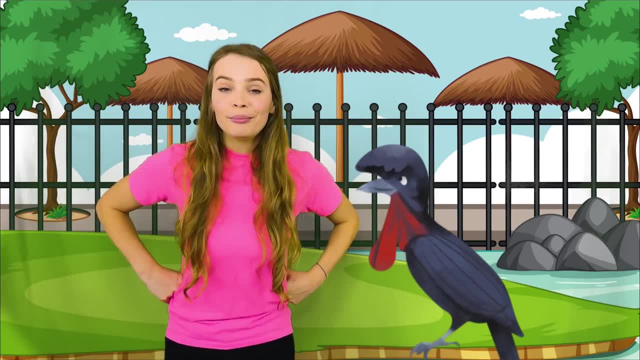 Umbrella bird says: yeah, I've got an umbrella on top of my head. That's really cool. Umbrella bird, do you like jumping in puddles? Oh yeah, says umbrella bird, Let's pretend to jump in puddles together. 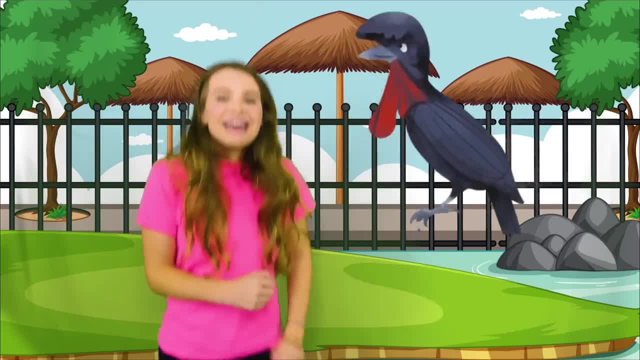 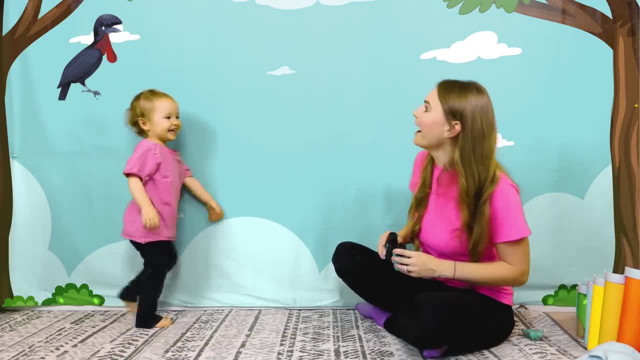 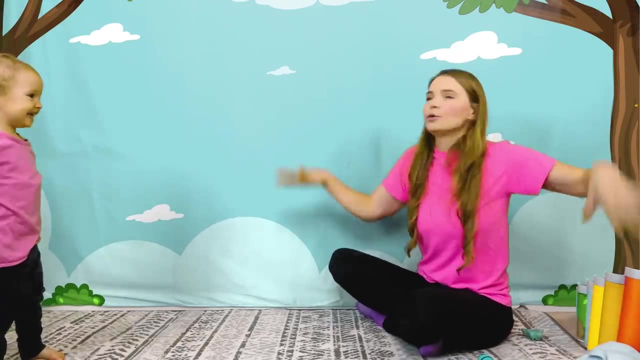 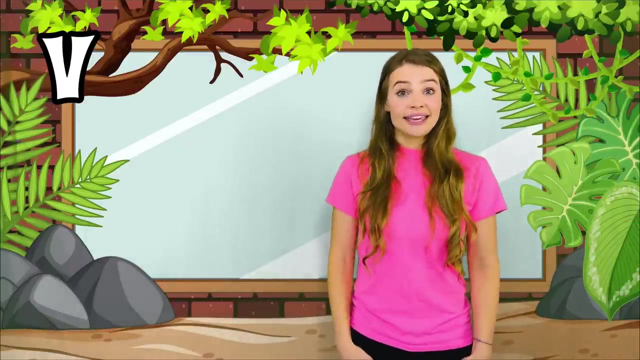 Ready. Splash, splash, splash, splash, splash, Great jumping. Hello umbrella bird. Hello, Hello, Hello, Hello, Hello. How do birds fly So fast? Now I'm walking, walking, walking and I'm looking for the letter V V makes the v v v sound. 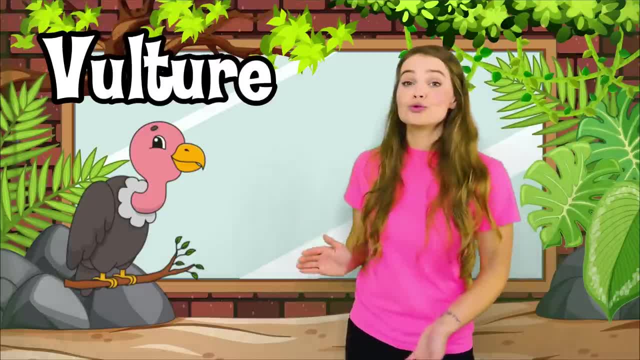 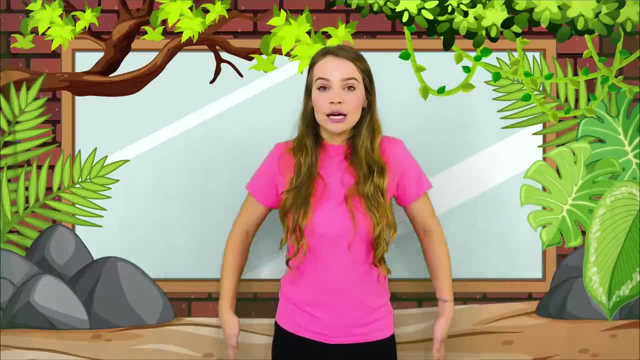 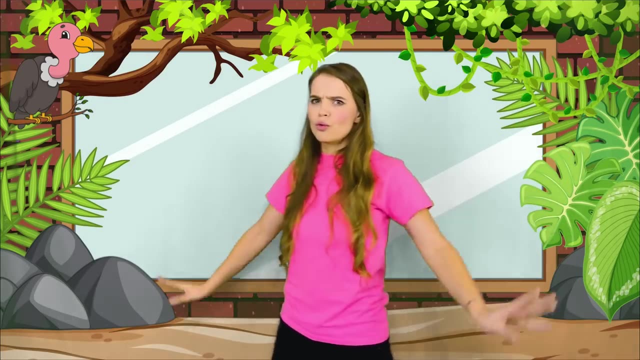 for vulture. Ooh, vultures are really big birds. They have big wings Ready. Let's pretend to be vultures together. Get your wings out, We'll flap them. Let's fly around. Ooh, we're vultures. 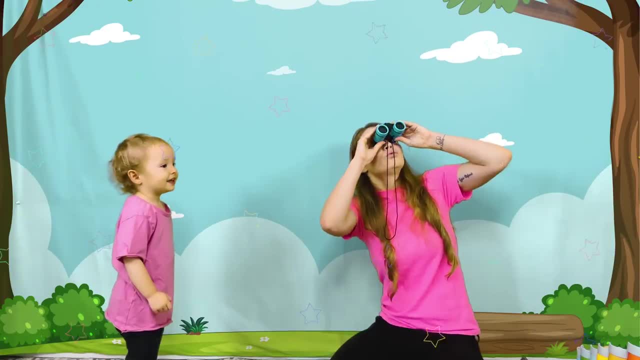 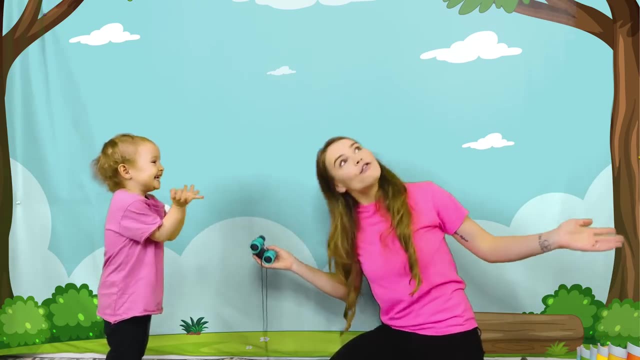 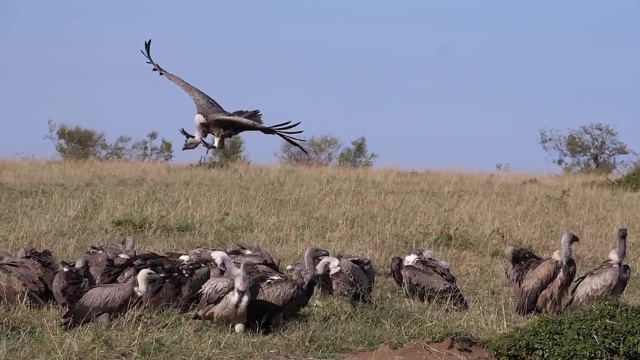 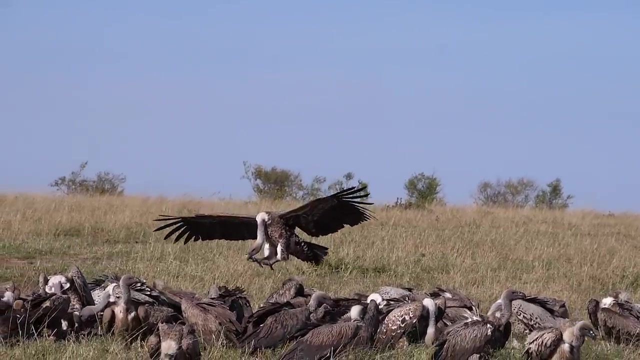 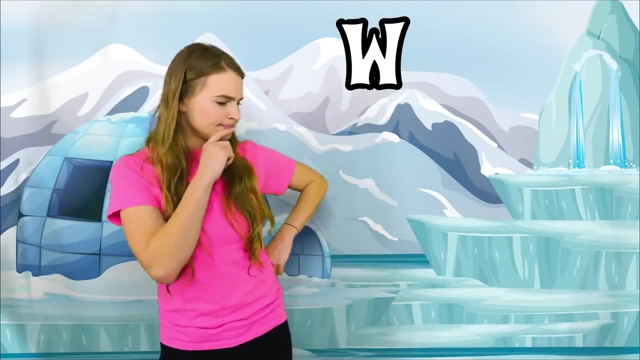 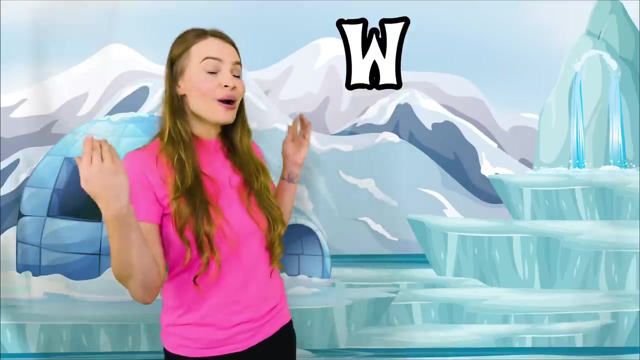 Flying, flying, flying. Great job, Wow. a vulture With big wings. A vulture, Yeah, I'm looking for the letter W. Do you see a letter W? Hmm, Oh, yeah, right there. W makes the w-w-w sound for w-w-walrus. 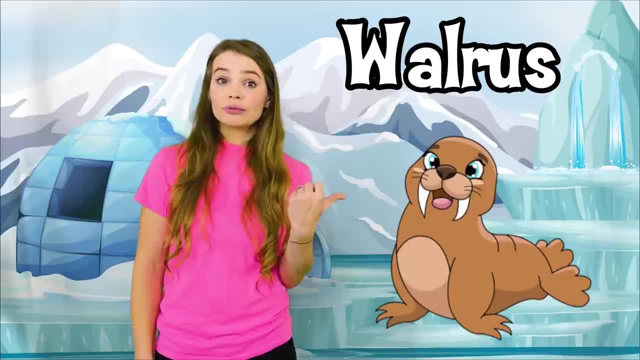 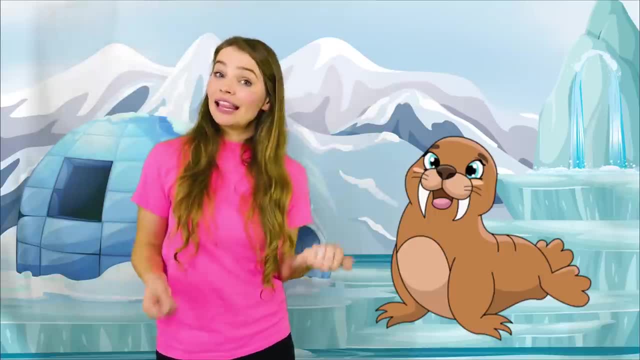 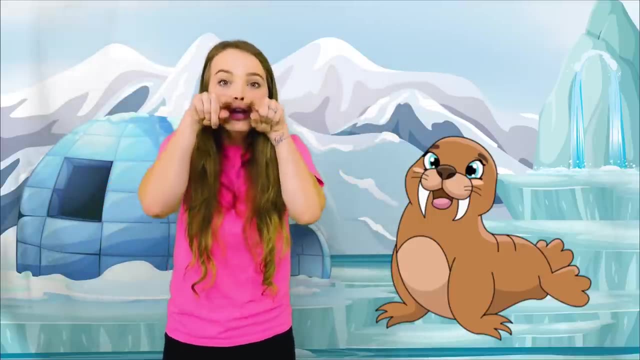 Hi walrus. How about this walrus? It's got two tusks, Kind of like two big teeth up front Tusks. Elephants have tusks too. huh And walrus do two tusks. Can you put your fingers out like tusks? Tusks. 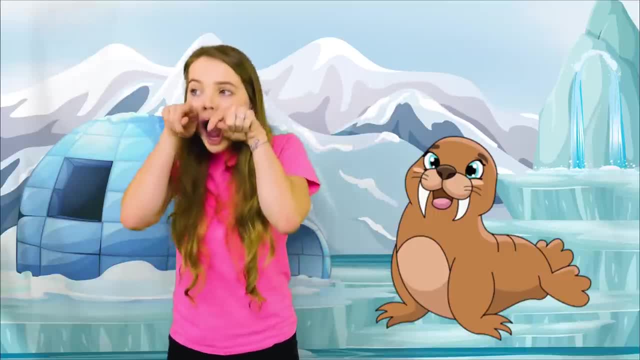 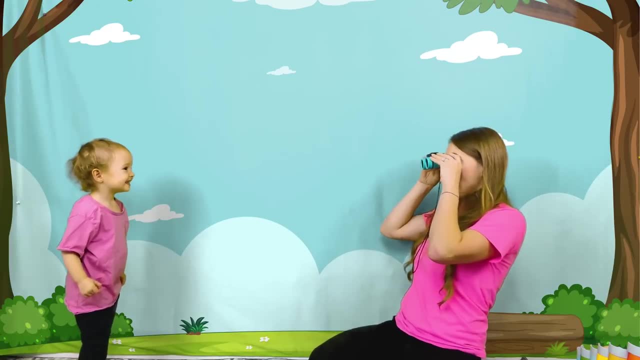 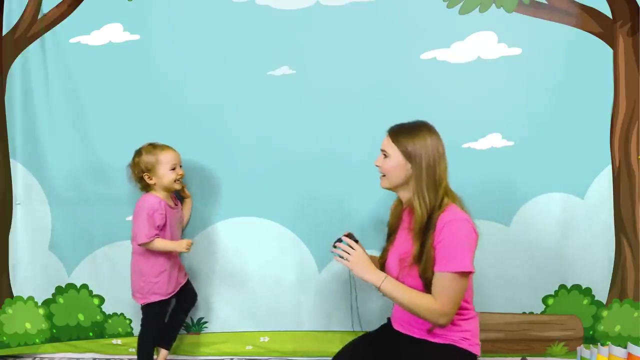 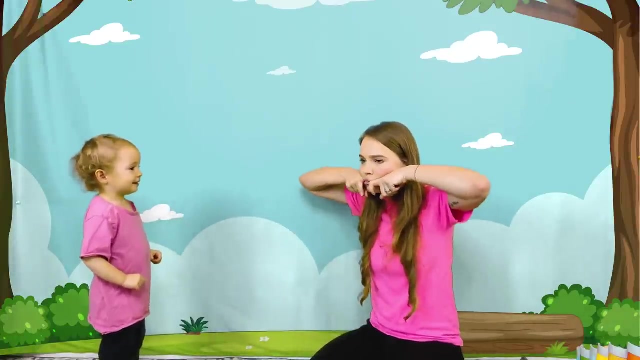 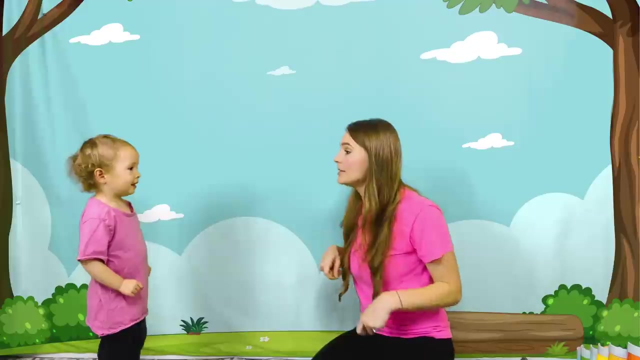 I'm a walrus. I'm a walrus. How silly. Wow, Wow, A walrus. Wow, Did you know? walrus have tusks. Think of my language: Giraffes have horns, Walruses have tusks. Helps them eat their food better, It's like their teeth. 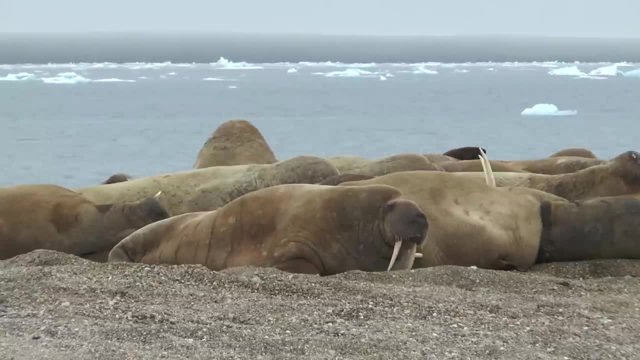 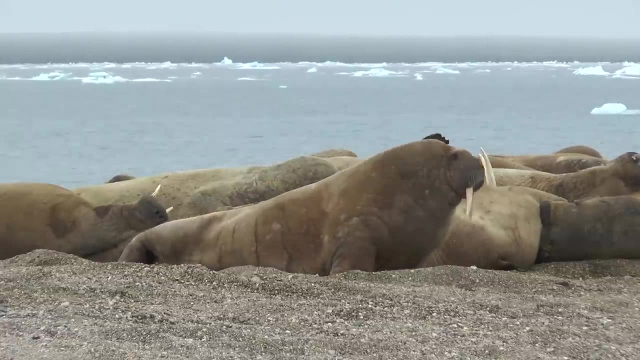 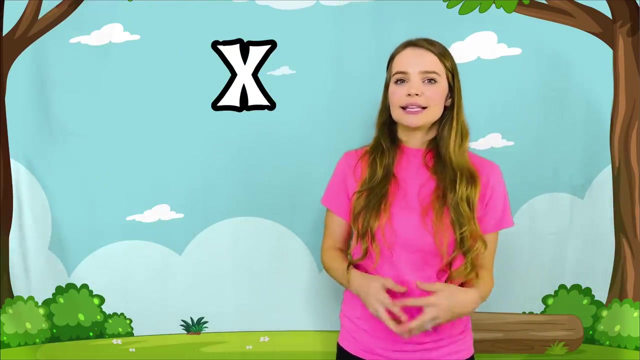 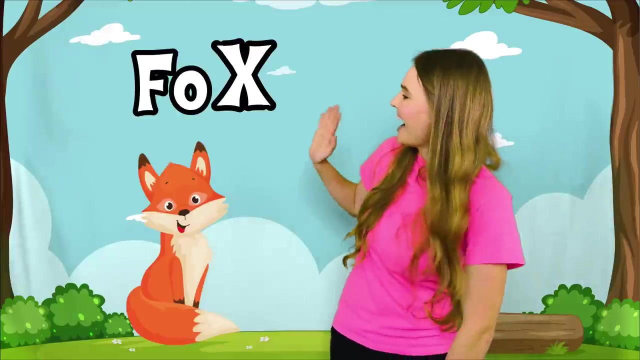 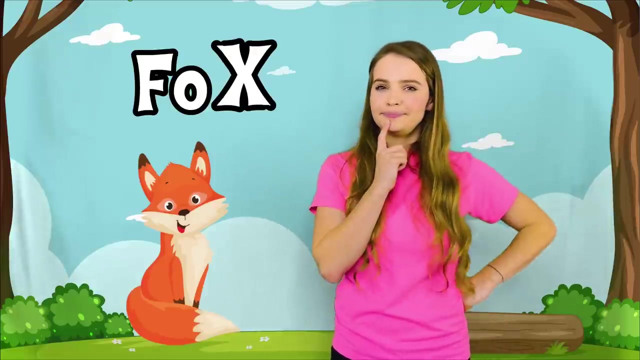 I'm a walrus. Now we're walking through the zoo and I'm looking for the letter X. X makes the x-x-x sound, and you can find it at the end of the word fox. Hi fox, Nice to meet you. How about a sillier rhyme about a fox? Hmm, How about a fox? 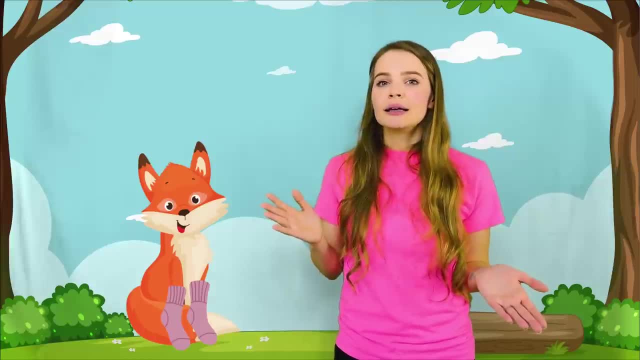 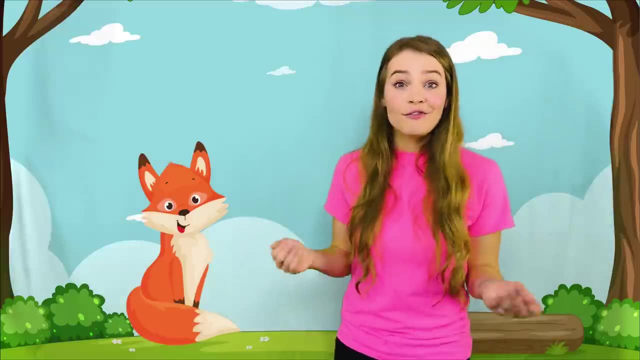 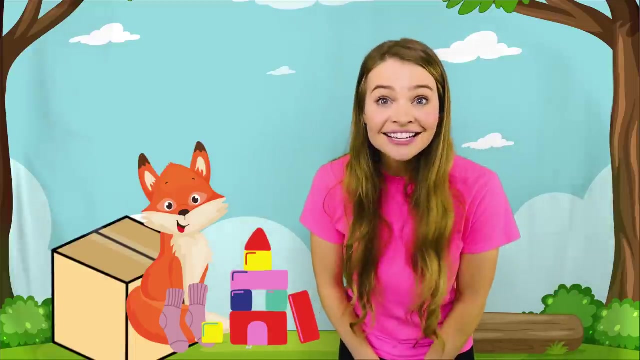 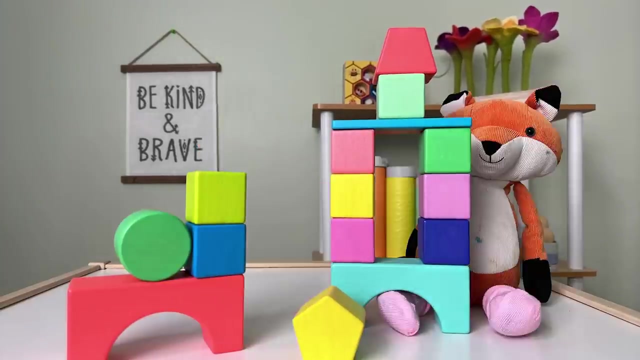 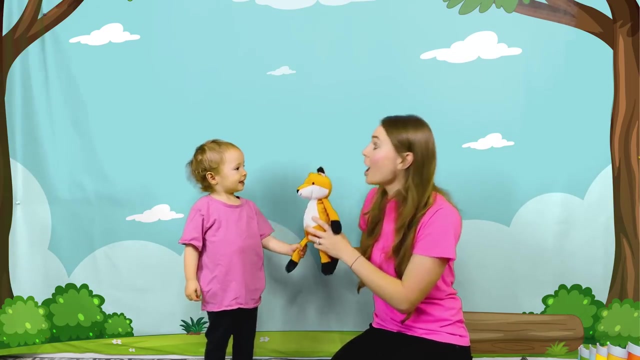 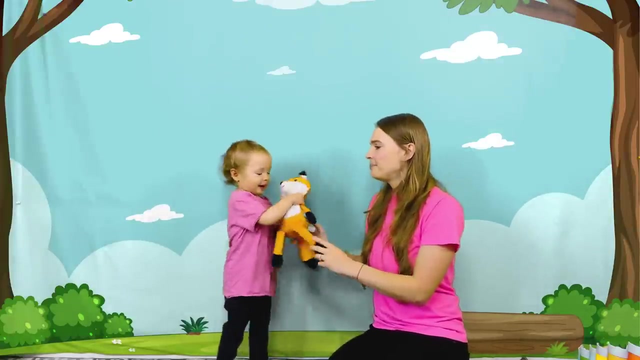 Wearing socks, Playing with blocks Inside of a box. That's pretty silly. A fox wearing socks, Playing with blocks Inside of a box- How silly. How about a fox playing blocks, wearing socks in a box? I like a box. 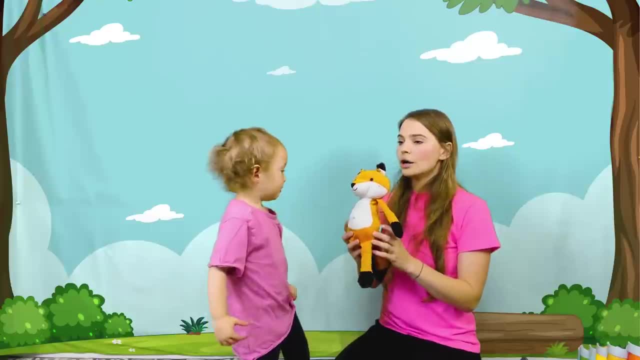 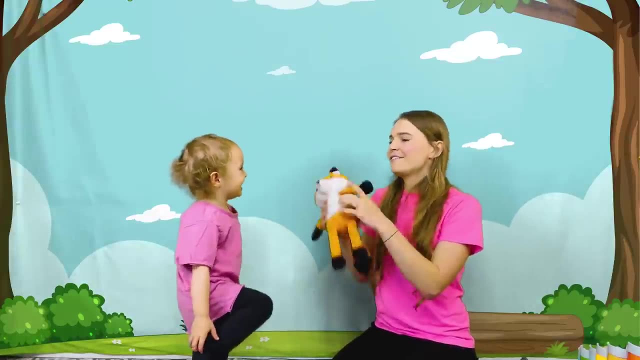 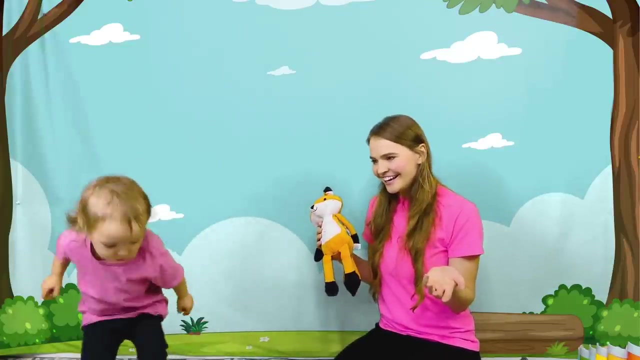 I also like blocks. Paisley, if you want to play blocks, Or do you know how to sign socks Like this would point at our feet: Socks Fox wearing socks, playing blocks in a box. Oh many emeralds. 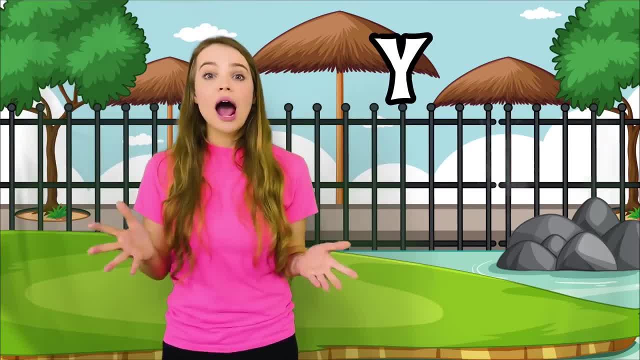 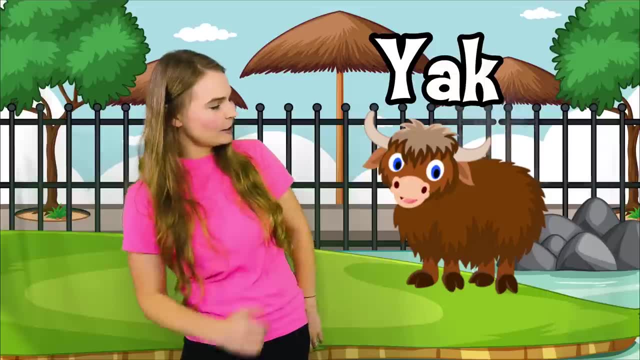 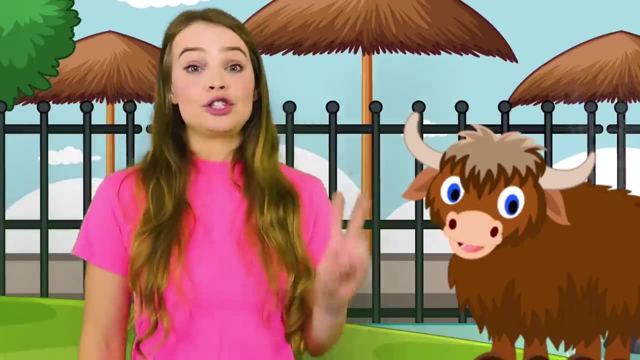 I'm walking through the zoo and I'm looking for the letter Y that makes the Y sound for yak Hi. yak Yak says hello, Hello, it's very nice to meet you. Did you know that yaks have two steps? One, they eat their stomachs and it helps them digest their grass better when they chop it. 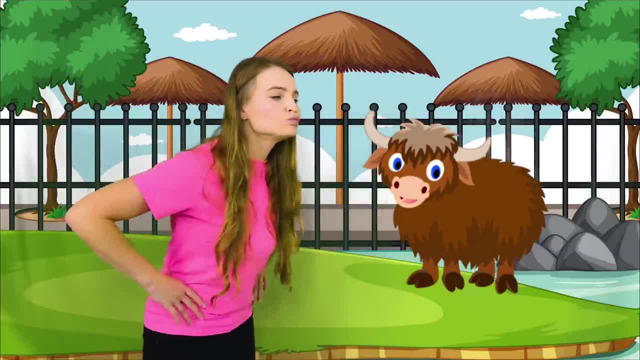 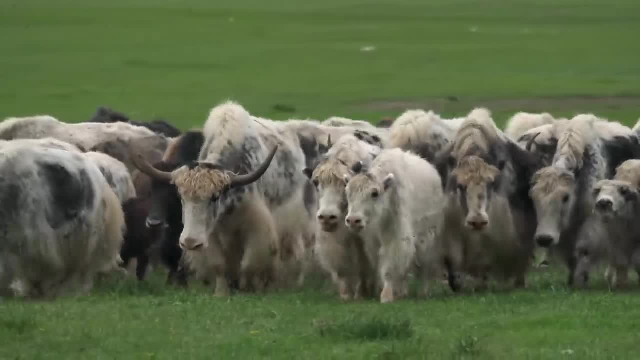 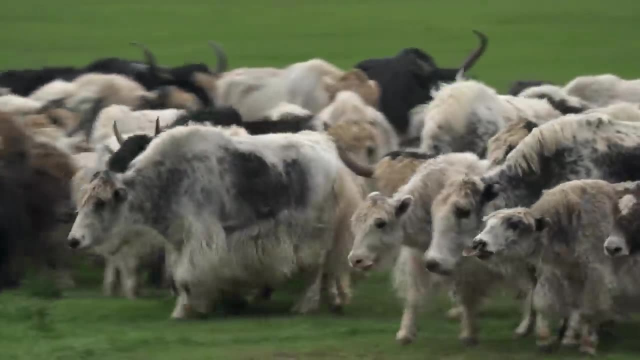 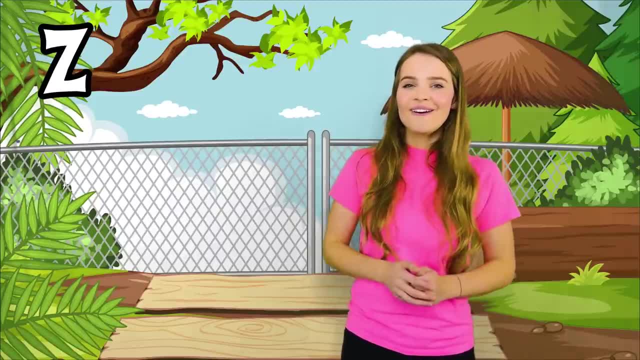 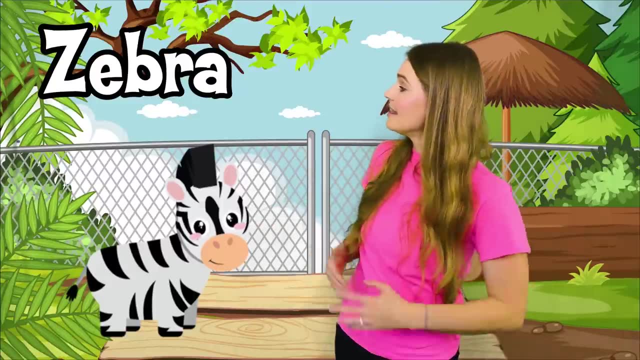 It makes the Z Z, Z sound for zebra. Hi zebra, I really like your black and white stripes. That's really pretty. Zebra says thank you. thank you, Zebra, it's very nice to meet you. 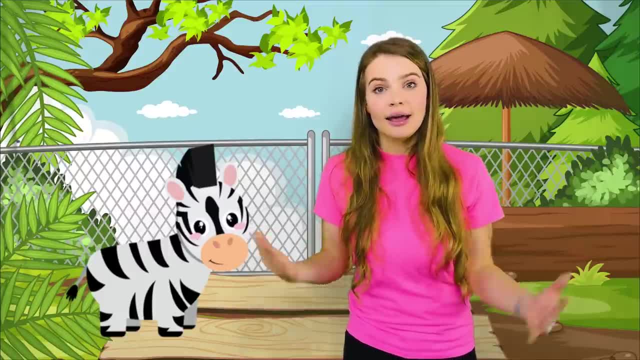 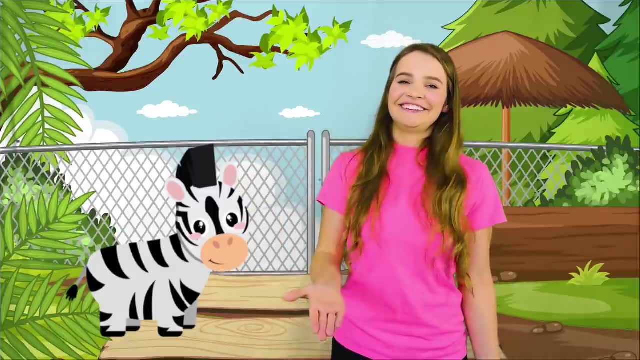 We've met so many animals at the zoo today. huh, It's been really adventurous. Thank you so much for helping me find these animals and all of the letters. Thank you, I'm lucky. Whoa, Is that a zebra? 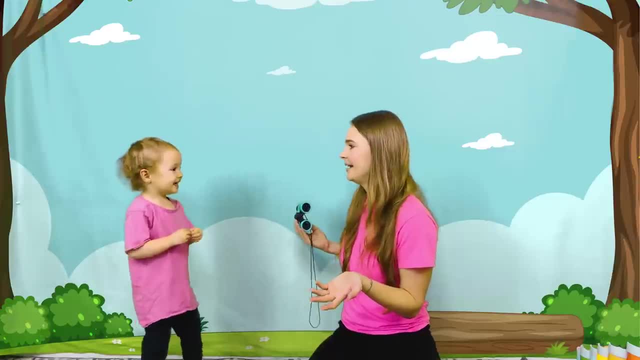 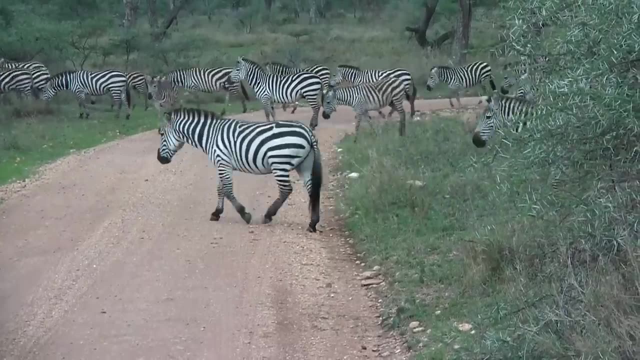 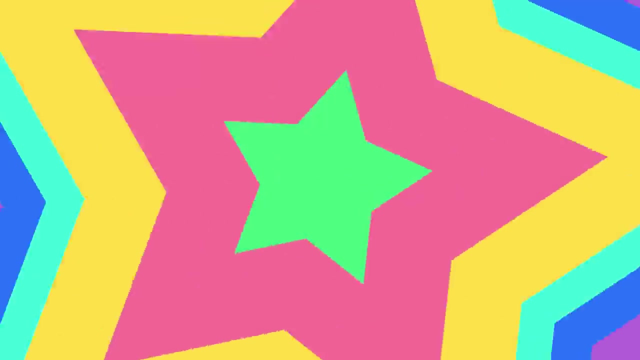 Zebra. What colors you got. What color is zebra? White and black, White and black. It's kind of got stripes. huh, Will you help me with this puzzle? I've got to help these animals get back in their spots. 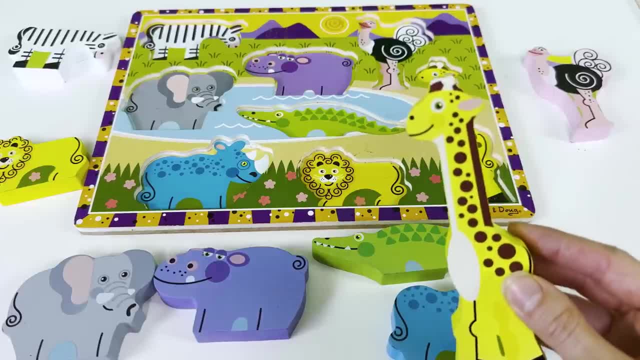 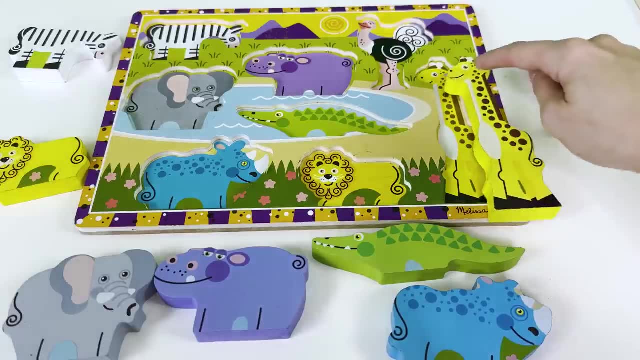 Hello, I'm a giraffe. Have you seen my spot? Hmm, do you see it on the board? Oh yeah, right here I put them in. I'll match the head to the head and the feet to the feet. 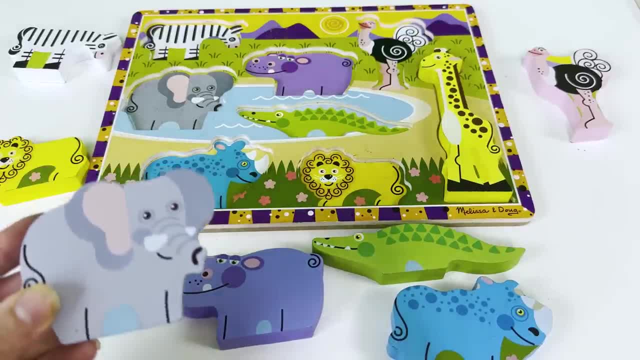 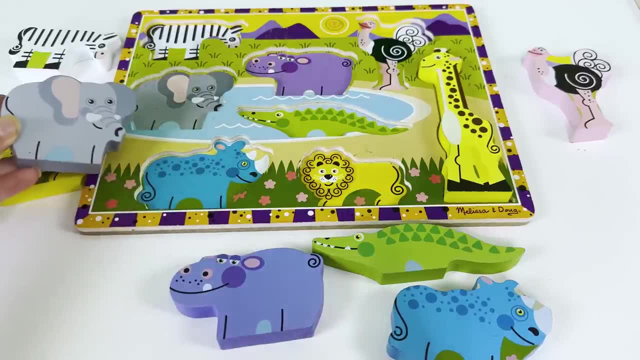 There you go, giraffe, Stomp, stomp, stomp. Do you see my spot? Hmm, let's take a look at the board. This is a rhino. Oh yeah, right here, Gently, gently, put them in. 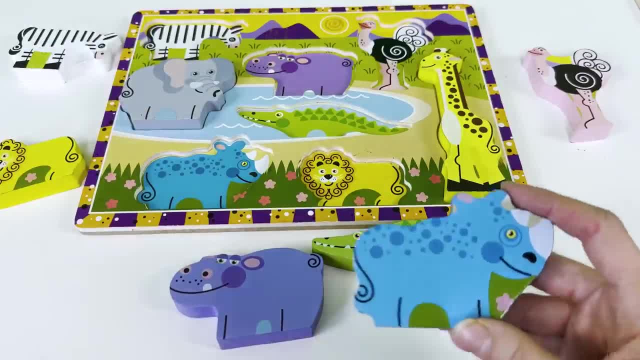 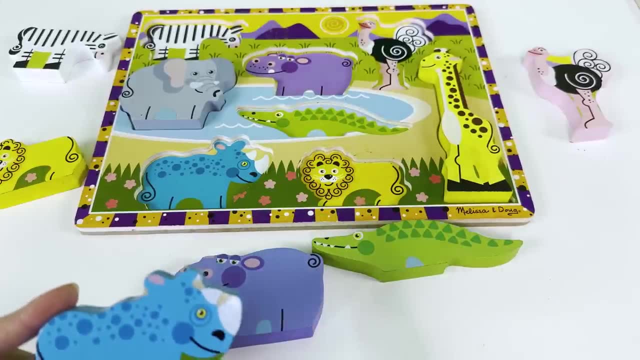 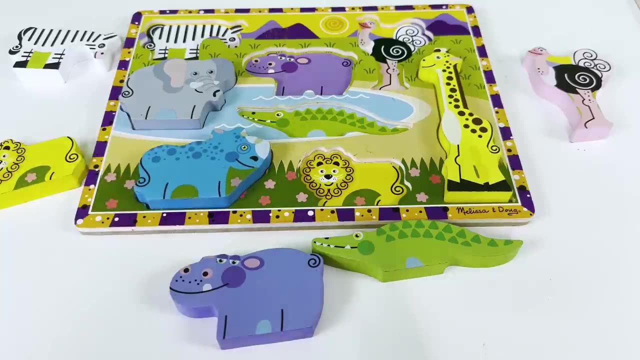 All right, Hello, says the rhino. Do you see my spot? Hmm, I'm looking for a blue spot with the rhino. Oh yeah, right here, I'll put the horns to the horns. There you go. Oh, I'm also looking for my spot. 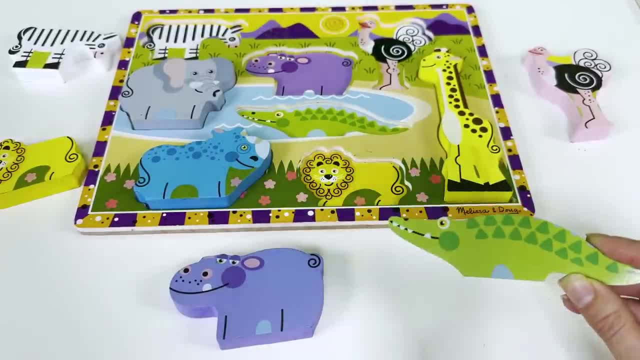 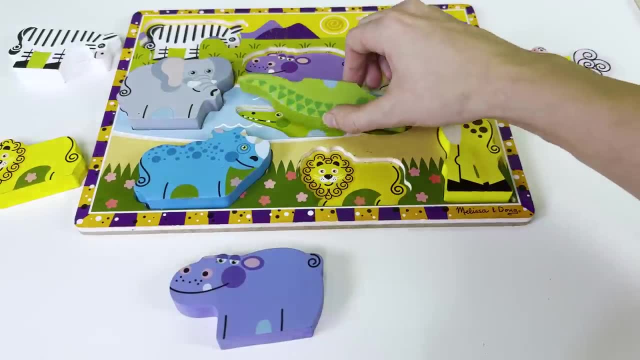 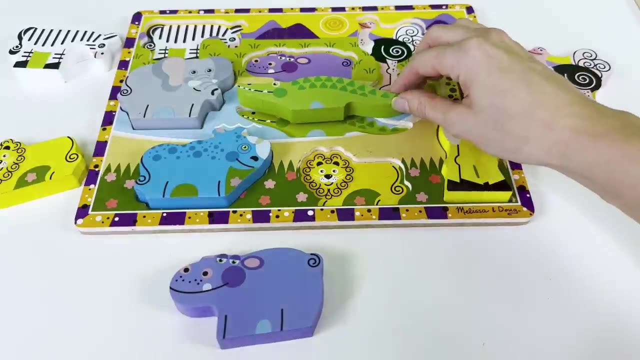 Maybe somewhere in the water. Let's see if there's any water we can find. Oh, yeah, right here. Hmm, That doesn't look right. Oh, maybe if I turn it I'll match the head to the head and the tail to the tail. 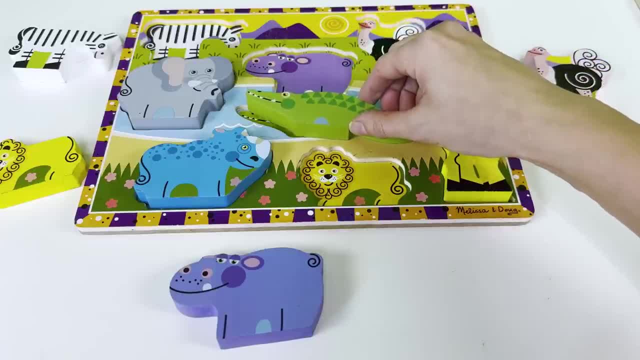 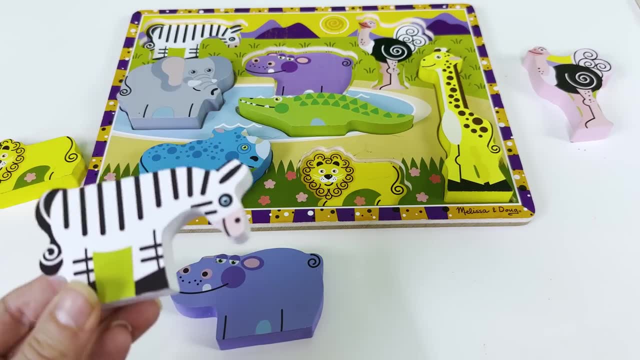 Not fitting. Let me do it slowly, slowly, Gently, gently, in All right, Hello, I'm a zebra and I'm looking for my spot. Let's see if we can help you find it. This is a lion. 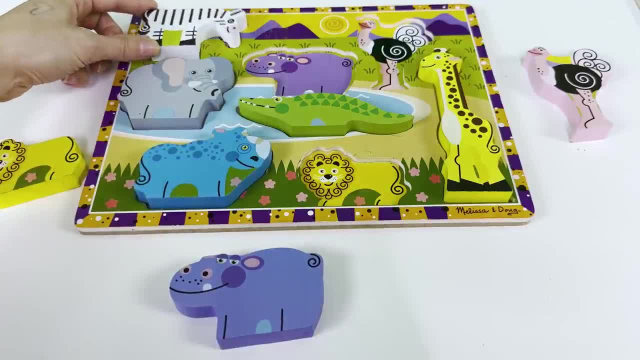 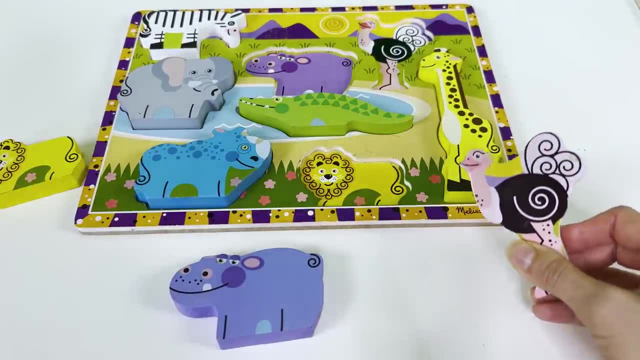 I see a black and white spot right here. Here you go, zebra. I'm an ostrich. Do you see my spot anywhere on the puzzle board? Let's take a look. Oh, how about up here? All right, Thank you. 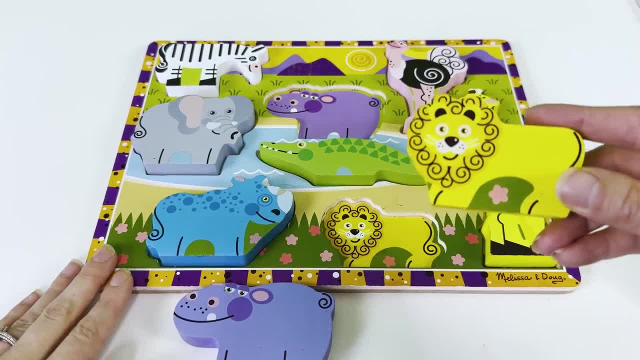 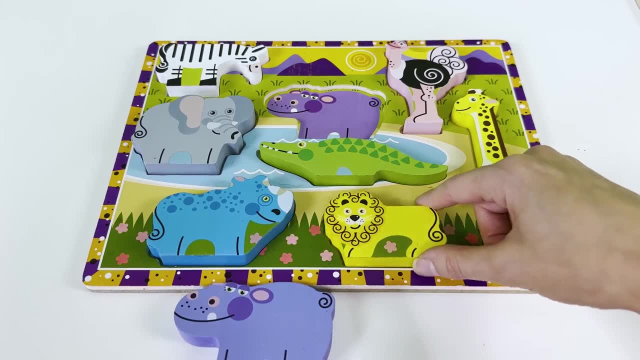 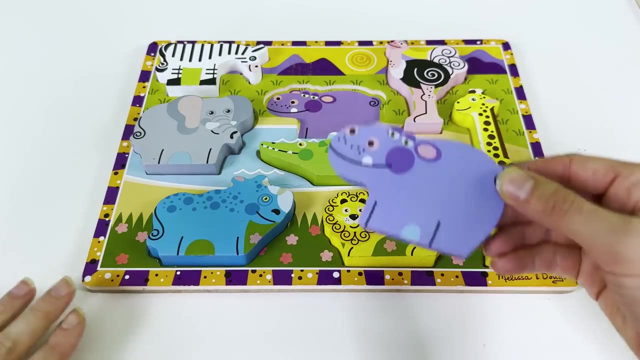 Roar. Have you seen my spot of a lion? Hmm, Oh yeah, right here by the flowers, Here you go, lion. I'm also looking for a spot. Hmm, I've got this one spot left right here. Here you go, hippo. 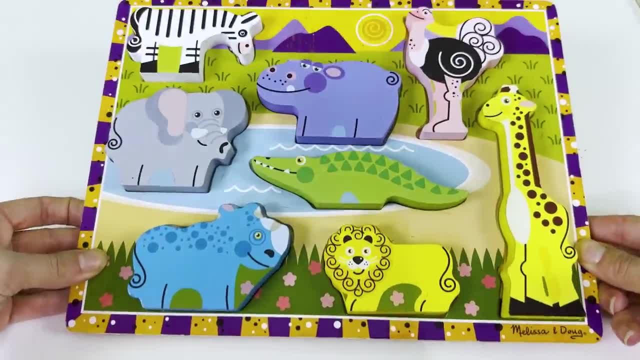 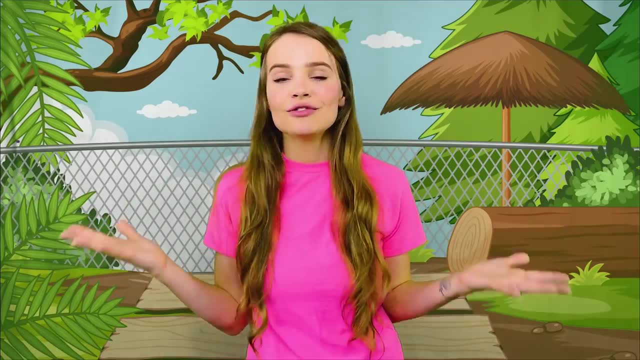 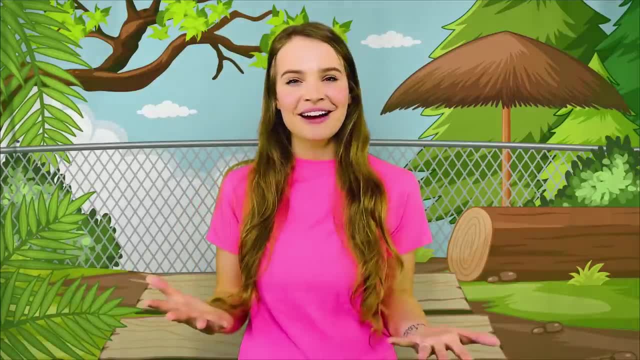 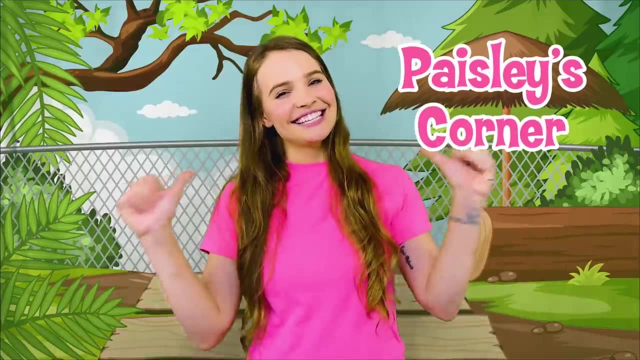 I love playing with you. You're such a great friend and I'm really proud of you. Well, that's the end of this video, But if you're looking for more of our videos, make sure you search for Paisley's Corner with Silly Miss Lily. 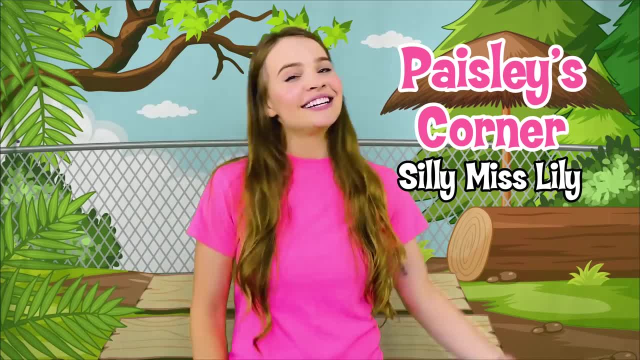 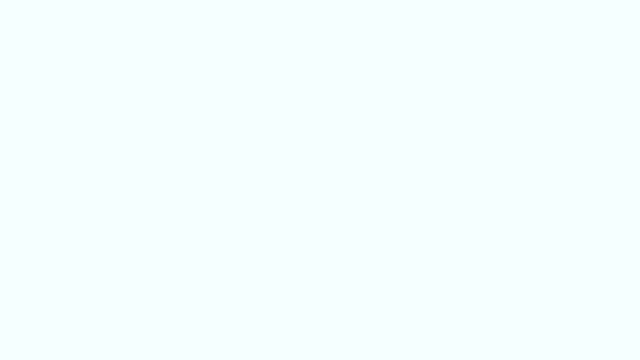 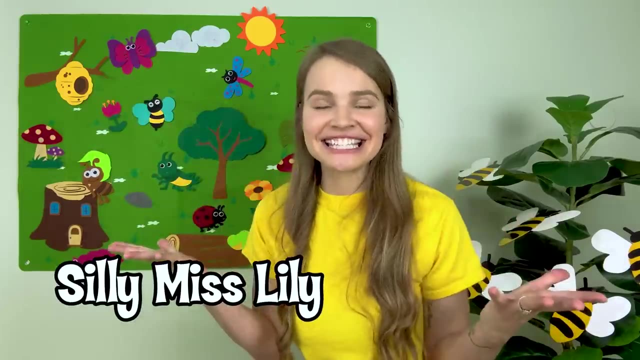 And I'll see you then. Bye-bye, Bye-bye, Hi friends. It's me Silly, Miss Lily, and I'm so excited to play with you today. Today, we're going to talk about insects, or bugs. 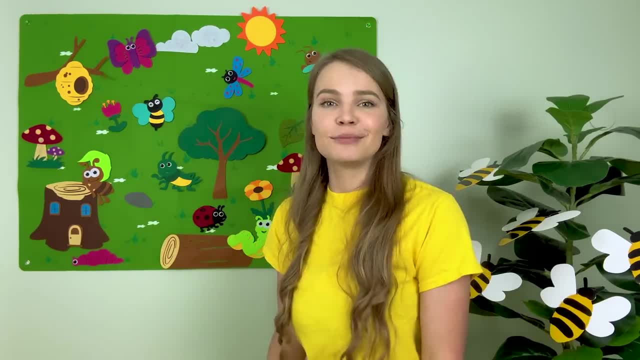 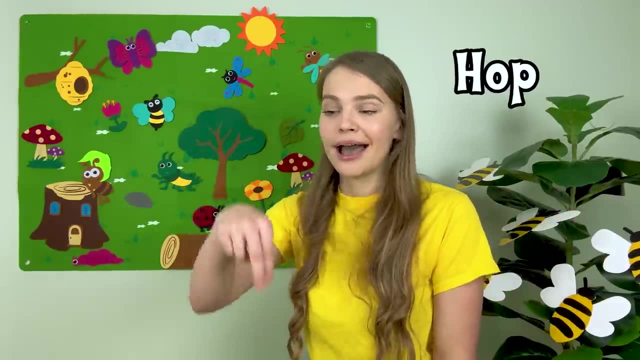 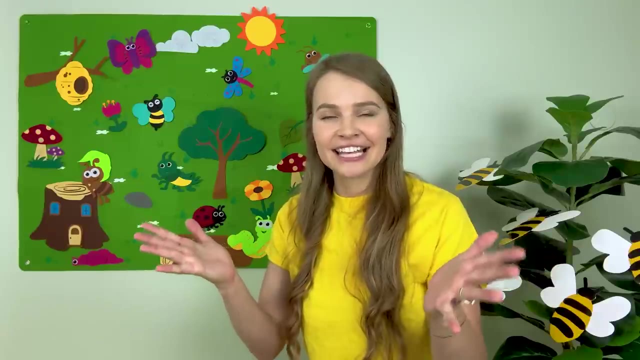 And there are so many different kinds of bugs. There's bugs who can fly, There's bugs who crawl And there's bugs who like to hop, hop, hop, hop, hop around. I'm so excited. Sometimes, when I'm excited, I like to clap my hands. 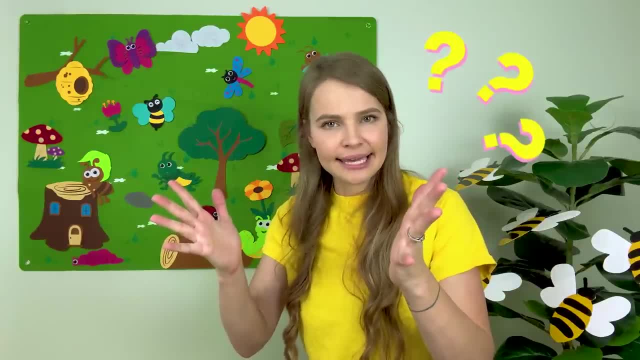 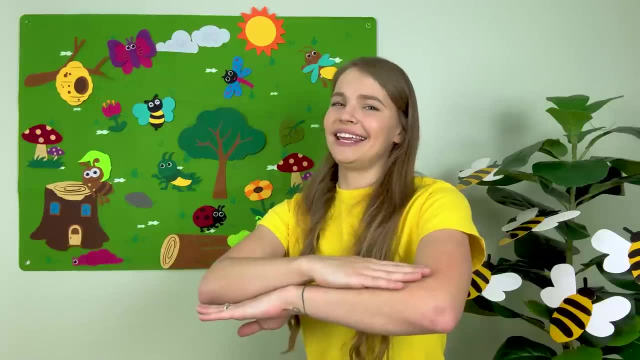 Wait a minute. How do I clap my hands? Was it like this? That doesn't seem right. Like this, That's not right either. Oh, with my hands And I put them together. That's right, This is clapping. 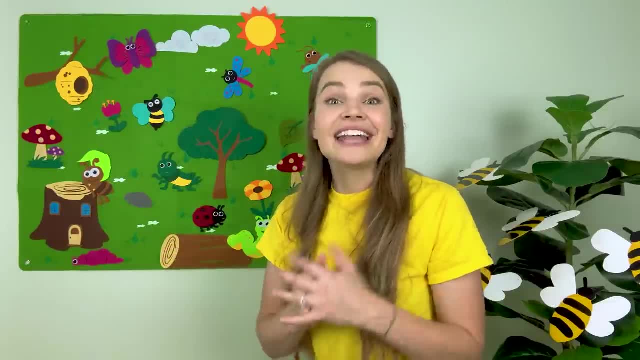 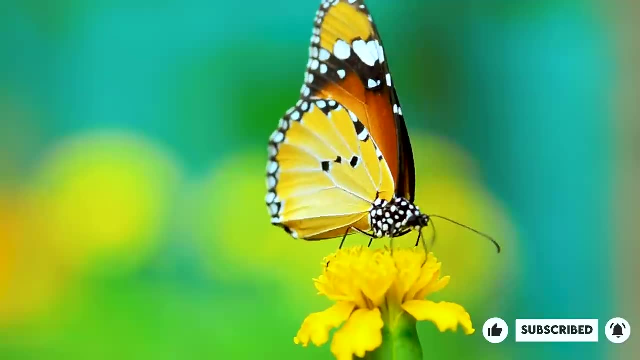 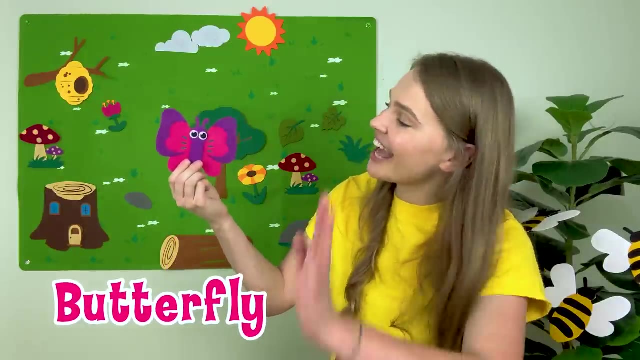 Thank you for teaching me. You're a great helper. Now let's learn about some bugs together. Come on, Oh look, Fly, fly, fly. Here comes a butterfly, Hello butterfly, Hello friend, says the butterfly. 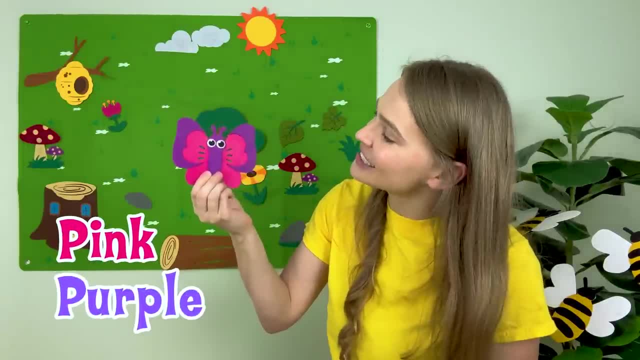 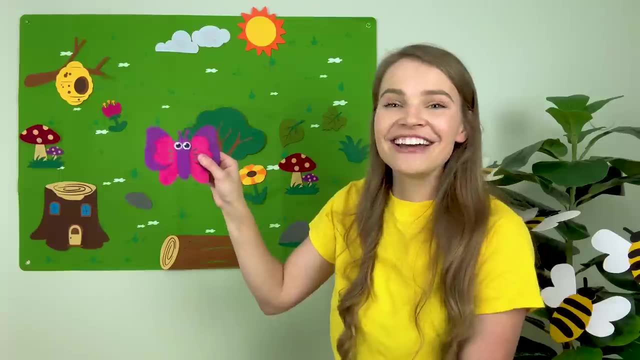 Butterfly, I like your pink and purple wings. Oh, thank you so very much, says butterfly. I'm just flying around. We'll go, fly, fly and have fun. butterfly, Here you go. Do you want to fly around like a butterfly with me? 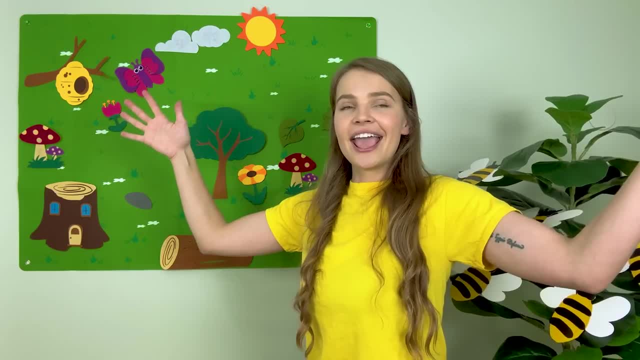 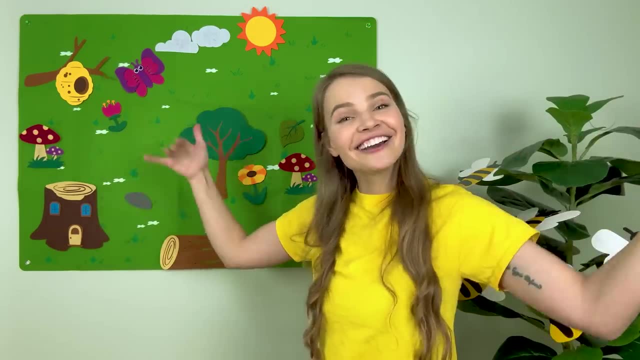 Okay, let's get our wings out And we'll fly, And we'll wave our arms around. Ready Wave, wave, Flying, flying. Wow, you make a great butterfly, Great job. Here's a fun little caterpillar activity you can play at home. 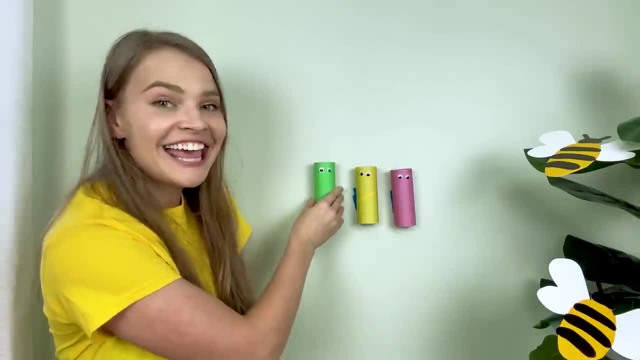 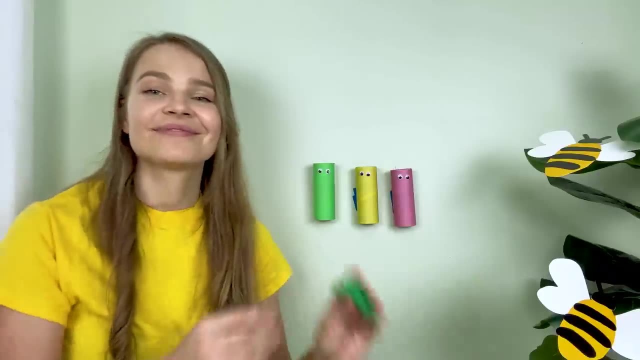 You just need a cardboard tube and you can tape it to the wall and then help feed the caterpillars. You can use little cutout shapes for leaves, or I've got some of these leaves. Will you help me put them in? 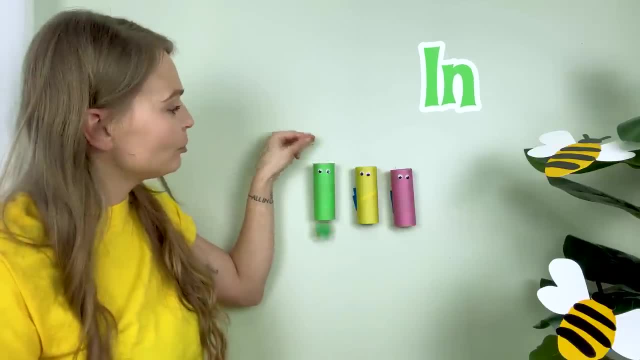 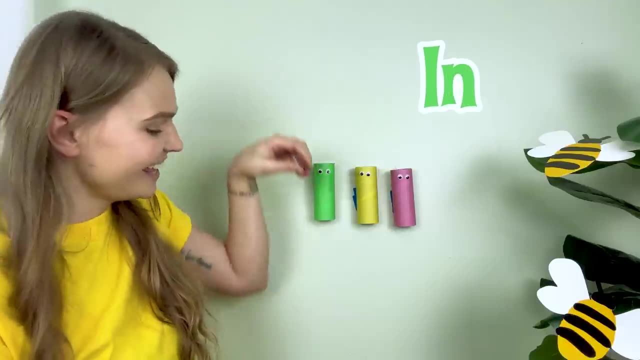 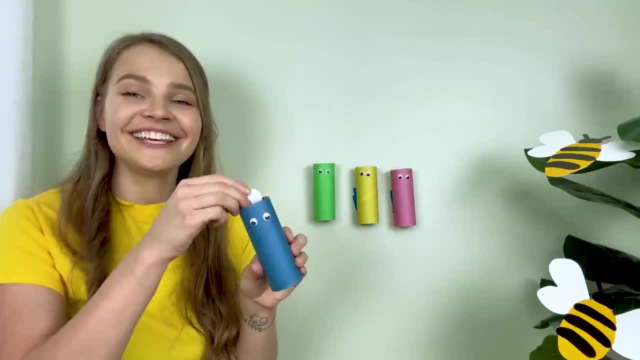 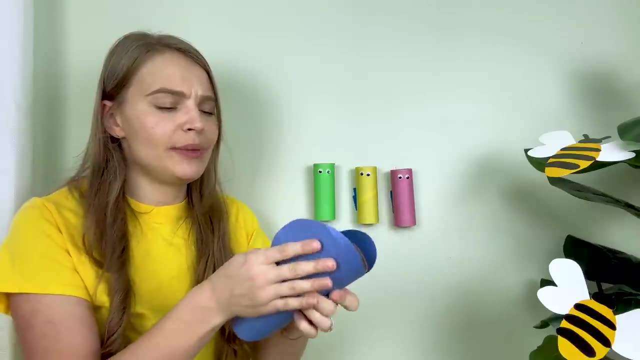 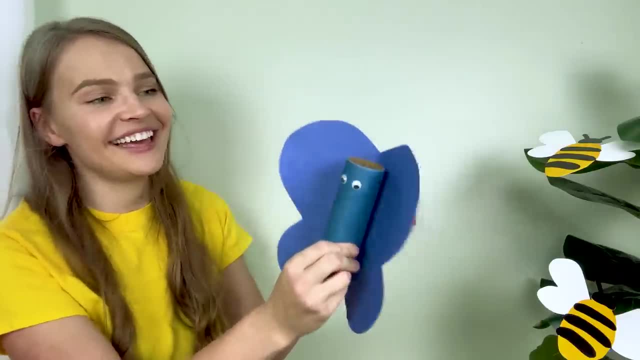 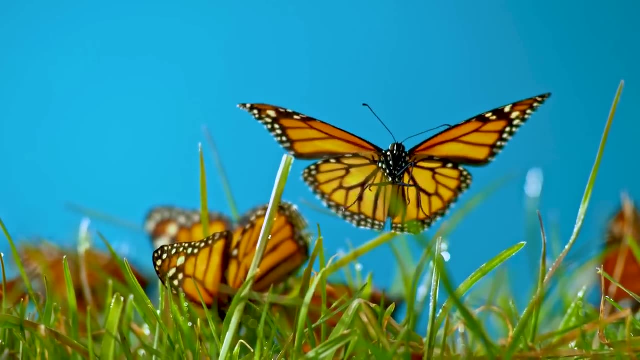 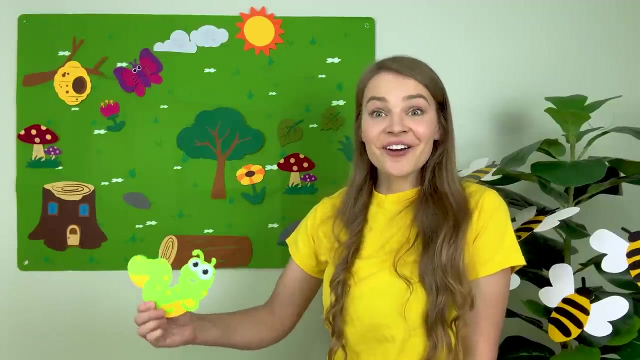 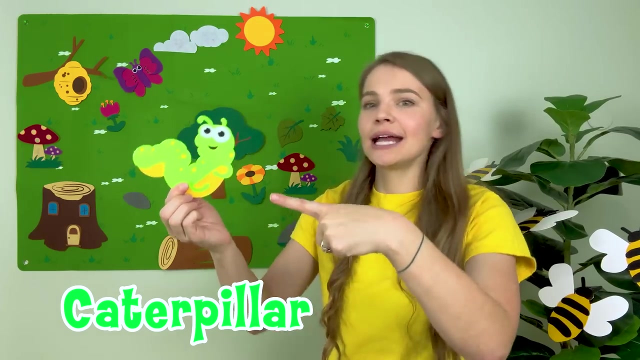 and go flying, flying, flying, flying, flying, flying, flying. They fly off and they fly away. They fly off and they fly away. Caterpillar, how are you Craw crawl? Oh look, it's a caterpillar. 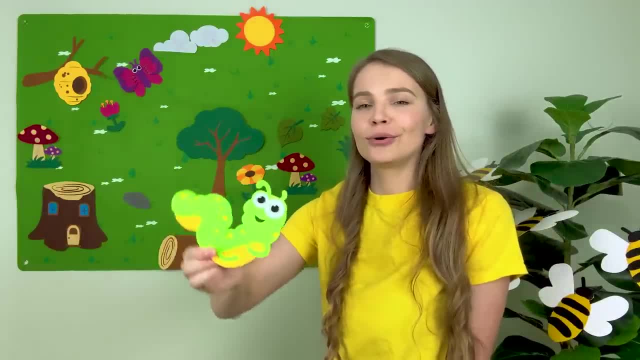 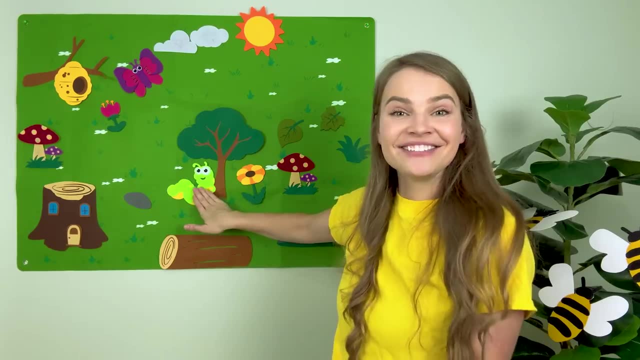 Caterpillar- caterpillar, That's a fun word. Hi, Caterpillar, How are you? Hello friends, Craw crawl, crawl. Here you go, little caterpillar friend, You can walk around in a little cocoon, the tree. Go find some leaves and branches. 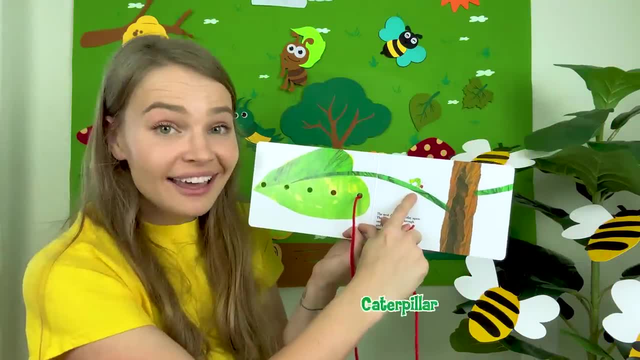 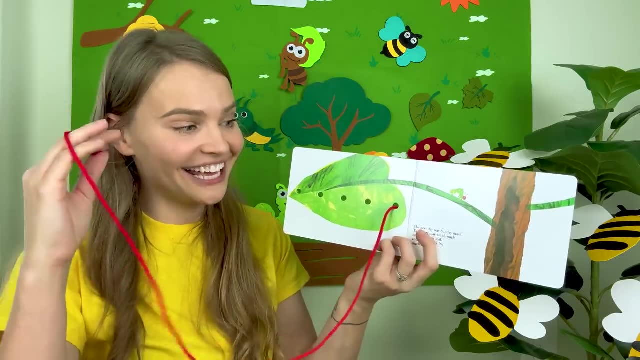 Crawl, crawl, crawl, crawl, crawl. This little caterpillar wants to get through the leaf but can't find his way. I thought we could help him. I grabbed a little red shoelace that we could poke through the holes and thread it through to help the 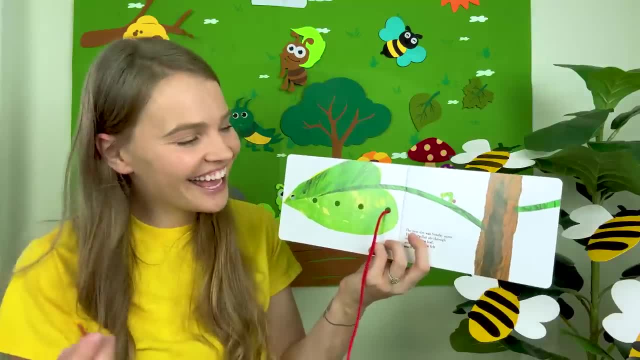 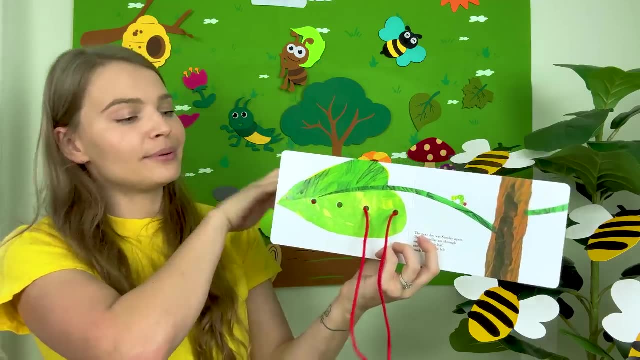 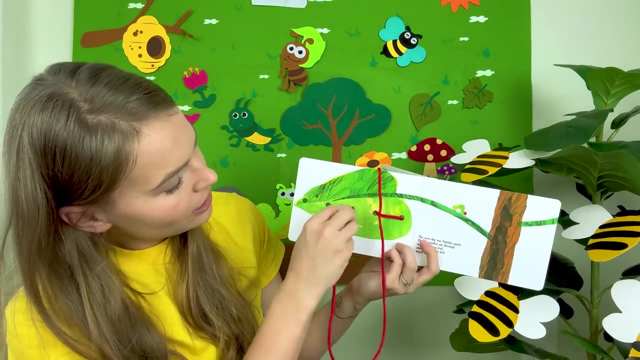 caterpillar find his way. Will you help me? All right, We'll put the shoelace part in and pull it out. All right, caterpillar, now you can go this way. You can also go around the leaf and go in here and pull. 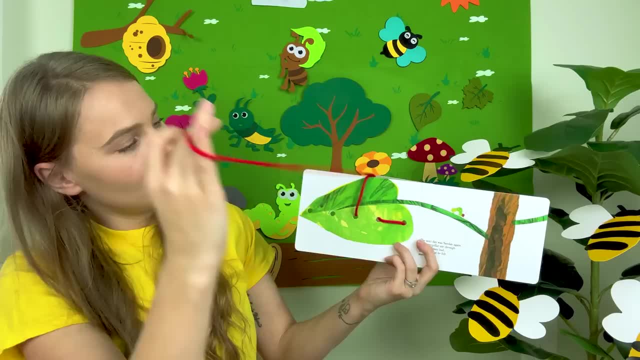 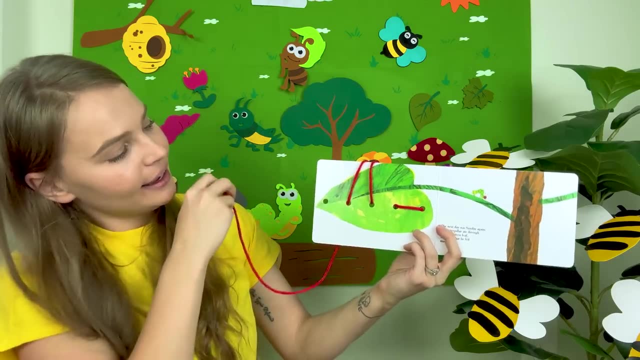 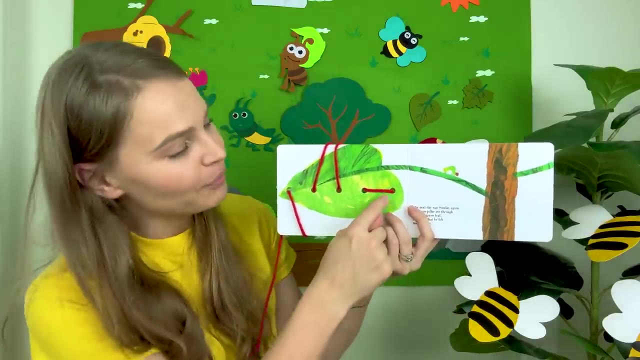 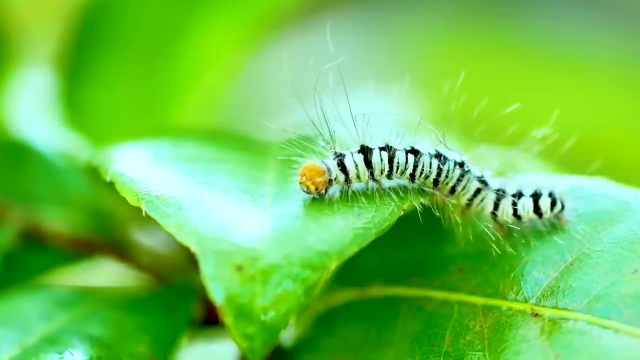 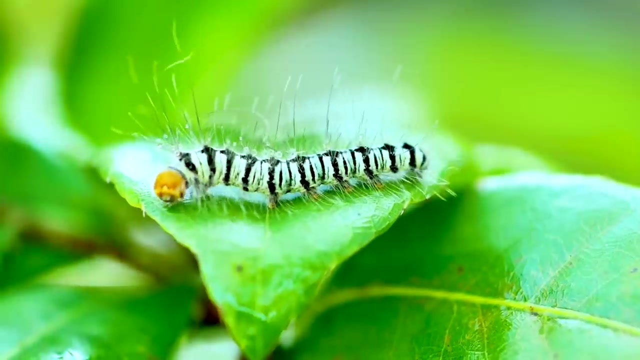 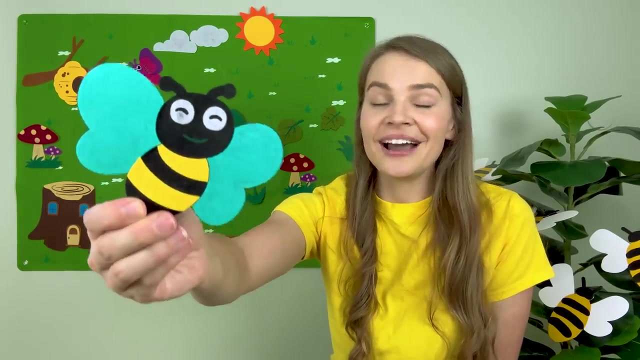 it through and over and in. and let's put it in again: Wow, Look at all the different ways that the caterpillar can go This way, or up, or even from below. Thank you so much for helping me. Hello, Hello, little bumblebee. Hi, Hello friend, I'm a little bumblebee. 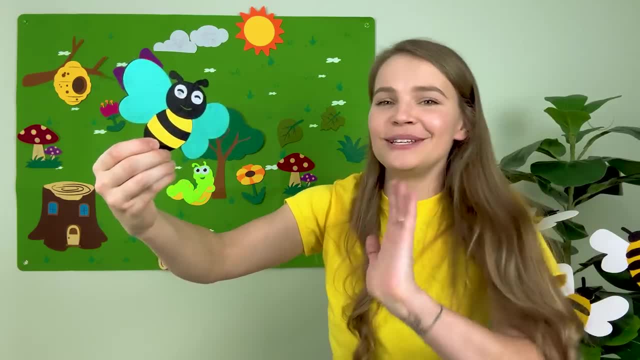 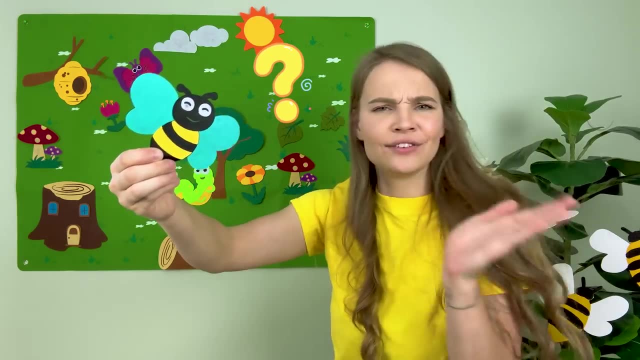 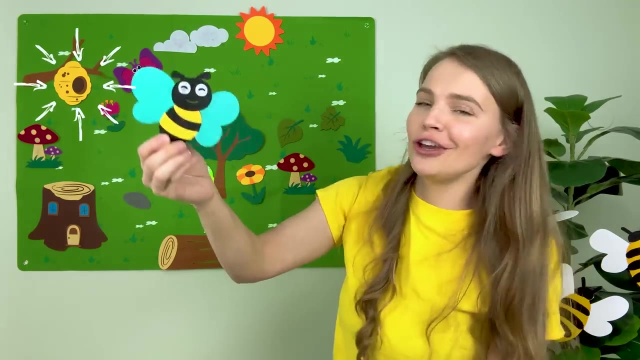 I have yellow and black stripes. Oh, so nice to meet you, bumblebee. Have you seen my beehive? Have you seen a beehive Where Over there? Oh, yeah, right there. Oh, thank you so much, friend, Thank you. 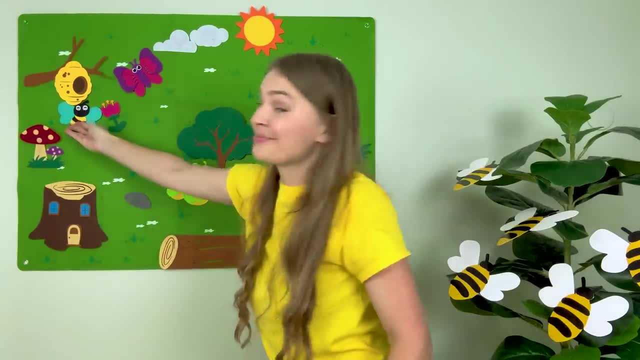 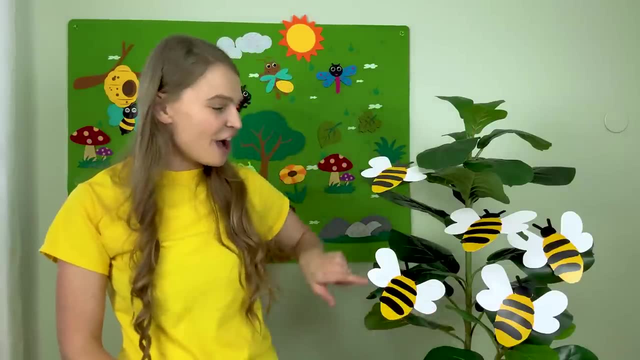 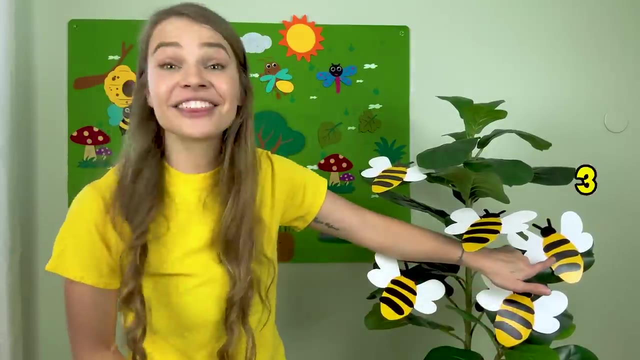 Thank you. Thank you, Wow, great job helping the bumblebee. Will you help me count the bumblebees? All right, One bumblebee, Two bumblebees, Three bumblebees, Four bumblebees. 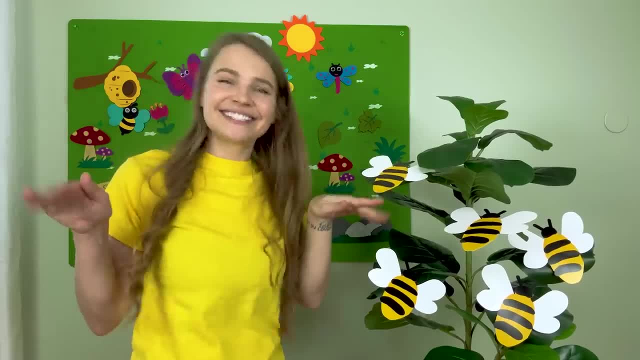 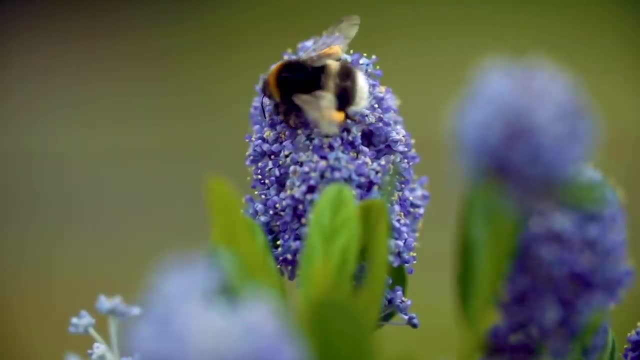 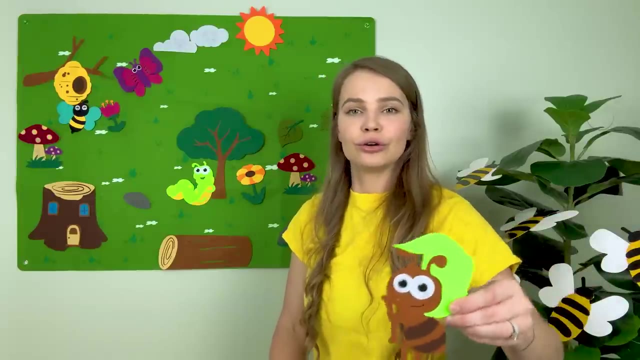 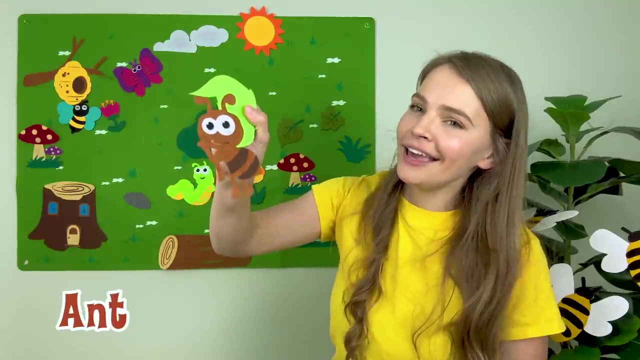 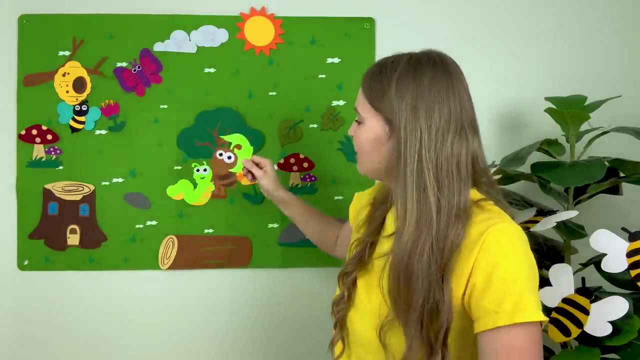 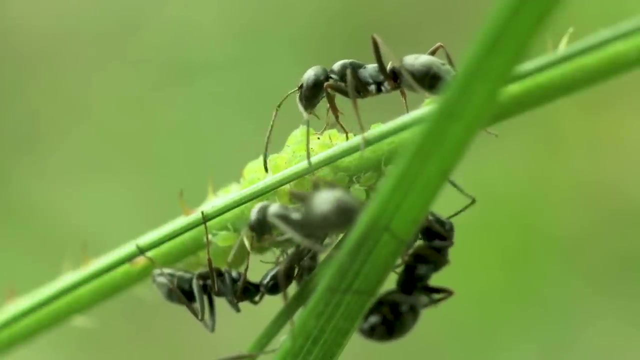 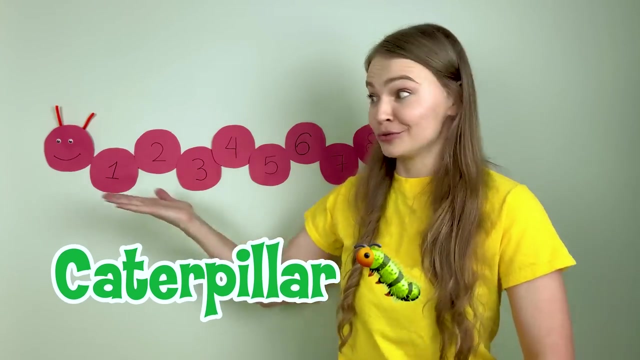 Five bumblebees Marching, Marching. Here we go Marching, Marching, stand slow. hello hi everybody. i'm an ant. i can go marching, marching into my ant home. hello, little ant, nice to meet you. oh wow, look at this caterpillar. it's really long and it's made out of circles. 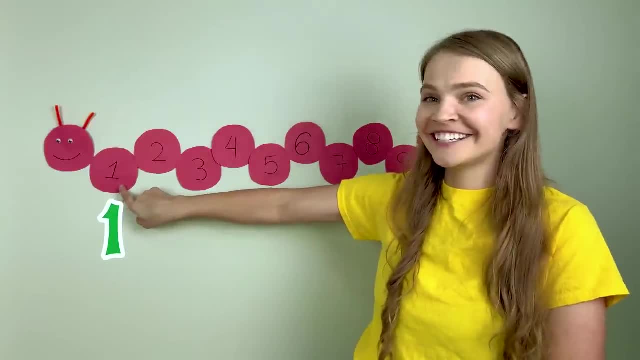 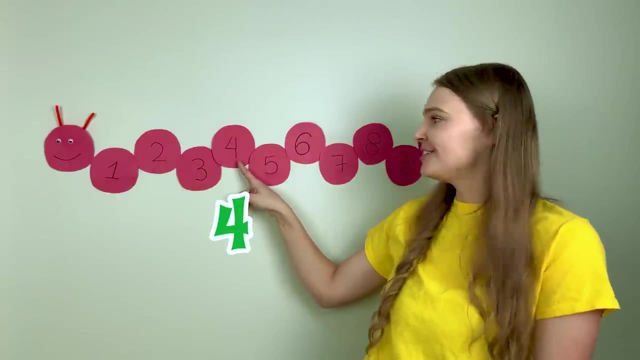 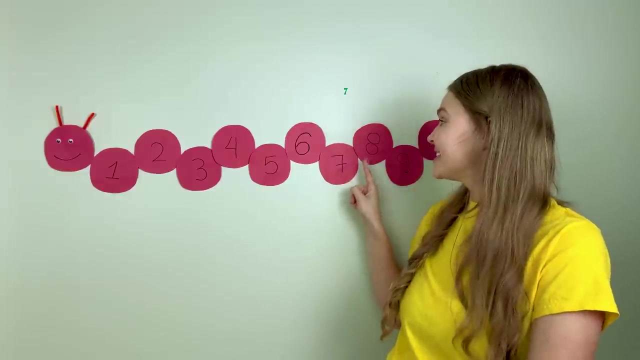 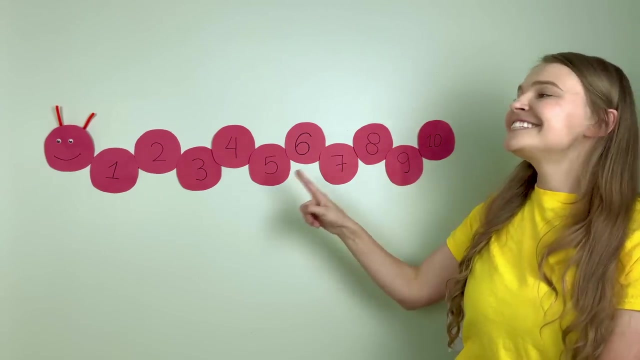 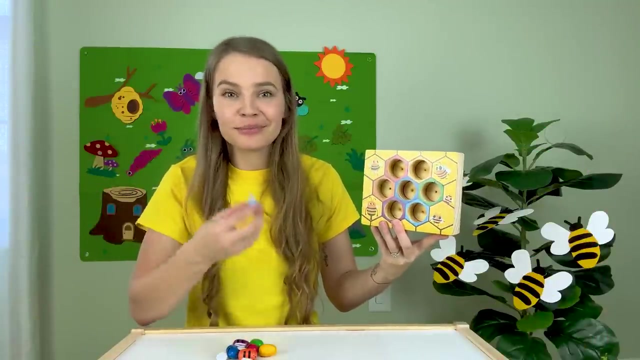 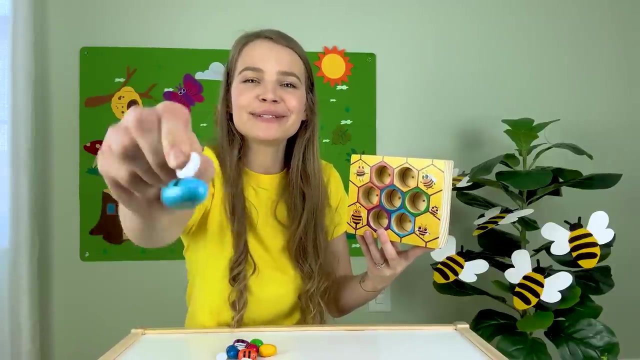 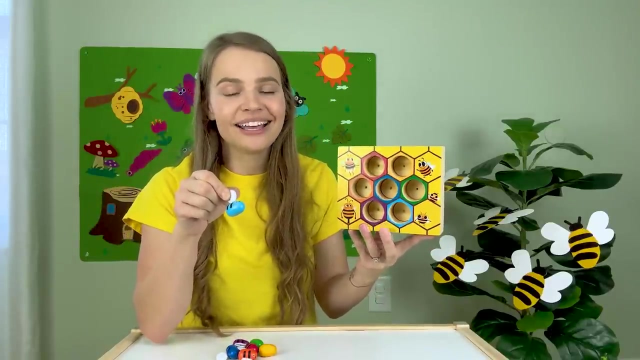 let's count the circles: one circle, two circles, three circles, four circles, five circles, six circles, seven circles, eight circles, nine circles, ten circles, ten circles. thank you for counting all right, i've got a little light blue bumblebee. hello, hello, friend. hello, hello, hello. do you see a light blue spot in the beehive? hmm, oh yeah, right here. thank you. 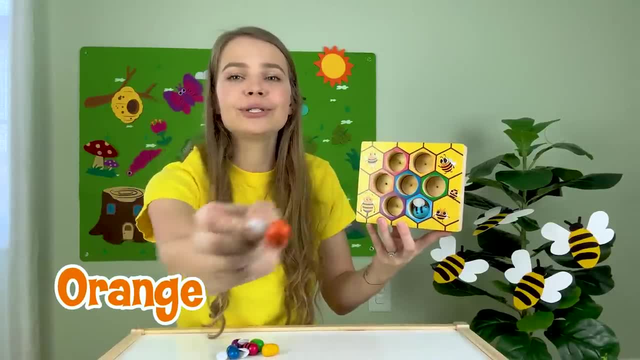 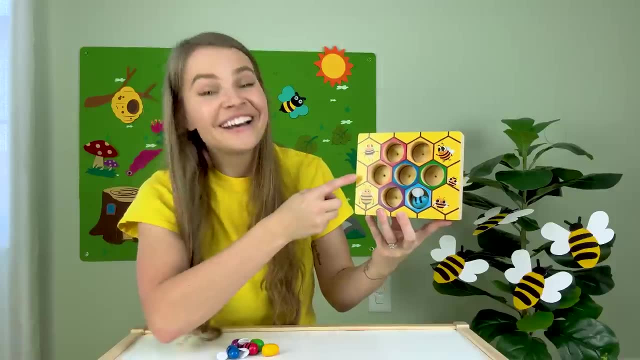 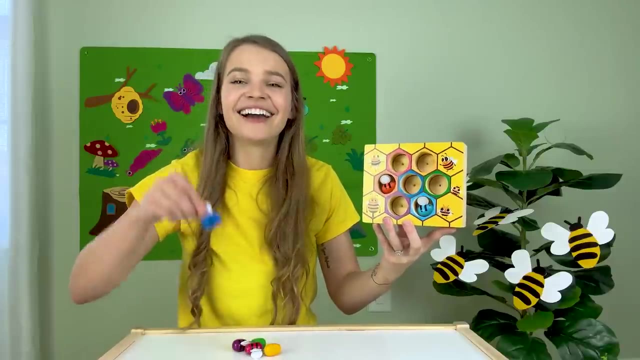 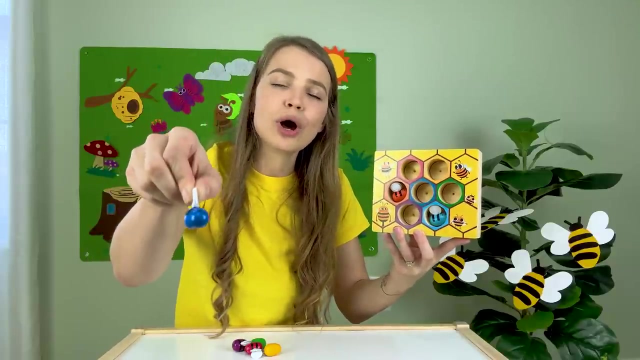 now i've got a little orange bumblebee. hello friend, do you see a little orange spot i can go into? hmm, right here, thank you. here we go. now i've got a little blue bumblebee. do you see a dark blue spot in the beehive? hmm, oh yeah, right here in the middle. oh, thank you, thank. 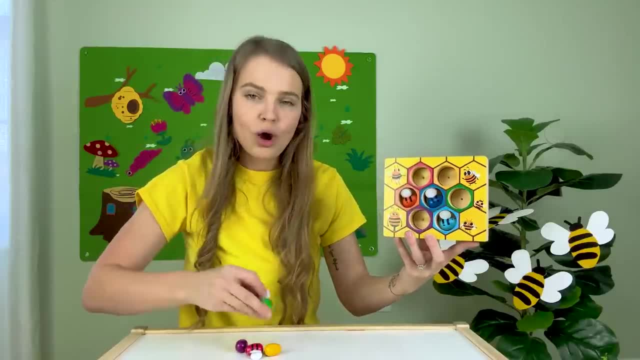 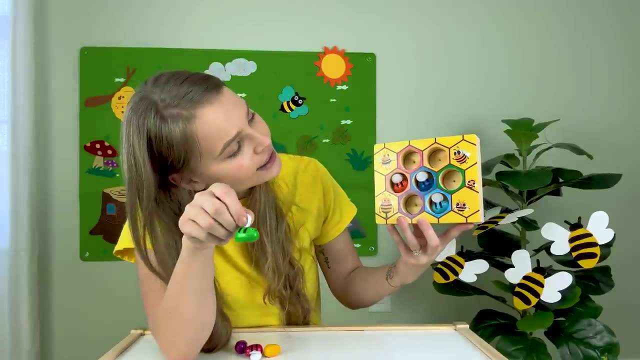 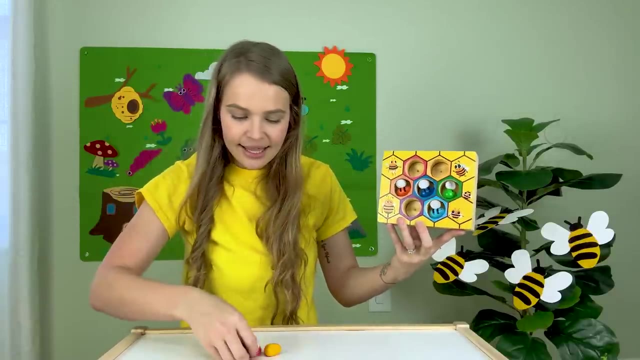 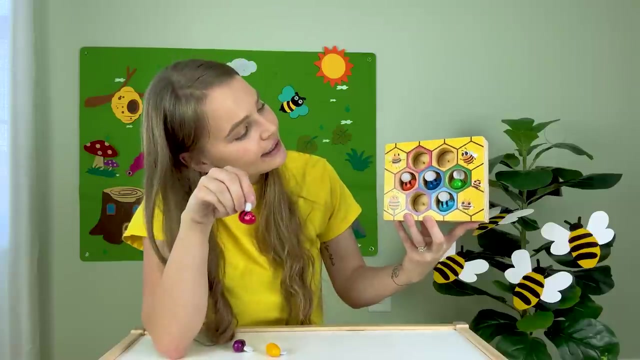 you. oh, hello, hello, hello. i'm a green bumblebee. is there a green spot in the beehive? hmm, let's take a look. hmm, oh, how about? right here? that's right, here we go. i'm a red bumblebee. hello, hello, hello. is there a red spot? let's take a look. oh, right here. thank you. 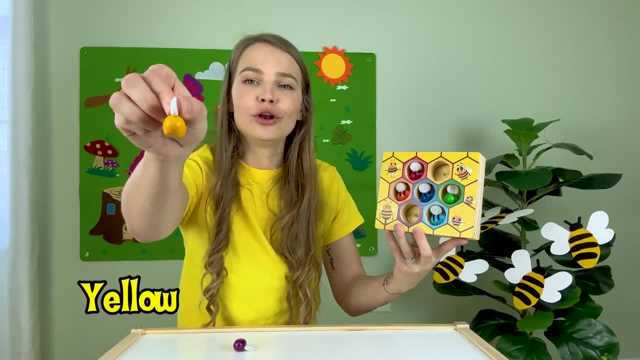 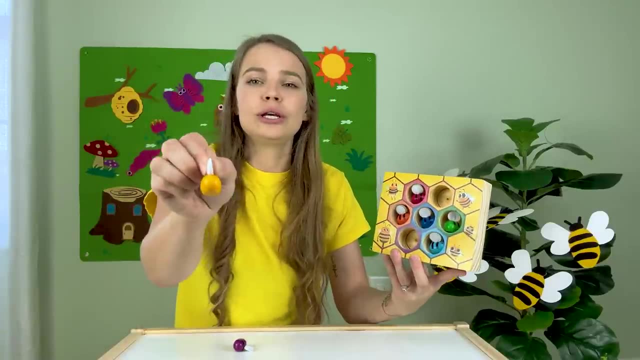 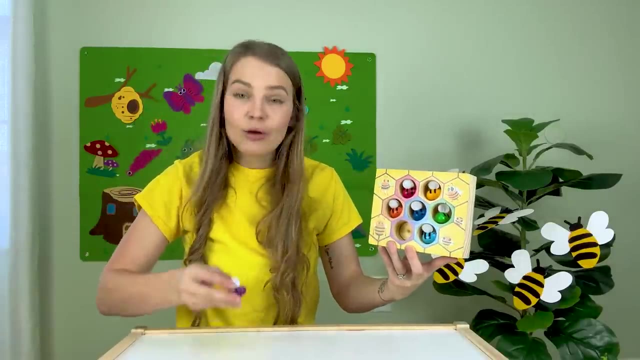 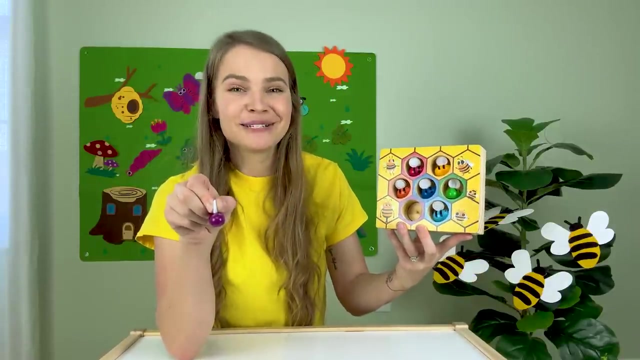 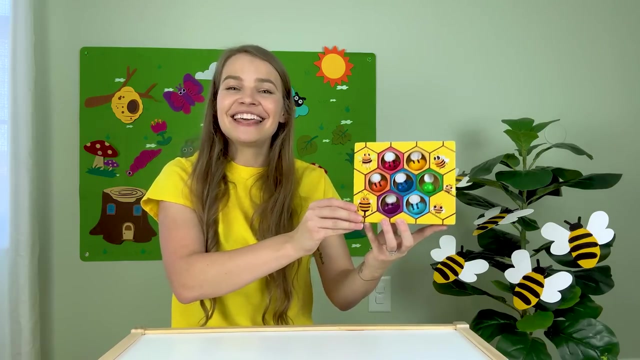 in. oh, my yellow bumblebee, hello, hello. do you see a little yellow spot for me? hmm, right here. thank you, i'm a little purple bumblebee and i'm looking for a purple spot. hmm, do you see the purple spot? yeah, we've got one left and it's problems. right here. here you go, bumblebee. wow, thanks for helping all. 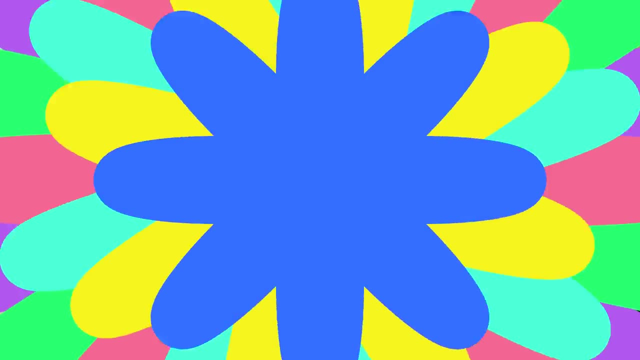 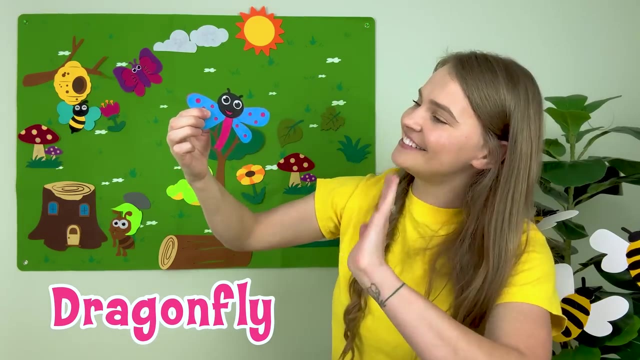 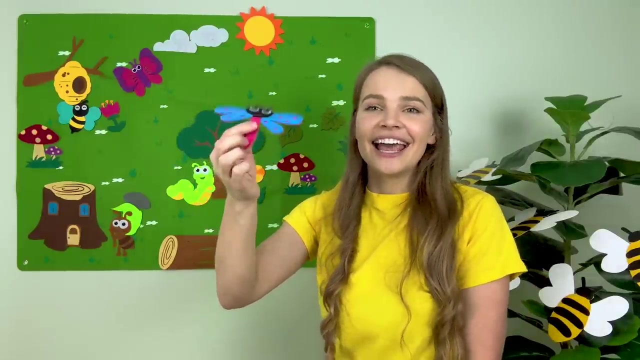 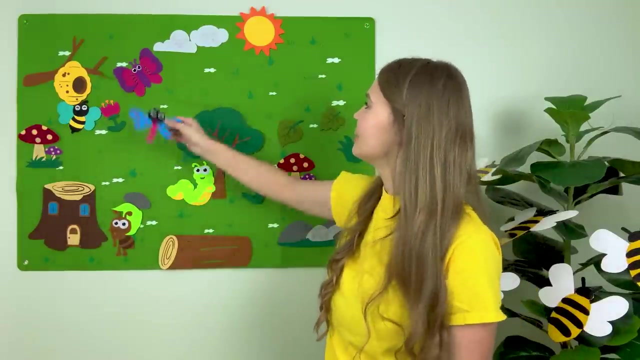 of the bees find their spots. thank you, hmm, oh, look, it's a little dragonfly. hello, dragonfly, hello, friends. how are you today? we are doing so good. thank you for asking. hello, hello, hello. have you seen my other bug friends? we have it right there. oh, thank you for helping me in the right direction, thank you. 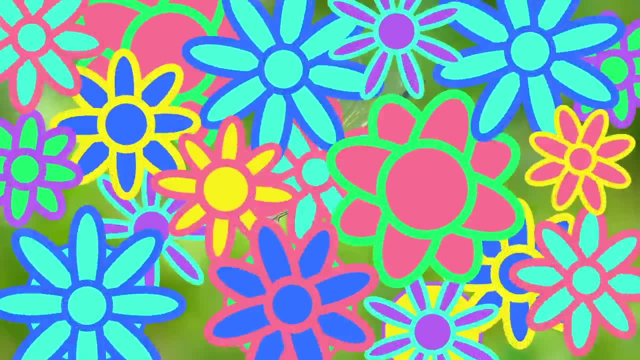 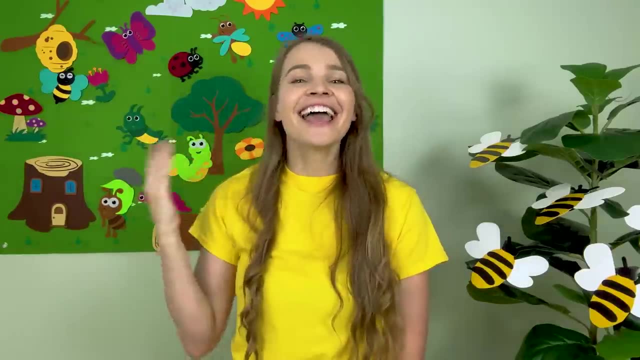 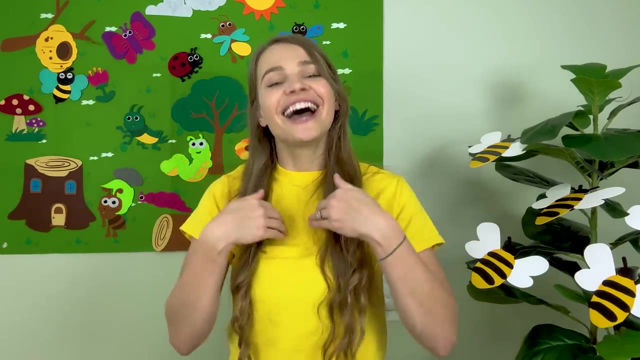 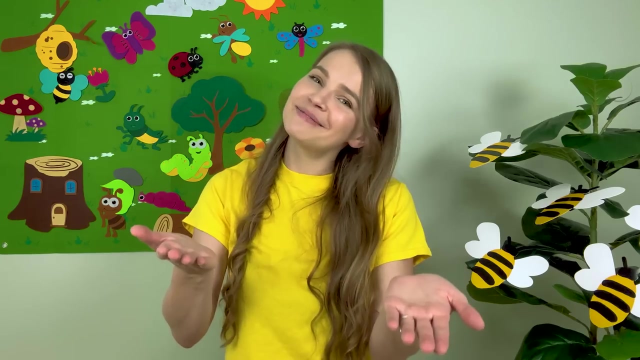 baby ocho. oh, oh, okay, please go réal, because don't be smart. ci hello, how are you hello? how are you hello? how are you? how are you this morning? i am fine, and i hope you are too. i am fine, and i hope you are too. i am fine, and i hope you are too. i hope you are too this morning. Oh, look, he's standing and he wants to get a hug. 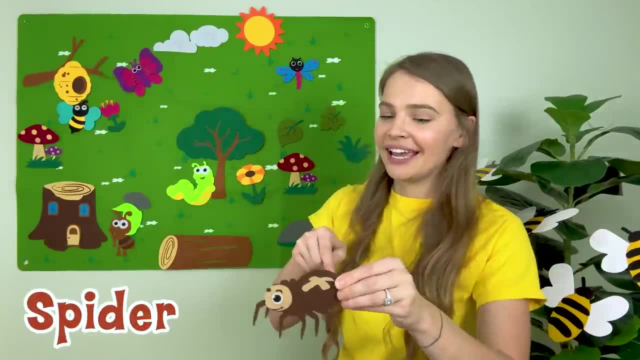 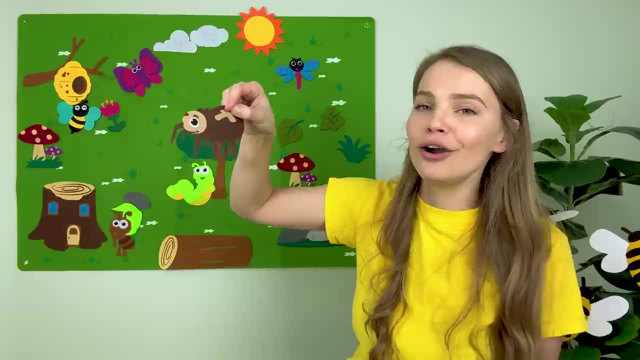 Do you see this bug right here? This is a spider Crawling, crawling, crawling. I'm a spider and I'm looking for my bug friends to say hello, Oh, hello, spider, Nice to meet you. Here's the rest of your bug friends. Here you go, Hello friends. 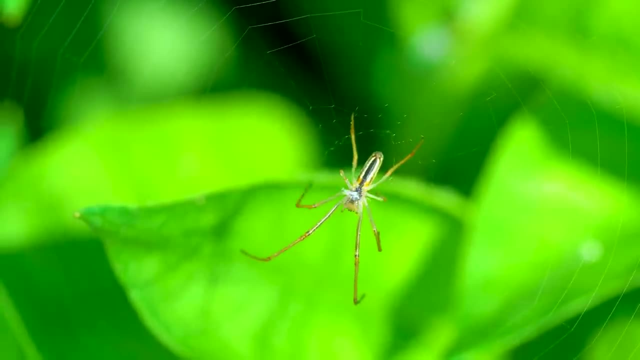 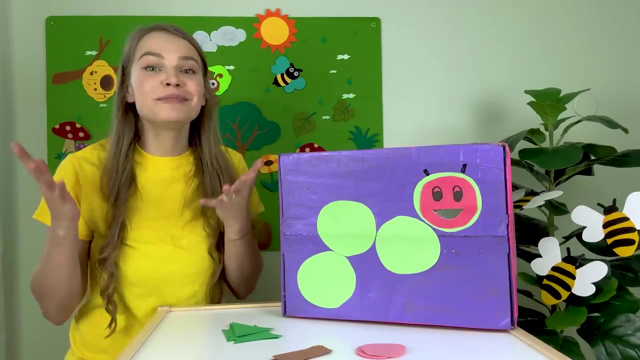 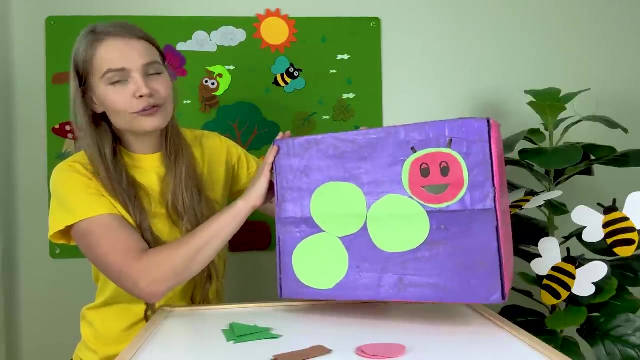 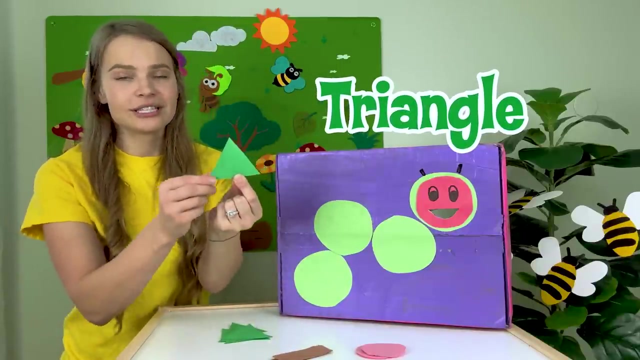 Will you help me feed the caterpillar? Oh, I'm very hungry and I would love to eat some leaves or flowers or branches, says the caterpillar. All right, Well, I've got some green triangles That could be a leaf. Oh, yeah, I would like that. Here you go. Yum, yum, yum, yum. 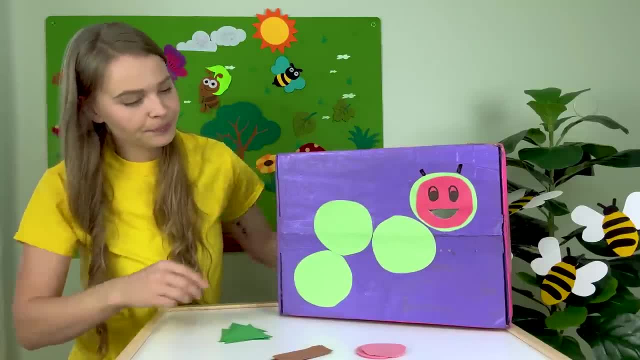 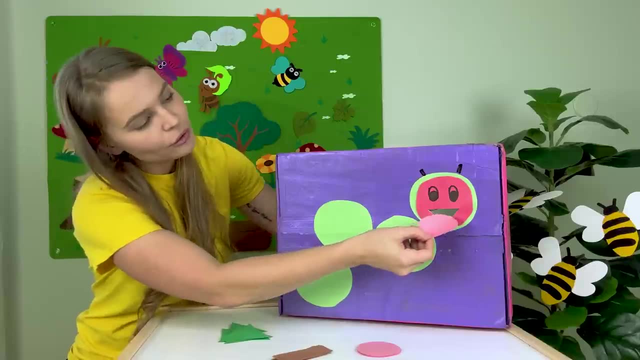 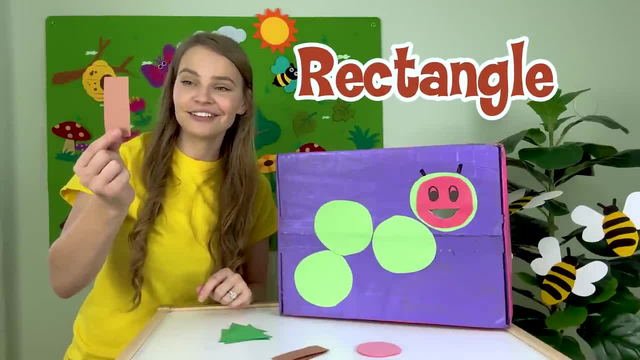 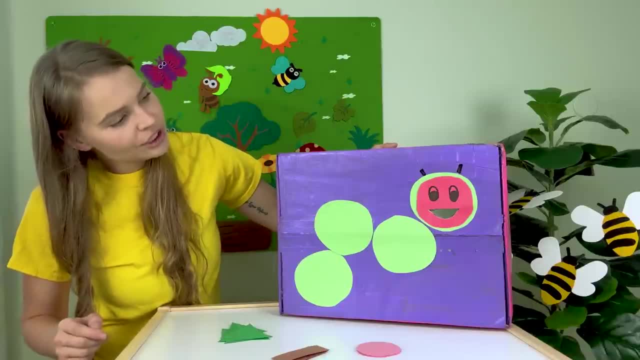 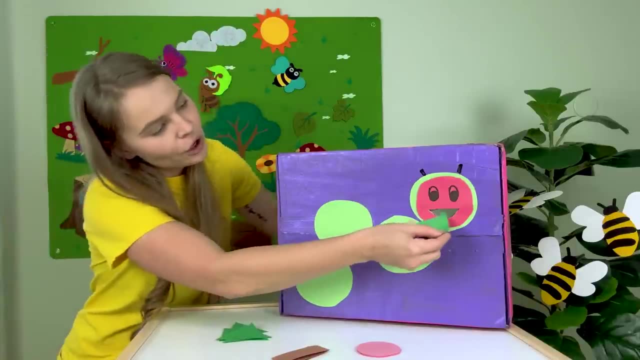 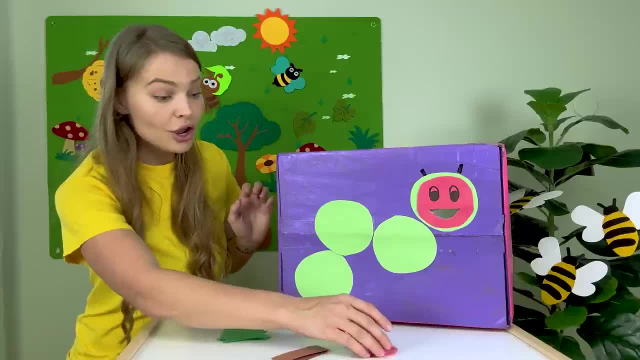 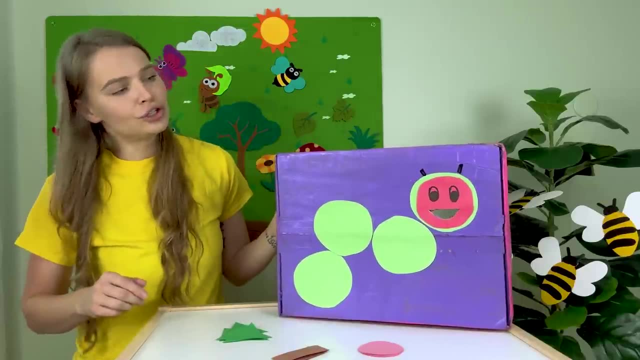 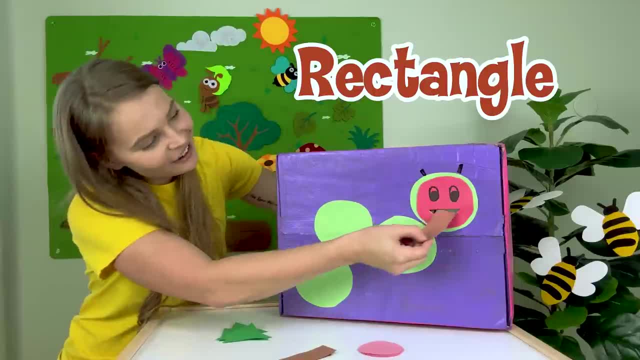 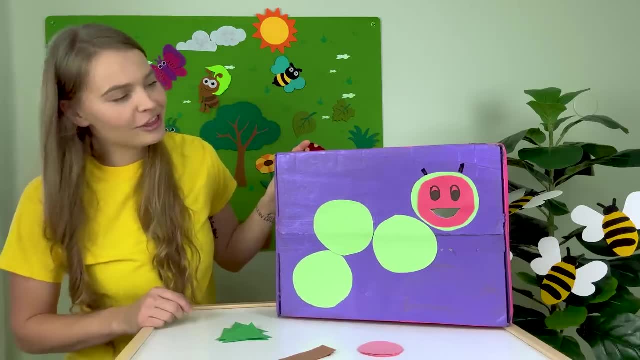 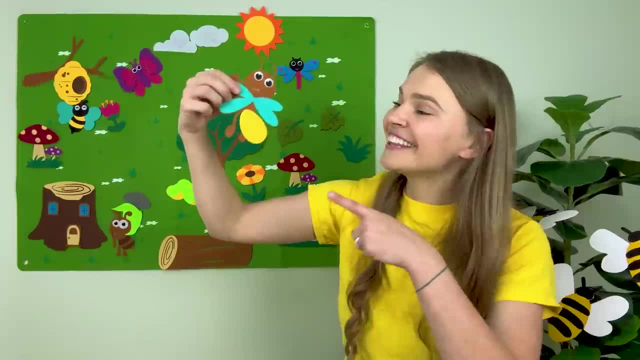 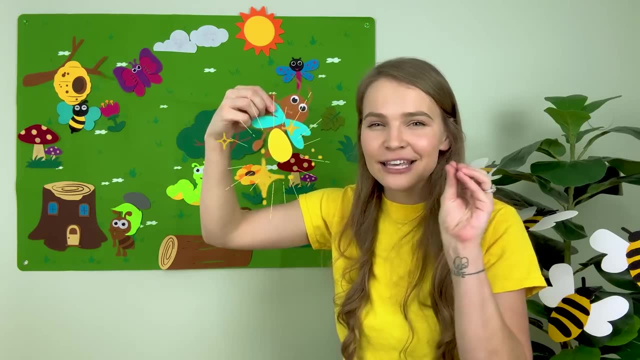 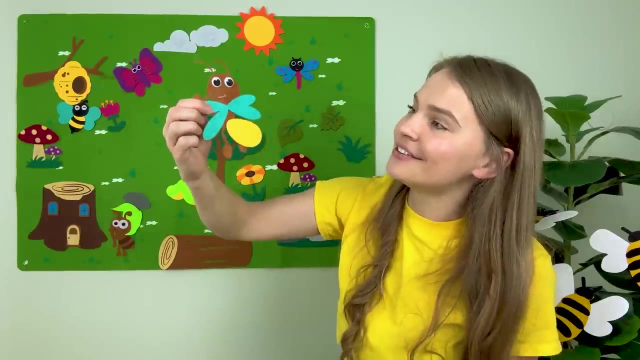 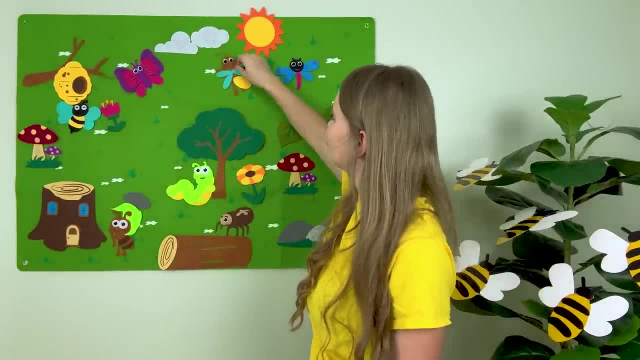 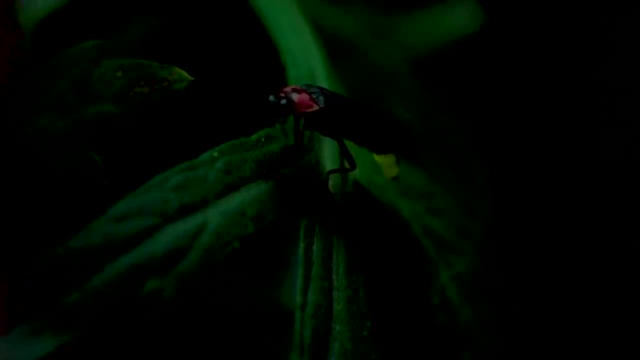 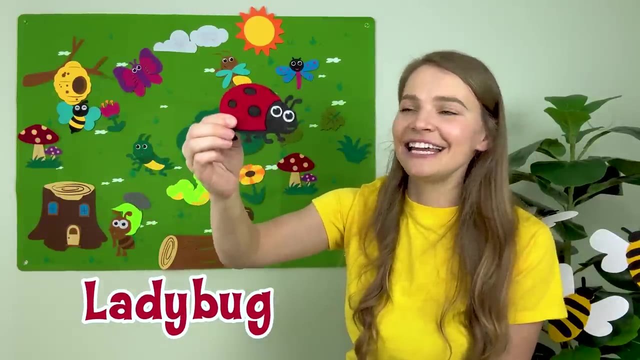 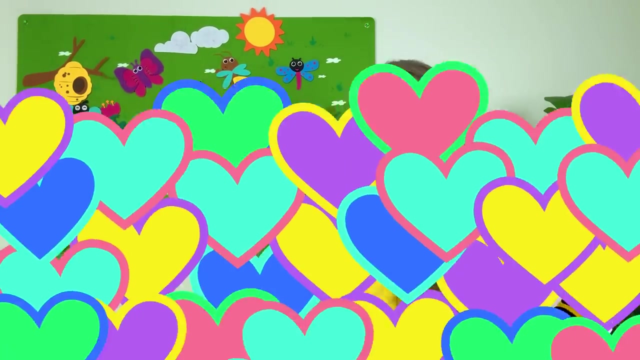 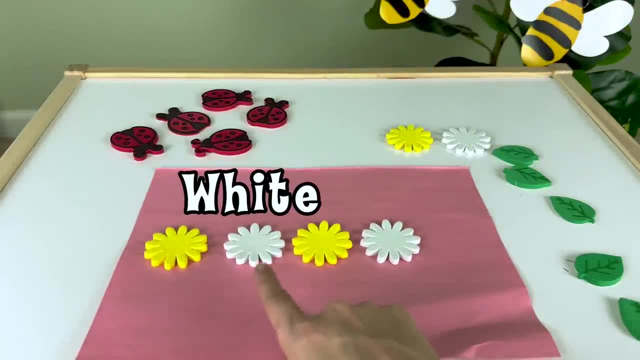 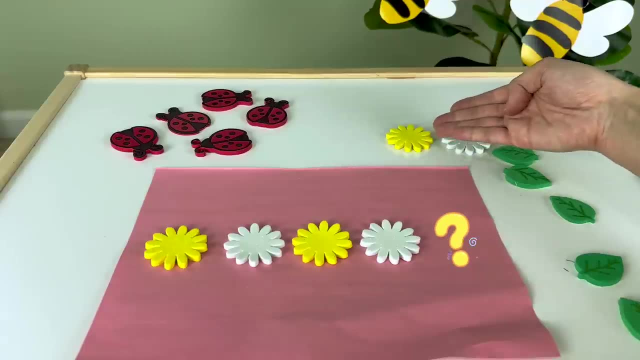 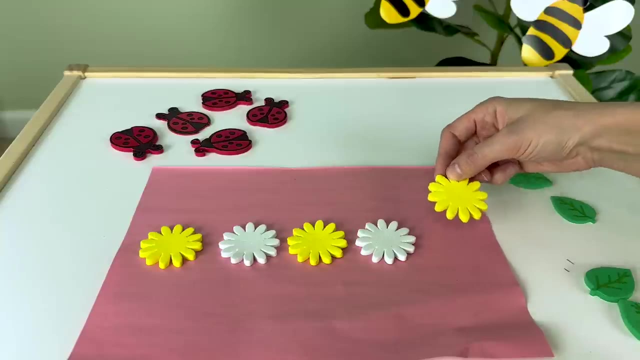 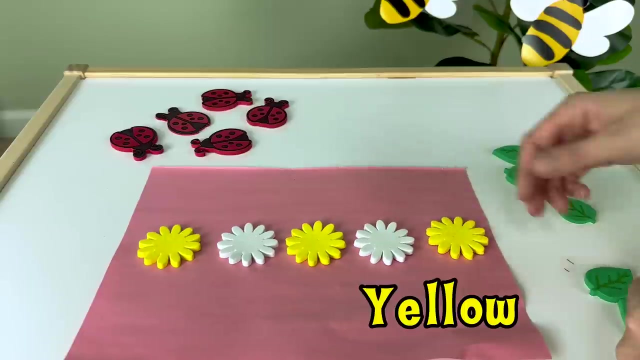 Oh, look, here is a ladybug. Hello friend, I'm a little ladybug, Hi ladybug, it's nice to meet you. flower, white flower. and which flower should go next? yellow or white? hmm, white or yellow? let's see. yellow, white, yellow, white, yellow. all right, thank you. now let's add some leaves, one leaf. 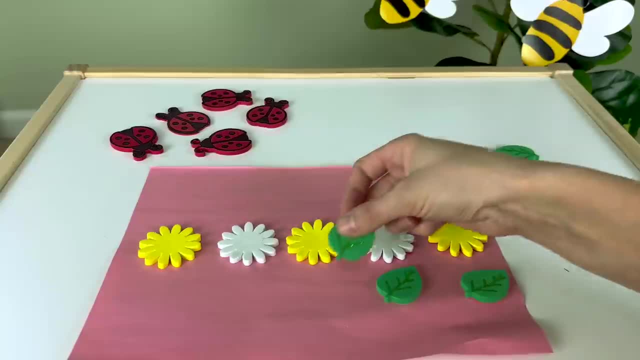 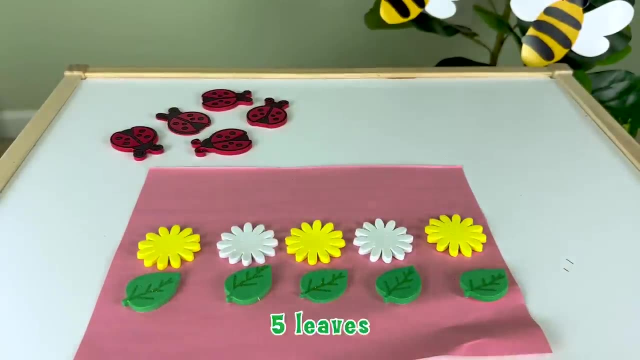 two leaves, three leaves, four leaves, five leaves, five leaves and five flowers. now let's add some ladybugs. oh, i'm looking for a flower. have you seen one? yeah, ladybug, here's a yellow one. yum, yum, yum. this ladybug says hello, hello. i would like a white flower, please. oh sure, right here, ladybug. 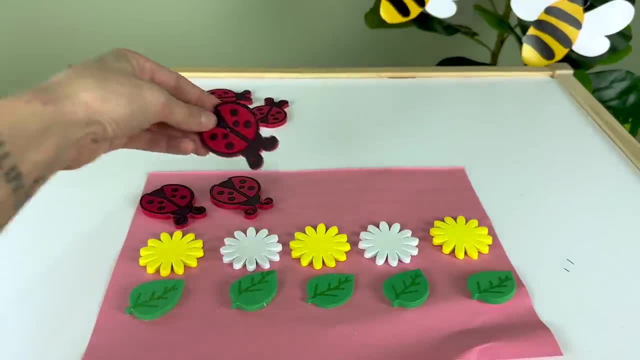 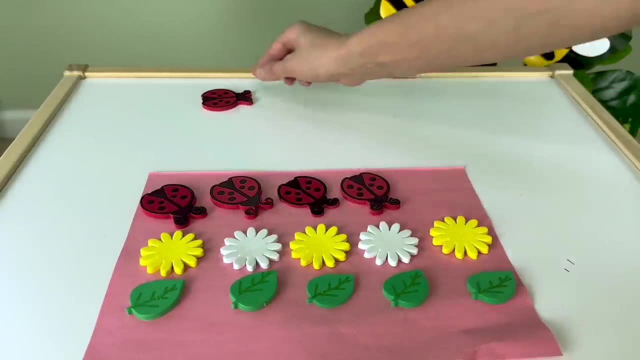 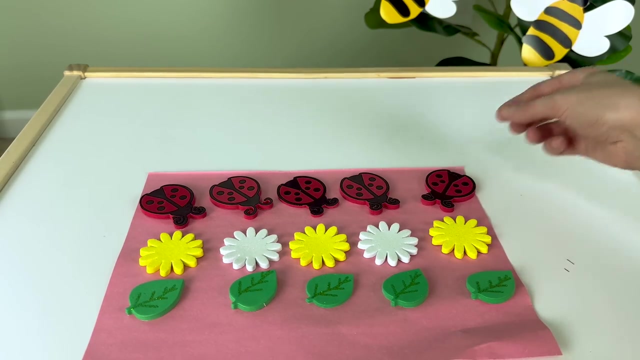 oh, hello, hello, hello, hello. i would like a yellow flower, please. here you go, ladybug. hello, hello, hello, hello. i would like a white flower, please. here you go, ladybug, hello, hello, hello. i would like a flower too, please, here you go, ladybug. here's one more for you. thank you for helping me. 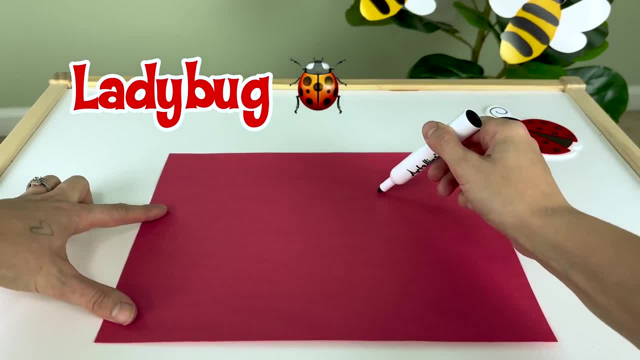 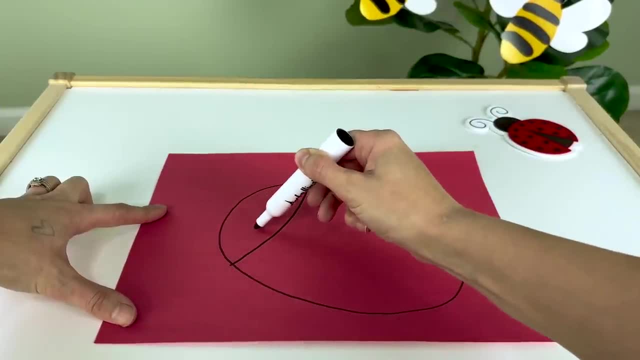 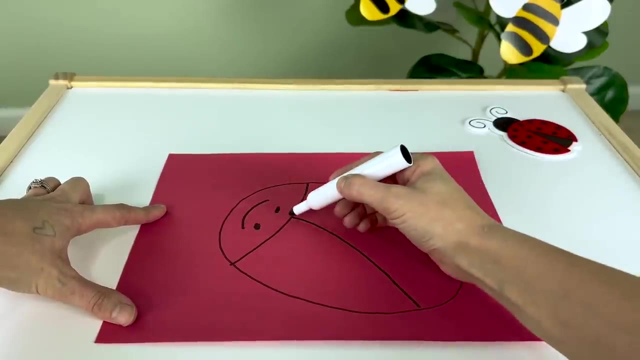 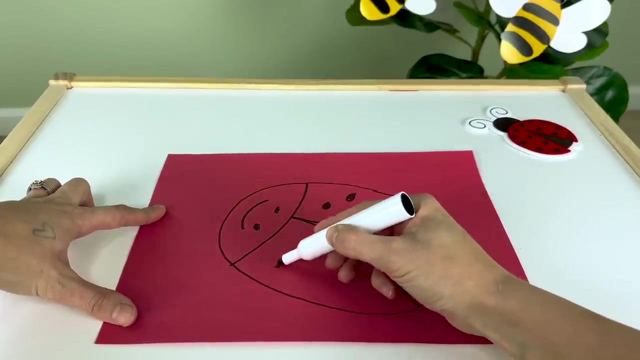 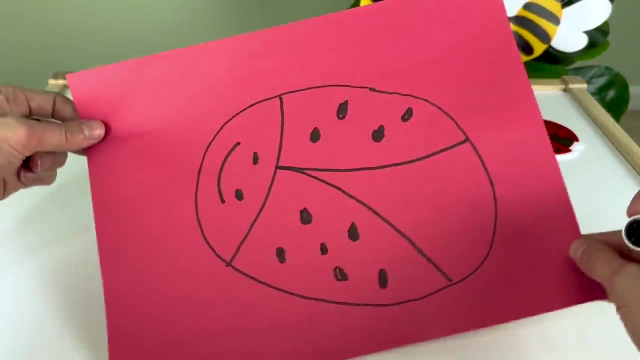 let's draw a ladybug together. draw an oval- more area for the face. i i come out, two wings and some boba cups and now we've got a little ladybug. ladybug says hello, let's draw a cute little bumblebee. we'll do an oval. 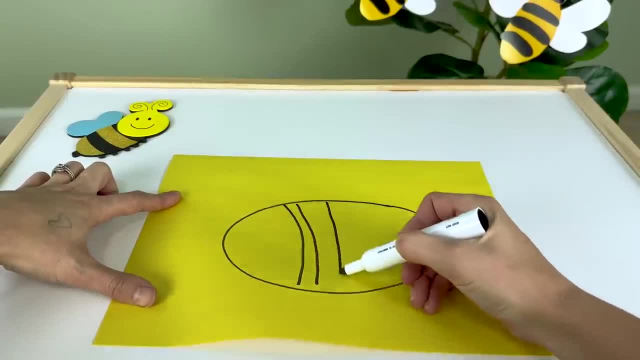 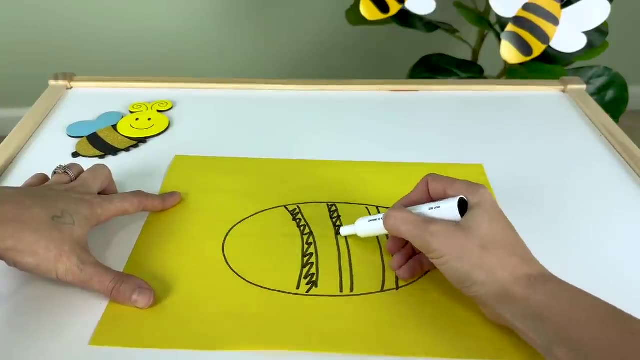 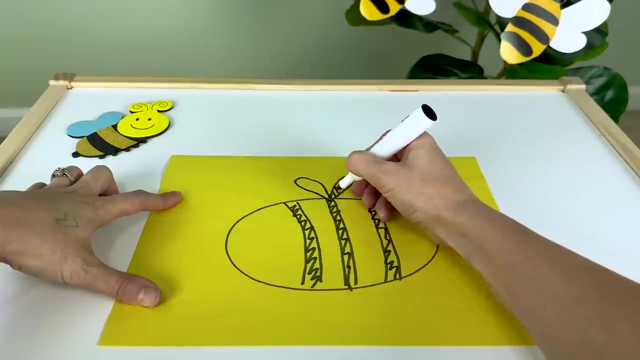 and some couple of more. lobster called: let's draw a little. let's draw a little yak and let's teach this ladybug to. i hear a alullah attitude. let's really guide the lady. Grub Br tonnes called: we'll look at the wings, we'll open. 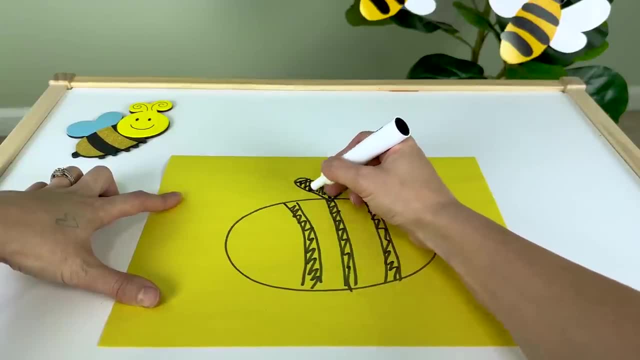 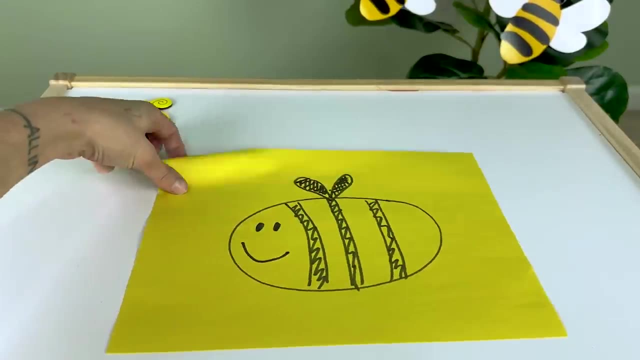 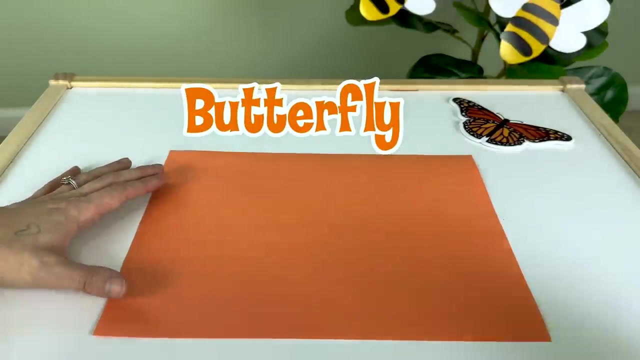 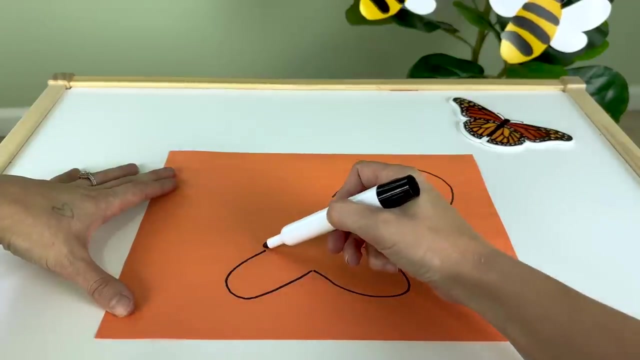 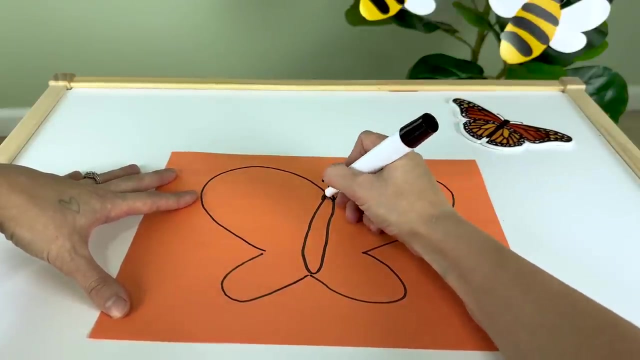 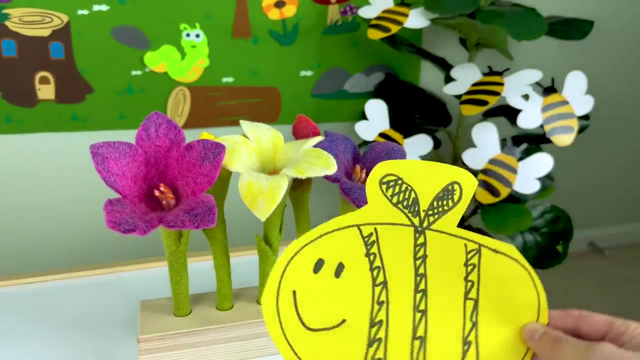 we'll open guide the, the listen ears, we'll take you go. oh my gosh, soap box. Let's draw a butterfly together. We'll do some wings. We'll draw a butterfly in the middle. Hello, butterfly, Bumblebee, bumblebee, bumblebee. 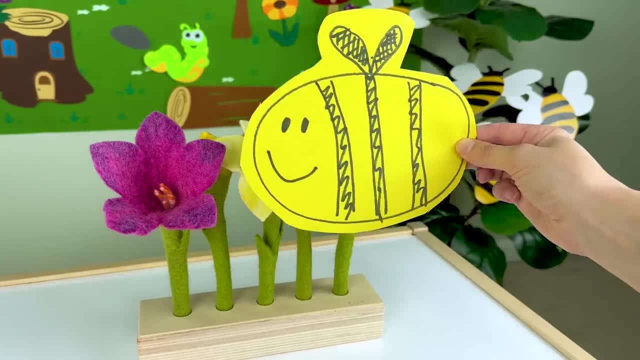 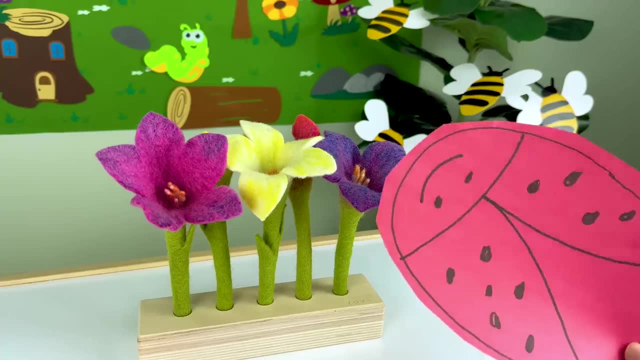 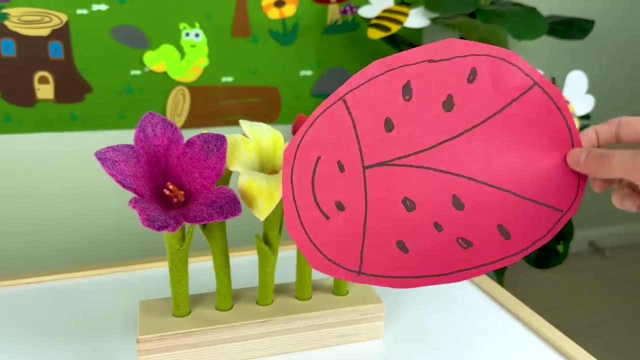 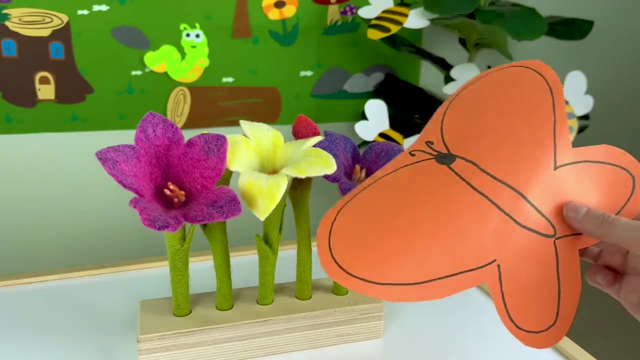 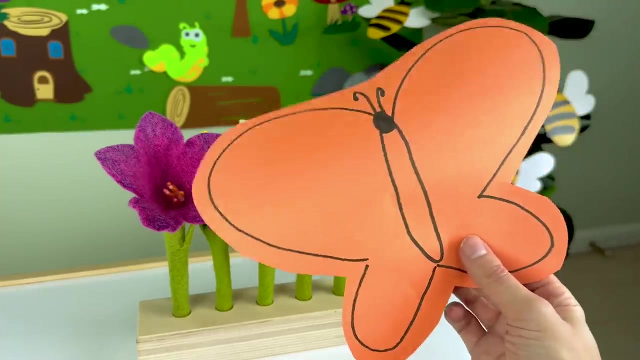 Bumblebee, bumblebee, bumblebee, Ladybug, ladybug, ladybug, Ladybug, ladybug, ladybug, Butterfly, butterfly, butterfly, Butterfly, butterfly, butterfly, Butter, butter, butter, butter, butterfly. 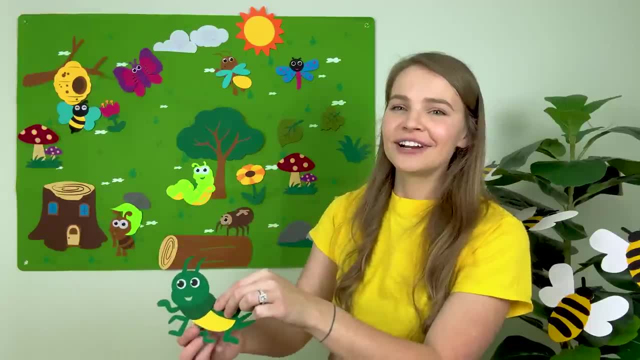 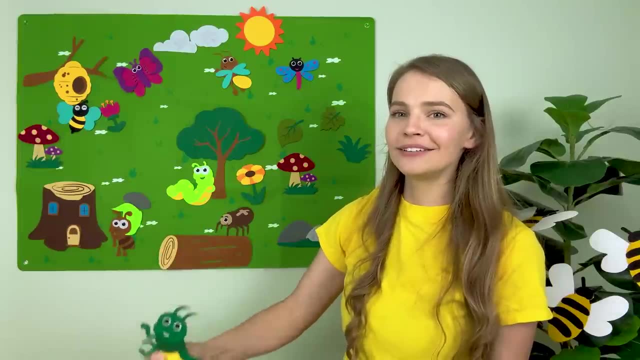 Hop, hop, hop, hop, hop. Hello friends, I am a little grasshopper, Hello grasshopper, And I like to hop, hop, hop around the grass. Hop, hop, hop around the grass. Wow, so nice to meet you little grasshopper. 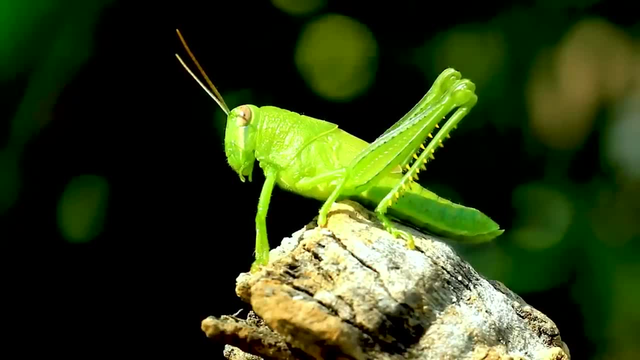 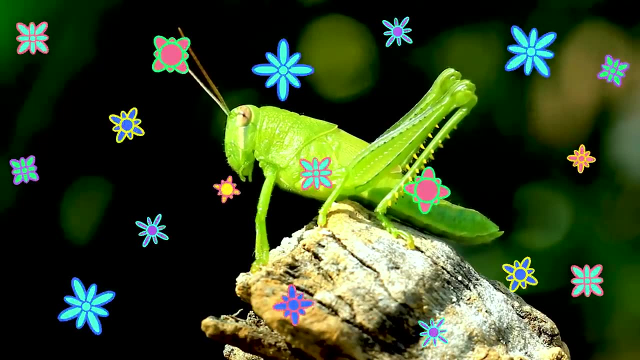 Here you go. You can go hopping in the grass, And I like to hop around the grass, I like to hop around the grass And I like to hop around the grass. Here's the butterfly that we drew, And the butterfly says thank you, thank you for drawing me. 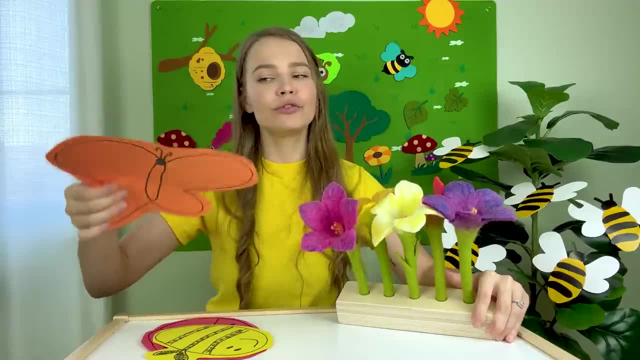 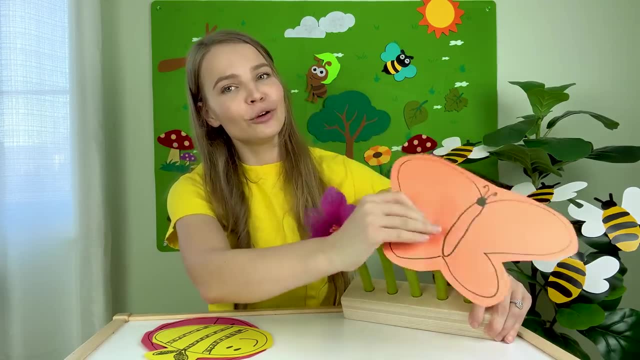 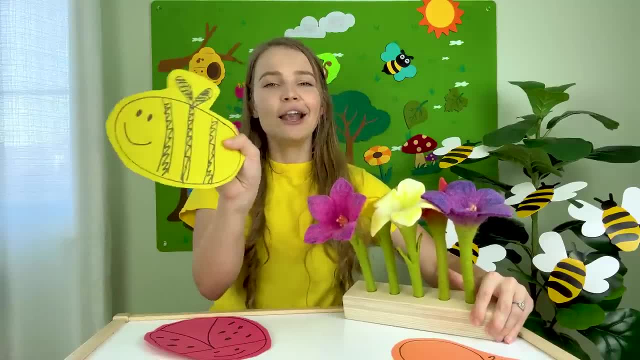 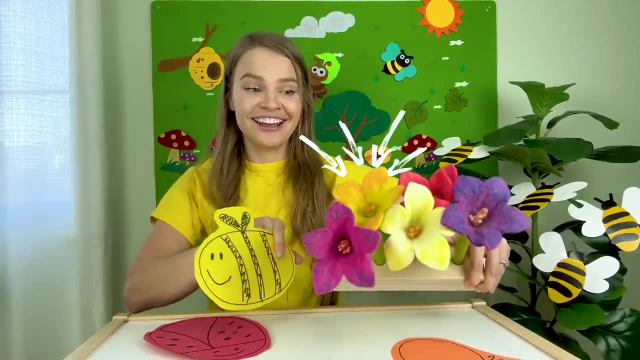 Here's our bumblebee: Bzz, bzz, bzz, bzz, bzz. Hello friends, I am looking for a yellow flower. Bzz, bzz, bzz, bzz, bzz. Do you see a yellow flower? 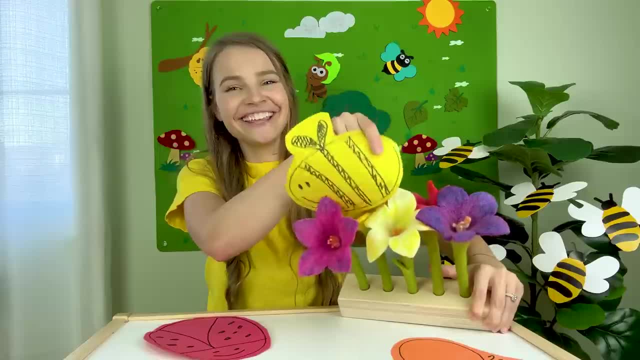 Right here, Here you go, bumblebee. Yum, yum, yum, yum, yum, yum yum, Thank you, thank you. Here's a ladybug. Oh, hello, hello, I'm looking for a red flower. 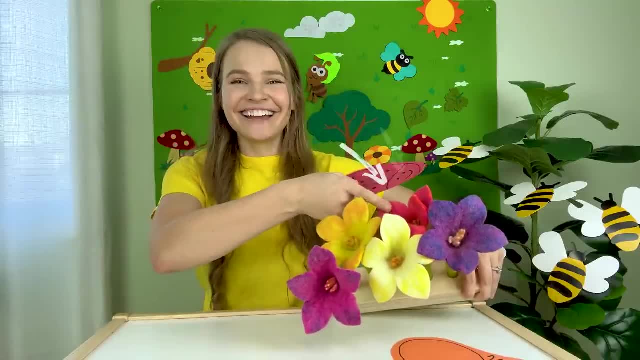 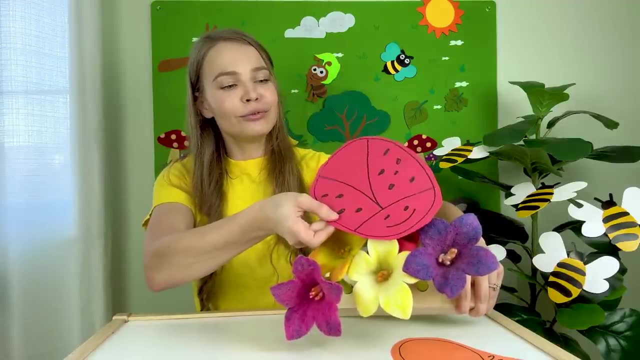 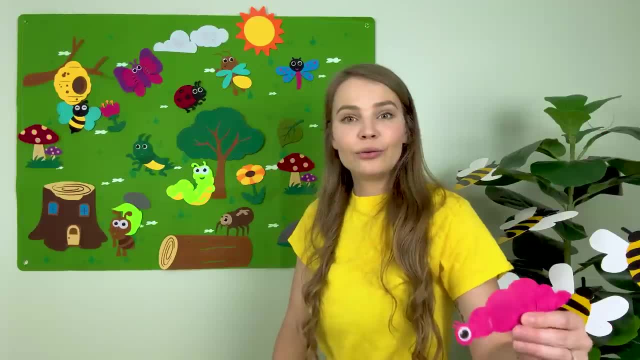 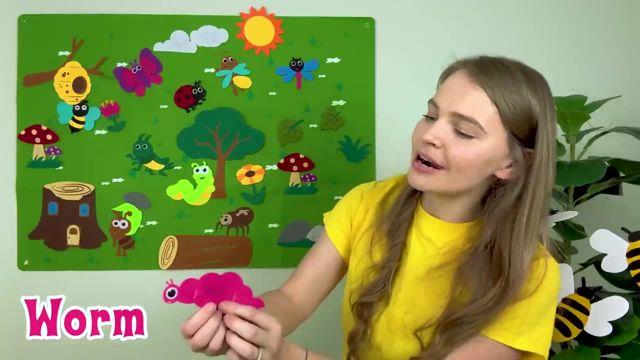 Thank you, thank you, Wake up, wake up, wake up. Wiggle, wiggle, wiggle, wiggle, wiggle, wiggle. Hello, little worm. Hello, I'm a tiny little pink worm And I like to go wiggle, wiggle, wiggle wiggle. 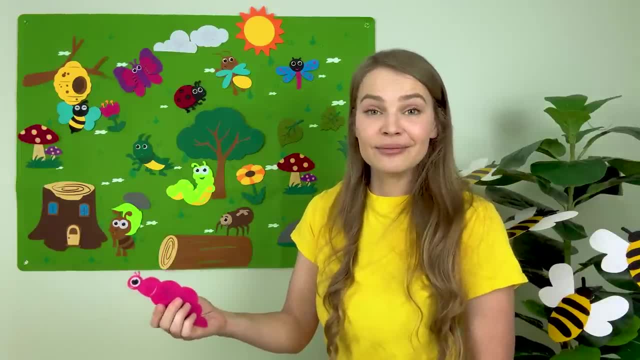 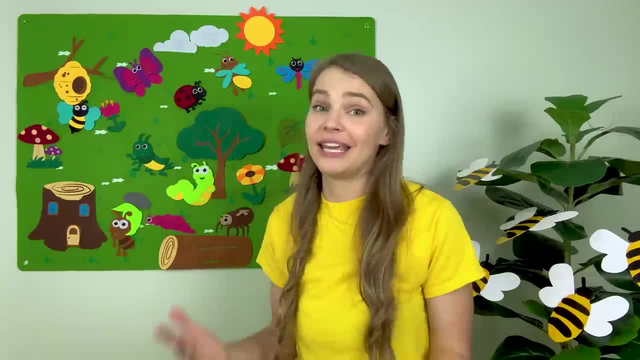 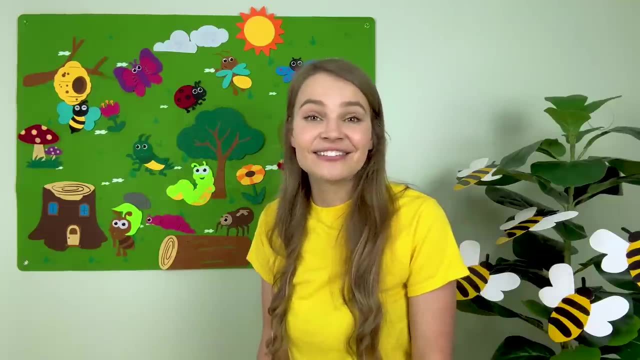 Wow, This was so much fun. Thank you so much for playing with me and helping me learn about all of the different bugs. You're such a great friend and I love playing with you. Well, that's the end of this video. 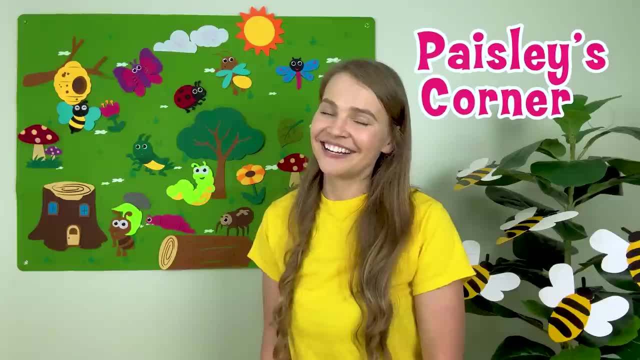 But if you're looking for more of our videos, make sure you search for Bailey's Corner with Silly, Miss Silly, And I'll see you then. Bye-bye, Bye-bye.